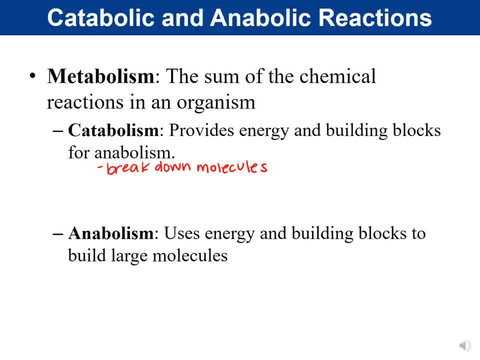 break something down, what type of reaction is that? Is that going to be hydrolysis or dehydration? And remember back to our reactions in lab. If we're looking at if an organism metabolizes a particular substrate, what type of reaction were we talking about? And the answer is: we talked about hydrolysis. 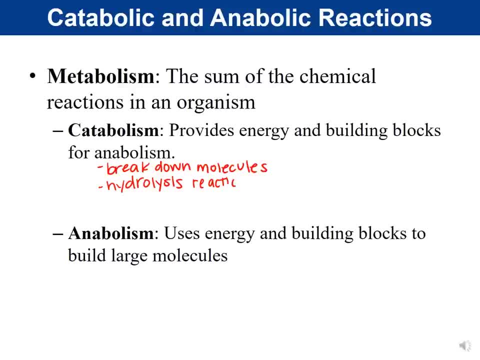 reactions. So we looked at starch hydrolysis, right. We looked at casein hydrolysis. We talked about lots of different reactions and remember that hydro water lysis is breaking, So using water to break apart these substrates. So 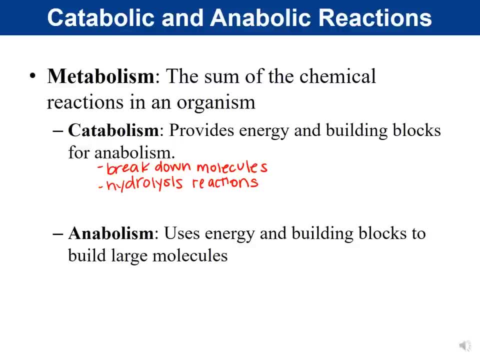 we're going to be using hydrolysis reactions, we're going to be breaking down molecules. So we're starting with something bigger and we're going to be breaking down molecules. So we're starting with something bigger and we're breaking it down into smaller parts Now in terms of energy. so, if you 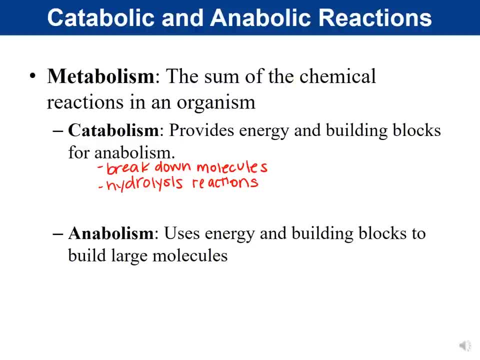 think about building something or breaking it down, right? So if we compare building something versus breaking it down, imagine I'm building a tower with blocks. Which one is going to require the input of energy? Which one are we going to have to put energy in to do To build the tower or to break it down? And the 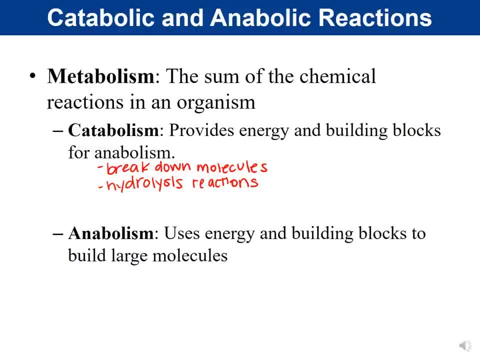 answer is: we have to put in energy to build the tower When we break it down, like in the casein hydrolysis. we're going to have to put in energy to build the tower When we break it down, like in the casein. 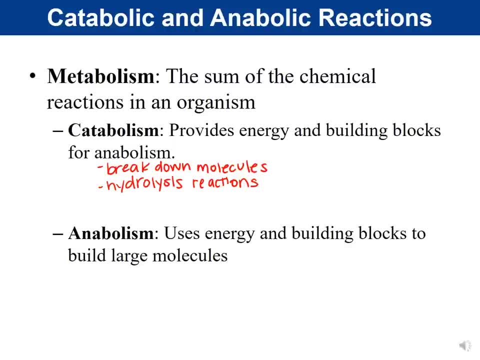 like in the casein catabolism, when we break down molecules we release the energy that's stored in those bonds. So we call these types of reactions exergonic. so exergonic reactions, energy is released. So the energy that's stored in that bond that's holding that molecule together is a. 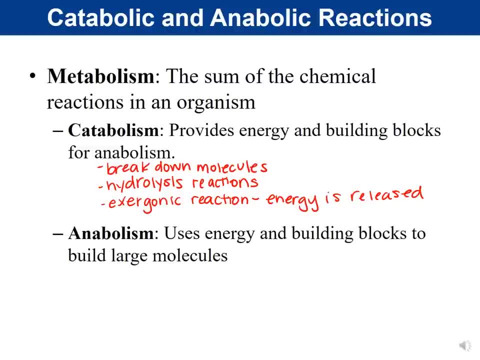 energy that's stored in that bond that's holding that molecule together. when we break that bond, we're going to release energy, And so, again, this is why we call that exergonic- Think of energy exits, So energy is released when we break. 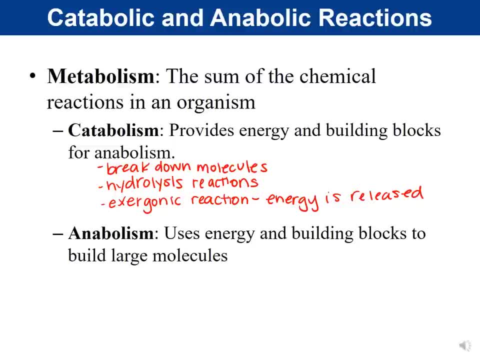 things down, And so the purpose of catabolism is that it's used to provide energy and building blocks for what's called anabolism, which is going to be to build stuff up. So these types of reactions are going to be coupled with one another. These catabolic reactions, these reactions. 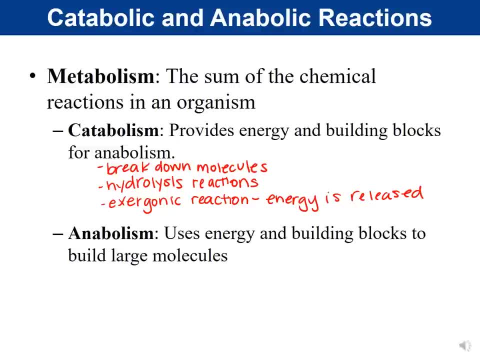 that break things down are going to be used to help build other things up, And we'll talk more about that in just a minute. So if we talk about anabolism, when we think about that, the way that I remember this one is that catabolism it's a catastrophe. It all falls. 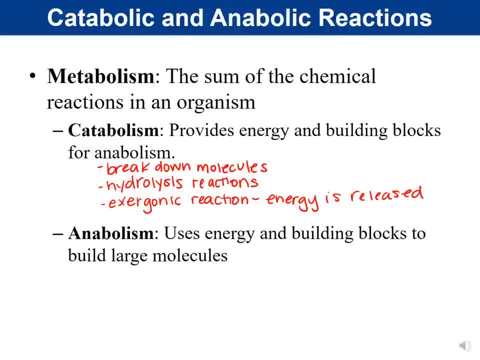 apart Anabolism, the way I remember that one is, I think, about anabolic steroids. So if an athlete is taking anabolic steroids, for example, what is that athlete trying to do? Well, it's trying to build muscles. So this is used to build molecules. 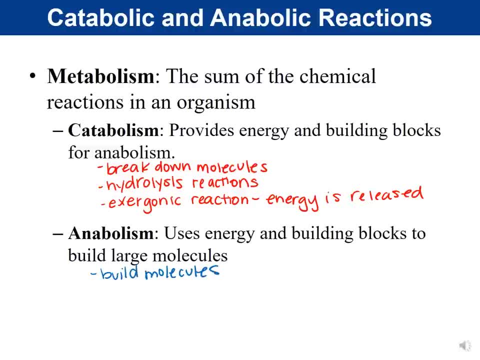 So catabolism is breaking them down. Anabolism is building them up right And again, just like anabolic steroids would be to build muscles. Anabolism is referring to building molecules. So catabolism is breaking them down, Anabolism is building them up right And again. just like anabolic steroids would be to build muscles. So catabolism is breaking them down, Anabolism is breaking them down. Anabolism is building them up right And again, just like anabolic steroids, is breaking them down. Anabolism is breaking them down. Anabolism is breaking them down. Now, if we are 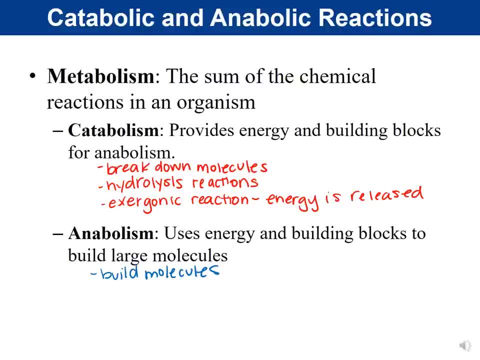 synthesizing macromolecules. is that hydrolysis or dehydration? And the answer is dehydration. So, for example, if we were building a protein, for example, and we were linking amino acids together, that would be an example of a dehydration reaction. We have to remove water in order to form that bond. 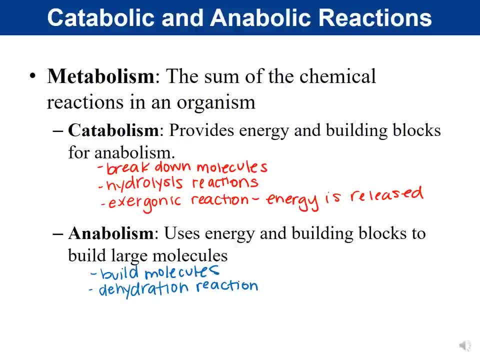 between the amino acids. Now, if we're building something, these types of reactions are going to be endergonic, So it's an endergonic reaction. Energy must be put in, Energy has to be invested in order for this reaction to occur. 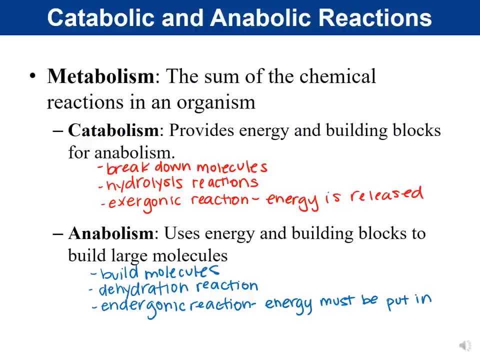 And so this would be an endergonic Think of. in Endergonic, energy must be put in, And so in anabolism, it's going to use the energy in the building blocks that come from catabolism to then. 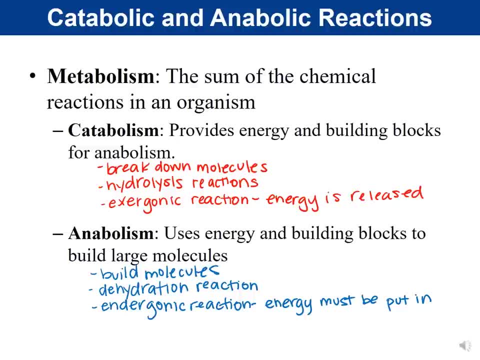 build large molecules, And so a good example for you to think about for this is if you think about protein metabolism. right, Organisms get their source of nitrogen. many of them take in nitrogen in the form of proteins. Right, They decompose proteins, So they are going to metabolize, They're going to break down through. 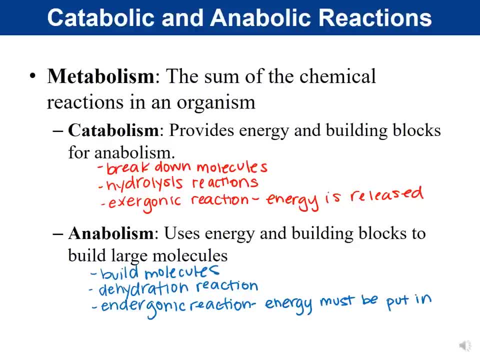 catabolism They're going to break down that protein. When those building blocks get released, then in anabolism we're going to use those building blocks and the cells and the organisms are going to use it to make their own proteins, for example, And so these reactions are going to be coupled. 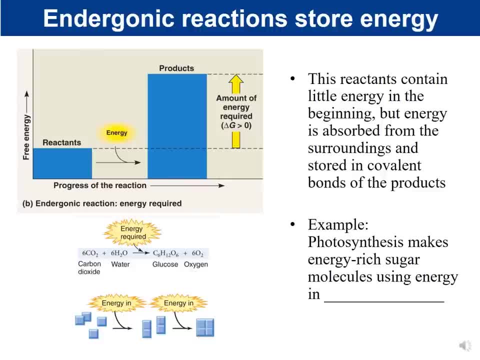 One reaction helps the other, the other. So if we look at endergonic reactions or exergonic reactions, again endergonic means we put in energy. Endergonic reactions are used to build stuff. So what you're looking at on the top, 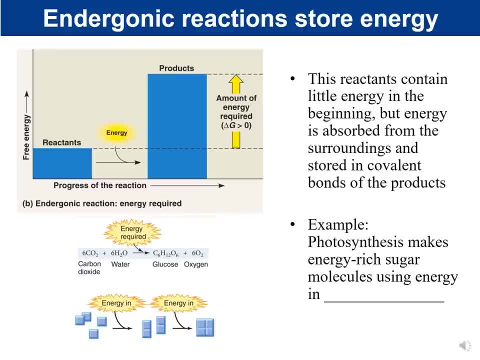 is. you're looking at an energy diagram And so notice that we have our reactants, That is what's going in And our products are what are coming out, And notice that on the y-axis we have an increase in free energy. So in an endergonic reaction our reactants start with very little. 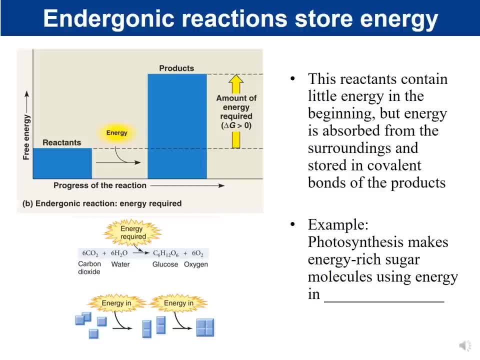 energy. Energy must be put in And we get products notice that have a much higher amount of energy, And that's because the energy that's provided is going to be used to help build those molecules. A good example of an endergonic reaction would be photosynthesis In photosynthesis. 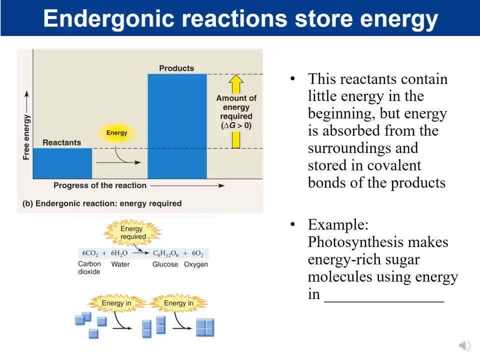 plants or algae or, in some cases, bacteria, will take carbon dioxide water and they will build. So they're going to link carbon dioxides together and they're going to build glucose. So that again is endergonic right, Because we're taking 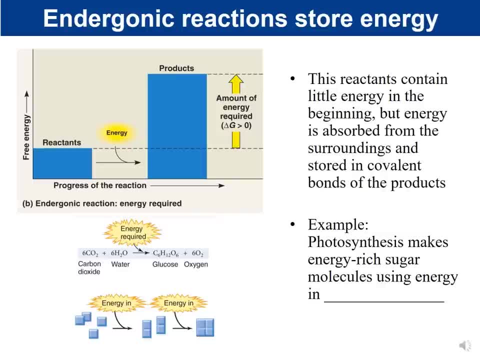 this carbon dioxide, and we're building glucose. Energy must be put in in order to make the glucose. What is our source of energy in the case of photosynthesis? And the answer is sunlight. So energy in the form of sunlight is going to be used to build sugars, And so, again, 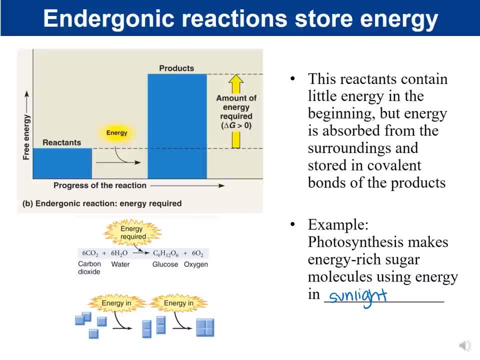 this type of reaction is going to be endergonic. Energy has to be put in in order to build that sugar, And then that energy is going to be stored in that sugar And so when animals, for example, come along and they eat the plant, they're able to take that stored energy in the plant. 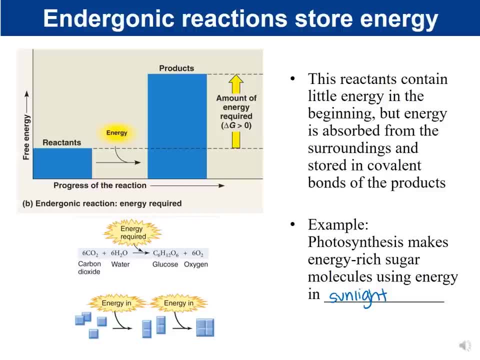 and then break that down, And when they do, they release that energy. So endergonic reactions require the input of energy. Our products have more energy than the reactants right. Glucose contains more energy than carbon dioxide. Exergonic reactions, on the other hand, 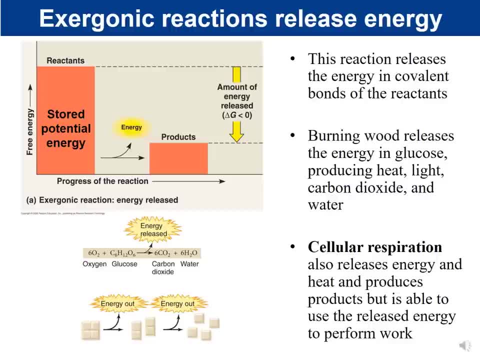 exergonic reactions release energy. So again, energy is going to exit. So if I look at my reactants, what goes in has a lot of energy And it's energy that's stored in those chemical bonds When those reactants are. 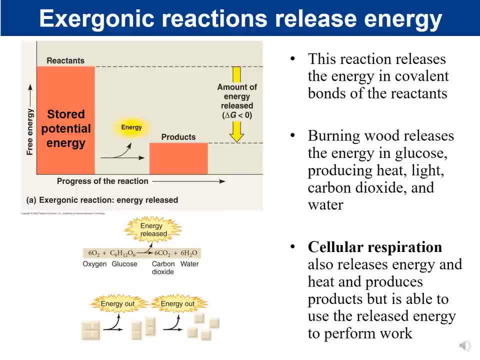 broken down, they're going to release energy And our products have less energy than the reactants. Now, when we talk about potential energy, so when we talk about types of energy, we have potential energy, Which is stored energy, And we have kinetic energy, which is the energy of motion. So in the case of 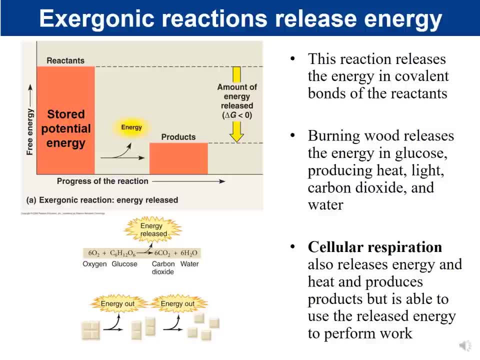 these exergonic reactions. one of your questions asks which type of reaction requires high potential energy, Which one requires high potential energy. And you have to be careful with that type of question because, yes, endergonic reactions require energy to be put. 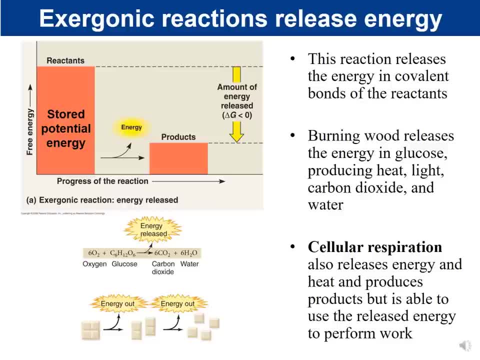 in. But in the case of these exergonic reactions, which type of reaction requires high potential energy? But the question is not asking you that. It's asking you which type of reaction requires high potential energy. Potential energy is stored energy. That is going to be the exergonic reactions. 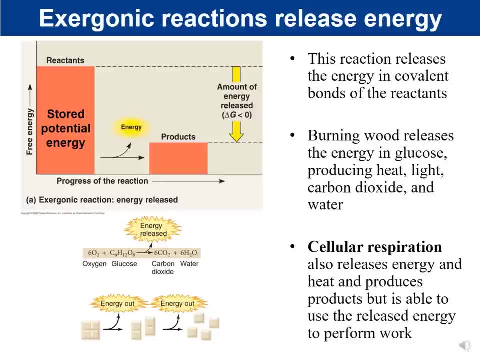 because it has energy stored in those bonds. When we break it down, that energy gets released and our products have less energy than our reactants. So be careful if we're talking about energy. what type of energy, right? Endergonic reactions require energy to be put in. Exergonic reactions require potential energy. 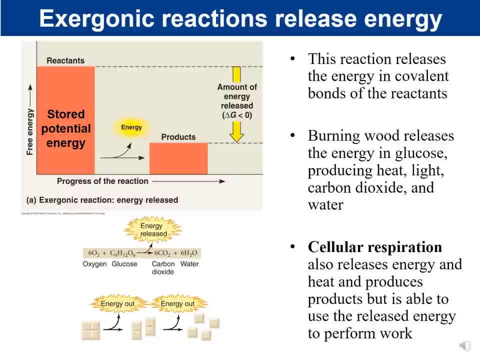 They have to have energy stored. An example of an exergonic reaction would be cellular respiration, And so notice that, if you look at the bottom, cellular respiration is essentially the opposite of photosynthesis. So our reactants in this case are oxygen, O2, and glucose. And so when we eat, 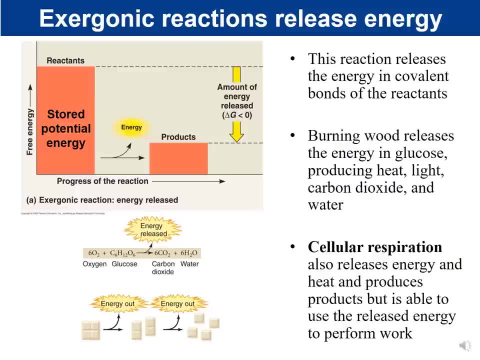 we are going to metabolize our food. We're going to break it down. So glucose is higher energy than my product, which is carbon dioxide, And so during the process of breaking that glucose down, the energy released from the glucose is used to produce ATP for the cell. 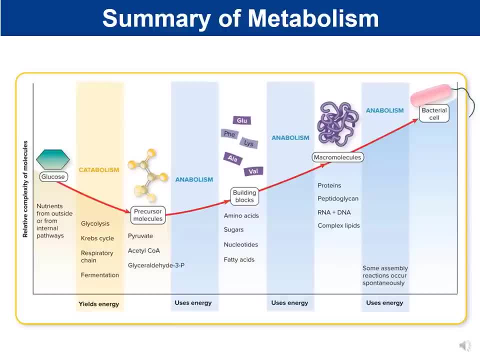 And ATP is cellular energy. So this slide is just kind of summarizing metabolism and how all these parts are interconnected. Interconnected at when we eat food, for example, or when a bacterial cell takes in food. right, So they're going to take their nutrients, so our glucose or our proteins, et cetera. 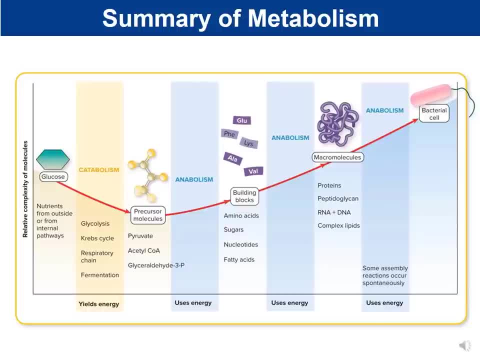 and they're going to take those food sources and they're going to undergo catabolism. They're going to break down that glucose. So, in terms of catabolism, it's going to break down the glucose using glycolysis, the Krebs. 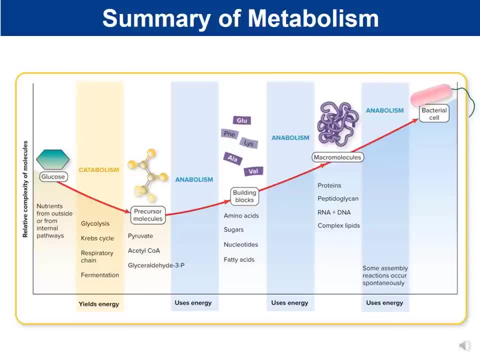 cycle, the electron transport chain, fermentation, et cetera, And so it's going to break down that sugar and it's going to produce various precursor molecules. So in the case of glycolysis, it's going to produce pyruvate. 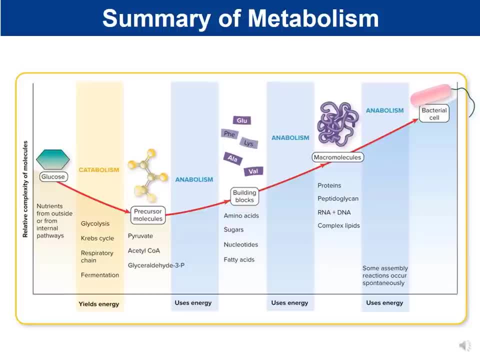 We have glyceraldehyde 3-phosphate, We have acetyl-CoA, which forms in a transition step, et cetera. So as we break down these pre- as we break down our food, we are going to produce these precursors. 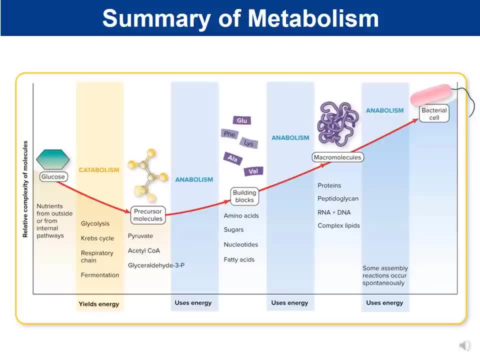 When we break down our food, we're going to release energy that's stored in that food. So, again, those reactions are going to be catabolism, They're going to produce energy. Those precursors are then used to build building blocks. 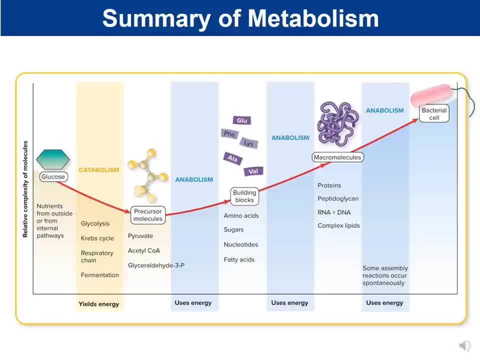 So those precursors are going to be used to make amino acids, to make carbohydrates, to make nucleotides, to make fatty acids. so the building blocks, the monomers that are going to be needed to make our polymers, If we're taking our precursors and we're converting them into building blocks again, endergonic. 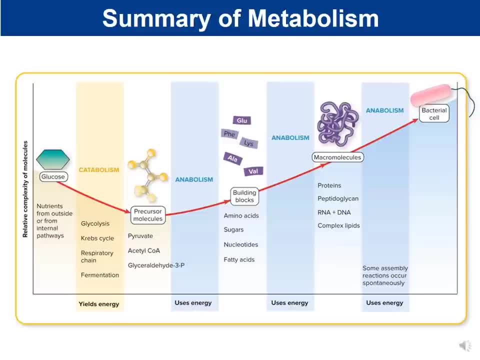 right, it's anabolism. We have to put in energy to build those. Then we take those monomers or those building blocks and we put them together and we form our macromolecules, So our proteins, our peptidoglycan, if we're talking about bacteria. 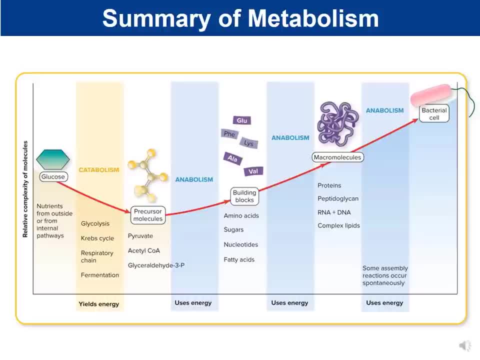 Our DNA and RNA, Our lipids, etc. Again, that's anabolism, because we're building up macromolecules And then, lastly, we have to put those macromolecules together in those structures and that will form our bacterial cell. 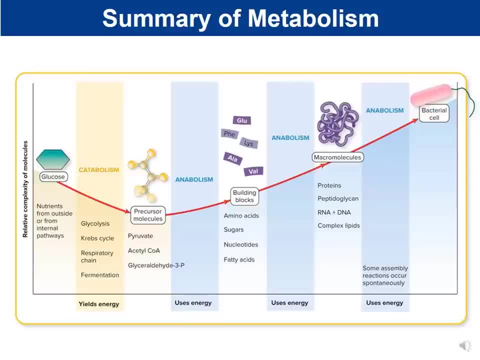 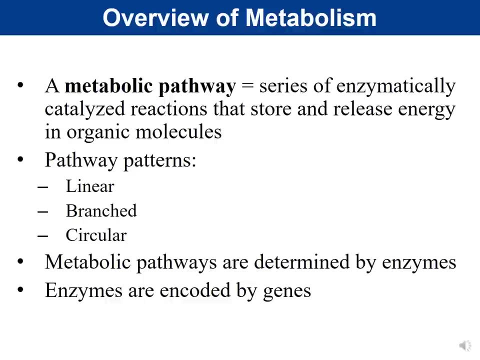 And so again, metabolism is going to be the sum of its parts, So it's both the anabolic reactions and the catabolic reactions put together. So if we talk about a metabolic pathway, So if we talk about a metabolic pathway, what we're referring to is a series of enzymatically 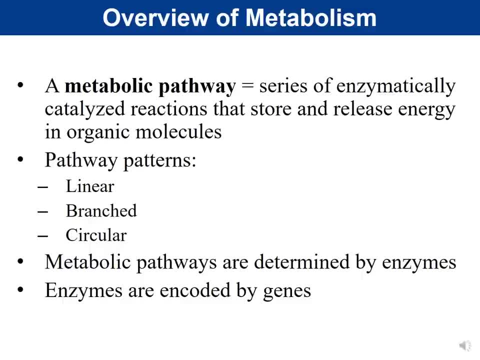 catalyzed reactions that store and release energy in organic molecules. So it's this group of reactions that happen in the cell, And so if we talk about types of patterns or types of pathways that we can have, we can have what we call a linear pathway. 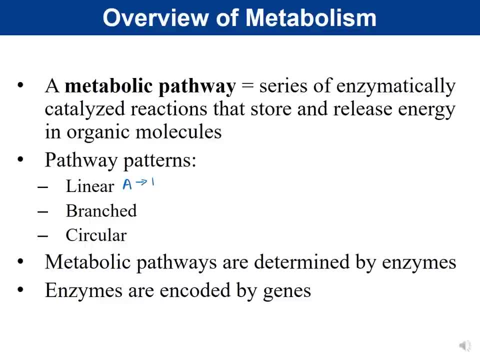 And that is: A goes to B, B goes to C, So that's linear. This breaks down to this, which breaks down to this. An example of this would be starch hydrolysis, And so starch gets broken down to maltose. 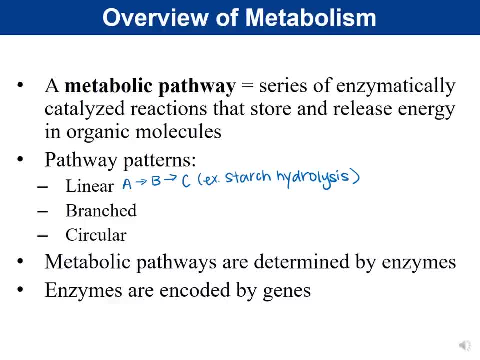 Starch is a polysaccharide. Maltose is a disaccharide. Maltose then gets broken down to glucose, which is a monosaccharide. That's a linear pathway. Starch gets broken down to maltose. 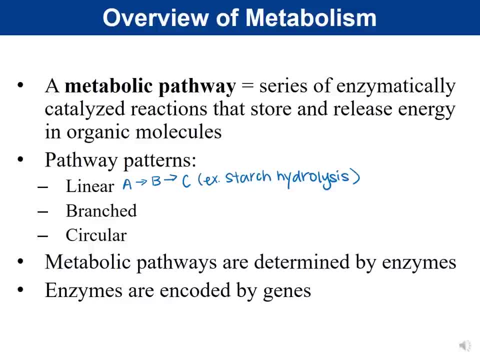 Maltose gets broken down into glucose. That's a linear pathway. Now, not all pathways are linear. Some pathways are branched, And what that means is that A can go to B or C. There's a branch in this pathway. An example of this would be oxidation versus fermentation. 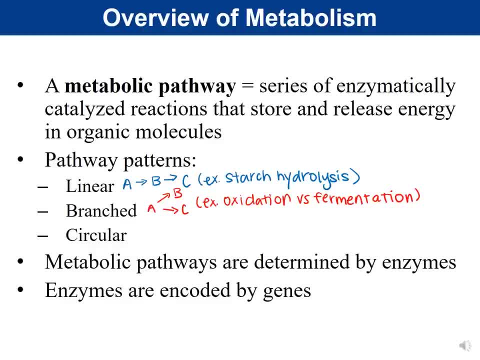 And so we talked about this when we talked about our OF test, our oxidation and fermentation test. And so both types of metabolism, both oxidation and fermentation, both use glycolysis, They're both going to take that 6-carbohydrate. 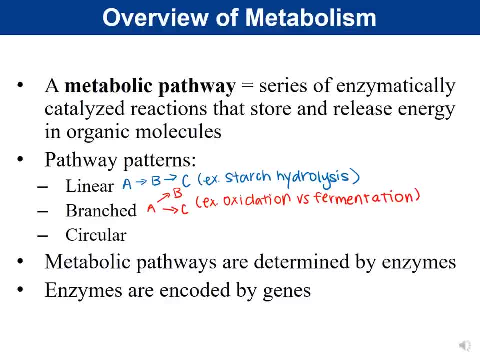 So they're going to take that 6-carbohydrate. They're going to take that 6-carbohydrate and break it down into pyruvate. Now the branching comes in after the pyruvate, So the A would be representative of pyruvate. 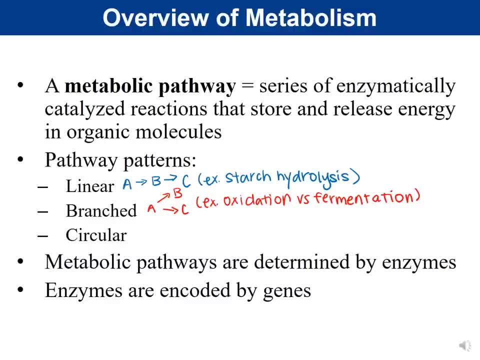 If O2 is available, pyruvate is going to go through oxidation, So it's going to go into the Krebs cycle and then the electron transport chain. If, however, O2 is not available, if there's no O2, we're not going to go through oxidation. 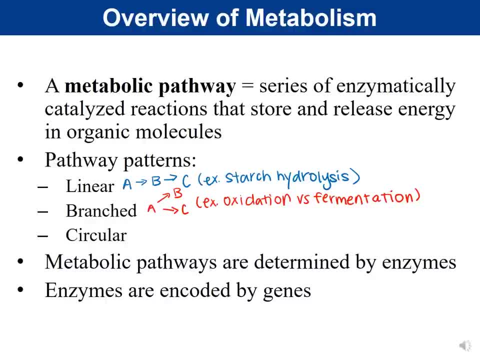 but instead we're going to go through fermentation, fermentation, And so that's C right? So pyruvate kind of acts as this key branching point between whether the cell does oxidation or whether the cell does fermentation, And then lastly, 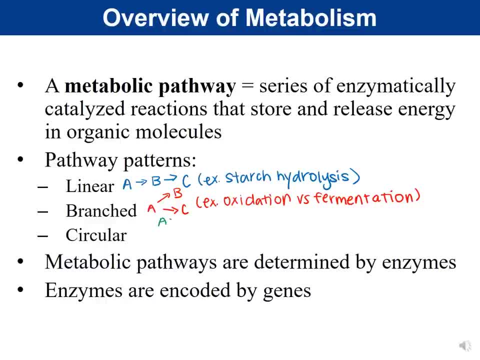 the last type of pattern that we can have is: A goes to B, B goes to C and C goes back to A. It's a circular pathway. An example of this would be the Krebs cycle, which you're going to see in this chapter. It's a circular pathway, right? It's cyclical. 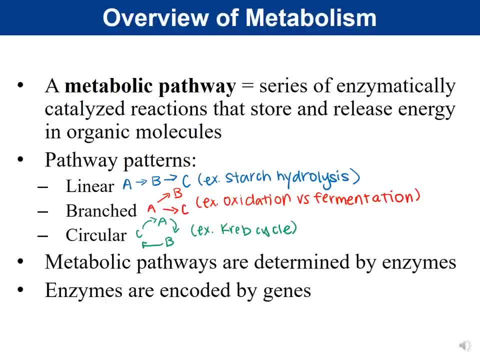 So it's going to produce a circle. Now in lab we've been doing our biochemical tests right, And in our biochemical tests we are looking for if bacteria can do a particular chemical reaction. And remember that what that really means essentially is we're testing if 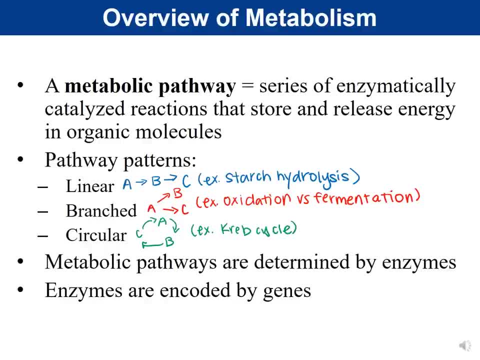 bacteria can do a particular chemical reaction, And remember that what that really means essentially is we're testing if bacteria can do a particular chemical reaction, So like if we talk about our urease test, urea is the substrate and we're testing if bacteria 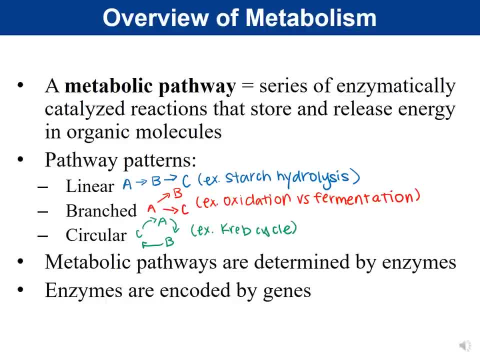 produce urease. If they make that enzyme, they are able to do that reaction, And so those metabolic pathways are determined by what enzymes an organism produces. If they produce that enzyme they can do that metabolic pathway. If they don't produce that enzyme, 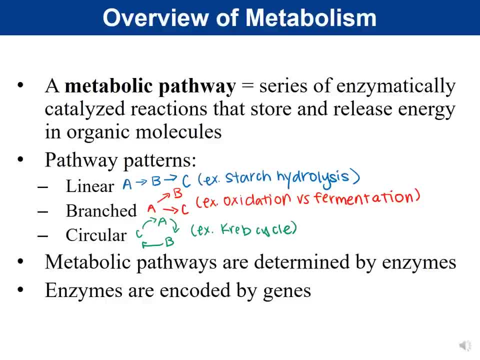 they cannot. Now, how is it determined if bacteria have that enzyme? Enzymes are proteins, right? Proteins are encoded for by the DNA. So what determines whether or not an organism can do a particular pathway is it's actually looking at? do bacteria have that gene? Do they have that DNA? 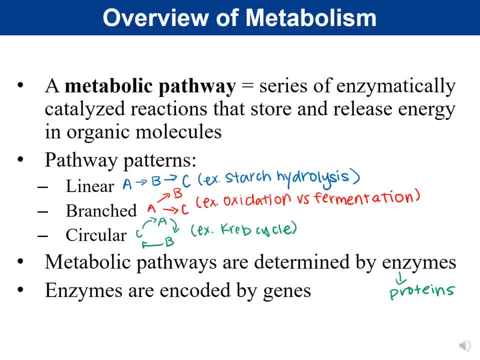 sequence that codes for that gene, And so what we're looking for is a particular pathway, And so the jot in the Untersign-. você precisamo sempre identificar onde a chemical reaction can be made, that enzyme, If they do, if they have that gene and they produce that enzyme. 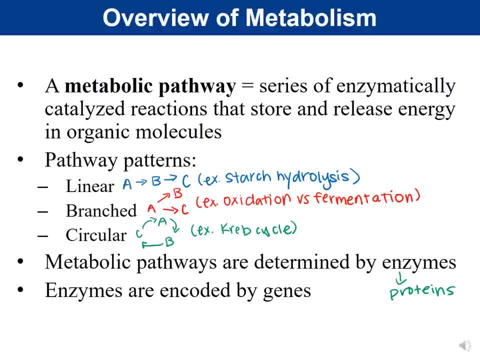 they can do that chemical reaction. So a good example to think about for this is fermentation. Fermentation: there are two main types. There is alcoholic fermentation, which produces alcohol, and there is lactic acid fermentation- Our cells in our body do. our muscle cells do lactic acid fermentation, El cell us bícondo não faz fermentação de lácteos, Então a capa é o ligume de creme. Então, quando você faz fermentação de expectations after reduction of Olivetinspires na Commeça, Luismos, the Polish mouve athlete, fermenteipM Brazil. 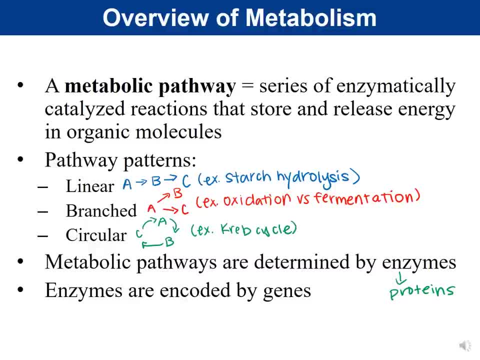 So if you're exercising very heavily and you're not getting enough O2, your cells are temporarily going to switch over to fermentation because they're not getting enough oxygen. Now yeast have the ability to do, and some bacteria can do, alcoholic fermentation. 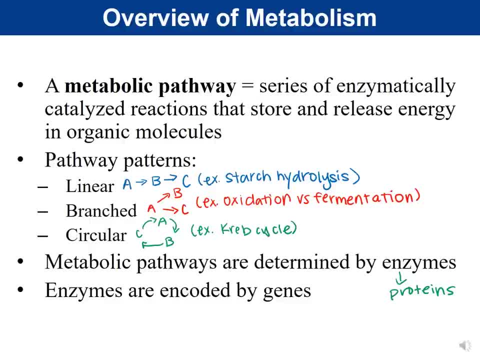 And what that means is that they still form their pyruvate, but when O2 is not available, they're going to take that pyruvate and they're going to produce alcohol. They're going to produce alcohol, And so this is why yeast is used to make beer, bread, wine, etc. 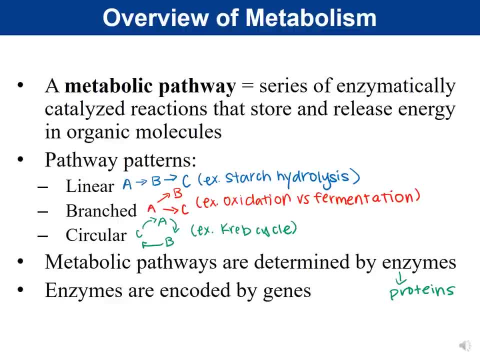 So, if you think about it, why do yeast do alcoholic fermentation and we don't? The answer is the yeast have the enzymes to do that metabolic pathway. We don't. We don't make those genes. therefore we don't make those enzymes. 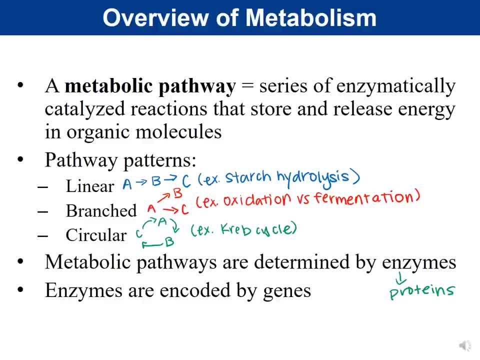 And our cells don't do alcoholic fermentation right? If so, people would be potentially holding their breath if they had a rough day because they wanted to have some alcohol. Doesn't work that way, okay, Deprived of oxygen, our cells are not going to do alcoholic fermentation. 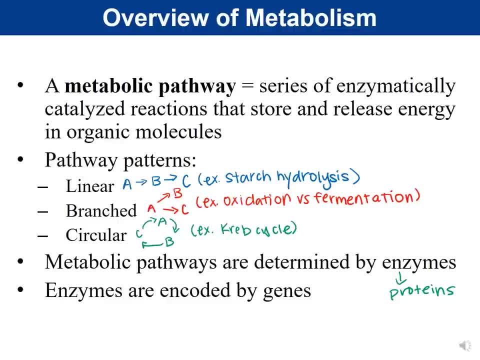 We lack those enzymes, We lack those genes to be able to do alcoholic fermentation. And so what dictates? What dictates if an organism can do a particular pathway has to do with its genetic code. What genes do they produce? And if they produce those genes, they produce those enzymes. 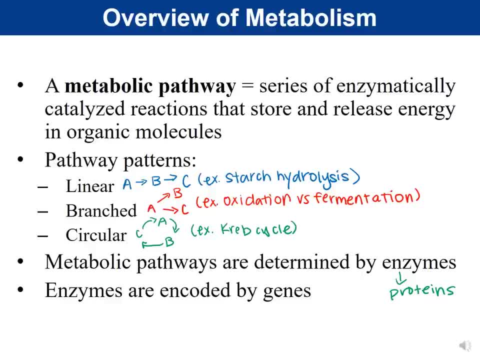 And if they make those enzymes, they can do those metabolic pathways. That's also why there are certain genetic conditions like, let's say, humans- for example I talked about in lab PKU phenylketonuria- And what happens is that people 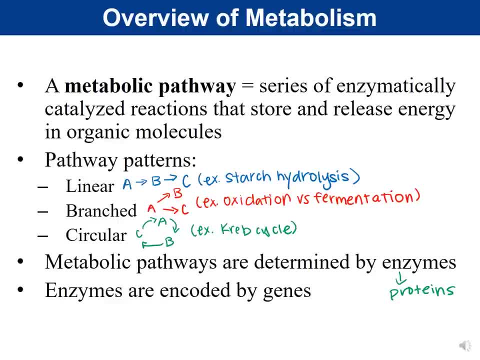 Who have PKU inherited two mutated copies of the gene that encodes for an enzyme to metabolize phenylalanine, And so they have a mutation in their DNA which then makes that enzyme not make properly. So the enzyme is not functional and therefore they cannot metabolize the substrate which 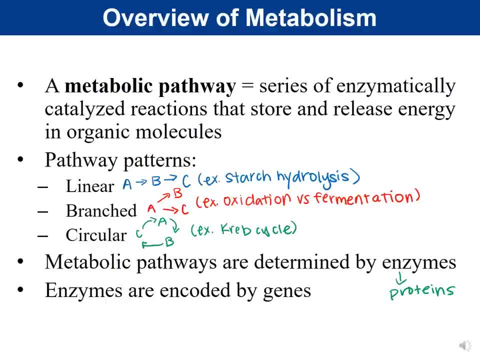 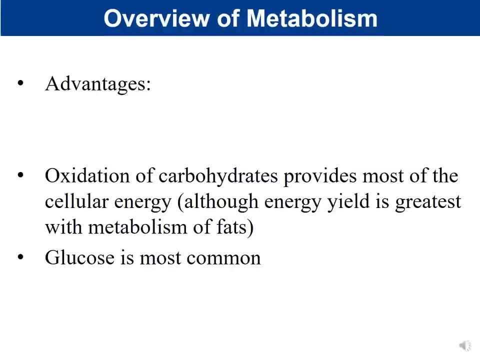 is phenylalanine. And so again, all of these metabolic pathways come down to: Do the organisms have phenylalanine? Do they have those genes? Do they have those genes, Do they produce those enzymes Which then will dictate if they can do a particular chemical reaction? 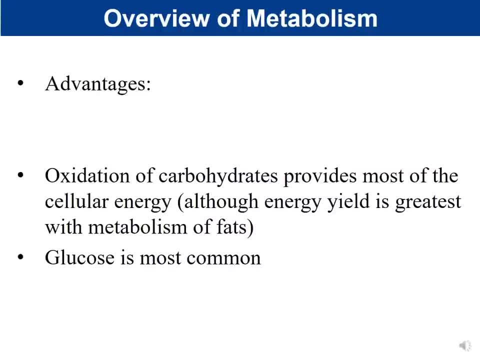 So if we look at an overview of metabolism and we talk about what is an advantage of doing metabolism, why do we build things and break them down, et cetera? so the advantage for this is that it allows for Concentration, Concentration. 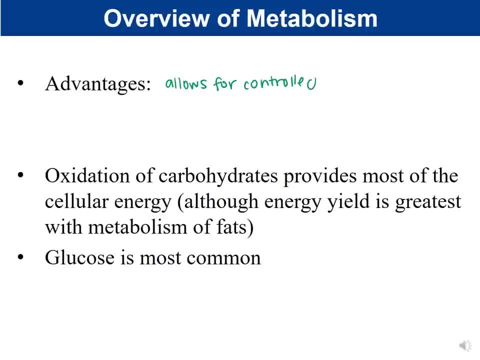 Concentration, Controlled storage and release of energy, often in the form of ATP. So by having these metabolic pathways, By having the stepwise process, it allows for controlled storage and release of energy, And what that means is that if the cell does not have enough energy, it's going to break. 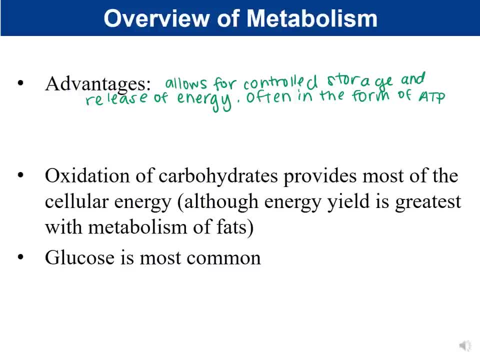 other things down in order to get that energy. Or if the cell has an abundance of a particular something, then they can store it for later use. So basically, this is going to allow for controlled storage and release of energy, So it's going to be the most efficient in terms of how that energy is utilized by the 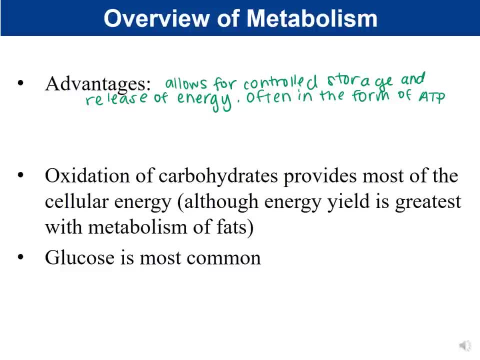 cell. Now, oxidation of carbohydrates provides most of the cellular energy, meaning it's the most common. It doesn't produce the highest yield, meaning it doesn't give us the most ATP per molecule, but it does provide the most energy, But it does. 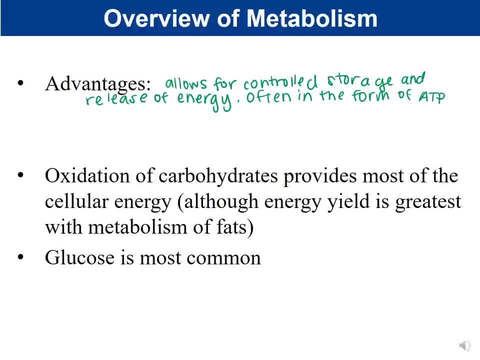 Fats are going to give us the greatest energy yield. It's just that fats are not metabolized as often. Typically, it's sugars that are going to use most of, Are going to produce most of the cellular energy, And glucose is going to be the most common. 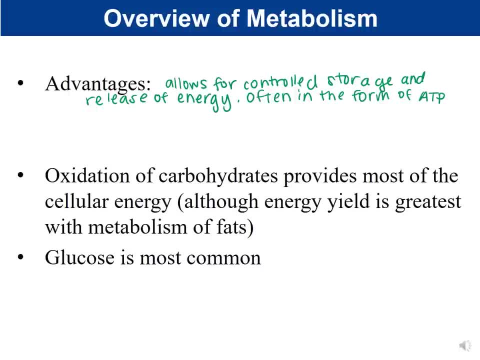 And so when we go through and we talk about cellular aspiration, we're going to talk about the breakdown of sugar, breakdown of glucose to produce ATP. But what you need to realize is: do we eat only sugar as a food source? And the answer is no right. 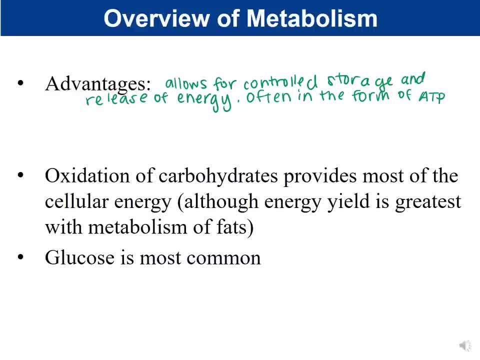 We're able to metabolize proteins to get energy and lipids and so on and so forth, And so it's not limited to glucose. Glucose is just the most common, And so that's why you see those overviews of metabolism, starting with our substrate. 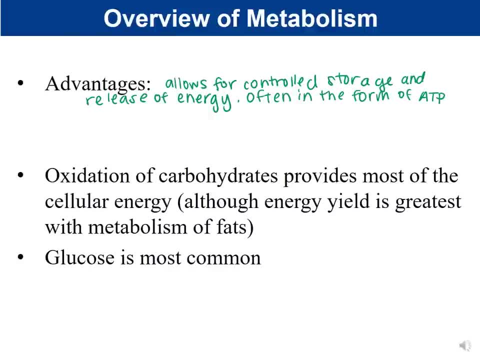 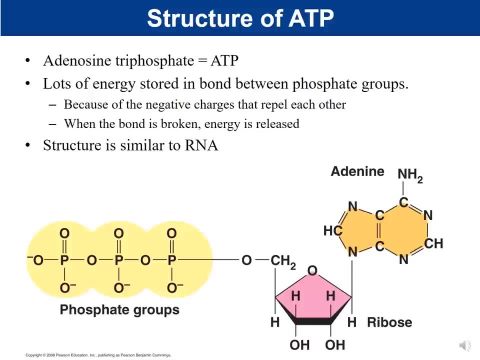 which is glucose, But be aware, it's not the only substrate. So let's talk about glucose. So let's talk about now ATP. So ATP stands for adenosine triphosphate, adenosine triphosphate, So let's underline, adenosine triphosphate is ATP. 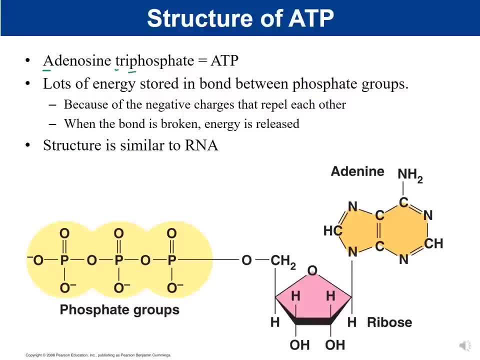 What ATP looks like is if you think about the building blocks of DNA. we have. our building blocks of DNA and RNA are nucleotides. Nucleotides have three parts: It has a sugar, A phosphate And a nitrogenous base. 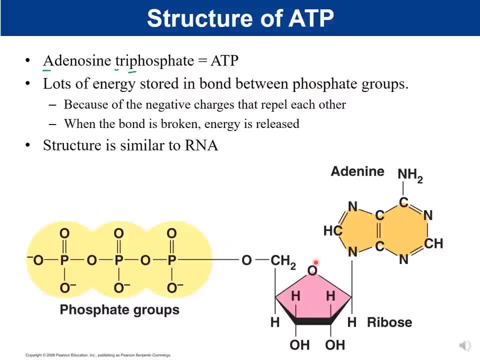 And so, if I look at my ATP molecule here, here is my pentose, my five-carbon sugar: one, two, three, four and five. This is our five-carbon sugar, And in this case the five-carbon sugar is going to be ribose. 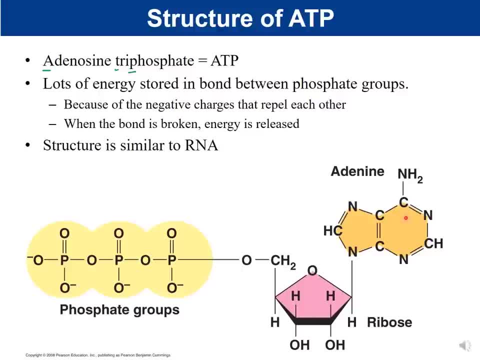 It has its hydroxyl group at carbon two. We have our base, So sugar. Here's our base. over here, This is adenine, So this is our nitrogenous base. And then we have our phosphate group. Notice that our phosphate group in this case is a triphosphate. 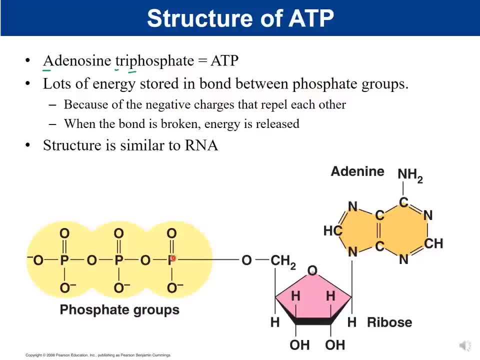 It has three phosphate groups on it, So this structure is similar to RNA. It's like the building blocks, in fact, of RNA, Because it's a sugar, a phosphate and a nitrogenous base. Now Let's look at these phosphate groups. 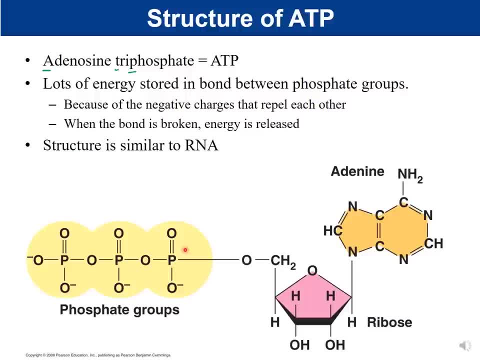 Phosphate groups carry a negative charge. So if you think about this, if this phosphate is negatively charged and this phosphate is negatively charged and this phosphate is negatively charged, do those negative charges want to be together? Do they want to be next to one another? 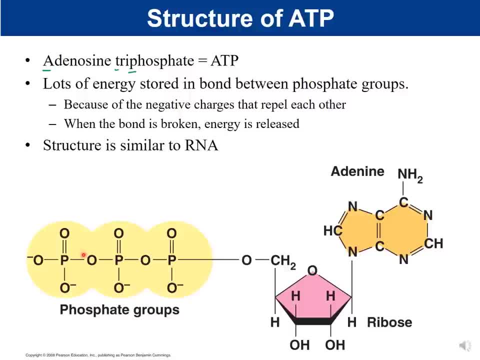 Do like charges attract? The answer is no. Like charges do not attract. Like charges actually repel one another. They don't want to be together. Opposite charges attract. So in order to build ATP, in order to put those phosphate groups together, energy had. 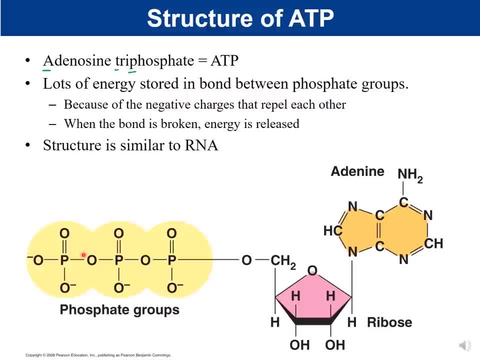 to be invested, Because linking those together is not energetically favorable. They don't want to go together, So energy had to be put in to form the bond between those phosphate groups, And so when energy is put in, that same energy is stored in this bond. 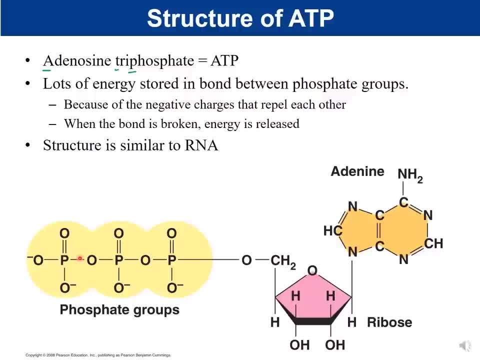 So the way that the energy gets released- And you're going to see that in a minute- Is that the bond gets broken And all that energy that was stored in that bond now gets released And it's going to drive cellular work. It's going to drive production of polymers for other things. 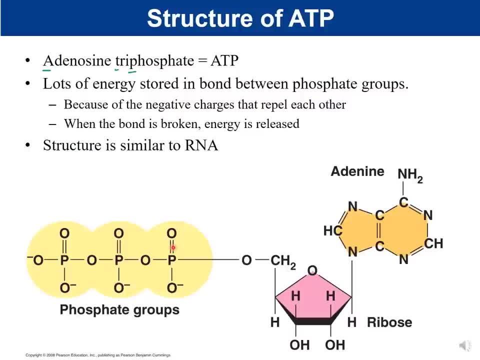 So the reason that ATP is so high energy is because it has three negatively charged phosphate groups- Those phosphate groups that are all negatively charged. They're not going to be together And because they don't want to be together, it took a lot of energy to form the bond between. 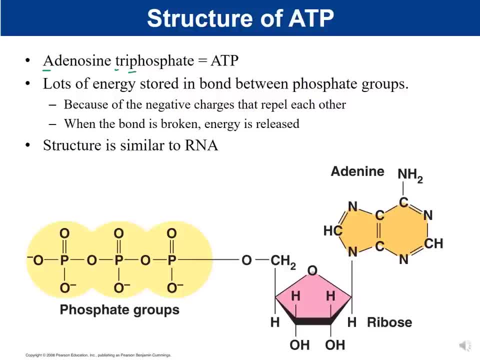 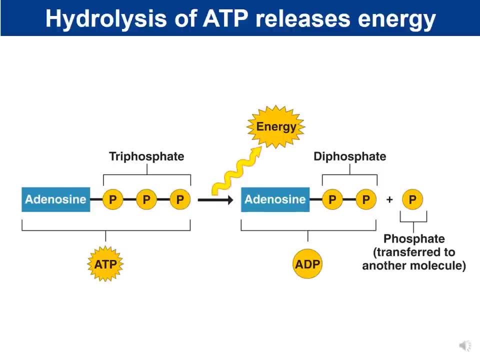 those phosphate groups And that energy is now stored in that bond. When that bond is broken, that energy gets released. So we just talked about how ATP is high energy, And so now we're going to focus on how does ATP release energy. 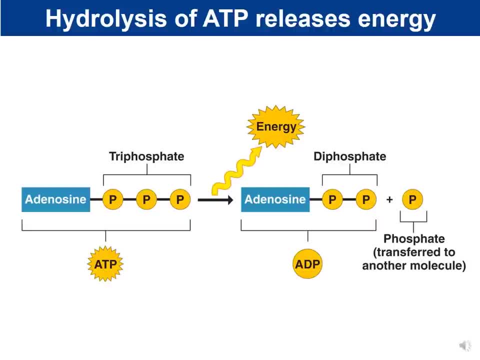 And so, again, ATP is adenosine triphosphate. So there's the triphosphate. So we have one, two, three phosphate. Remember that those three phosphates are all negatively charged, And so in order to link those phosphate groups together, a lot of energy had to be put in. 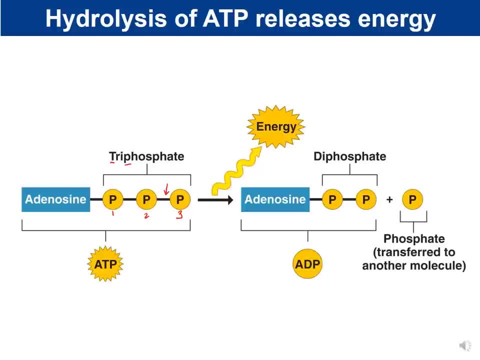 And the energy is stored in those bonds. So here's where the energy is stored, And so what happens is Is that ATP becomes hydrolyzed. So remember that when we're breaking something down, we have hydrolysis. We use water to break apart that bond. 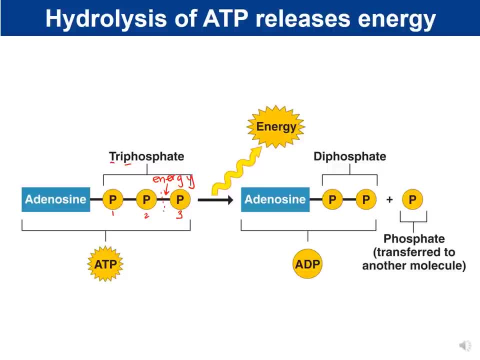 So we're going to break that bond. We're going to release that phosphate And you'll see that abbreviated PI And that is referring to an inorganic phosphate, Because it has no organic component to it. It's not carbon and hydrogen together. 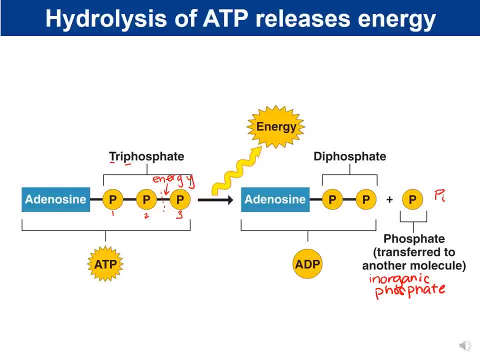 It's just a phosphate group. So when we break the bond between the second and the third phosphate, When we break that bond, energy is released And our products now are ADP, adenosine diphosphate. This can be broken down further. 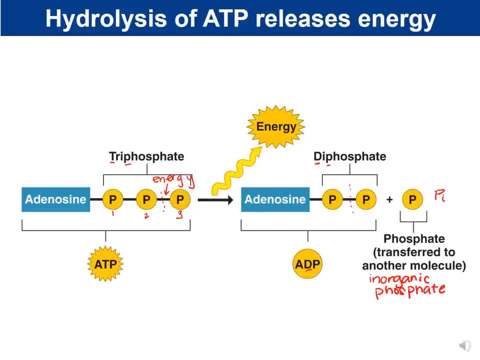 And this bond can be broken down And we end up with AMP or adenosine monophosphate. But for now we're going to focus on the hydrolysis of ATP specifically. So ATP releases energy when ATP is hydrolyzed. 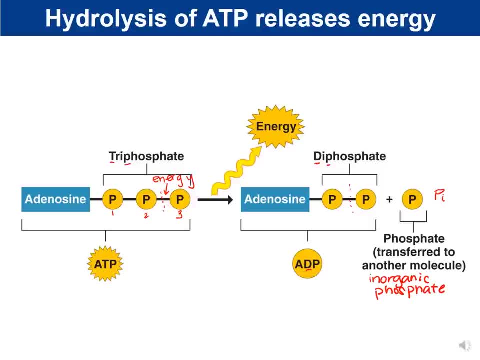 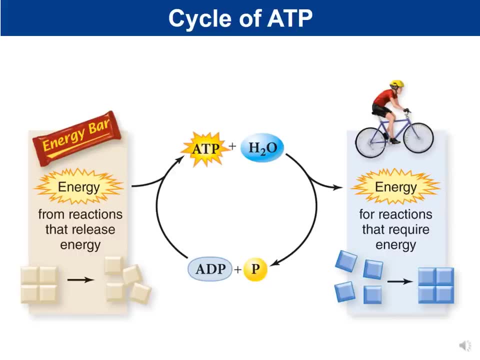 When it's broken down, it's going to release the energy that's stored in that bond. Now, in terms of ATP, One of the things that you need to realize is that cells Do not Do not Do not Store The high energy. 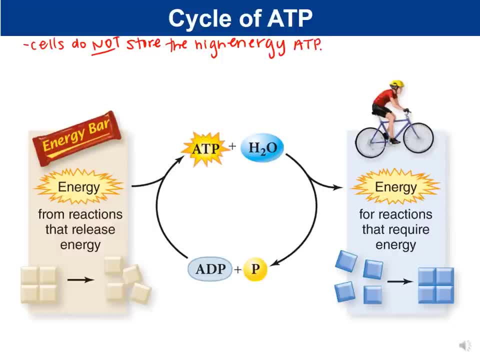 ATP. So ATP is high energy, but it's not how the cell stores energy. long term, ATP is too high energy. So if we think about the way that cells store energy, Think about what types of macromolecules that the cell might store energy, as So one would be polysaccharides, right Sugars. So instead 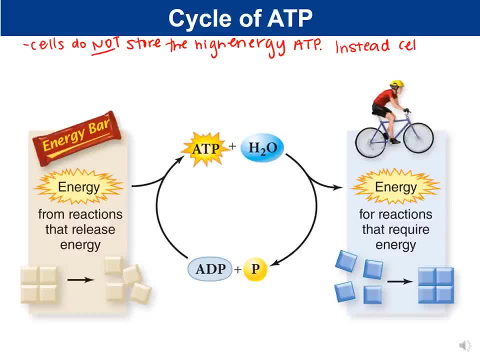 cells store energy-rich molecules such as so polysaccharide. How do animal cells store polysaccharide? What form of polysaccharide do animals have? Answer: glycogen Right. Animal cells store glycogen in the muscle and in the liver. How do plants 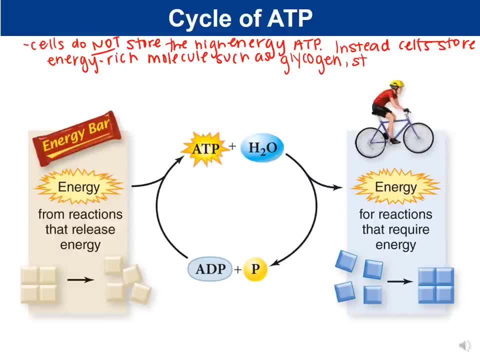 store their sugar And the answer is starch. And organisms store energy in fats. So the long-term storage of energy is not ATP. ATP is temporary energy. It's used pretty quickly. Long-term storage of energy is by producing macromolecules, producing these large molecules which can store. 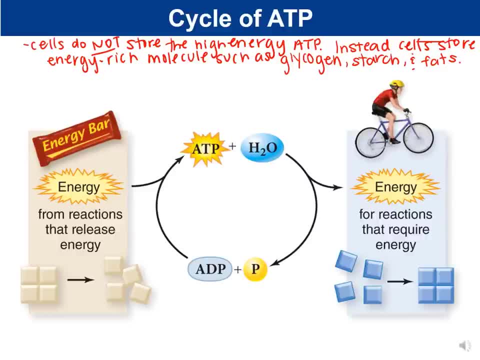 the energy And, when needed, that energy can be broken down. that glycogen can be broken down and release sugar, And then that can be used to produce ATP. So cells don't store high-energy ATP. Instead, they're going to store energy as glycogen, starch or fats. 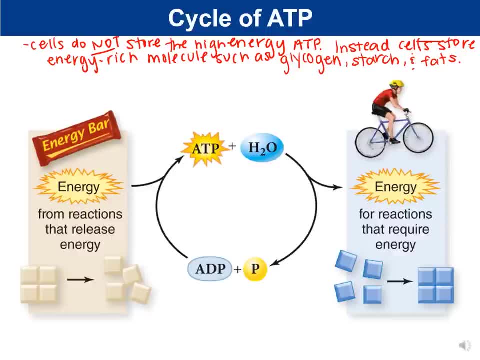 So what we're going to do is we're going to store energy as glycogen, starch or fats. So what we're looking here is we're looking at what is referred to as coupled reactions. So let me explain what this means. So, coupled reactions: So if we look at breaking down, 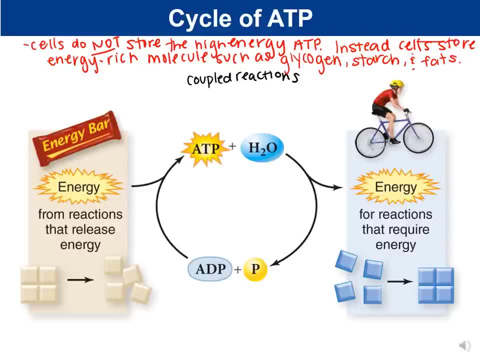 food. so let's say we are breaking down glucose to CO2 during cellular respiration. So we're breaking down glucose to CO2 during cellular respiration. So if we break down food, we are going to release the energy that's stored in that bond. So what do we call cellular respiration? 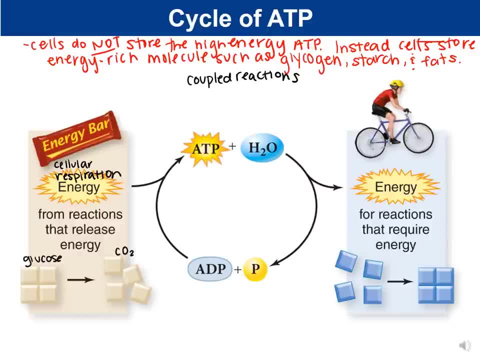 Indergonic or exergonic? And the answer is that this reaction- breaking down food- is exergonic. Energy is going to be released Now that energy that's released. so here's the energy: the energy that's released from this process is coupled to. 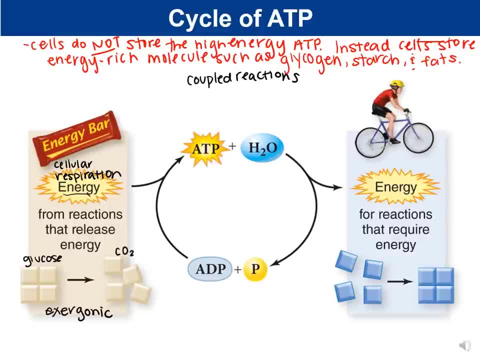 production of ATP, meaning this is how the cell is going to produce ATP. Now, this part of the reaction going from ADP, adenosine diphosphate and building ATP, is that reaction building ATP? is that indergonic or exergonic? And the answer is: building ATP requires the input of energy. 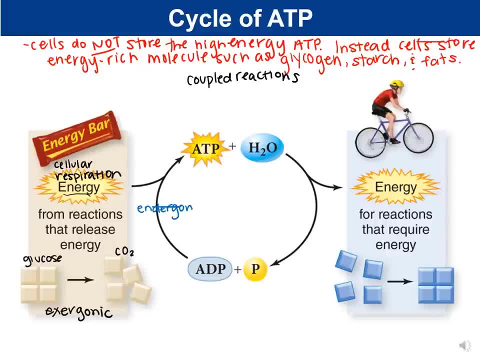 This part of the process is indergonic. Energy must be put in to build ATP. Where does that energy come from? It's paired with the exergonic reaction of cellular respiration. So when we take that sugar and we break it down, we're going to release energy. That energy is used to produce ATP. 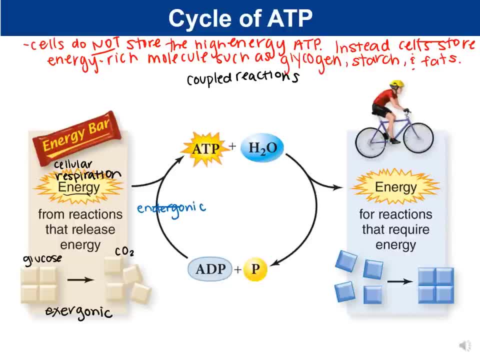 Now ATP can be hydrolyzed and when it's broken down, notice we have ATP plus water. When ATP is broken down, that is exergonic. It's going to release energy and that energy is going to be used to build molecules. 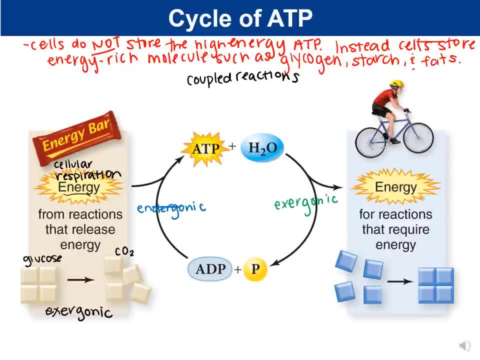 so it's going to, let's say, take glucose and build to form glycogen, adenoglycoside, Right, And then glycogen would come over the food chain and deliver, and so we're going to add at the end of the metabolism. And when that location is broken down, notice we have ATP plus water. When ATP is broken down, that is exergonic, It's going to release energy and that energy is going to be used to build molecules, right, And so it's going to, let's say, take glucose and build to form glycogen. 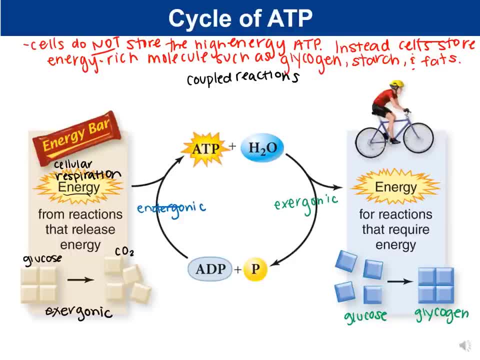 And then glycogen will work and then build to form a�이크ogen, depois de recuperar u tipo grécoli, and then glycogen can be stored. This part of the reaction, glucose to glycogen building up a polysaccharide- is endergonic. If we're building a sugar, energy has to be put in. 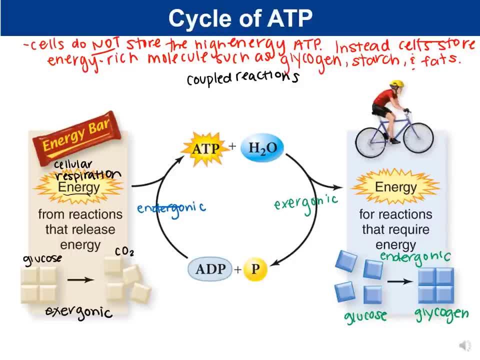 The energy comes from the exergonic reaction of ATP being broken down. So this is what we call a coupled reaction, and that is that an endergonic reaction, one that requires the input of energy, is paired with an exergonic reaction. The exergonic reaction is going to release energy. 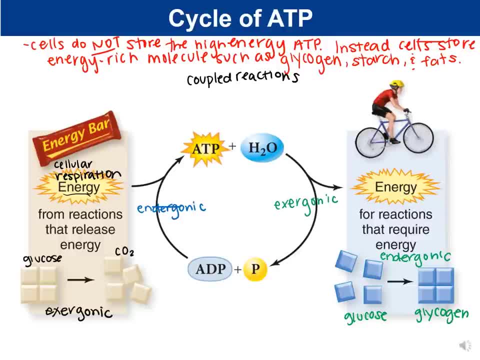 and the energy released from the exergonic reactions are used to power the endergonic reactions. So let's put a little note on here. So cells hydrolyze or use ATP during anabolic reactions. So when we're talking about coupled reactions, cells hydrolyze ATP during anabolic reactions. 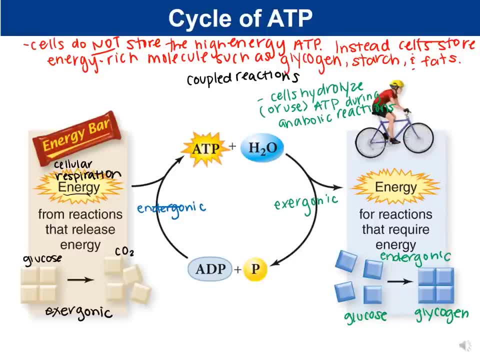 so those endergonic reactions, Because the energy that is released from ATP being broken down is going to be used to power those anabolic reactions On the flip side over here. So we're going to write cells synthesize or produce ATP during anabolic reactions. 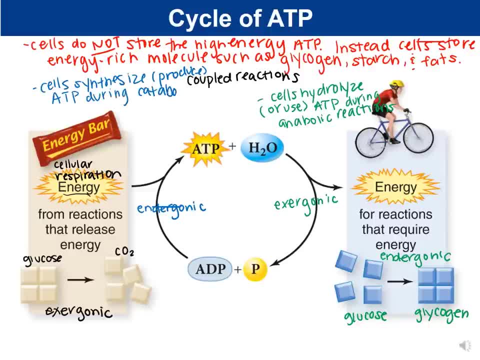 catabolic reactions. So what that is essentially saying is that cells are going to make ATP when other catabolic reactions are occurring. So again, if we break down food, that is a catabolic reaction, That is exergonic, It's going to release energy and that energy is used to build ATP. 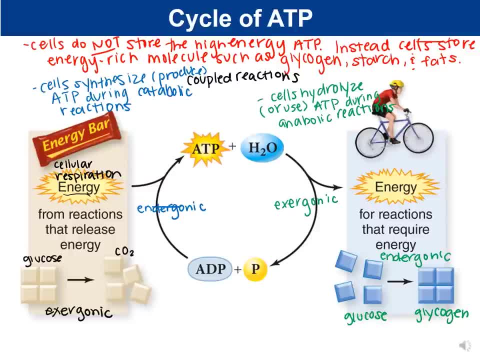 And so this is what we mean when we talk about coupled reactions. The two reactions are coupled to one another. If you need energy to be put in for a reaction to occur, that energy has to come from somewhere. That energy is going to come from other exergonic reactions. So this is what we call. 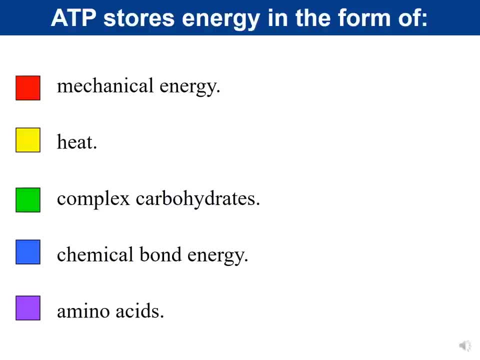 a coupled reaction. So question for you: ATP stores energy in the form of blank. So we're not talking about cells, It's not cell store energy. How does ATP itself store energy? So would you say red mechanical energy, yellow heat. 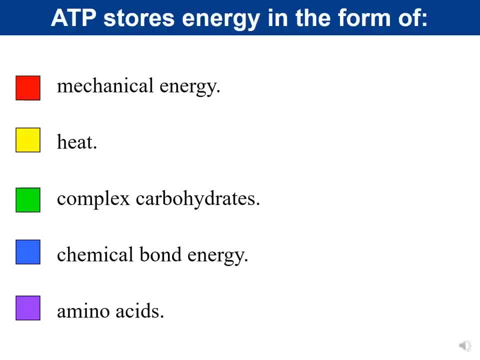 green complex carbohydrates, blue chemical bond energy or purple amino acids. So when you're ready, let's go ahead and resume it. So if you said blue, you are correct. ATP stores energy in the form of chemical bond energy. 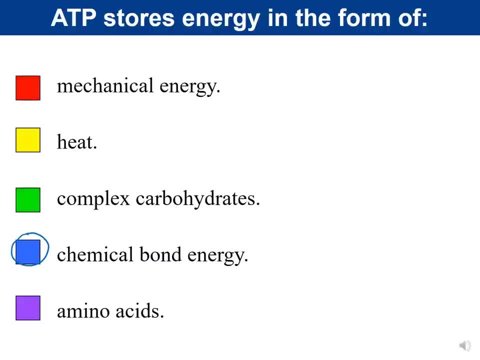 meaning it stores its energy in the bond between the phosphate groups, And when those phosphate groups are broken, that energy is released to power cellular work. So ATP itself stores energy in the chemical bonds. If this had said blue, you are correct. So if you said red, mechanical energy. 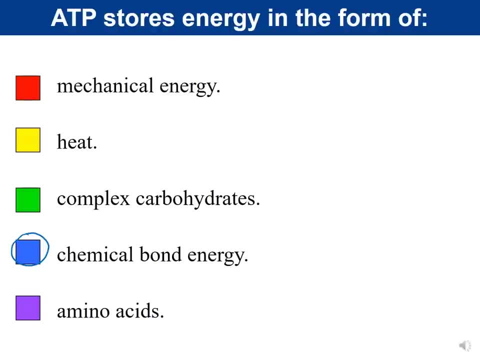 blue and yellow complex carbohydrates could be correct. right, But we're not talking about the cell. We're talking about how ATP stores energy. Where does ATP get its energy from? And it gets it from its chemical bond energy. So, in order to understand a little bit more about chemical reactions, we need to have a few terms, And the first term is what we call the collision theory. So if you're a chemical bond energy人, have a few terms, And the first term is that is what we call the collision theory, And the first term is, that is what we call the collision theory, And the second term is the herauskommelenza. So if you wanted to understand the whole energy relationship, what do you have to do? Well, what do you do, And I'm going to have to do- is do a little bit of a breakdown. So the first term is that 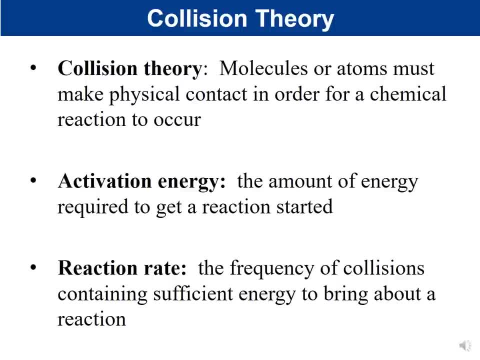 that is what we call the collision theory, And that is that molecules or atoms must make physical contact in order for a chemical reaction to occur. So, if you think about it, molecules are in motion, right? They're constantly moving. So in order for a reaction to occur, they must collide. There's the collision theory. 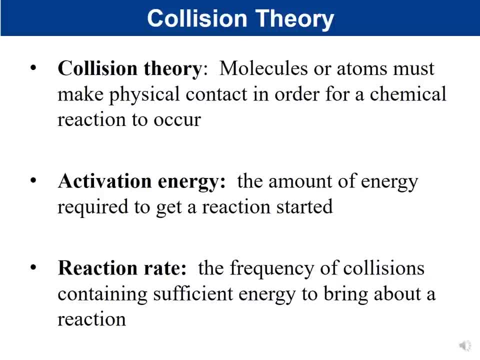 They must collide and when they collide, that contact can allow the reaction to occur. So if you think about ATP hydrolysis, right, Not only do we need ATP, but ATP has to come in contact with water in order for ATP to be hydrolyzed. 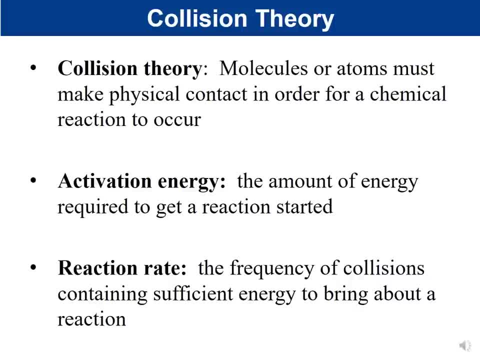 So that's the collision theory. They must make contact in order for the reaction to occur. And what you're going to think about in a minute is what can be done to make those collisions more likely, And we'll talk about that in a minute. 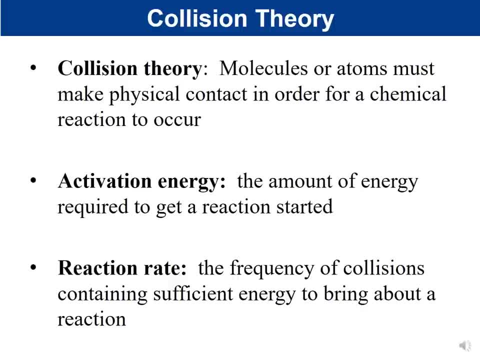 Activation energy. Activation energy is the amount of energy required to get a reaction started, And so what that means is that even reactions that are exergonic, even reactions that are going to release energy, have to have a little bit of energy inputted to get the reaction started, And that energy that has to be put in is 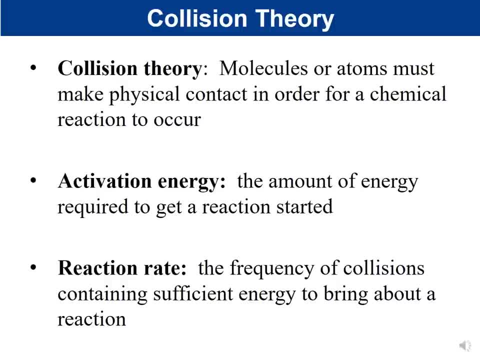 activation energy. When we talk about reaction rates, the reaction rate is the of collisions containing sufficient energy to bring about a reaction. So, basically, how fast does this reaction occur? And so that is going to be the reaction rate, And so the reaction rate. 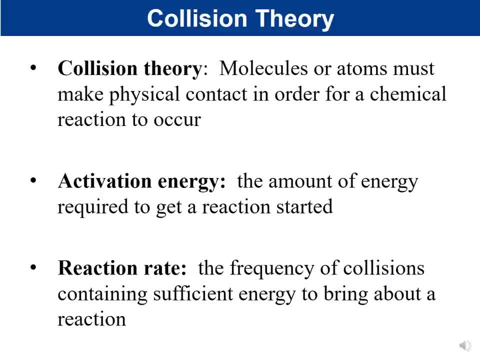 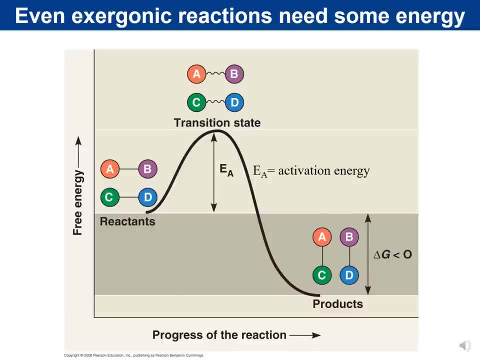 depends on the number of reactive molecules at or above the activation energy. So again, even exergonic reactions need some energy to be put in in order for the reaction to occur. So notice, if we look at this energy diagram, on the bottom we have the progress of the reaction on the y-axis. 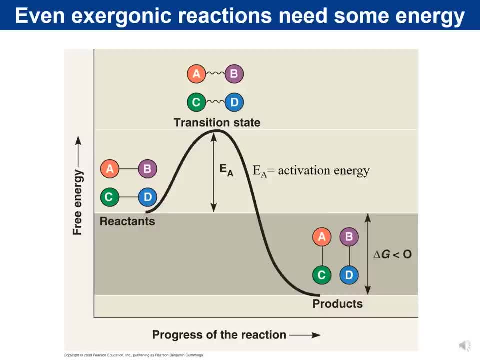 we have free energy And so what you're looking at is that your reactants- notice on this- have more energy than the products, So the reactions have higher energy. So this reaction is exergonic, It's going to release energy. However, in order to get the reaction going, energy must be put in. 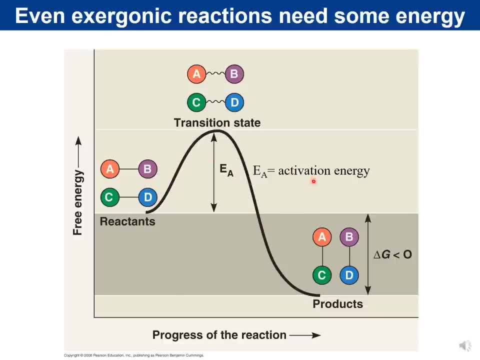 That hill that it must overcome is called the activation energy And that's going to be abbreviated EA. So when you see EA, you're thinking activation energy. So even exergonic reactions, even reactions that release energy, have to have a little bit of energy put in to get the reaction. 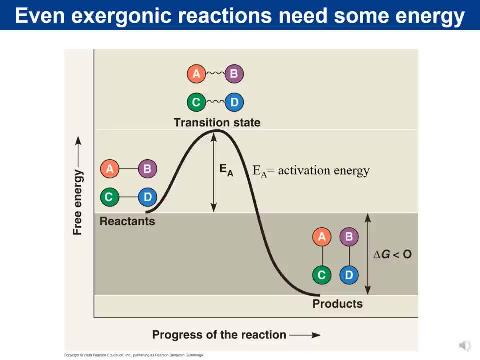 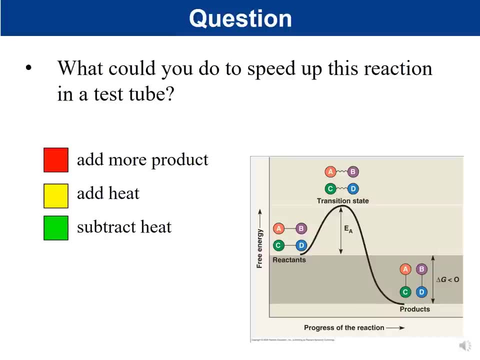 started And again, that is going to be our activation energy. So question for you: what could you do to speed up this reaction in a test tube? Is it red, add more product. Yellow, add heat. Green, subtract heat. So pause your video and when you're ready, push play to resume. So if you said 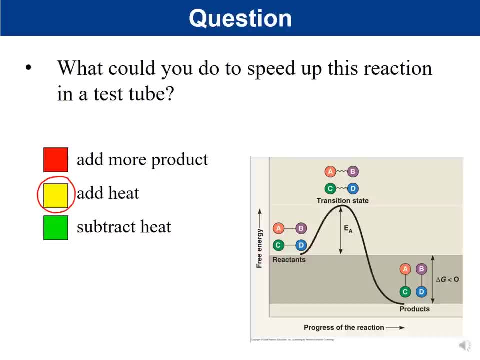 yellow, add heat. that would be correct Because if you think about it, what happens to molecular motion when you add heat? Do molecules move faster or slower? And the answer is that molecular motion increases, Molecules start moving faster. And if molecules 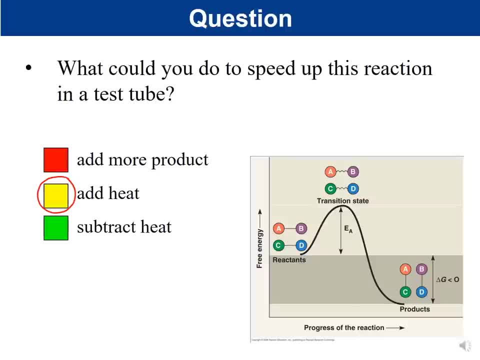 move faster. it makes collisions more likely, Because remember that collisions have to take place in order for the reaction to occur, And so adding heat is going to make the reaction occur faster. Subtracting heat will do the same thing. So if you add heat, it will make the reaction. 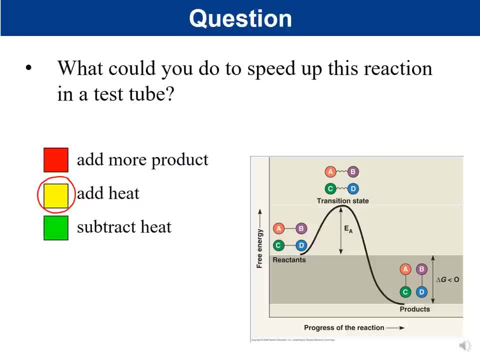 do the opposite. right? If you remove heat, molecular motion is going to slow down and would make the reactions less likely. Now, adding more product is not going to make the reaction go faster, right? The product does not influence this substrate and the enzymes or the reaction to occur. 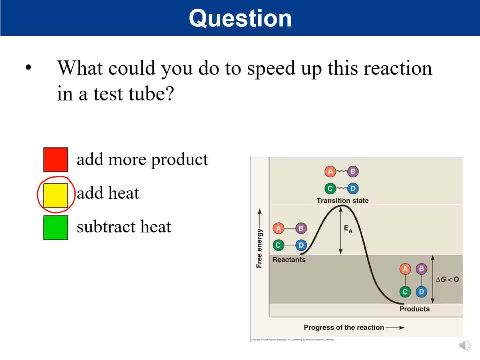 So adding more product is not going to make it go faster. Now, in terms of cells, do you think living organisms or cells would add heat to speed up their chemical reactions? Is that an efficient way to make the reactions go faster? And the answer is no, that is not efficient, For one thing. 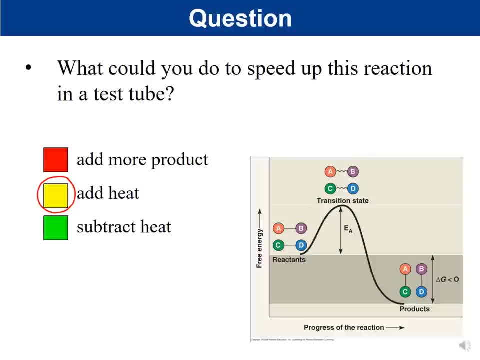 if heat goes up too much, proteins denature. Remember that proteins are going to fall apart. So heating the cell up to get the reaction to go faster is not necessarily the best idea for a cell. The other problem with adding heat to get the 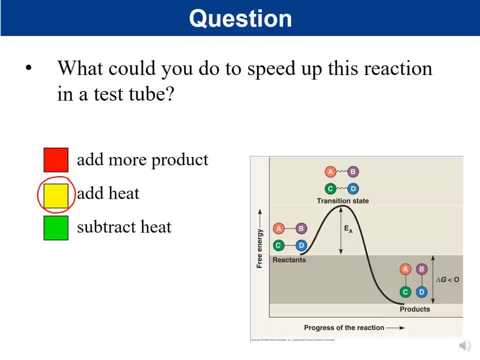 reaction to go in a cell is. not only do proteins denature, but if you use that method to speed up a chemical reaction, is it only speeding up a specific chemical reaction or would it speed up all chemical reactions? And the answer is: if you added heat, it would speed up all chemical. 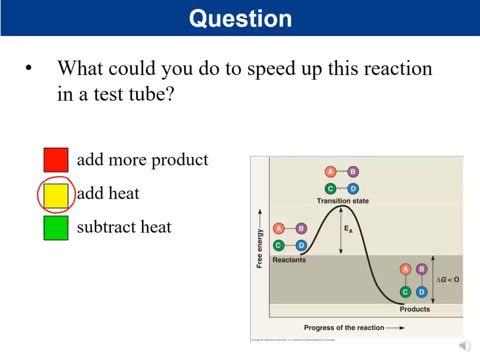 reactions. The cell doesn't want to do that. The cell wants controlled storage and release, So it's going to speed up certain reactions and inhibit others. That allows for a control of metabolism. So adding heat is not how living cells will do it. 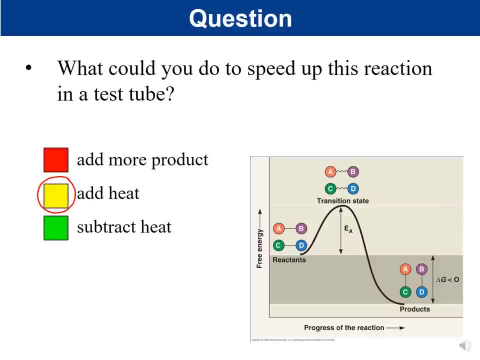 Reactions in a test tube can add heat to make them go faster, but in living cells that's not the answer, And we'll talk about how living cells deal with this in just a minute. So there are several ways that the reaction rate can be increased. 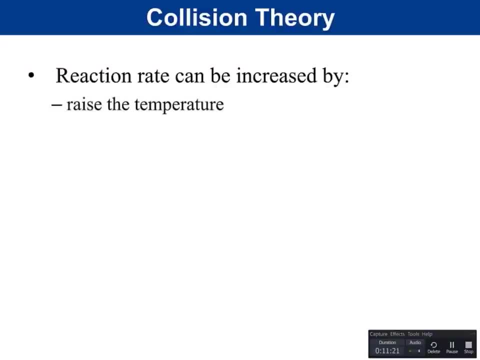 One that we talked about was to simply raise the temperature, because again, the temperature that is going to increase molecular motion or kinetic energy and the reaction is more likely, Stir right, By simply stirring the tube that can help with the reaction occurring, because, again, it could make collisions more likely When pressure is increased. So if the 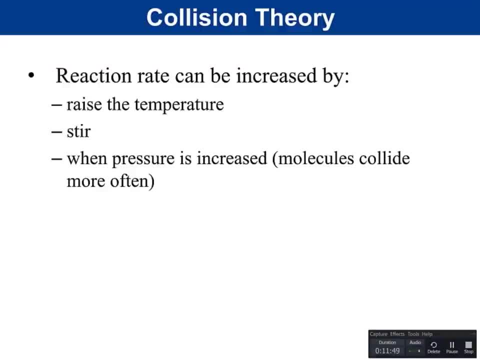 amount of pressure in the system is increased. that can make molecules collide more often. Higher concentration of reactants, so more concentrated, Because the distance between the molecules decrease, which makes them more likely to collide. So adding more reactants or more substrate is likely to make the reaction go faster, up to a point. 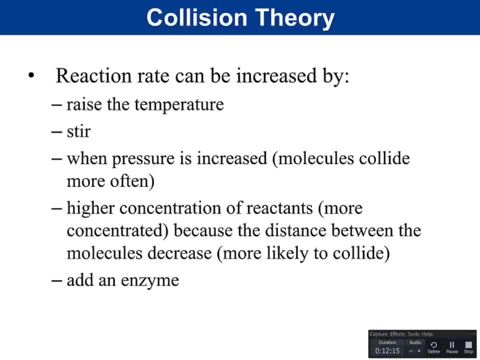 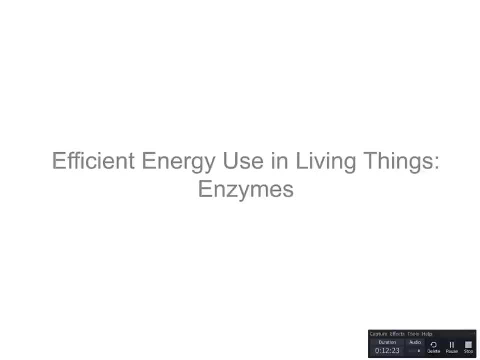 which you'll see in a little bit. And then, lastly, the way that living things speed up chemical reactions, add an enzyme, And so we're going to talk about what enzymes do. So efficient energy use in living things, enzymes. So 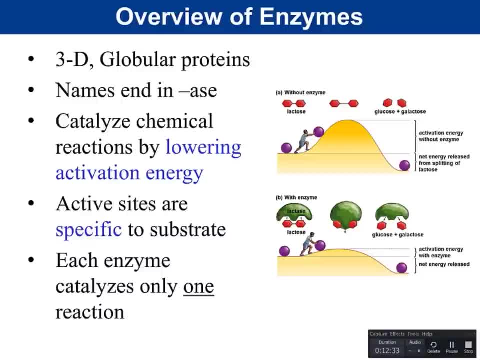 an Overview of enzymes. Enzymes are three-dimensional globular proteins. Their names end in ace, A-S-E. So when you see ace, ace tells you enzyme. So lactase, for example, is the enzyme that hydrolyzes or breaks down lactose. 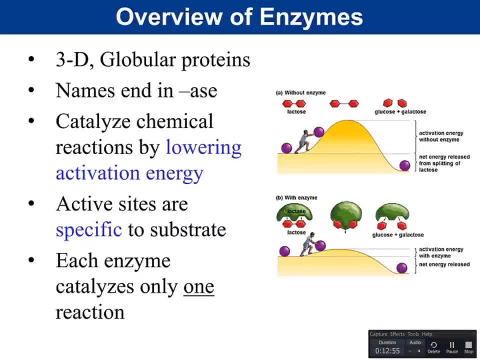 The way that enzymes work, the way that they catalyze chemical reactions, is by lowering the activation energy, Lowering the amount of energy needed to get the reaction going. So what do I mean by that? So let's look at two examples. 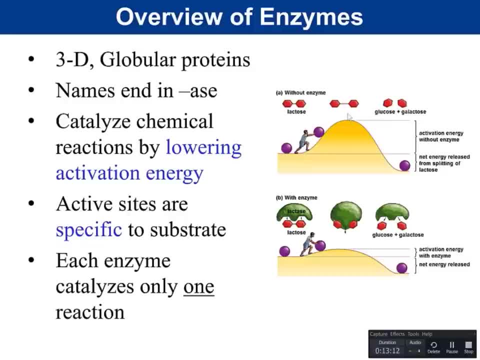 So on the top, this is our system without an enzyme. on the bottom, with the enzyme. So if we're looking at without an enzyme, hydrolysis of lactose is a favorable reaction because we're breaking something down that is exergonic. 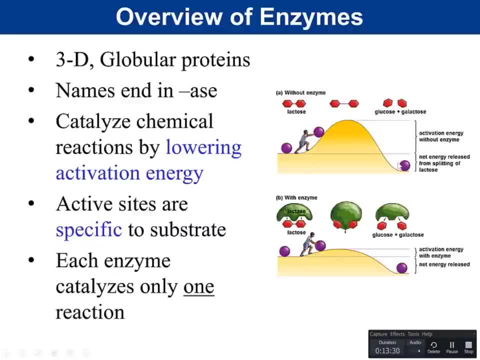 So notice that our lactose has more energy relative to our mottomers, which are the glucose and the galactose. So, even though this is going to be a process that releases energy, energy still has to be put in to get the reaction going. 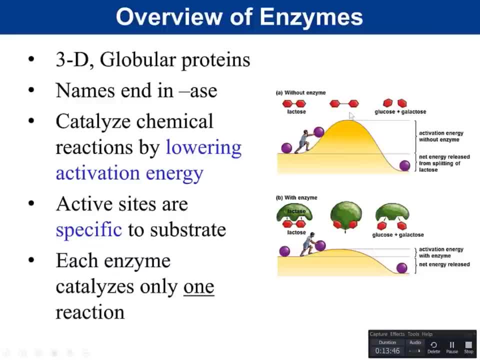 So this person needs to get the ball up and to the top of the hill before it can go down Now with an enzyme. so if we have lactase, for example, it helps bring substrates together. So remember that for something to be hydrolyzed. 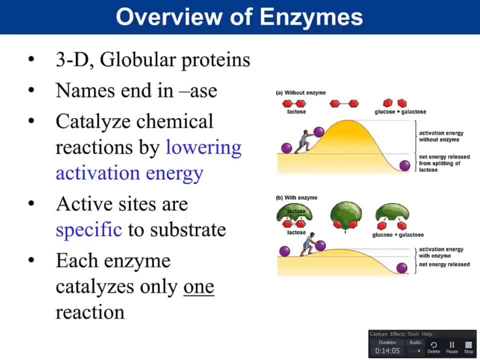 we need the substrate And we need the water. So the enzyme helps facilitate and bring those substrates together, And so that is going to make the reaction go faster, because what it's essentially doing is it's lowering the activation energy, It's making the Hill smaller. 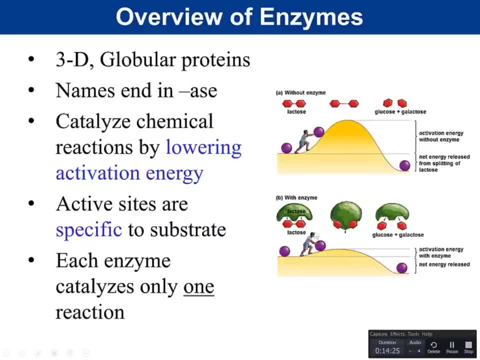 If the hill is smaller, it's much faster for the man to get the ball up to the top of the hill so that it can roll down. There's a smaller hill, It's going to occur at a faster rate, And And so the way that enzymes work is that they lower the activation energy. 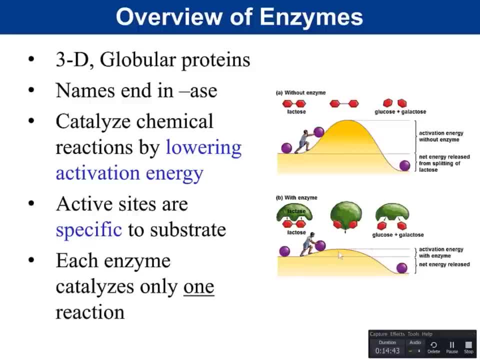 Now, the active site is the site on the enzyme that binds to a substrate, And these active sites are highly specific to a particular substrate. So, for example, if you're looking at lactase, lactase is an enzyme that breaks down lactose. 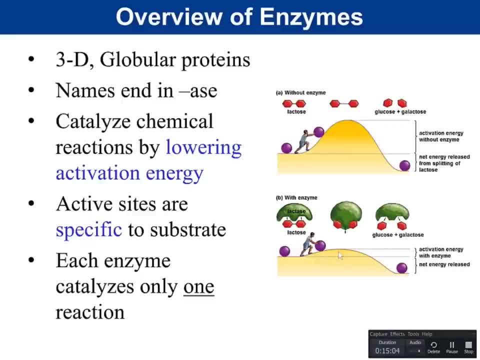 Lactose is a disaccharide. It's two sugars put together. Sucrose is a disaccharide. Sucrose is made of glucose plus fructose. Notice: lactose is glucose plus galactose. Sucrose is glucose plus fructose. 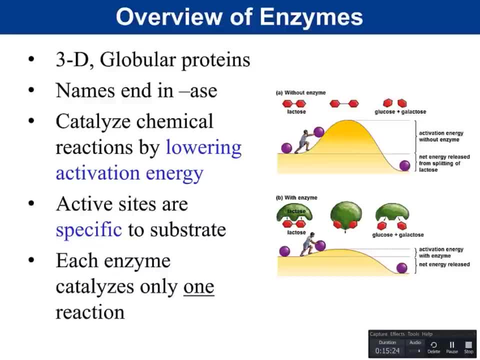 They're both disaccharides. They're both made of sugar. Lactase will bind to lactose and break it down, but it will not bind to sucrose, even though sucrose is also a disaccharide, And so the active sites are very specific to a particular substrate. 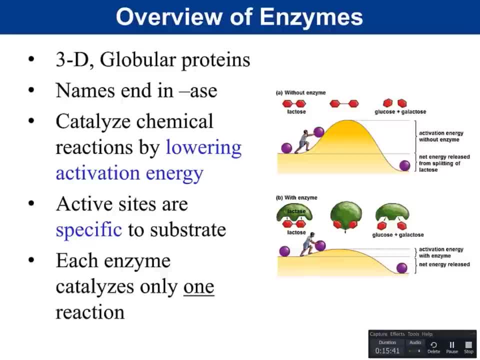 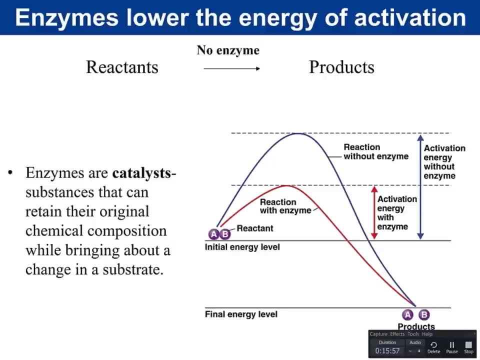 Each enzyme typically catalyzes only one reaction. So again, lactase is going to hydrolyze lactose, That's about it. So each enzyme typically catalyzes only one reaction. So enzymes, again, the way that they work is they lower the activation energy. 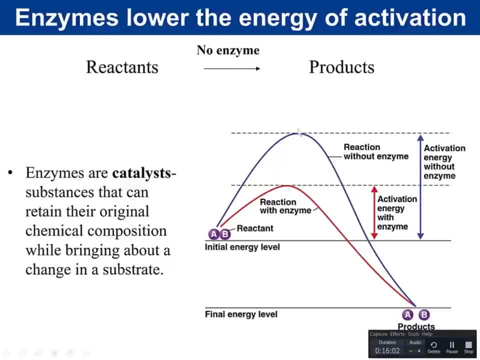 So if we look at this on a graph, the blue is without an enzyme and the red is with an enzyme. We still get the same amount of energy released Either way. it's simply that with an enzyme and we lower the activation energy it makes. 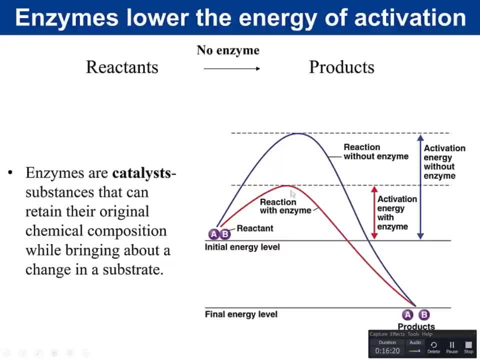 the reaction go faster because it takes less time to get up and over the hill than if it was without an enzyme. So without an enzyme the reaction will happen, but it happens much faster when an enzyme is present. It's going to speed up the chemical reaction. 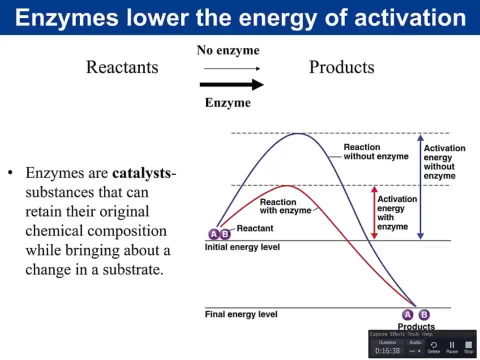 Now enzymes are catalysts, substances that can retain their original composition. So when an enzyme is done with its reaction and it releases its products, the enzyme itself remains unchanged, The products will leave and the enzyme is ready to do the reaction again. 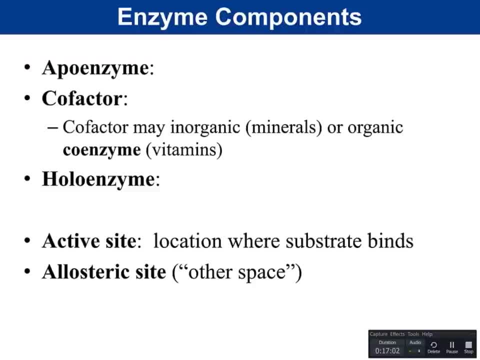 So if we talk about enzymes, enzymes are primarily protein, And so the protein portion of the enzyme is referred to as the apoenzyme. The apoenzyme is the protein portion, But what you'll realize is that enzymes are not the same as the protein portion. 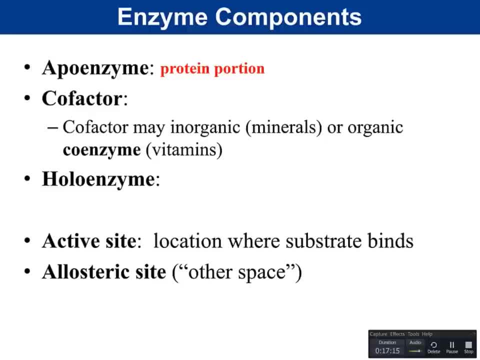 Enzymes are not only protein. They often have a cofactor with them, And the cofactor is the non-protein portion. Cofactors may be inorganic, which we would refer to as a mineral, So like for iron, for example. 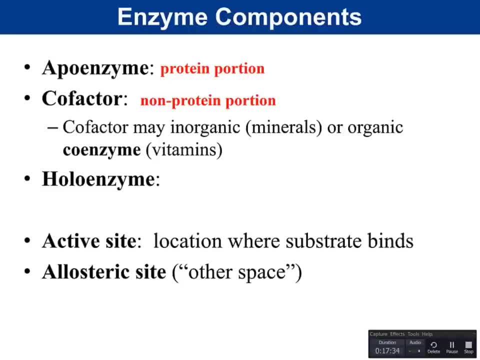 Hemoglobin, the protein in your red blood cells that carries oxygen. Hemoglobin requires iron, requires that inorganic molecule. Some need organic Coenzymes, which we also refer to as vitamins, But again notice that there's a protein portion and a non-protein portion. 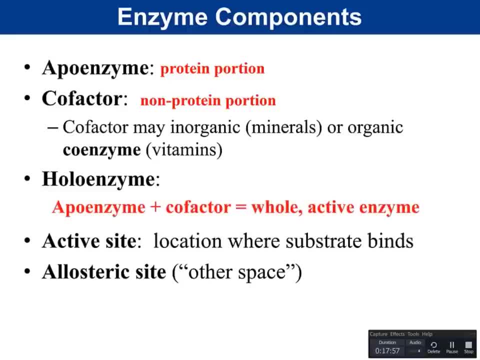 Putting the apoenzyme and the cofactor together, you get the hollow enzyme. I think hollow-whole It's the whole active enzyme. On an enzyme we have an active site. The active site is where the substrate binds, And some enzymes have what's referred to as an allosteric site. 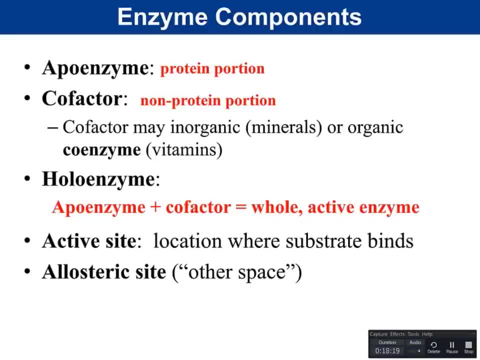 Allosteric refers to a site where the collagen is present. When you go to the cell, you want to know how it's called to other space, and that simply means that there's a space on the enzyme that can be used for regulation, and you'll see that in a little bit. 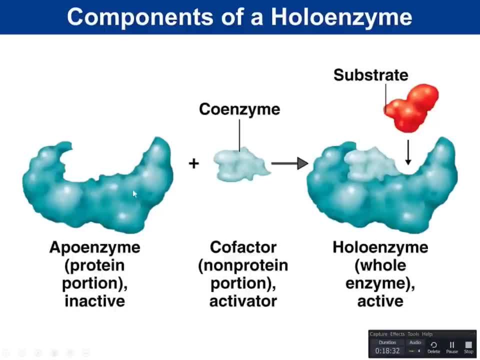 So, if we look at the components of a hollow enzyme, we have our apoenzyme, which is our protein portion. by itself, it's inactive. We have our cofactor, in this case it's a coenzyme, which means it's organic. 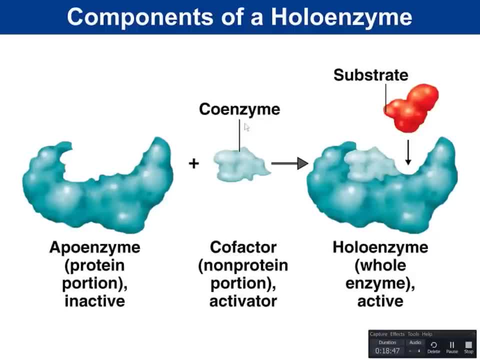 This is our non-protein portion and it's our activator, meaning it helps the enzyme function. So when we put the apoenzyme with the coenzyme or the cofactor, now we have the appropriate active site and now the reaction can occur, meaning now the substrate can come in and 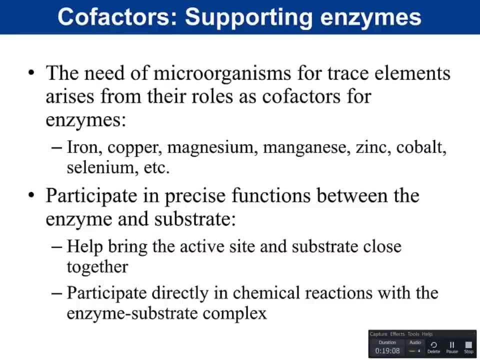 it can bind to the active site. So the need of microorganisms, and other cells, for that matter, for trace elements, arises for their role as cofactors. So again, iron, for example, can act as a cofactor: copper, magnesium, manganese, zinc, cobalt. 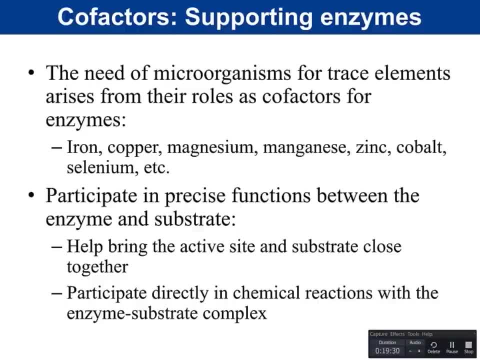 selenium, etc. And the purpose of these cofactors is that they participate in the precise function between the enzyme and the substrate. They might help the active site and the substrate come close together. In some cases they will participate directly in the chemical reactions with the enzyme. 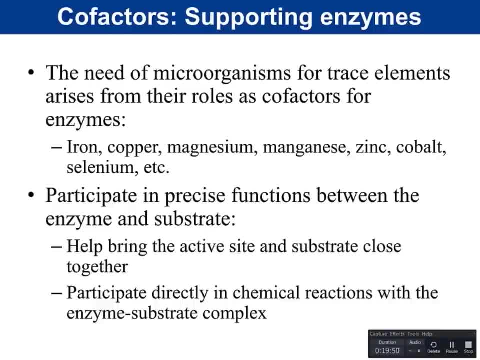 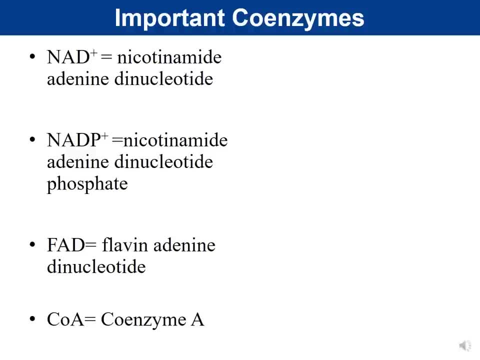 substrate, But basically they support the enzymes. So there are several important coenzymes that you should be aware of. The first coenzyme is going to be NAD, NAD+, And NAD plus stands for nicotinamide adenine dinucleotide. 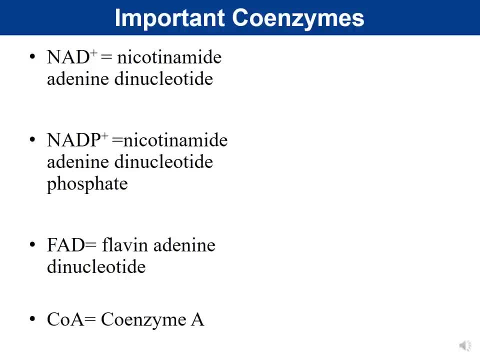 And so what that is is that NAD, NAD plus and NADP plus NAD plus and NADP plus, NAD plus and NADP plus NADP plus and NADP plus. These are both electron carriers, whoops carriers that are derived from the B vitamin. 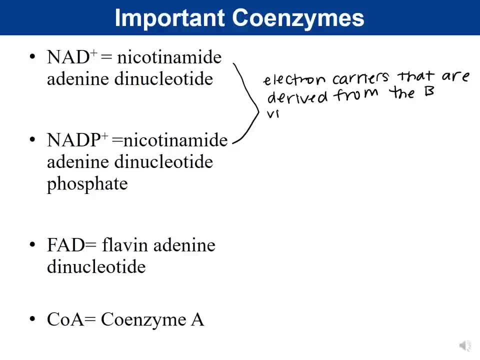 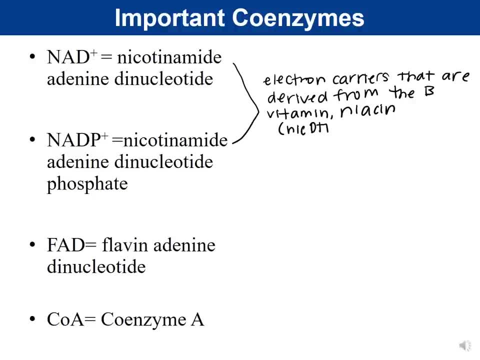 Anyways, you're welcome to write them down in the comments below. We will be glad to answer any questions. Thank you to everybody on the live stream for being here today. See you next time. Bye, Bye, Bye, Bye, Bye. 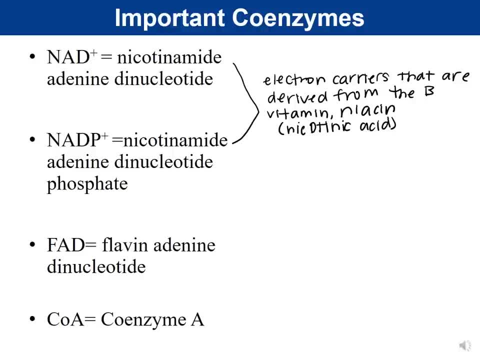 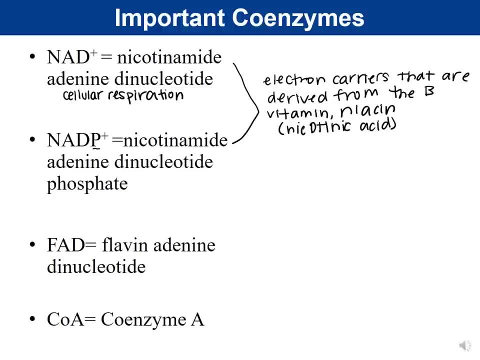 The way I remember what NADP plus is, think, photosynthesis, Photosynthesis, It's an important electron carrier in photosynthesis, And so both photosynthesis and cellular respiration, they both have an electron transport chain in them, And what's? 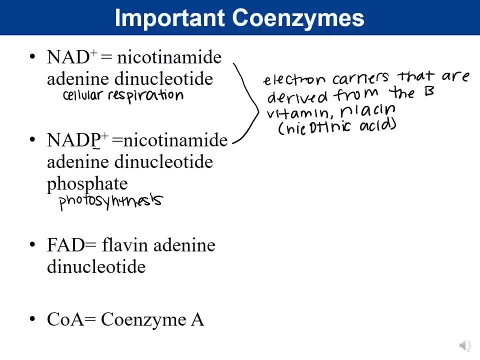 going to bring the electrons to the electron transport chain are these electron carriers? So my NAD plus and my NADP plus are going to be my electron carriers Now. FAD is an electron carrier but is derived from the B vitamin riboflavin. 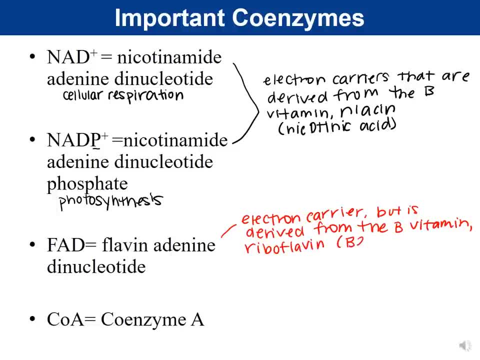 which is vitamin B2.. It is also used in the electron transport chain in respiration And you're going to see that FAD, when it gains electrons, it becomes FADH2.. And that's going to go drop off electrons at the electron transport chain. 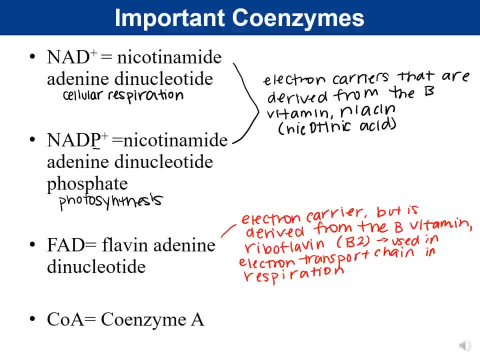 And then, lastly, we have what's called CoA or coenzyme A, And coenzyme A is derived from the B vitamin, pantothenic acid. This is where Sus Pew and I are going to deal with the microolba regulation. 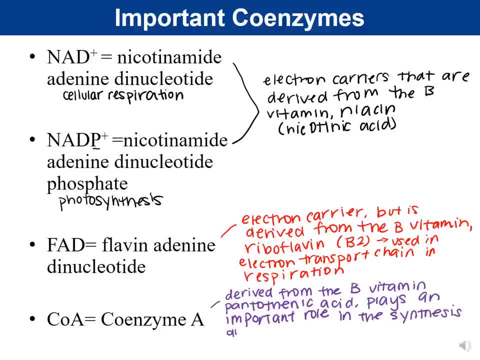 CoA and coenzyme A Right. So this Theory of Titanium, Panthenol Probiotics is our important receptor here. It's our dominant side carbon. and our dominant side carbon, It's astarothenic acid of fats and is used and in the Krebs cycle. 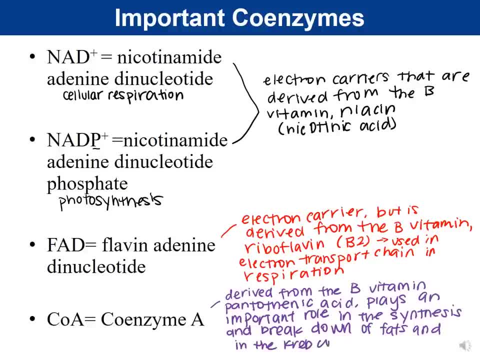 and so these are some examples of important coenzymes. coenzyme tells you it contains carbon and hydrogen. so these are some examples of important coenzymes that we will see again later in our cellular respiration talk. so we're going to walk through and talk about the steps. 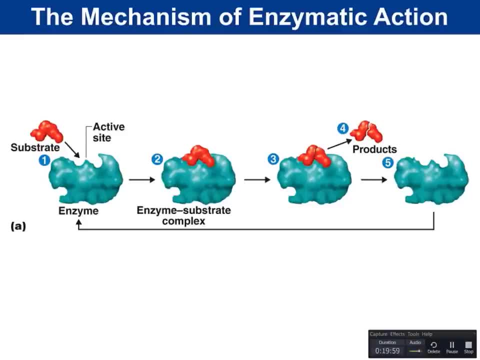 in the enzymatic action, meaning how do enzymes work? and so we're going to divide this into four steps. the first step is that the substrate is going to contact the active site, so the substrate comes in and it binds to the active site. Step number two: we have this temporary 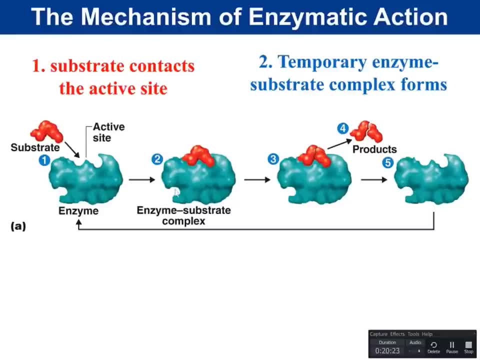 enzyme substrate complex that forms. So we have our temporary enzyme substrate complex. Step number three: the substrate is transformed into the products, So it's going to catalyze that reaction. And then, step number four, the products are released and the enzyme remains unchanged. 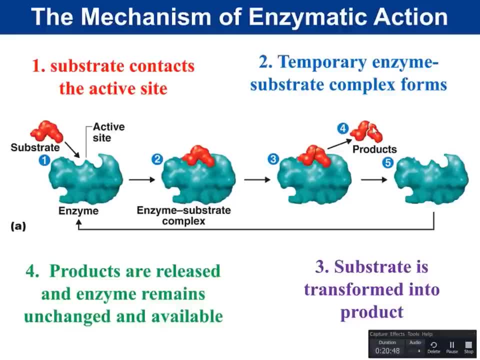 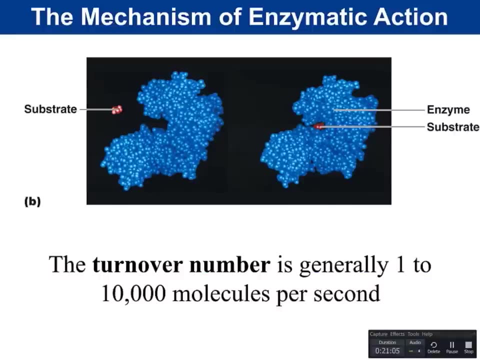 and available, It's ready to do the reaction again, And so this is the step of how enzymes work. And so again, when it's all finished, it's ready to go back and bind to another substrate. So if we think about how enzymes work, remember that I said that enzymes are very specific to a 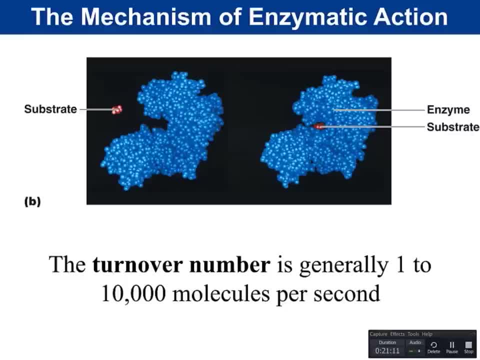 particular substrate. Now, sometimes you'll hear of an enzyme as being like a lock and a key right. So if you think of a lock, the key has to fit perfectly In order for the lock to open. However, it's not quite that rigid in the case of an enzyme. 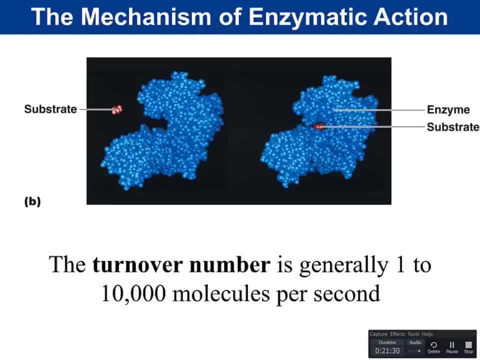 The enzymes actually are what we refer to as an induced fit, And what that means is look at the active site before the substrate binds. You can see that it has this particular shape. However, when the substrate binds, you'll notice that we have an induced fit. The enzyme changes its shape. 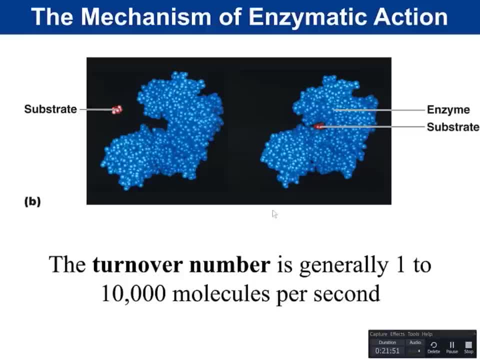 to a different shape. So if you look at the enzyme, it's like a baseball glove And the substrate is a baseball. If you've ever played baseball and you played catch with somebody, you know that if I leave my glove open and somebody throws me the ball, 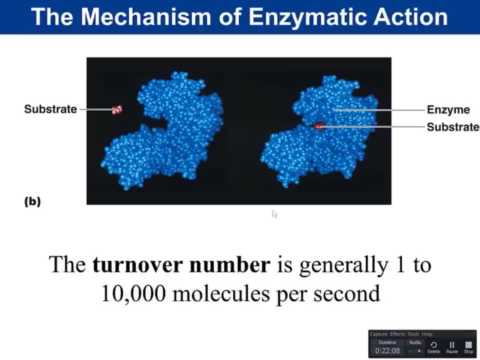 if I don't move my glove, the ball's going to hit the glove and it's going to come right out. However, if I want to actually catch the ball, when the ball goes into the glove, I need to close my glove. 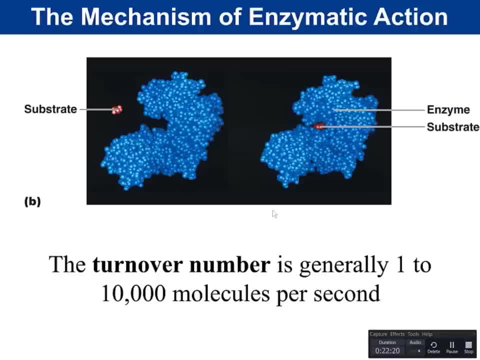 right. And when I close the glove I'm going to have to close my glove. And when I close the glove, that keeps the ball in the glove. Same idea with the enzyme and the substrate. The enzyme is like the baseball glove: It has to close. It has to change its shape to accommodate that substrate. 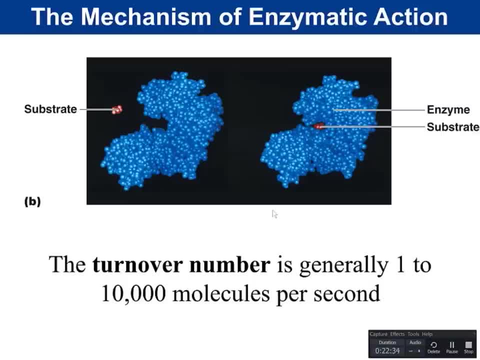 to help keep it in Now. in terms of reaction rates, the turnover for many enzymes is typically between 1 to 10,000 molecules per second, But the fastest known enzyme, carbonic anhydrase, can do a million reactions per second. 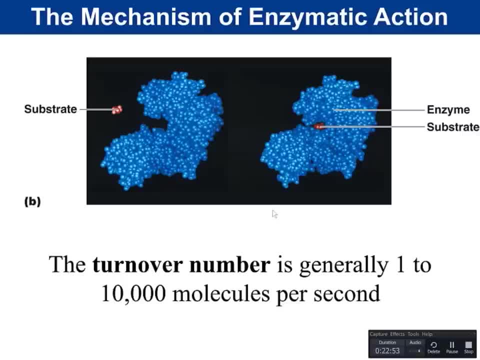 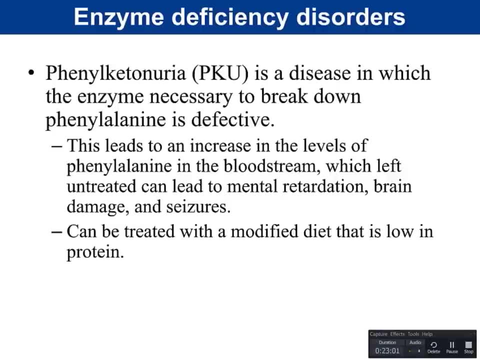 So think about that. Boom Just did a million reactions. That's pretty crazy. So enzymes are very efficient. There are many diseases that are associated with enzyme deficiencies. One genetic disease is phenylketonuria PKU. This is a disease in which the enzyme necessary. 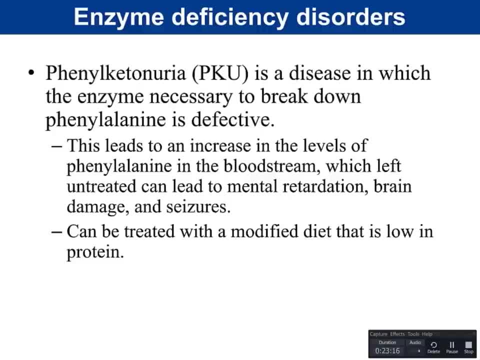 to break down. phenylalanine is defective. So the people who are born with PKU, they have a defective enzyme. And so what ends up happening is that if these patients, if these people eat proteins and their body can't metabolize that phenylalanine, which is an amino acid, if they can't metabolize, 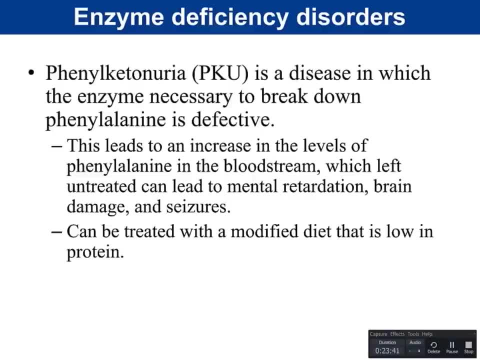 the phenylalanine. the phenylalanine leads to an increase in the blood which, left untreated, can lead to mental retardation, brain damage and seizures. And specifically, it's more critical to watch the phenylalanine levels in kids because, as the brain is developing, having these high 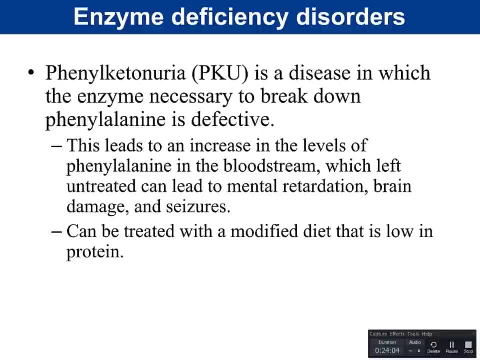 levels of phenylalanine causes damage to the brain, And we don't want that to happen. So PKU is a disease that is tested at birth. If you've ever seen them prick a baby's foot and take a blood sample, one of the metabolic diseases they're testing for is PKU, And PKU can be treated with. 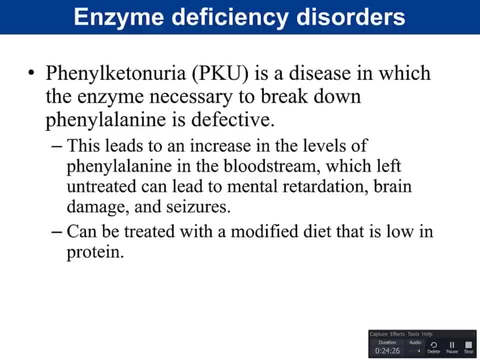 a modified diet that is low in phenylalanine And PKU can be treated with a modified diet that is low in phenylalanine And PKU can be treated with a modified diet that is low in phenylalanine And PKU. can be treated with a modified diet that is low in protein, And so it's simply through diet. 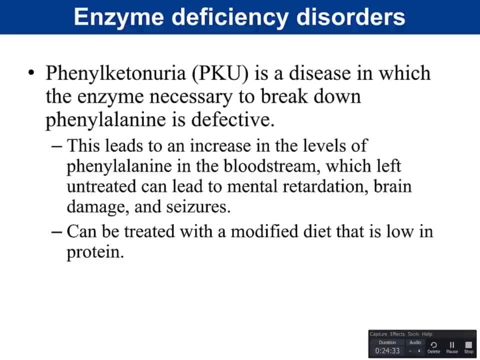 So people who have PKU have to be on a very low protein diet. My kids' uncles have PKU. they were both born with PKU and they basically have to be on a low protein diet. When they were kids they had to get their phenylalanine levels checked. 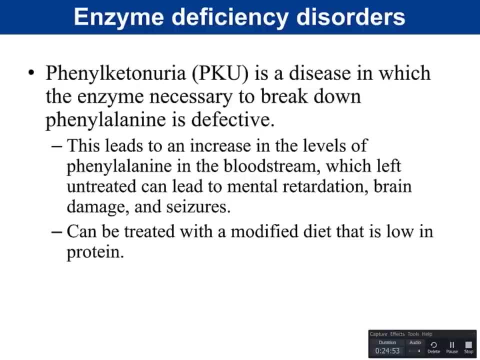 kind of like a diabetic has to often check their insulin levels. Somebody with PKU had to get their phenylalanine levels checked. kind of like a diabetic has to check their insulin levels. Somebody with PKU will have their phenylalanine levels checked. 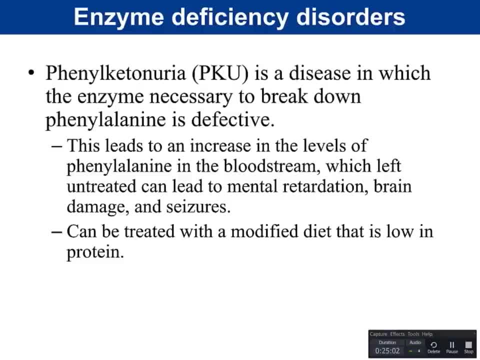 to make sure that it's being regulated properly so that the levels don't get too high and lead to damage. If the diet is followed, there are typically no problems associated with the disease. Patients can live very normal, healthy lives. They have to follow the diet, though They have. 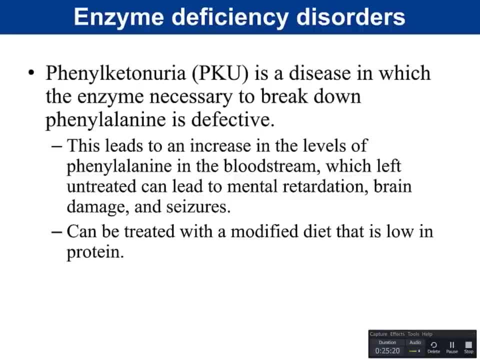 to eat low protein, And so that includes, basically, it's like being vegan. So no dairy, no meat. anything that's high in proteins has to be avoided. Now you might think, well, don't you need proteins? Answer is yes, you do. So these patients that have PKU, at least with 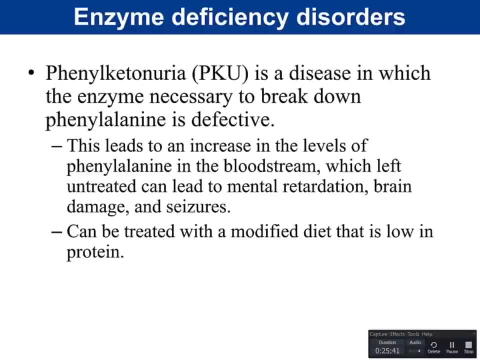 my kids' uncles. they have to drink this special milk. it's a prescription and it has the other amino acids that they need, but it does not contain phenylalanine, And so this allows them to get the other amino acids while not taking in phenylalanine, And so 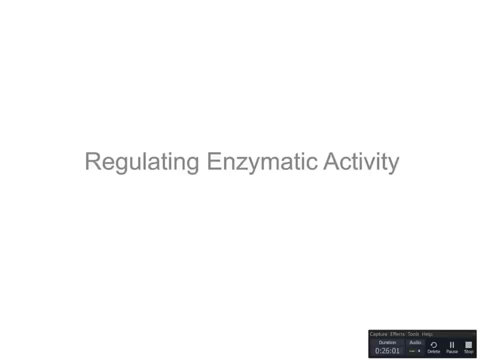 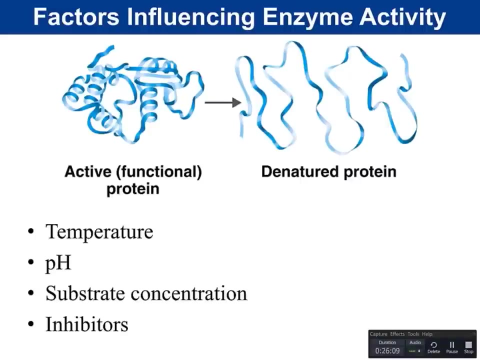 this is an example of an enzyme disorder. So next we're going to talk about regulating enzymatic activity, And so there are several factors influencing enzyme activity. Remember that enzymes are proteins and that proteins only function if they're in their correct conformation. If they unfold, they become denatured and they no longer function. 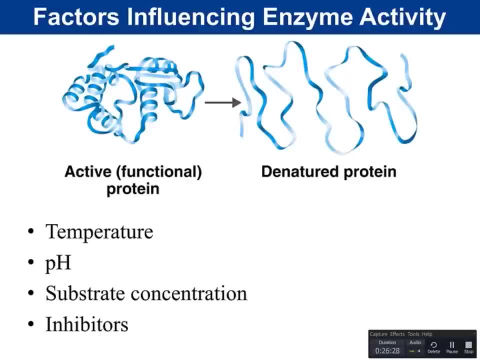 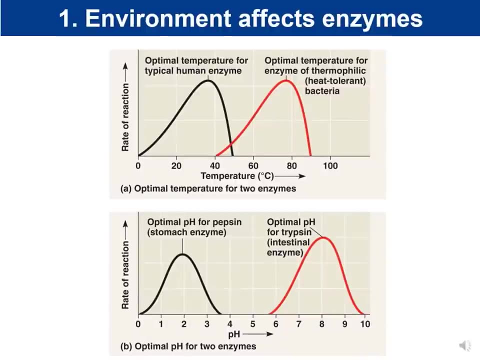 There are several factors that we're going to talk about and how they influence enzymatic activity. We will talk about temperature, pH, substrate concentration, as well as inhibitors. So the first part is looking at how the environment affects the enzyme and again looking at how temperature and pH play a role. So the top one- 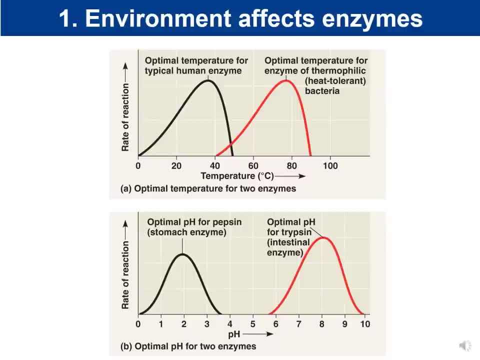 you're looking at the effect of temperature on the enzymes. So the black line is a typical human enzyme. And notice that if we're looking at the rate of reaction for that black line, the enzyme functions optimally about 37 degrees Celsius, which makes sense, right? Because our 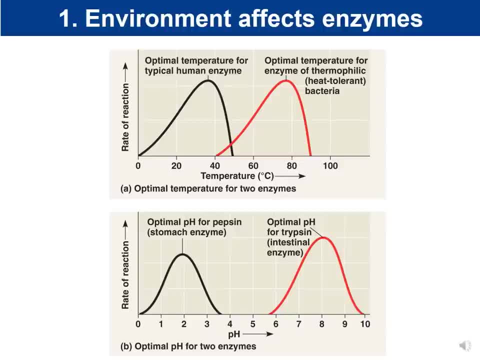 enzymes are in our body, so they should work best at human body temperature. If we get above about 45, our enzymes will denature. If the temperature is too low, right, it's going to decrease molecular motion, which is going to decrease the rate of the reaction. So temperature is going to. 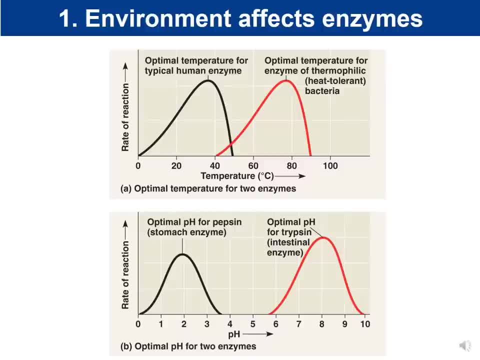 play a role in how the enzyme works. If I look at a thermophilic or heat-tolerant bacteria, that thermophilic bacteria is used to growing at high temperatures and so notice that its enzymatic activity is not optimal at human body temperature, which is why many thermophiles 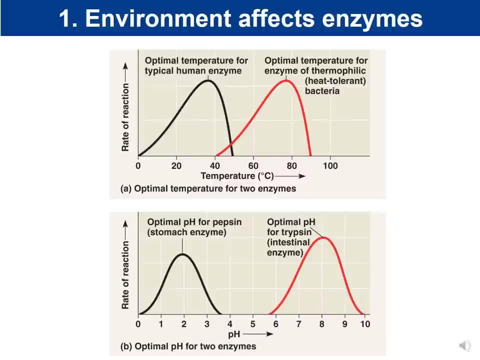 don't cause human disease because their enzymes are not active at our body temperature, But that enzyme instead functions at a higher temperature. so about 70 or so. It stops functioning at about 40,. it stops functioning at about 90, but notice that. 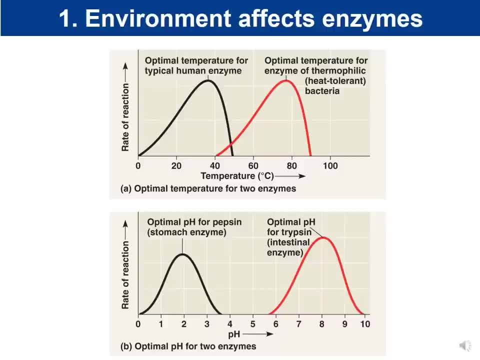 its range of optimal temperatures is different than that of human enzymes. Our range of temperatures is different than a thermophile. Think about what that means. Remember how I said that temperature influences molecular motion. If I raise the temperature, molecules are going to move faster, and if the 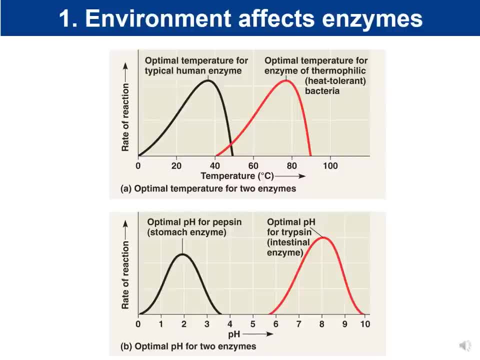 temperature becomes too high, it causes proteins to denature. So if you think about the types of interactions between the R groups, you want to think- if I'm thinking as a scientist and I'm thinking about protein structure- right, And I want to know: what is it about these enzymes in the thermophiles that allow them? 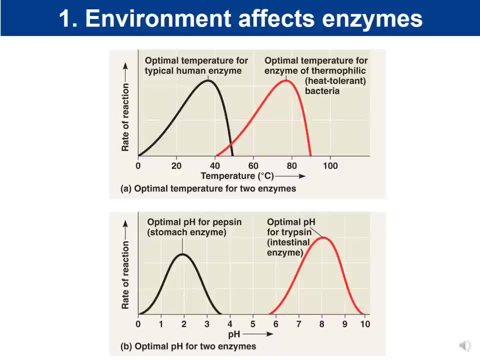 to work better at higher temperatures. What are the adaptations that those organisms have that allow those proteins to not denature at higher temperatures? And the answer is that it's the types of amino acids that are in those thermophilic bacterial enzymes that will influence the fact that they can withstand higher temperatures. 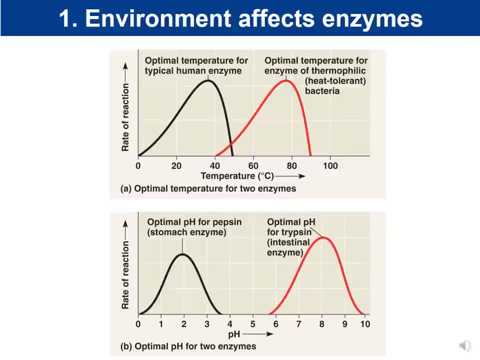 So, if we talk about our types of interactions, so again we have our hydrophobic interactions, we have ionic interactions, Remember. those ionic interactions, though, are within a cell, which is aqueous, meaning there's water. We have hydrogen bonds and we have covalent bonds. 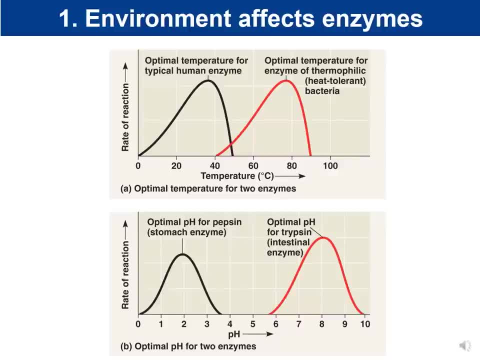 Of those four types of bonds, which type would you expect to see more in the thermophilic enzymes, In thermophiles? which ones are going to make those proteins the most stable? And the answer is: those bacteria that live at higher temperatures have more covalent bonds. 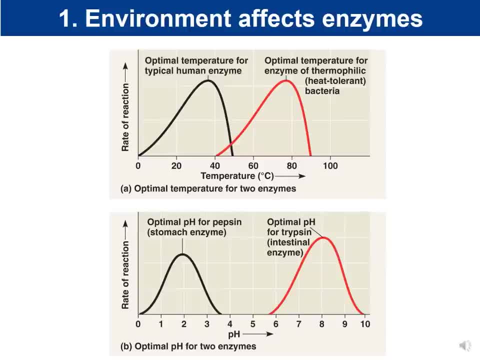 They have more disulfide bridges because that covalent bond is very strong. Ionic bonds are strong when not in water, but in water that ionic interaction is weaker. So bacteria that are thermophiles have a lot more disulfide bridges, which means that their proteins have more cysteine amino acids. 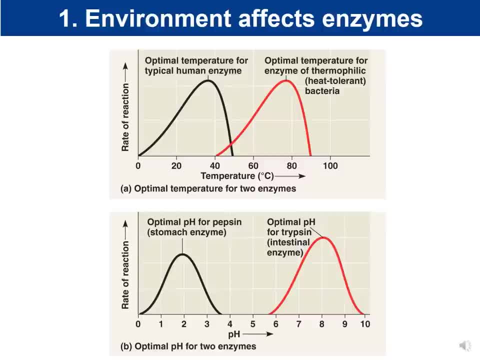 because those cysteines are going to form those disulfide bridges, And those disulfide bridges are what are responsible for holding that protein together. So just a little something to get you thinking right about. well, why do enzymes function? 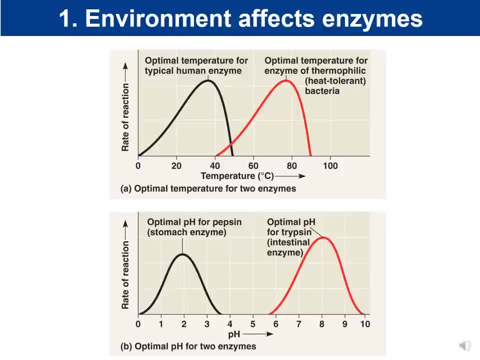 different at different optimal temperatures. It has to do with protein Structure, has to do with the sequence of the amino acids. The sequence of the amino acids is going to dictate the way that the protein folds In terms of optimal pH. different enzymes in our body have different optimal pH. 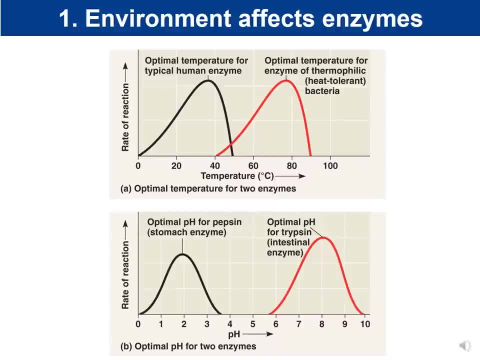 So even within the same organism, there might be enzymes within the body that function at different optimal pHs. So pepsin: Pepsin is an enzyme used to Break down protein right, and pepsin is an enzyme that is produced in the stomach. 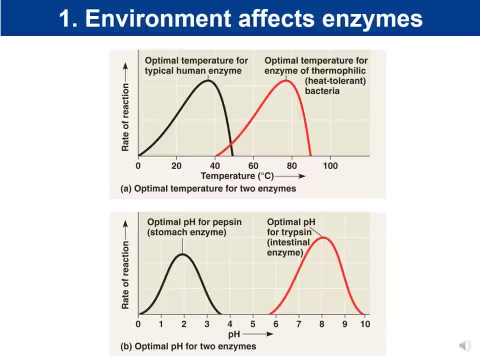 So if you look at the optimal pH for pepsin, notice that it peaks at about two. That makes sense, because our stomach is a very acidic environment and so pepsin needs to be able to function at that very low pH. Trypsin is a different enzyme. 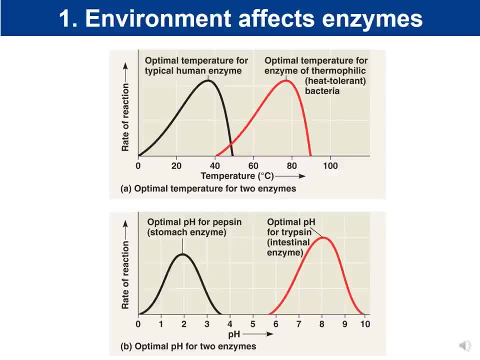 It also is used to metabolize proteins, So to help break down proteins. but trypsin is an intestinal enzyme, meaning that it's produced and then sent to the intestines to help break down the proteins in the intestines. The intestines are not very acidic and in fact they're more on the alkaline side. 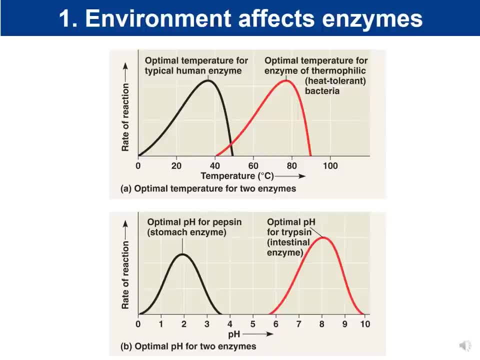 So as the food goes from the stomach to the intestines, that food gets neutralized, And so the intestine is going to be a slightly alkaline type pH. So notice that trypsin functions optimally at about a pH of eight. It does not function at all at a pH of two. 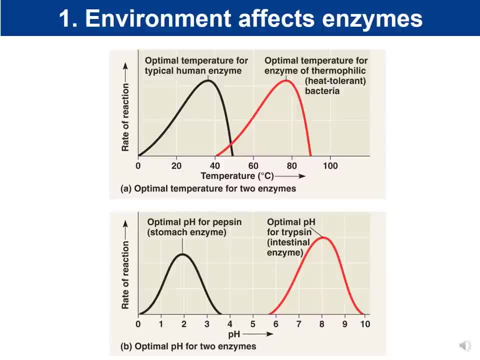 Pepsin, which functions best at a pH of two- notice- does not function at a pH of eight. They each have their own optimal range through which the enzyme is active. So even within our own body we have different enzymes that have different optimal pH. 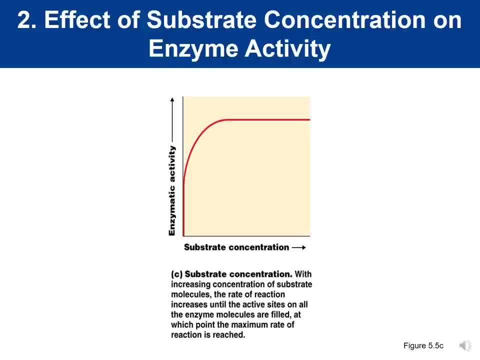 So the next variable, The next variable that affects enzymatic activity, is the substrate concentration. So if we increase, so if we increase substrate concentration, we will increase reaction rate Until saturation is reached. So we'll write it and then I'll explain it. 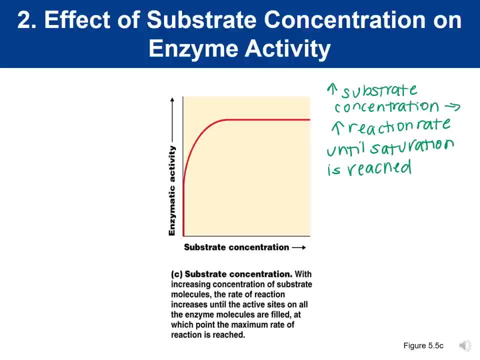 So if we increase our substrate concentrations, we will increase the reaction rate until saturation is reached. So what do I mean by that? Well, if you think about it, if I add more substrate- right. if I put in more substrate, that makes collisions between the substrate and the enzyme more likely, right? 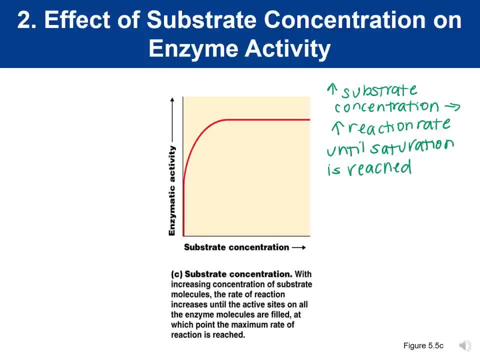 They're going to come in contact more likely because I have more substrate available to bind to that enzyme. So as I add more substrate, the reaction rate increases. Now notice that at some point we reach what is referred to as saturation, And what that means is that adding more substrate. 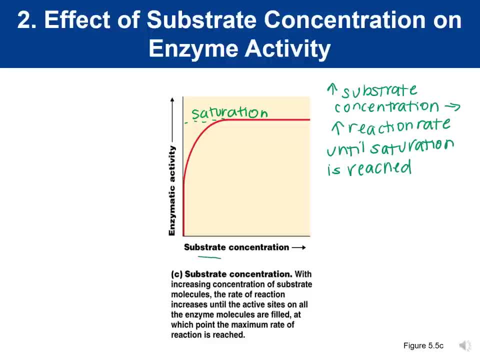 So notice this is our substrate concentration. Adding more substrate, once it gets to this point, no longer increases the reaction rate, And the reason for that is is that at some point- So let's say you had, Let's say you had- 10 enzyme molecules and you started with one substrate, right? 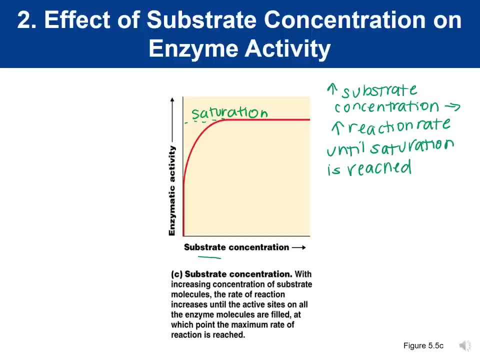 Or let's say we start with two. So if I have 10 enzymes and two substrates, adding three substrates or four substrates is going to make the reaction go faster because I still have enzyme available. However, once I have 10.. 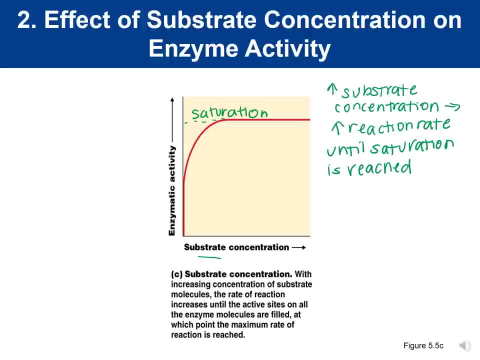 Substrates and I have 10 enzymes Adding 11,, 12, 13.. 1415- adding more substrate is not going to do anything. It's not going to make the reaction go any faster because I only have 10 enzymes available. 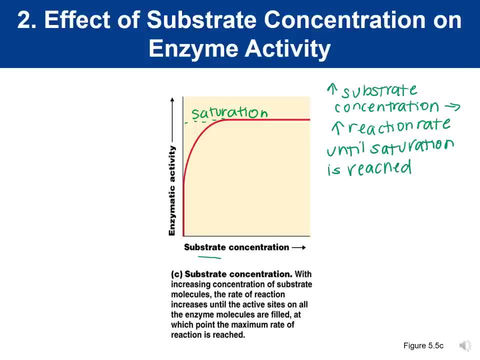 My enzymes are now the limiting factor, And so if I don't have any more enzymes available, adding more substrate is not going to make the reaction go any faster. That's what it means when we talk about saturation. So the substrate becomes saturated. 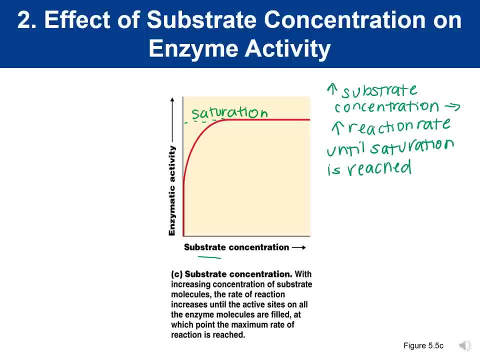 Yeah, There's no longer enough enzymes to make the reaction go any faster than it's already going. So you can think of this like um monkeys in a banana, right? So let's say you take monkeys and you put them in a room and you give them some bananas. 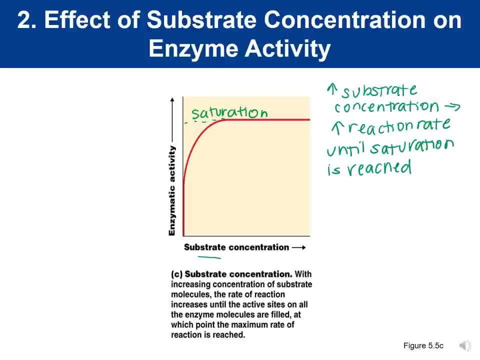 right, They're going to start to eat those bananas And as you add in more bananas- right, as I added more bananas, which are going to be our substrate- Um, the monkeys are going to be able to eat them and it's going to happen faster. 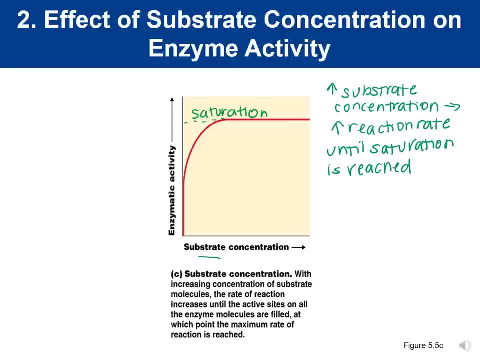 You're going to end up with more banana peels because there's more substrate available. However, if I take a dump truck and I just dump in a bunch of bananas, dump in a bunch of substrate, that's not going to make the reaction go faster at that point, because we've 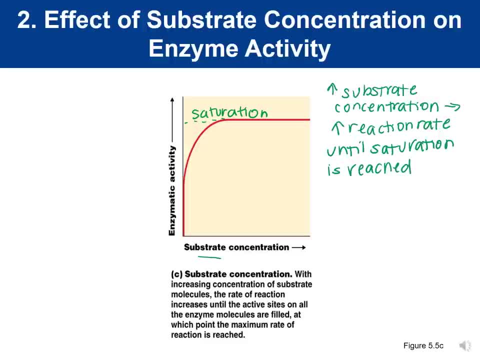 already reached saturation. There's only so many monkeys in the room to eat the bananas. Adding more bananas is not going to make the reaction go faster. Yeah, It's going to make the reaction go any faster, And so that is the effect of substrate concentration. 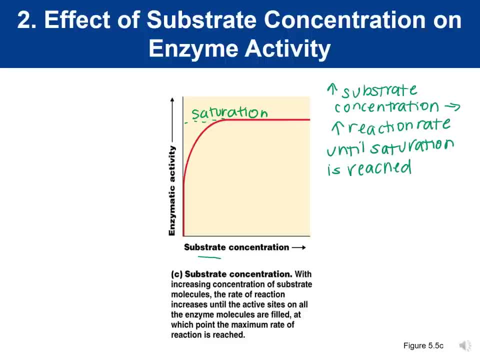 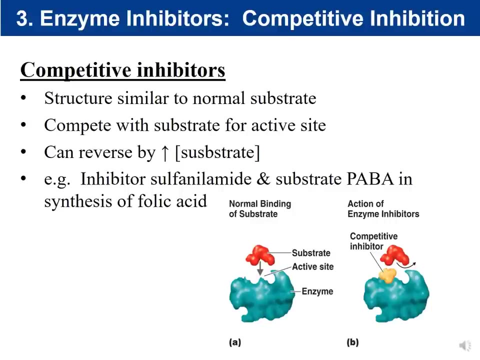 So if you increase the concentration of the substrates, you will get the reaction to occur faster until saturation is reached, And then there's no longer enough enzyme to make the reaction rate go any faster, And then we have our enzyme inhibitors. So our enzyme inhibitors. 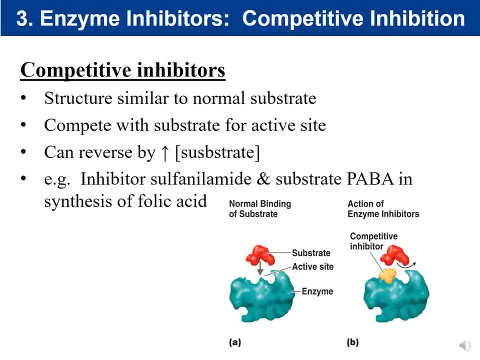 So our inhibitors are going to be molecules. They're going to be molecules that inhibit the enzymes, meaning that they turn them off. We're going to talk about two main types of inhibitors, And the first one that we're going to talk about is competitive inhibition. 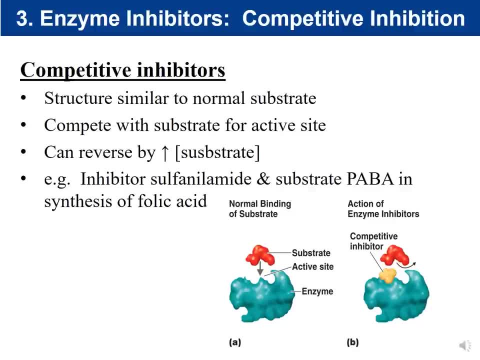 So competitive inhibition is where. so if you look at A on this bottom diagram, so the green is the enzyme, the red is the active site. So normally the substrate is going to bind to the active site And then the enzyme is going to catalyze that reaction. 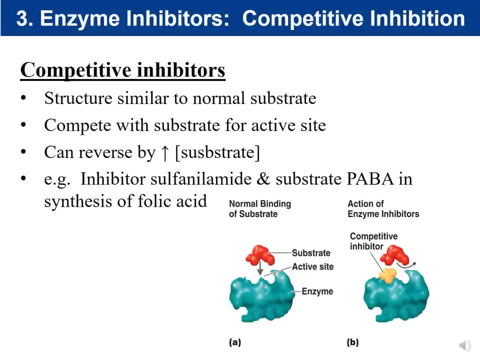 In the case of a competitive inhibitor. So yellow is the competitive inhibitor. The competitive inhibitor has a structure similar to the substrate, meaning structurally it looks very similar. Because they have similar structures, the inhibitor is going to bind to the active site. 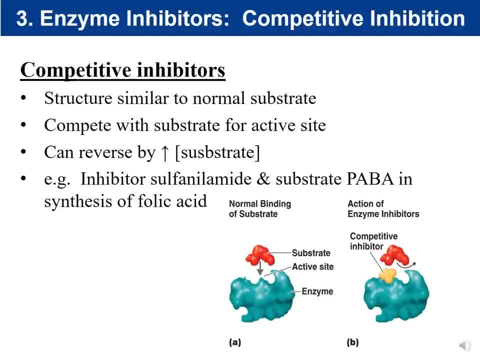 And when it binds to the active site, it prevents notice, it prevents the substrate from binding, Because the inhibitor binds the substrate from binding. inhibitor is sitting in the active site, which is essentially blocking, which is essentially blocking the substrate to get in. Think of it, if you've ever played basketball and you're trying. 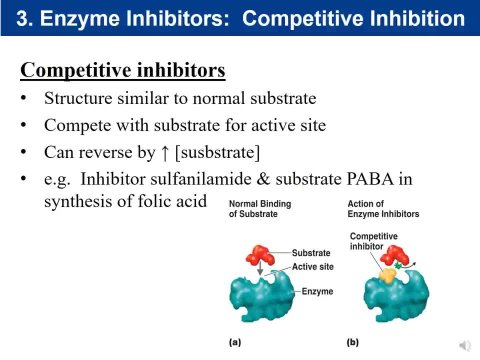 to get a rebound and you box out right, You push somebody out. If you do that, the ball's more likely to come to you because you're occupying that space. Same idea here. So this yellow, this inhibitor, is boxing out. It's preventing that substrate from getting in to the active site. 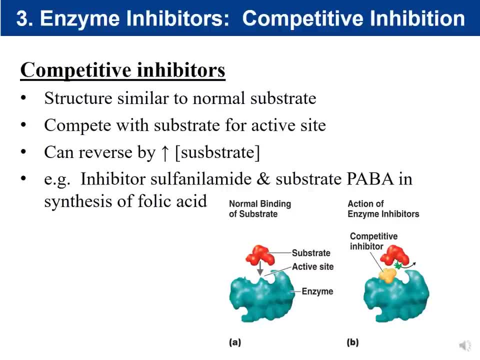 and having the reaction occur. So it does that because the inhibitor has a structure similar to the substrate, So both can bind to the active site, And so the competitive inhibitor. the reason it's called competitive is that it's competing with the substrate for the active site. 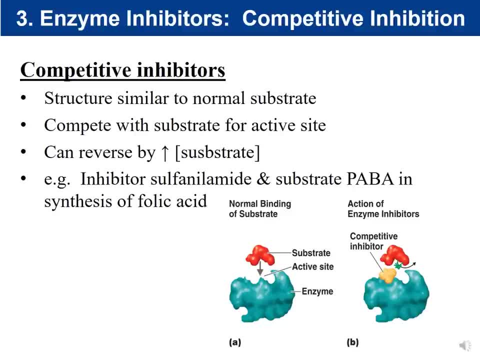 Now in competitive inhibition. um, this can be overcome by increasing the substrate concentration. So these little brackets around substrate refer to concentration. So this can be overcome by increasing the substrate concentration, Because if I now have more substrate again, it comes down to: 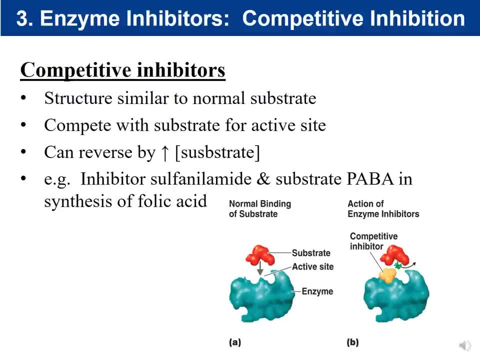 interactions between the substrate and the enzyme. More substrate means it's more likely to make contact with the enzyme if I now have more substrate than I do. inhibitor. So in competitive inhibition this can be reversed by increasing the concentration of the substrate. Now one example of competitive inhibition is to think about, if you ever know about. 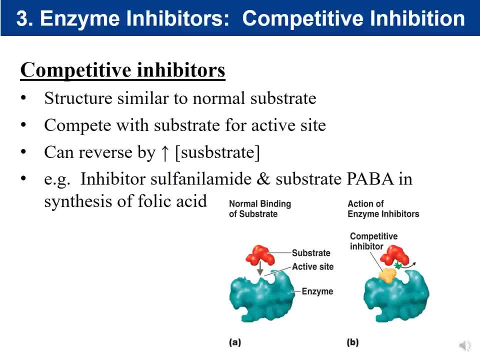 um, the statin drugs. The statin drugs are a class of um, a class of drugs that are used to lower cholesterol. So if you've ever heard of Lipitor, Lipitor is a drug used to lower cholesterol. Now, one of the things that you need to realize about cholesterol: 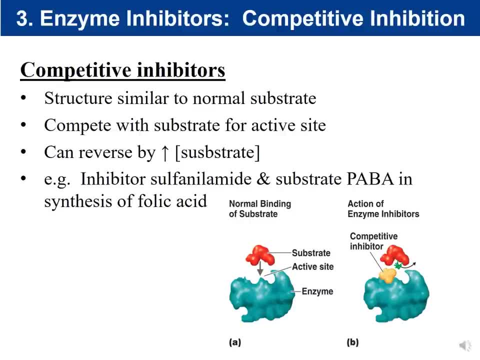 is that some people have what's called familial hypercholestemia. They are born with genetically high cholesterol. The reason for that is is that people that have this condition, they have a mutation in their LDL receptor And the LDL receptor binds to what's called LDL. 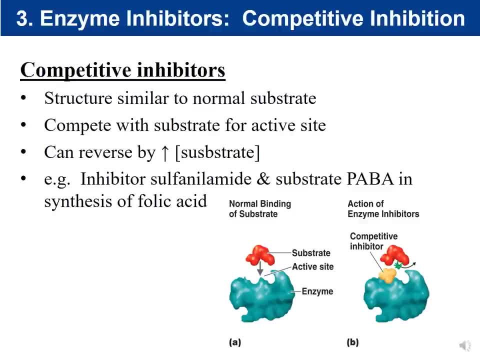 low density lipoprotein. LDL is a cholesterol carrier. It's going to help carry cholesterol through the blood. So what happens is is people who are born with familial hypercholestemia have mutated LDL receptors. Normally, the LDL receptors will bind to the LDL to help get cholesterol into the cell. 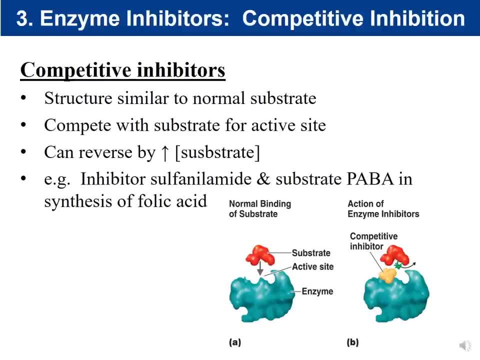 because your cells need cholesterol. for your cell membrane Cells in the gonadal tissue, uh, the testes, for example, use cholesterol to act as a precursor to make testosterone. So your cells do need cholesterol And so normally the LDL receptor binds to the LDL in the 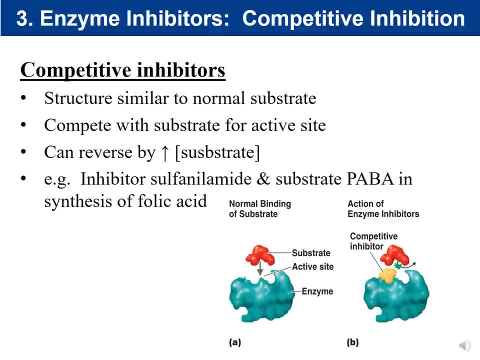 cholesterol And it helps bring the LDL into the cell, which keeps your blood cholesterol levels low, meaning within the normal range. If somebody is born with familial hypercholestemia, So if you, let's say, a trend where in all the generations you're seeing high. 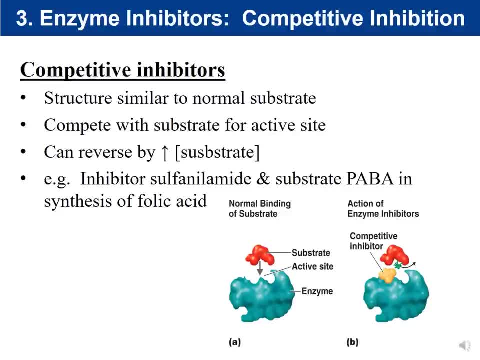 cholesterol, even though the person has a good diet and is healthy. if you see that trend, it's likely that that family has that familial hypercholestemia and that is, their LDL receptors are mutated. LDL does not bind to the receptor, which means that the LDL stays in the bloodstream, that cholesterol stays in. 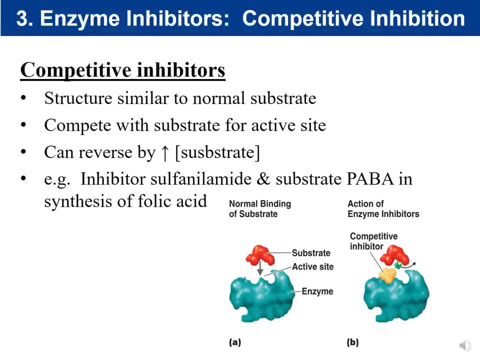 the bloodstream and that leads to abnormally high cholesterol levels. right, because when we get our cholesterol levels checked, we're looking for cholesterol in the blood. if the LDL can't get into the cell, the cholesterol stays in the blood and you lead to elevated cholesterol in the blood. now 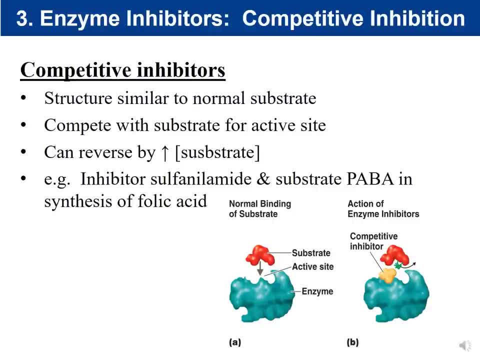 currently we don't have a way to really fix the LDL receptors, so that is not the approach of cholesterol lowering drugs. the way that that's called on episodes- when you suppress them, essentially there's a like Lipitor work- is that, instead of targeting the LDL receptors to help get 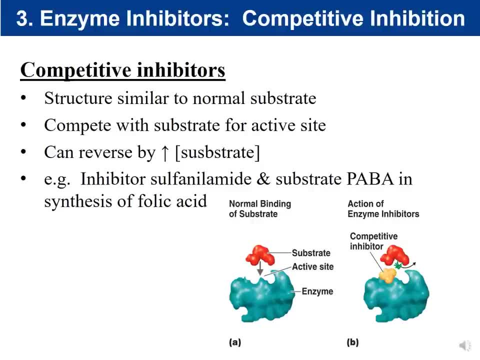 LDL in. instead, Lipitor acts on the liver cells to inhibit the production of cholesterol, So normally your body, in the liver, is going to synthesize cholesterol. So the way that Lipitor works is that it's going to inhibit cholesterol from being produced, And the way that that works is that there's an 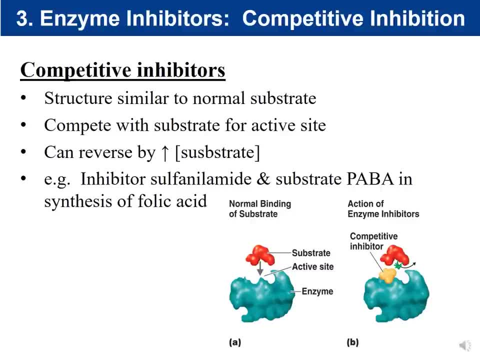 enzyme that normally will take a cholesterol precursor and it will take that cholesterol precursor and convert it into cholesterol, meaning that's how your body is going to produce cholesterol. Lipitor is a competitive inhibitor for that enzyme, So Lipitor comes in and it binds to that enzyme and 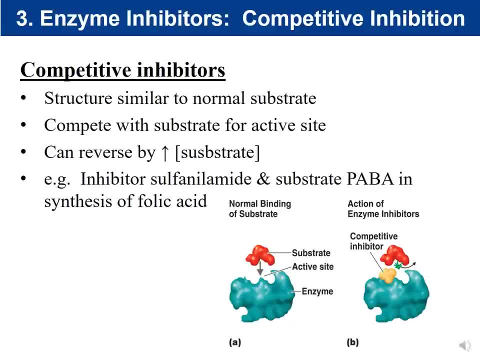 it prevents the cholesterol precursor from binding. And when it prevents the cholesterol precursor from binding, it's going to block the production of cholesterol and the body is not going to make cholesterol or as much, and that will end up lowering the patient's blood cholesterol levels. So that is one. 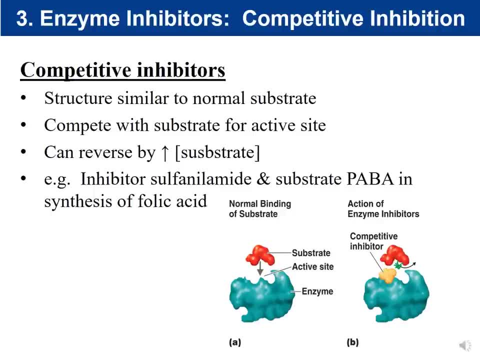 example of a competitive inhibitor. So Lipitor its job to reduce cholesterol levels and it does so by inhibiting the production of cholesterol. Another example that we're going to talk about- and again we're going to talk about this more in our lecture on antibiotics, but in the 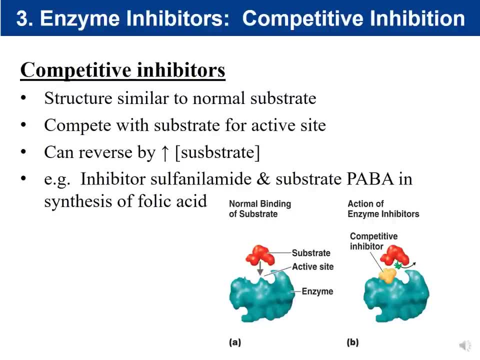 lab we learned about sulfanilamide, And sulfanilamide is a competitive inhibitor for an enzyme that normally will take PABA- something called PABA, which we'll talk about in a second- and will convert PABA to folic acid. 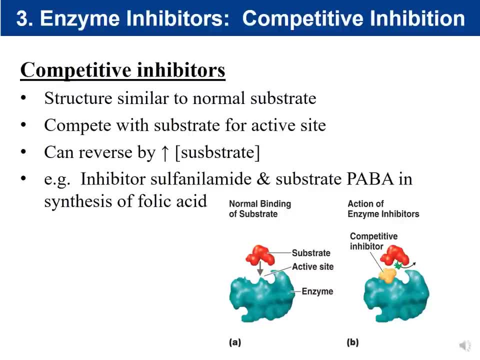 Now bacteria produce folic acid to make their nucleic acids, And so by taking sulfanilamide it's going to inhibit bacteria, because bacteria can't synthesize their folic acid. So let's walk through and see how that works. So 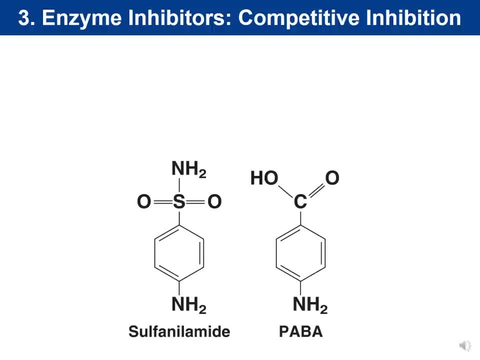 what you're seeing here is, on the left, we have sulfanilamide, so that's our antibiotic, And we have PABA, which is normally our substrate, And so PABA- let me change my ink here. So PABA is para-amino benzoic acid and it's an essential and essential. 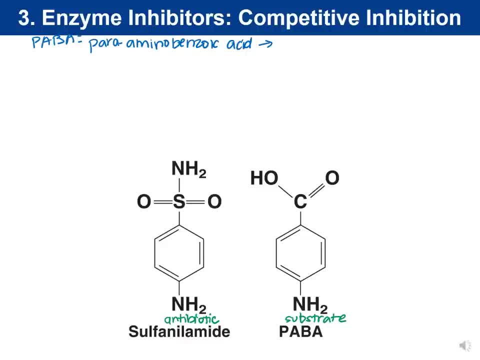 to all sleep disorders. It'sварic acid is an absolute mineral that alight Adam. 이걸 переход refers between liar advocate. This is called illec, although Italyそれ babouch o, because he's no leprosy or something and disease or something heで. 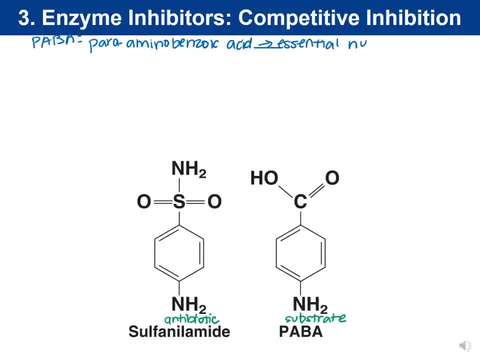 nutrient used by many bacteria in the synthesis of folic acid. so it's used by many bacteria in the synthesis of folic acid and folic acid is used to make nucleic acids. now, how does sulfonylamide work? okay, well, again, PABA is our. 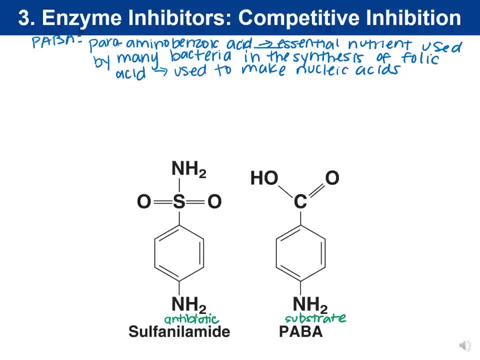 substrate and there is an enzyme that binds PABA and converts PABA into folic acid. so the way that sulfonylamide works or sulfa drugs work, so sulfonylamide is a competitive inhibitor and binds a to the active site. active site of the 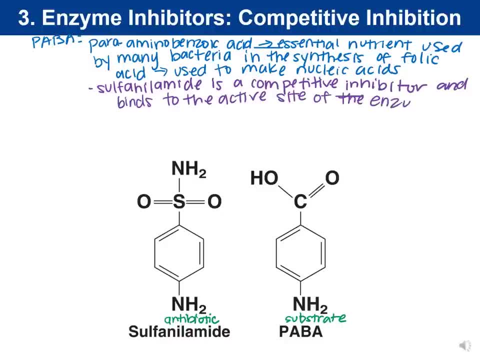 enzyme that converts. that converts PABA- whoops, PABA- to folic acid- flourish mistake. yeah, yeah, yeah, yeah, yeah, yeah, yeah, yes, yeah, yes, yes, yes, yes, Sure, Yeah, known as that bombshell theaters or nucleic acids as a result, and it inhibits bacterial growth. so it is what. 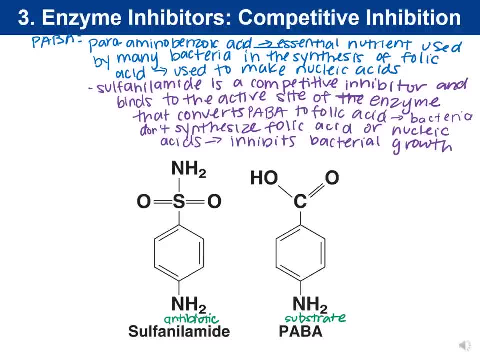 we call bacteriostatic. it's going to inhibit bacterial growth, because if the bacteria can't make folic acid, they can't make nucleic acids. if they can't make their nucleic acids, they can't replicate their DNA when they go to divide. so sulfanilamide is an antibiotic and the way that it works is it's a. 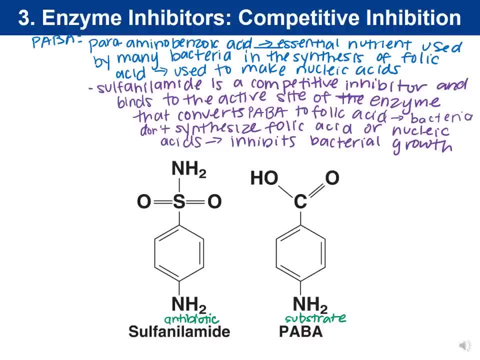 competitive inhibitor for the enzyme that normally binds to PABA, because, again, notice that their structure is very similar, especially the bottom part, so it's structurally similar to PABA. sulfa binds to the active side of that enzyme. it prevents PABA from binding and when sulfanilamide is bound, the bacteria can't make folic acid or nucleic acids. 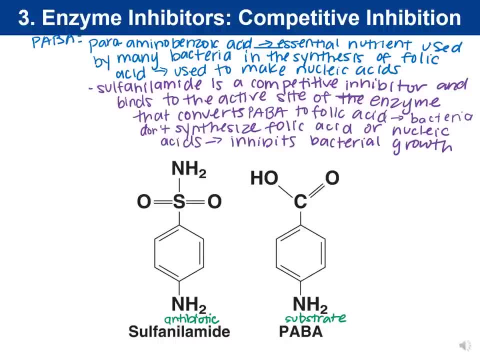 and it's going to inhibit bacterial growth. now, interestingly and again, something we're going to talk more about when we get to our antibiotic lecture is that when we choose antibiotics, we want an antibiotic that has what we call selective toxicity, meaning that it targets the microbe without 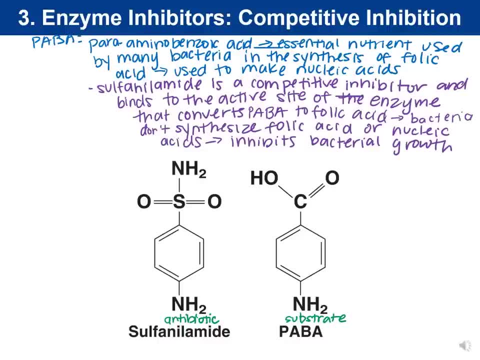 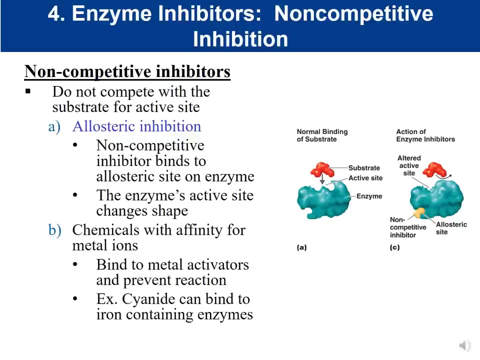 affecting the host, or affecting it at least less so. sulfanilamide is selectively toxic and that's because humans do not make folic acid. we get it from our diet. So this, so that drug will basically affect the, it'll affect the bacterial. 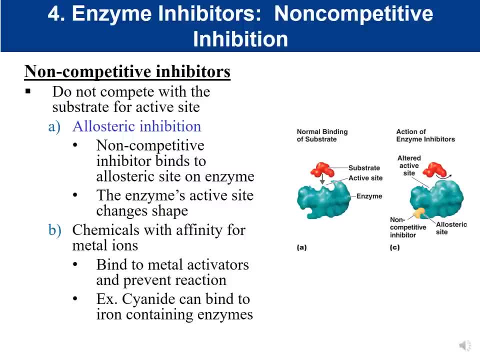 cell without affecting our cells. Now for non-competitive inhibitors. non-competitive inhibitors work in a different way And because it's non-competitive, notice that it's not competing for binding to the active site. So in this case the inhibitor does not bind to the 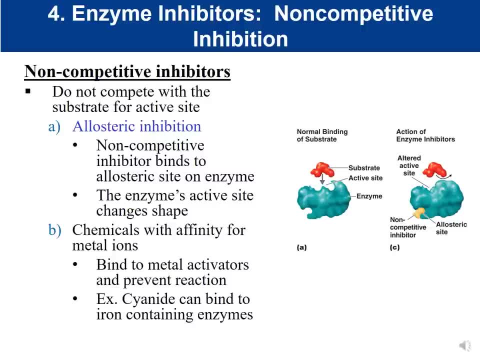 active site. Instead we could have what's called allosteric inhibition. Remember that allosteric means other site Binds somewhere other than the active site. So notice that here the yellow, this non-competitive inhibitor, is binding at this allosteric. 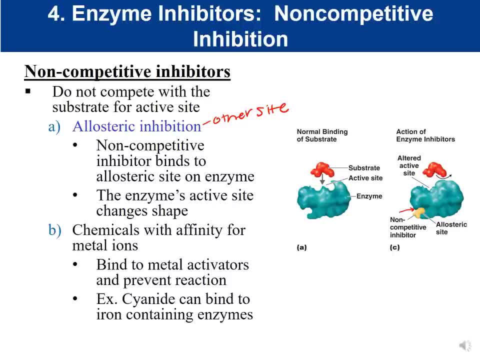 When it binds at the allosteric site. what ends up happening is is that when the inhibitor binds, it causes the enzyme to change shape. So notice that the enzyme no longer looks the same. Look at the active site. So if you compare A and B, look at the shape of the active site in A. 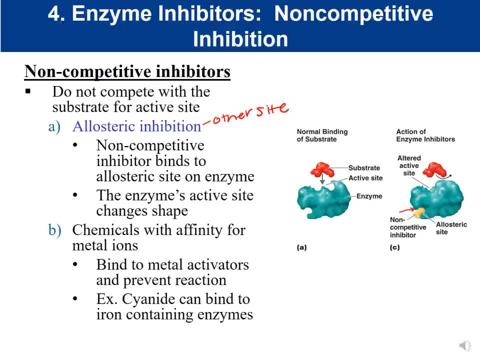 look at it in: actually that says C in C. So compare that with C, The active site. the shape has changed because when the non-competitive inhibitor bound to the allosteric site, it bounds somewhere other than the active site. It caused the enzyme. 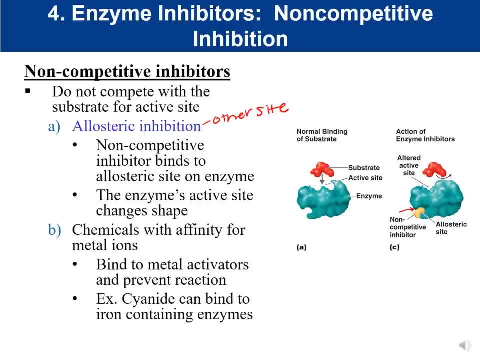 to change its shape. And when the enzyme changed its shape, the active site became altered And now the substrate can no longer bind. Now, when you talk about allosteric inhibition cannot be reversed by adding more substrate, And that's because in this case they're not competing for the same binding site. 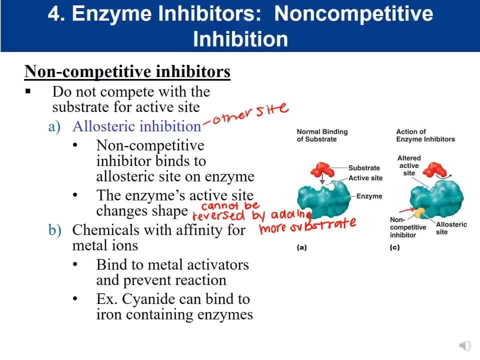 right. They're not competing for the same binding site. The non-competitive inhibitor is binding somewhere other than the active site. So this is different Competitive inhibition. we can overcome that by adding more substrate. Non-competitive inhibition or allosteric inhibition cannot be overcome by adding more substrate, because it's 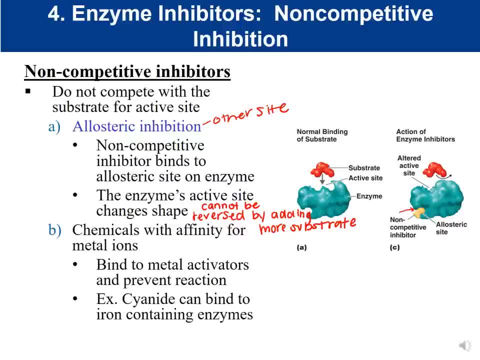 binding somewhere other than the active site. Now, in terms of non-competitive inhibitors, we can also have chemicals that have an affinity for metal ions, meaning that they bind to metal ions and they prevent the reaction. So notice, an example of this would be to bind to metal activators. 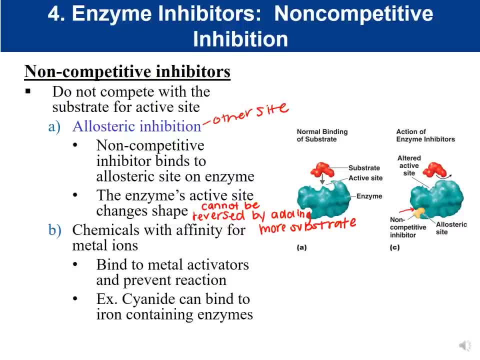 and prevent a reaction. Cyanide, for example, can bind to iron And when it binds to iron and it binds to iron-containing enzymes, it's going to inhibit the reaction from occurring. So it's going to make that cofactor not be a cofactor, meaning it's going to block. 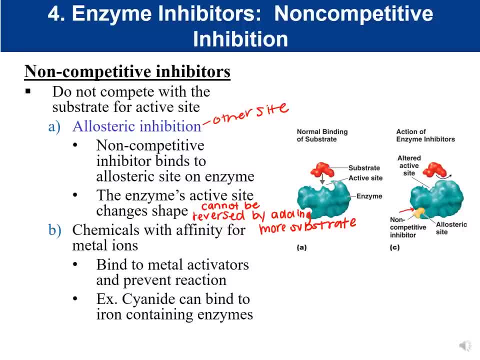 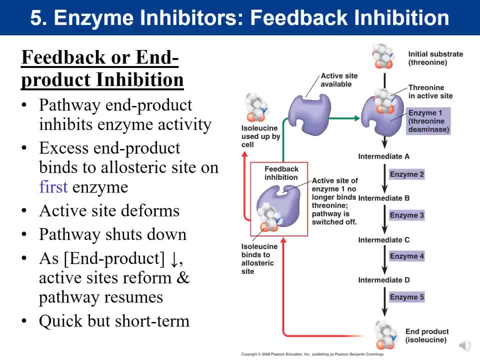 that reaction from happening, And so that is non-competitive inhibition. Along the lines of inhibition or allosteric inhibition, we can have what's called feedback or end product inhibition, And that is where the product of a particular pathway can feed back and turn off an earlier step in the pathway. So what do I mean by that? 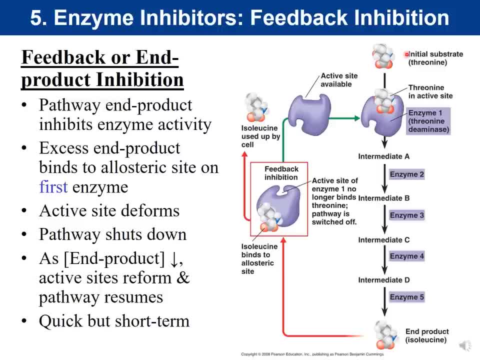 So let's take a look at this example. So here we have, cells can convert three and anine, which is an amino acid, into another amino acid called isoleucine, And so there are several steps along the pathway that will convert that three anine to isoleucine. And so notice that 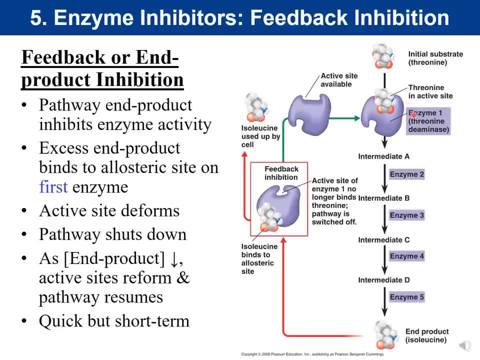 we have five enzymes in this pathway: Enzyme one, two, three, four and five, And after this fifth enzyme we end up with our product, which is isoleucine. So if isoleucine levels are low, 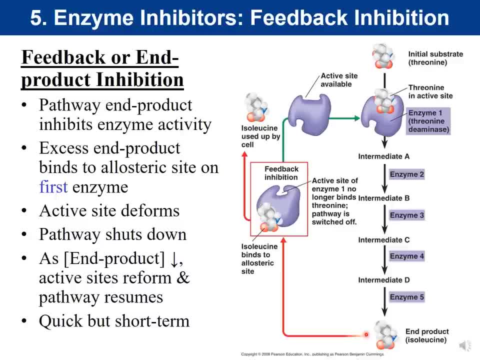 if the cell does not have enough isoleucine, this pathway is going to be turned on. So three anine is going to bind to the active site of the first enzyme, which is called three anine deaminase. I will not ask you the name of that enzyme. Three anine will bind to the active 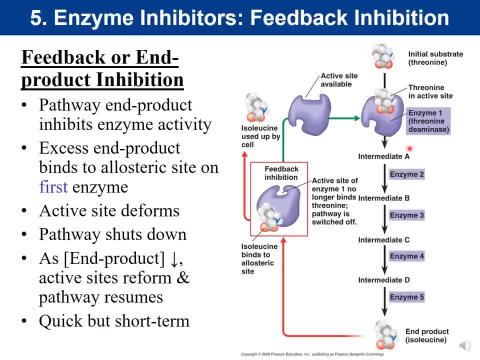 site of this enzyme. It will convert the three anine into this intermediate A, converts it to intermediate B, so on and so forth, until eventually we end up with isoleucine. Now isoleucine, though, let's say that the levels of isoleucine gets high in the cell. 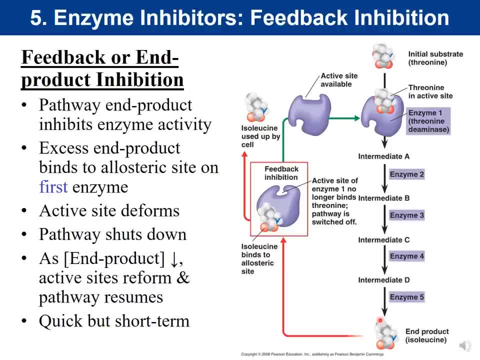 right If the level of isoleucine in the cell gets high. we don't want this pathway to be on. We don't want to continue to convert three anine which we get from the diet to isoleucine which we make. If we have enough isoleucine we want to save that three anine. 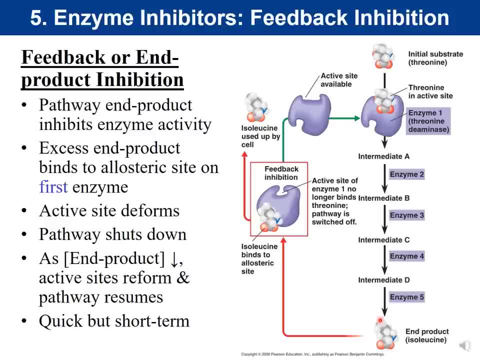 We don't want to utilize it and form more isoleucine if there is already enough, And so the way that that works is that the isoleucine binds to the allosteric site on this first enzyme. So see this little site here: Isoleucine binds to that allosteric site. 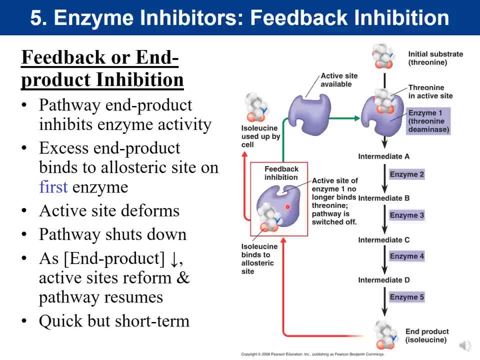 When it binds, it causes the enzyme to change shape, and now three anine cannot bind to the active site, And so that is going to inhibit this reaction. So as we get enough product, that product is going to feed back, It's going to communicate with its own pathway and it's going to turn off. 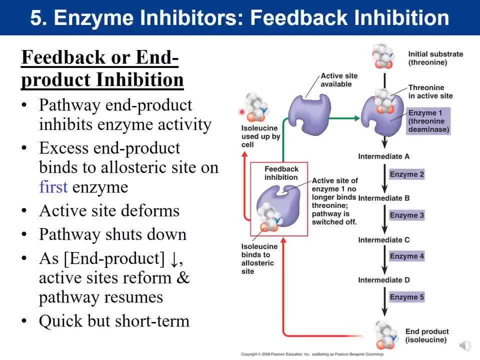 or inactivate this enzyme. Now, as the isoleucine is used up by the cell, so as the cell is utilizing the isoleucine to make its protein, isoleucine is going to come off. It's not going. 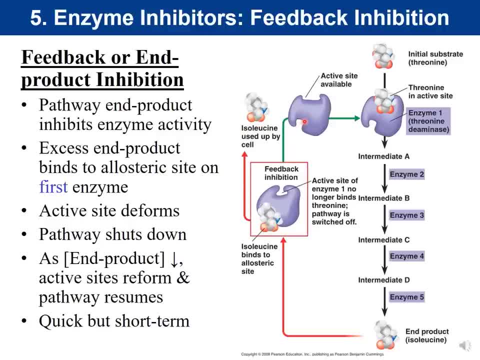 to be bound to the enzyme anymore. It's being used by the cell. Now the enzyme is going to change its shape back because it's not bound to isoleucine. It's going to change its shape back and it's going to change its shape back. So that's why it's so important that the active 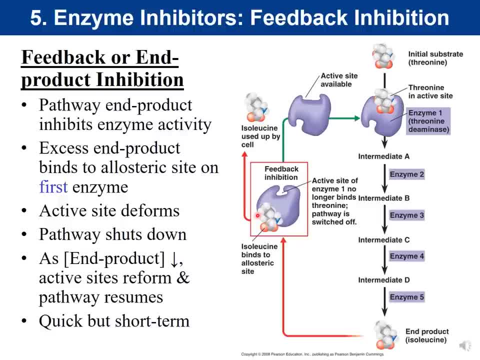 site is available and in its correct shape for the three anine to come in and bind and for the reaction to occur. And so this pathway is totally dependent on the concentration of the isoleucine. If there's not enough, the enzyme is active and the cell is going to produce isoleucine. 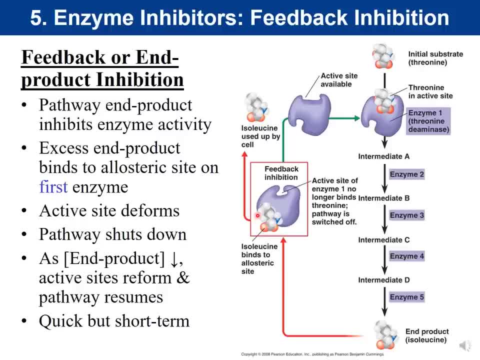 If, on the other hand, there is an excess of isoleucine, the cell does not want to keep making isoleucine. The isoleucine feeds back and it turns off an enzyme in its own pathway. It's basically shutting off its own pathway. So this type of regulation is quick. It happens very. 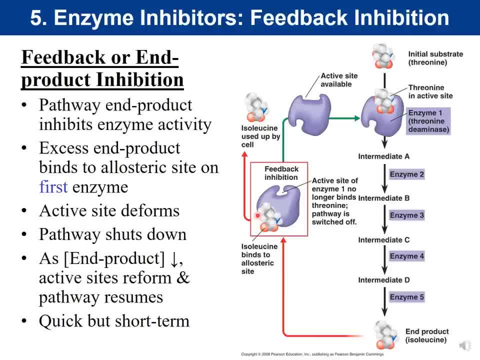 quickly, but it's short-term, meaning it's not long-lasting, because as soon as that product comes off, the reaction is ready to start again. And so, again, this is our feedback inhibition: The product is going to feed back and it's going to inhibit its own pathway, So that is what we call feedback inhibition. 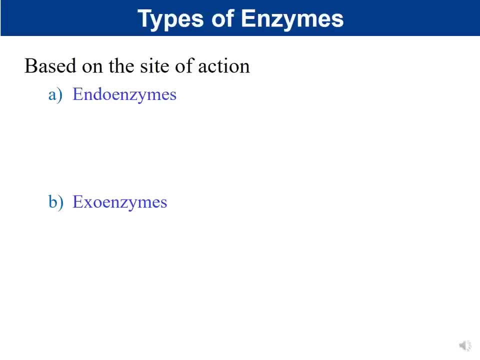 Now in terms of our types of enzymes, and again this goes with what we have learned in lab about endoenzymes and exoenzymes. So endoenzymes are those enzymes that stay inside the cell or are secreted. Endo means within, So these are inside the cell. 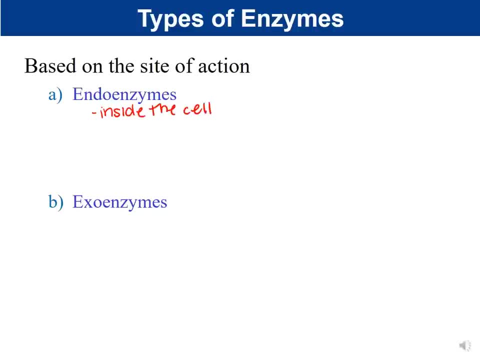 Are the substrates for endoenzymes usually larger substrates or smaller. And again, usually smaller substrates Because the substrates can get into the cell and therefore these enzymes can be within. so usually smaller substrates And usually. 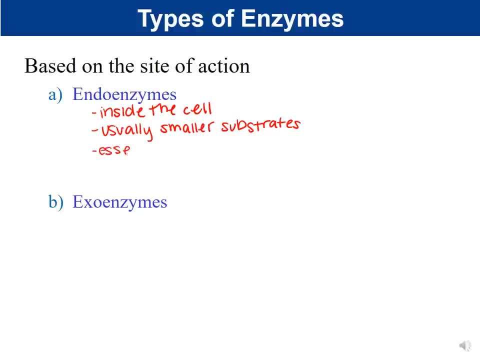 these enzymes are essential to metabolism. They are absolutely required. So enzymes in glycolysis, for example, would be in endoenzymes. The cell requires them. They're essential to metabolism. These enzymes need to be in the cell Exoenzyme. on the other hand, 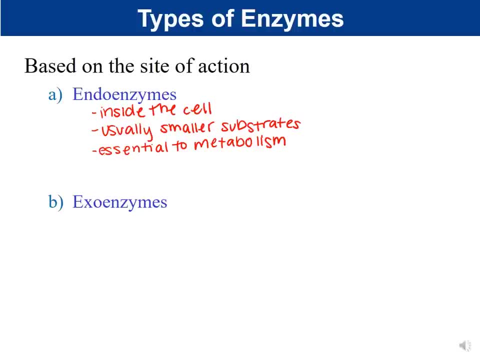 exo, remember, think exit. Exoenzymes are going to be secreted outside of the cell, And so if we think about our substrates for exoenzymes, usually we're going to have a lot of exoenzymes And so we're going to have a lot of exoenzymes. 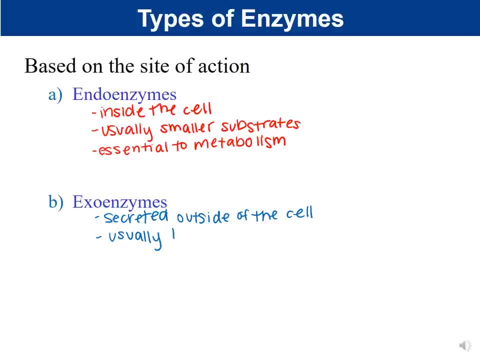 So we're going to have a lot of exoenzymes And so if we think about our substrates for exoenzymes- usually larger substrates, So the substrate could be like starch, for example, casein, gelatin, etc. Those larger substrates- they're too big and bulky, They can't get into the cell. 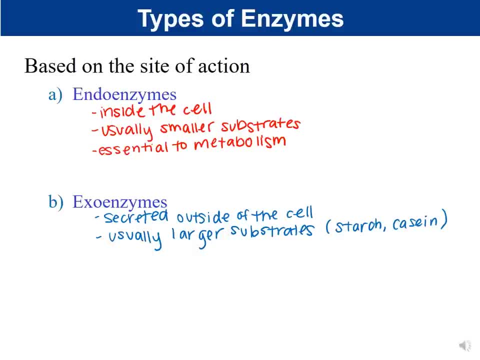 So instead the bacteria is going to secrete those enzymes out of the cell and it's going to break down the substrates outside of the cell and then transport the smaller products in. In terms of the function of endoenzymes or, I'm sorry, in terms of the function of exoenzymes, usually not. 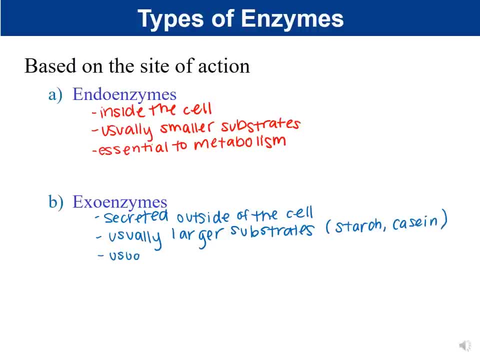 essential, Usually to help metabolize agriculturally unusual fridge, unusual food sources Or larger food, Or used to neutralize episodes of the Davis newborn prolapse�, harmful using stomach 엄마 Ebolaitel's microbiological responses. So that so it's very likely. So we're going to want to solve this issue or navigate the team andż. 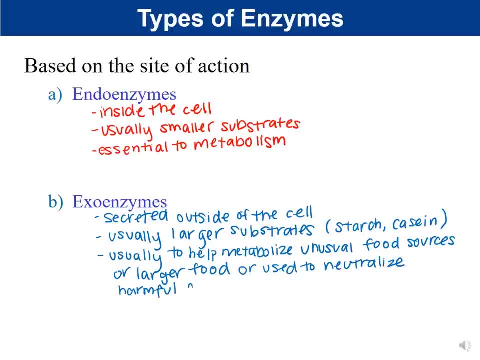 chemicals. And an example of this last one, think urease. right. So urea is a small substrate. however, urease is an exoenzyme because the bacteria, like Helicobacter pylori, is going to secrete urease outside of its cell and that urease is going. 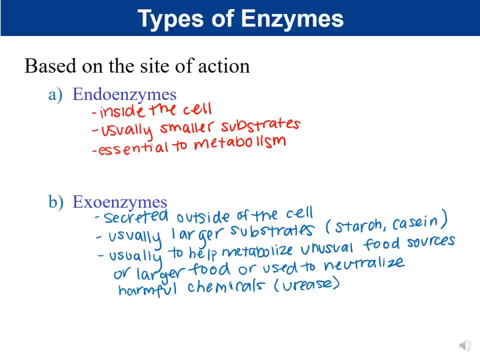 to take the urea in the stomach and it's going to convert it into ammonia. And when it converts to ammonia, that is used to help neutralize the stomach acid which allows Helicobacter pylori to live in the stomach. So exoenzymes are used for a different purpose than endoenzymes. 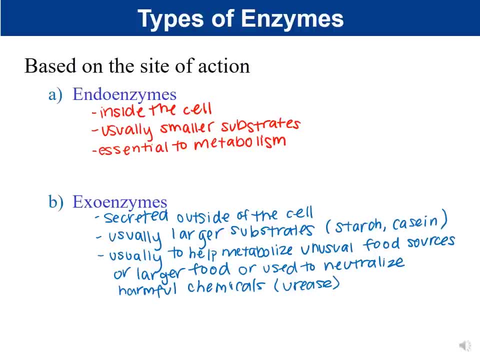 Endoenzymes are essential to metabolism. We've seen a lot of endoenzymes in class. We have our d-carboxylase, our d-aminase- right, We have beta-galactosidase, etc. 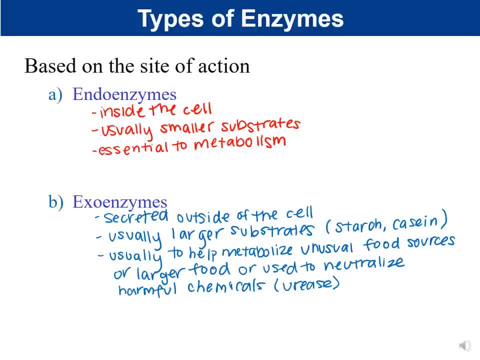 These are endoenzymes, they're within the cell. Exoenzymes are for a different purpose: right, Metabolize unusual food sources or larger food. So again, intact proteins, intact polysaccharides like starch, or they're used to neutralize. 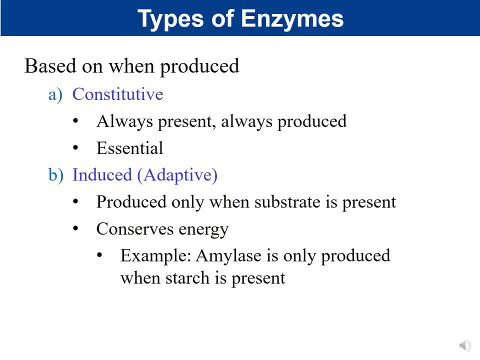 harmful chemicals like urease does. Enzymes can also be classified based on when they're produced, And so some enzymes are what we call constitutive. They're constitutive because they're always present. they're always produced. The cell makes these enzymes all the time. 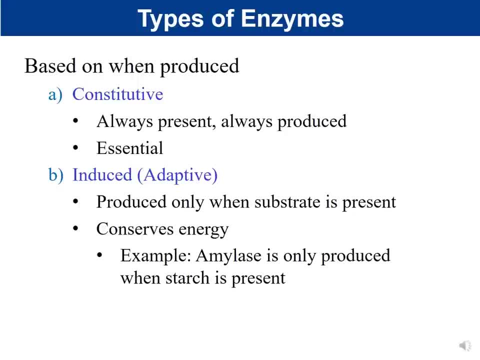 These enzymes are again essential to metabolism. The cell must have those enzymes. They're always present, Those enzymes. So an enzyme in glycolysis, for example, might be a constitutive enzyme, because the cell needs that enzyme all the time. 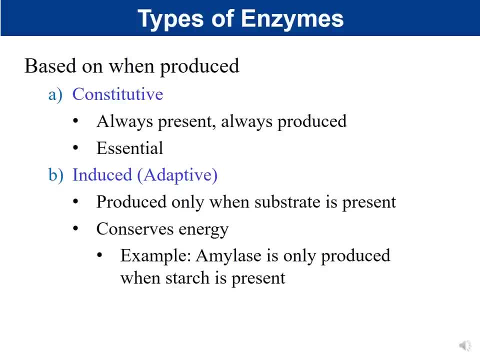 Other enzymes are what we call induced or adaptive enzymes, and those enzymes are only produced when the substrate is present. They're used to conserve energy. Amylase is only produced when starch is present For beta galactosidase, which is the enzyme used to break down lactose- beta galactosidase. 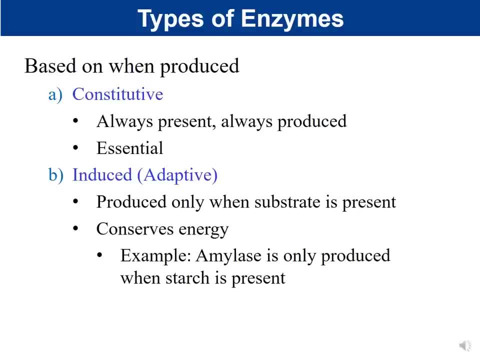 is an adaptive enzyme because it's only produced when lactose is present, So the substrate is present and glucose is not. Because, if not remember, if bacteria have a choice between a monosaccharide and a disaccharide, preferentially they're going to use the monosaccharide. So if glucose is available, bacteria are not going to produce beta galactosidase. So if glycoside is present, then it's not going to be produced. So if you have any bacteria in your cell, you can use a monosaccharide. 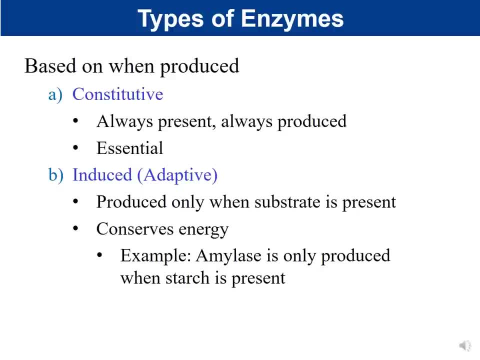 If you have bacteria in your cell, you can use a disaccharide, You can use a monosaccharide. There's no need. They already have their preferred food source. But if glucose is not available and lactose is now, the cell is going to invest energy to make the beta-galactosidase. 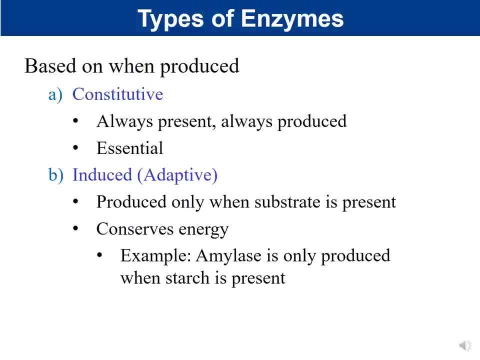 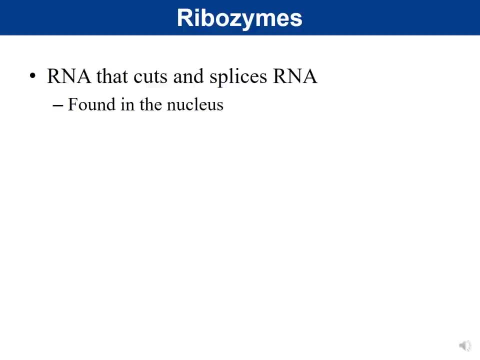 to be able to metabolize the lactose, And so that would be adaptive enzymes. And then the last type of enzyme that we're going to talk about is going to be our ribozyme, And ribozyme is actually an RNA-based enzyme, So while most enzymes are proteins, 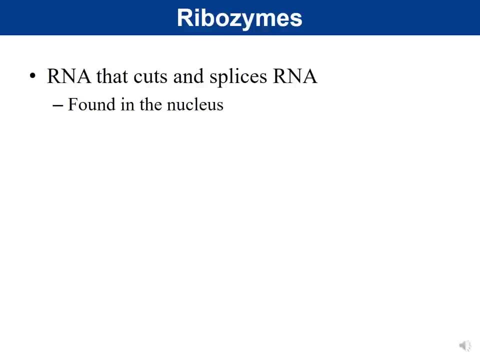 some enzymes are RNA-based, like ribozymes, And these RNA-based enzymes are going to cut and splice RNA. This is a type of enzyme that's found in the nucleus which tells you something about them. Would you guess bacteria have these? Do bacteria have ribozymes? No, 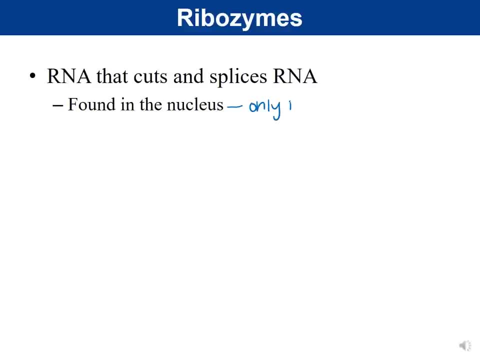 This is a type of enzyme that's found in the nucleus which tells you something about them. This is only in eukaryotic cells. So when we get to our genetics chapter, you will see that prokaryotic cells do not do something. 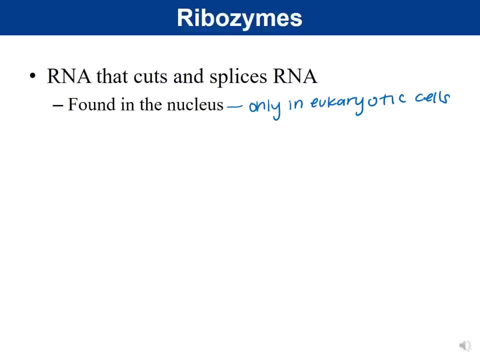 called RNA splicing. They don't cut the mRNA when it's made, because bacteria will translate the RNA as soon as they make it, But because eukaryotic cells have spatial separation of transcription and translation. the cell is going to make the RNA in the nucleus. 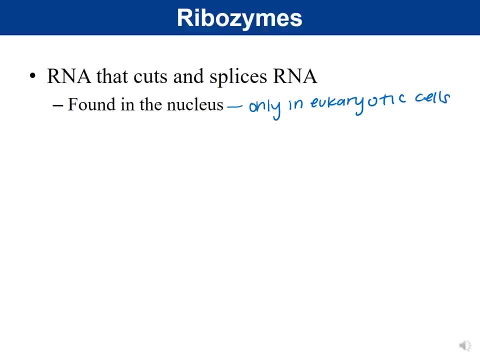 and then the RNA is going to be exported out to the cytoplasm to be translated, And so in eukaryotic cells they're able to do the splicing and to cut the RNA and put them back together, And that is cut by these ribozymes, these RNA-based enzymes, And so, again, we'll talk a lot. more about splicing, But what we're going to do is we're going to cut the RNA and put them back together, And so, again, we'll talk a lot more about splicing, And so, again, we'll talk a lot more about. 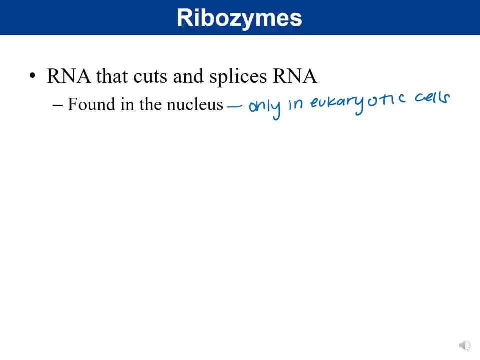 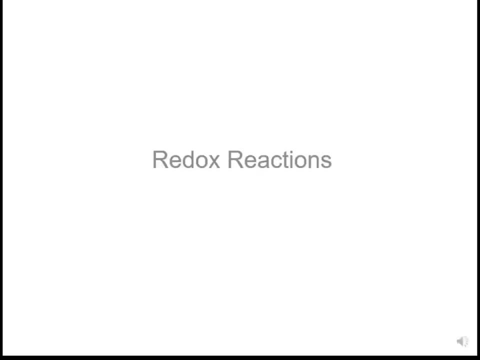 splicing when we get to our topic of genetics. So in order to understand cellular respiration, we have to understand redox reactions, And you guys started to learn about redox reactions in lab because we did a lot of tests that looked at redox reactions We talked about. 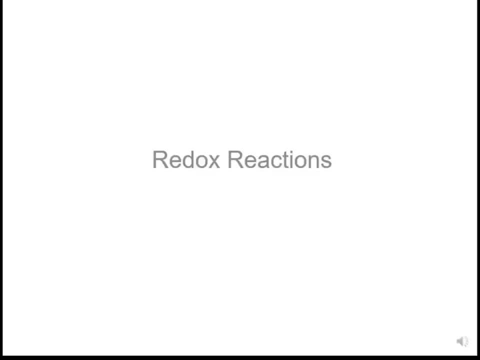 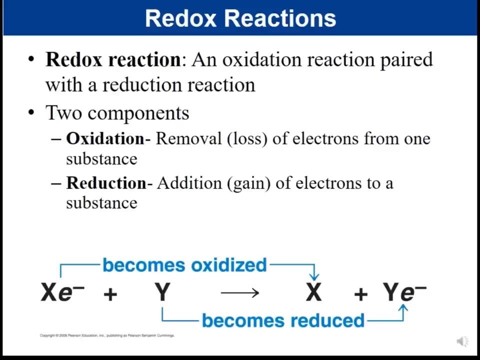 our anaerobic jar right And so we had to reduce O2 to water to make the jar anaerobic. We did nitrate reduction. So we've already talked a little bit about redox reactions, but we're going to review it here. So a redox reaction is an oxidation reaction paired with 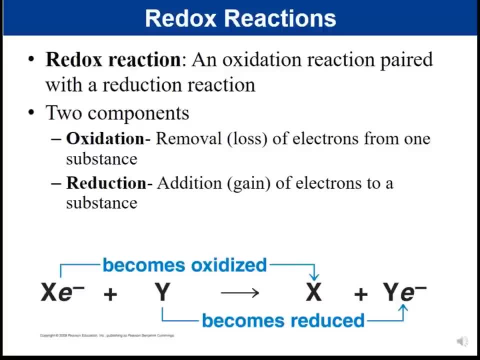 a reduction, And so what that means is that electrons are basically redistributed. One molecule or ion is going to contain the electrons and it's going to pass those electrons to something else, And so what that means is that electrons are basically redistributed. So in lab- you might recall that I taught you guys oil rig, And that is that an oxidation. 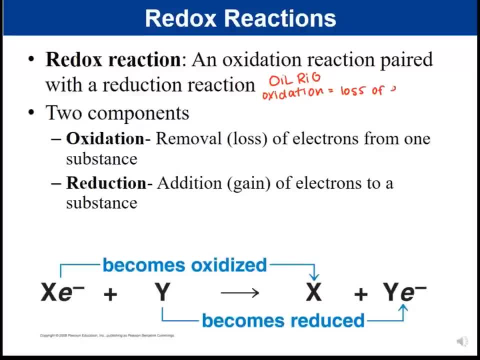 is a loss of electrons and a reduction is a gain of electrons. Reduction is a gain, So oxidation again is going to be the molecular atom that is going to lose the electron. So notice in this bottom diagram we have X. 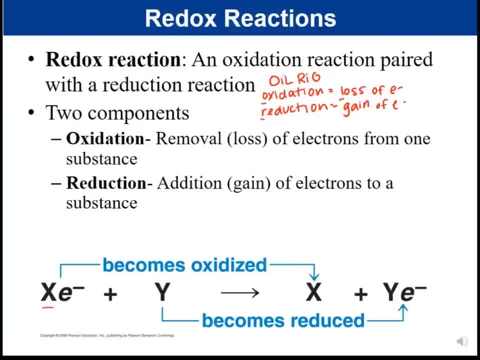 So when it gives its electron to Y, X becomes oxidized and Y becomes reduced, meaning it's going to gain the electron. So all we're simply doing in this case is we're redistributing the electron, We're transferring it from one substance to another, And so that's why you always have 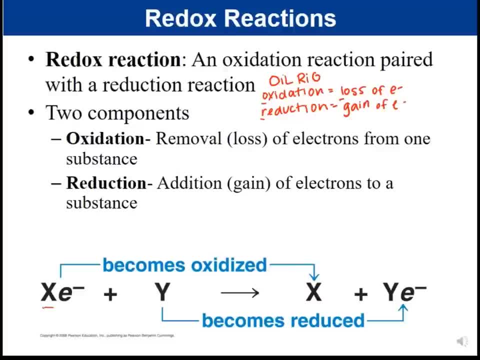 oxidation and reductions being paired, because the electron has to come from somewhere. One atom is going to donate, one is going to receive, And so that's going to be our redox reaction. So question for you to see if you understand your redox reactions. 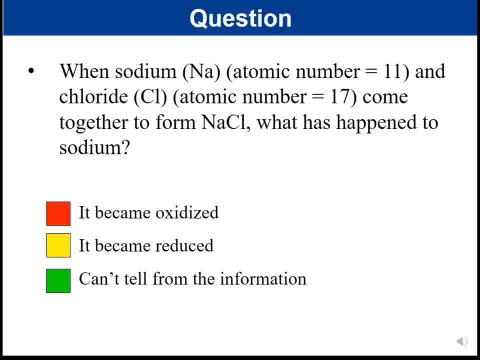 When sodium- atomic number of 11, and chloride atomic number of 17, come together to form sodium chloride, NaCl. what has happened to the sodium? Is it red, It became oxidized, Yellow, It became reduced, Or green? Can't tell from the information. So my hint to you, when trying to solve this: draw out. 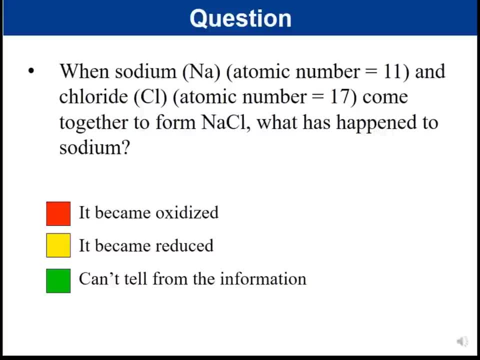 the electron shells, See how the electrons are going to move, and then that's going to help you with whether sodium becomes oxidized or reduced. So when you get a second, pause your video, And when you're ready- once you've tried to work through it yourself- go ahead and restart the video to get the 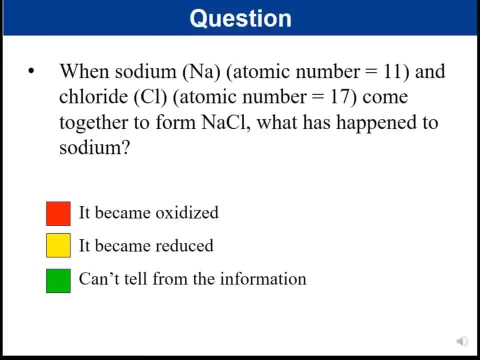 answer. All right, so let's go through this. So we have sodium. Sodium has an atomic number of 11.. Remember, if its atomic number is 11,, how many protons does sodium have? And the answer is 11, because the atomic number is. 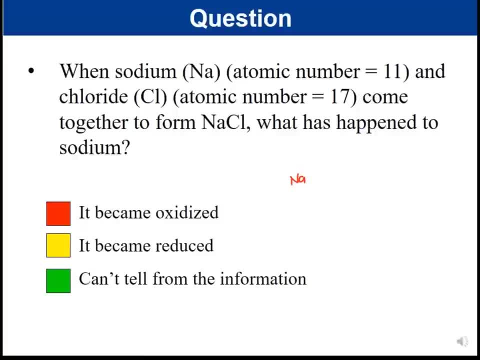 equal to the number of protons. So sodium has 11 protons. Protons carry a positive charge. So if sodium has 11 protons, how many electrons will sodium have total? And the answer is 11, because the positive charges and the negative charges balance each. 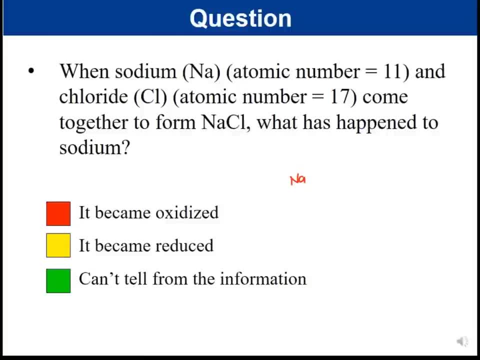 other out. So if we're looking at our electron shells, how many does sodium have in its first shell? Two, right, That's going to fill its first shell. How many in the second shell? Eight, That will bring me to 10 total. And so how many in the third shell? And the answer is one. 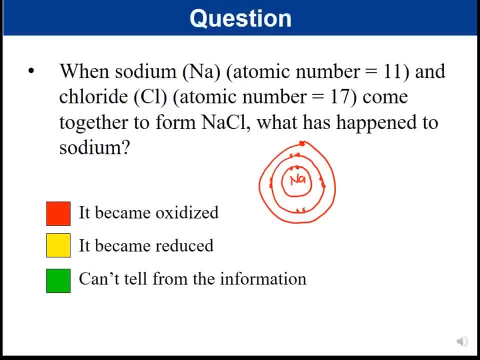 So we have two, eight and then one. That's my 11 electrons. So now let's do the same thing for chlorine. So chlorine has an atomic number of 17.. How many protons 17.. How many electrons, 17.. 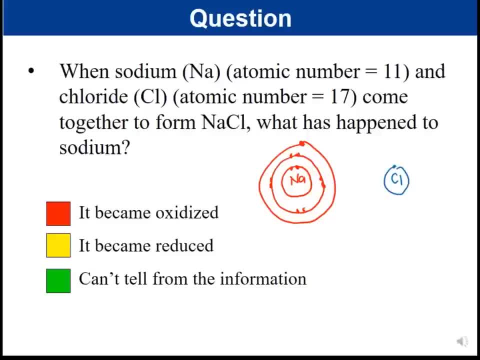 So how many in the first shell? Two? That's going to fill the first shell. How many in the second shell? Eight? That brings me to 10.. So how many in the third shell? So if we're at 10, that means there's. 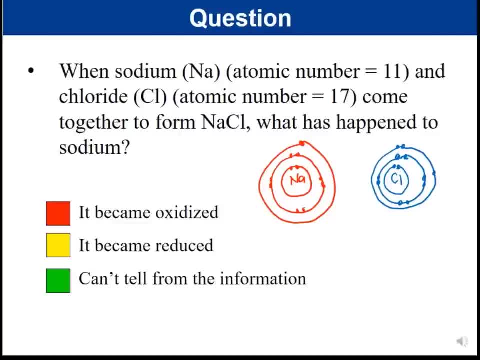 seven in the third shell. So one, two, three, four, five, six and seven. So if you're looking at your electron shells between sodium and chlorine, how many more does chlorine need to fill its outer shell? And the answer is that chlorine needs one more. 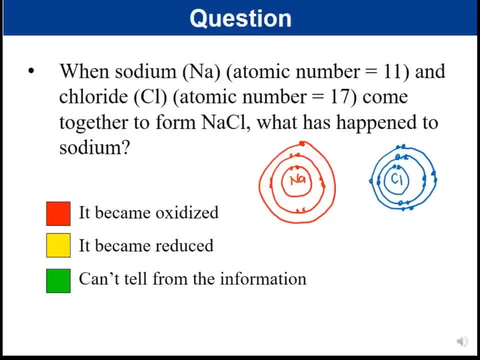 Sodium. on the other hand, right Sodium has one valence: electron. How many more would sodium need to acquire to fill its outer shell? And the answer is seven. That's not very likely. So sodium is not going to try and gain electrons. Instead, sodium is going to donate the electron, And when it. 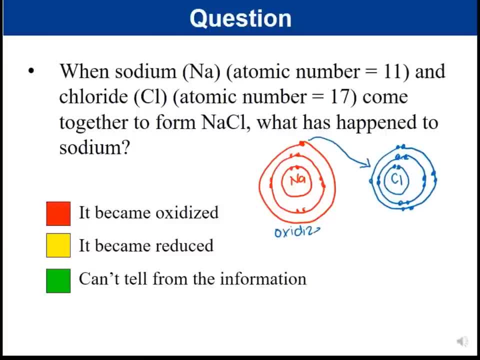 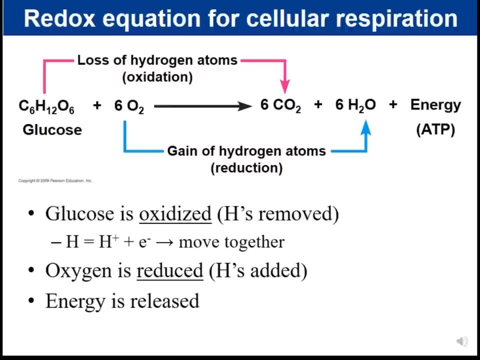 donates. sodium becomes oxidized. It loses the electron And chlorine becomes reduced Because it gains the electron. So the answer is: red Sodium becomes oxidized. So when we look at cellular respiration, cellular respiration is essentially one big redox reaction. 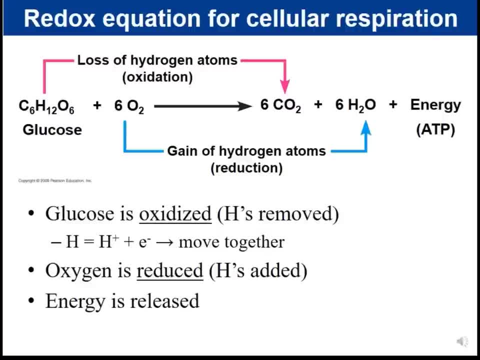 It's simply relocating electrons from one molecule to another, And when we do this, we are going to extract energy And we're going to talk about how. So if we look at our reactants, so what goes in and out of our reactants? So what goes in and out of our reactants? So what goes in? 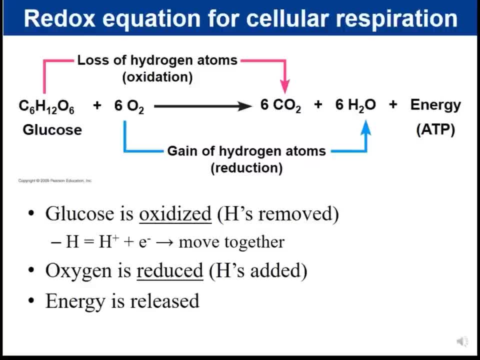 for cellular respiration. We have glucose C6H12O6.. And we have oxygen O2.. And so those are my two reactants. That's what needs to go in for cellular respiration. Now, in cellular respiration, what we are essentially doing is we're taking our glucose and breaking it down. 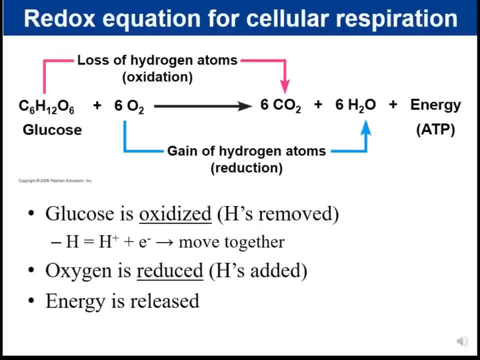 stepwise. So we're going to start by taking that six carbon glucose and chop it into two, three carbon pyruvates And we will just continue to break it down until we're left with a product which is going to be our carbon dioxide. So we're going to break glucose down completely. 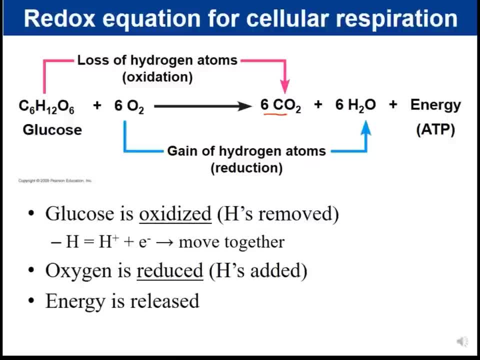 into the inorganic carbon dioxide. So what happens is is when we break those bonds, the electrons are going to be released And you're going to see in a minute that those electrons get put on an electron carrier. So we say that glucose becomes oxidized, It's going to lose electrons. 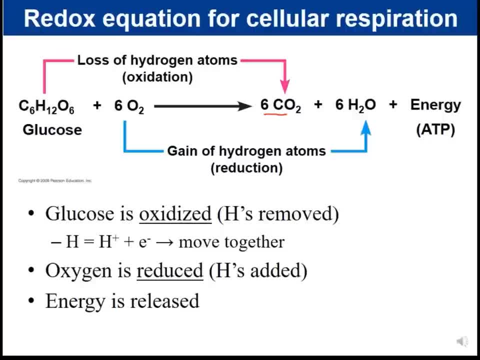 and lose hydrogens. Remember in lab that I told you that one of the things you can do to follow whether it's an oxidation or reduction is to look at hydrogens. So if hydrogens are removed, that means that electrons are removed Because a hydrogen is going to. 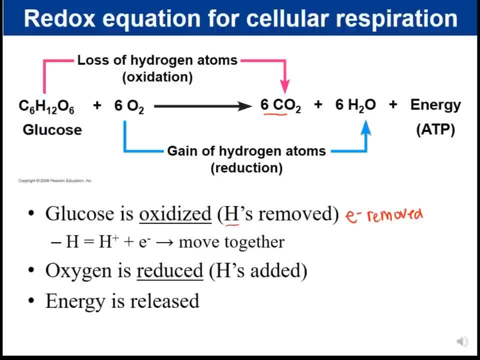 be at H plus at an electron And they're going to move together. So the hydrogens on the glucose are going to be transferred And at the end what's going to take those electrons and take those hydrogens is going to be oxygen, O2.. 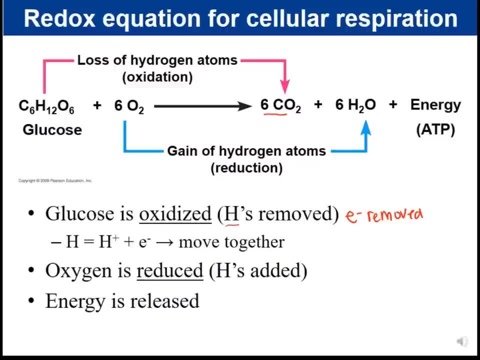 So we say that O2 becomes reduced because it gains hydrogens. it's going to form water. So when oxygen acts as the final electron acceptor, O2 gets reduced. It's going to gain the electrons and it's going to form water. So notice that O2 gained hydrogens, which means that it also 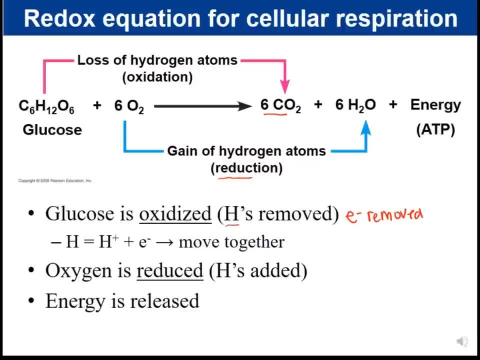 gained electrons And by doing this process, energy is produced Because, remember, we've talked about endergonic and exergonic reactions. Breaking down glucose is going to be an exergonic process. Energy is going to be released because the energy is stored in those bonds Food has. 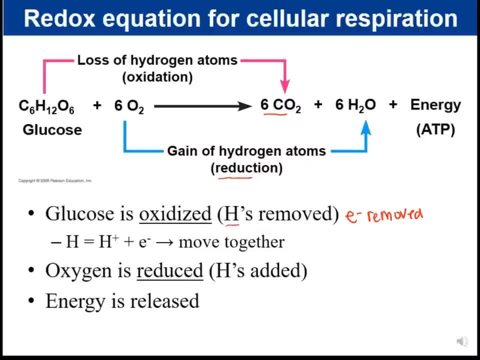 what we call potential energy. It has the potential to do work. So there's energy stored in those bonds and when we break those bonds, the energy gets released, And the energy that gets released is used to produce ATP. So now, thinking along these lines, right Thinking- 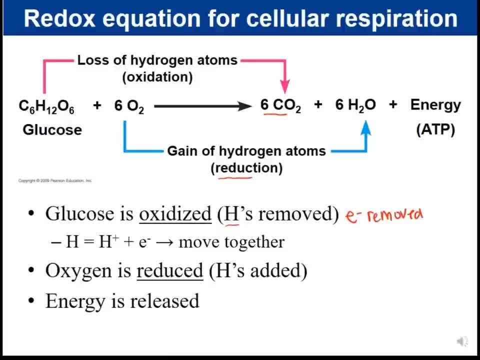 about following hydrogens, If I was to ask you this. and let's say the reaction goes this way, meaning that this time, carbon dioxide and water are the reactants, That's what's going in, And the products are going to be glucose and oxygen. 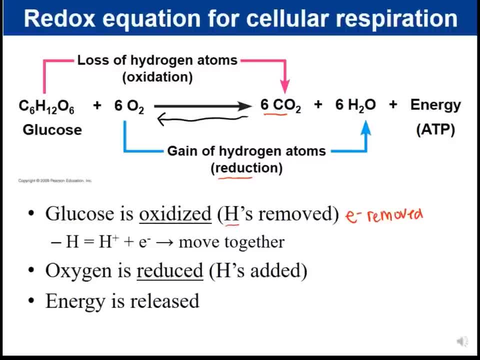 What is the name of that process where we take carbon dioxide and water and we build glucose? And the answer is: the name of that process is photosynthesis. So photosynthesis is the reverse of cellular respiration. So now, if I were to ask this, in terms of photosynthesis, we 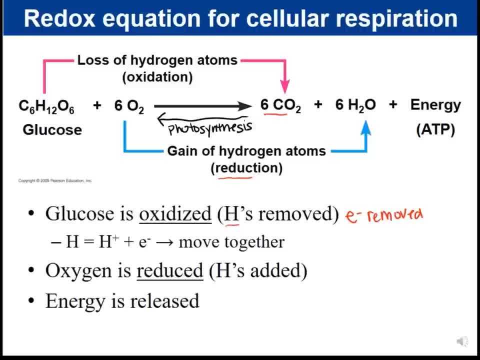 have two reactants- carbon dioxide, and we have water. Which of those two reactants is going to become oxidized And which of those two reactants is going to be reduced? So again, if you need time to think, pause, Think about which one is oxidized and which one is reduced. 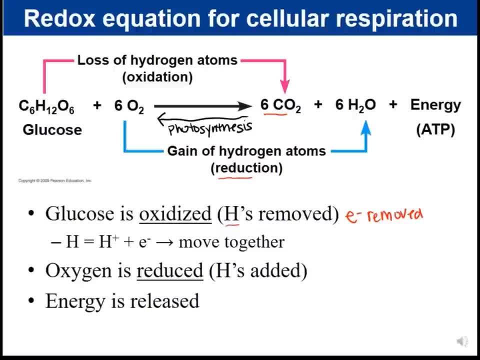 So if we're talking about oxidized, right, that's going to be the one that loses the electrons, which means that it also loses hydrogens. So if you're looking at carbon dioxide and you're looking at water, right, which one has hydrogens? And the answer is the water. So in the reverse, 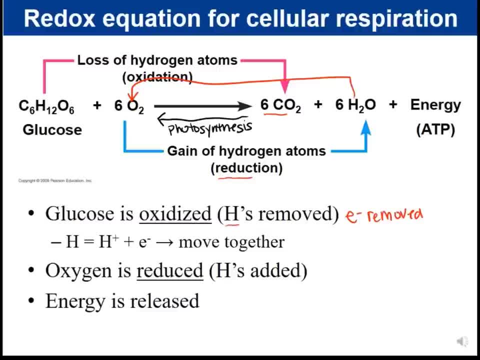 the water right would become oxidized, And that does happen in photosynthesis, because water donates electrons to an electron transport chain. So water becomes oxidized and the CO2, the carbon dioxide, is going to be reduced. It's going to gain hydrogens. 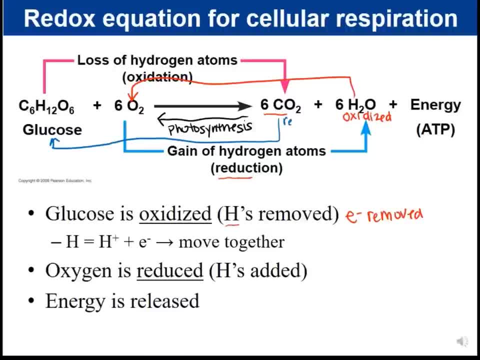 gain electrons, and so CO2 becomes reduced. It's going to be reduced and it's going to build a sugar. Now energy has to be put in for the reverse reaction to happen, right? So again, I'm going to Right. 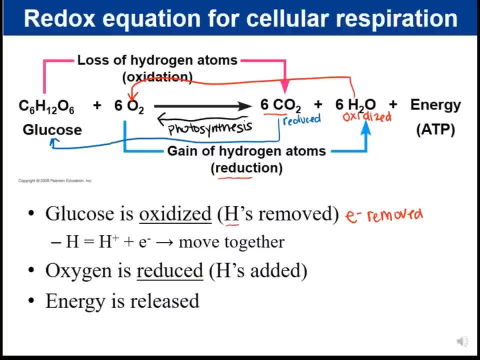 So to build sugar, energy has to be put in. Where does that energy come from? in photosynthesis, The answer: Light, Sunlight. Right Photo refers to light, So light is the energy that's driving that process. But notice that photosynthesis is also a big redox reaction. 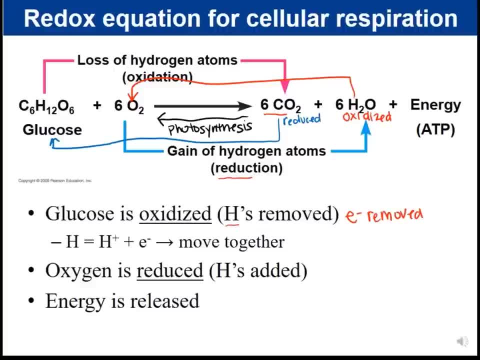 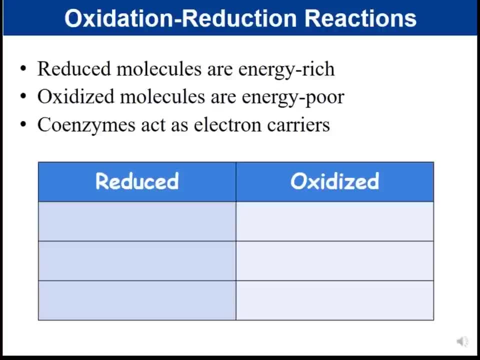 Something is donating electrons, something else is receiving it. So what we need to talk about next is for our redox reactions. In our redox reactions we have coenzymes, and these coenzymes act as electron carriers, And so you might recall that a coenzyme is going to be organic in nature, and they are. 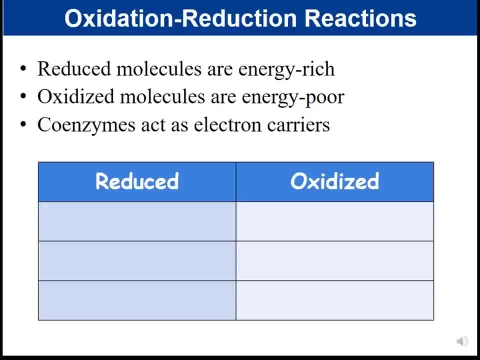 going to carry the electrons. Now, when the molecule, when the electron carrier is reduced, Meaning it has to be organic, If it has the hydrogen, it is energy rich, because those electrons are energy rich. So if it has, if a molecule has its hydrogen, it's energy rich. 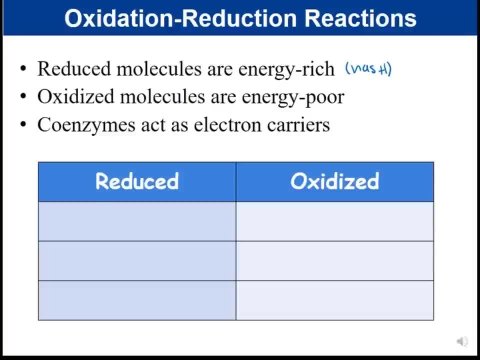 If it is oxidized, right. if it loses hydrogen, it's energy poor, because those electrons have energy, And so if it does not have those electrons, it's energy poor. So there are several electron carriers that we're going to talk about. 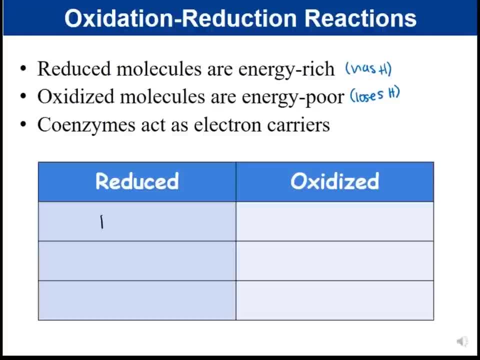 So the first one, in its reduced form, is going to be NADH. Notice, it has its hydrogens. In the oxidized form it's NAD+. So that's when it does not have its hydrogen, it does not have its electron. 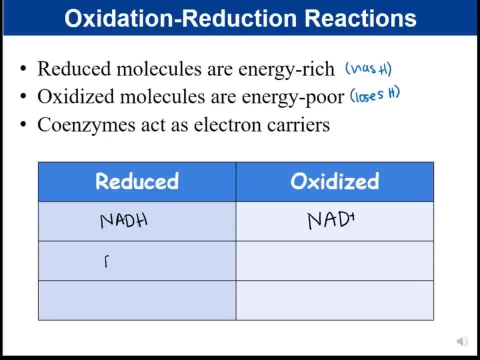 Another one that we're going to talk a lot more about as well is going to be oxygen. So we're going to talk about oxygen. We're going to talk about oxygen. There are FADH2 and the oxidized form is FAD. 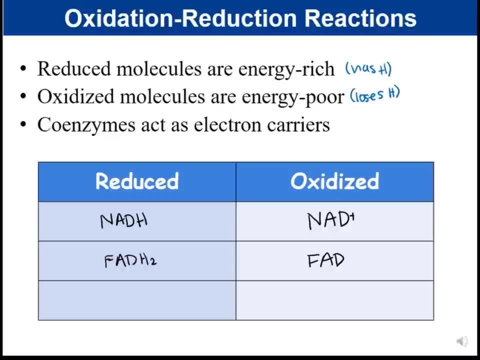 NADH and FADH2 are both used in cellular respiration. And then we have NADPH and the oxidized form is going to be NADP+ when it's oxidized, when it lost its oxygen. So the reduced forms are the ones that are energy rich. 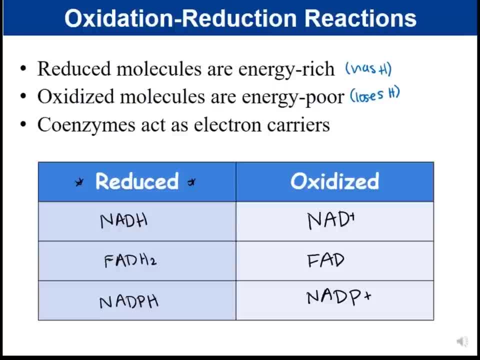 And the reason for that is that you're going to see in a little bit that when those electron carriers take those electrons to the electron transport, they're going to drop off electrons at the electron transport chain. That is where the bulk of the ATP comes from. 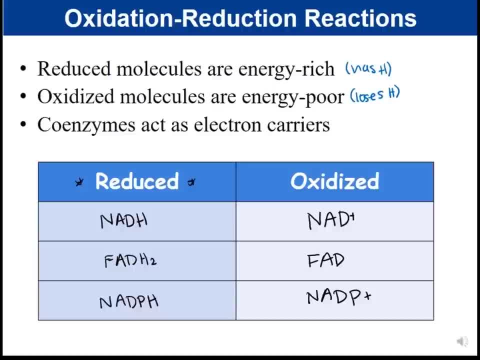 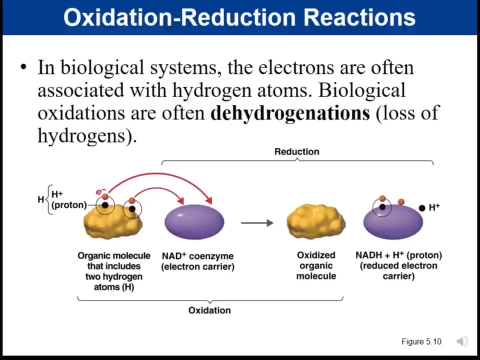 So that's why these reduced carriers, these electron carriers that have their electrons, they're considered energy rich because when they drop off those electrons, those electrons are going to be used to produce ATP. So this is just showing you an example of a redox reaction. 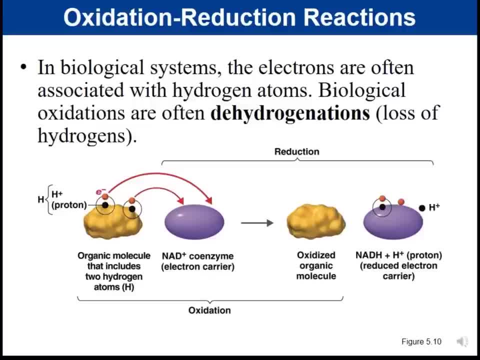 So the yellow blob is an organic molecule. So let's say glucose, for example, right? So glucose, remember, in respiration, is going to be our. the glucose is going to become oxidized, It's going to lose its electrons. 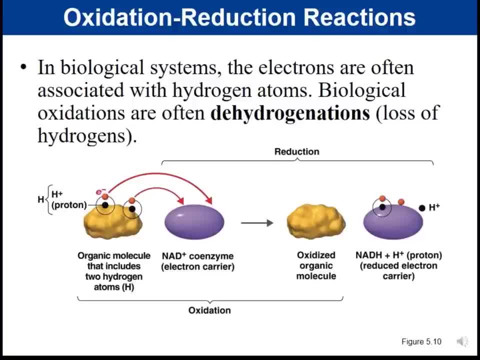 And so the way that that works is: this organic molecule has these hydrogens, So notice that each hydrogen is written as one proton, So that's the black dot and one electron right, And so that's my hydrogen atom, And the electrons are going to be passed from the organic molecule and put onto the empty. 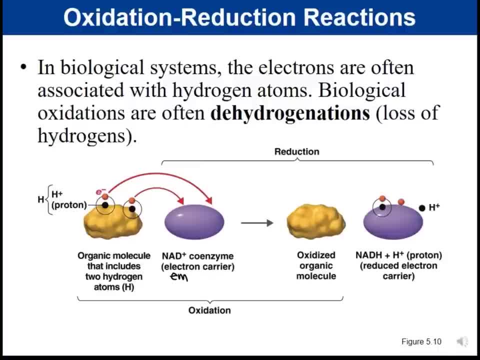 electron carrier. So again I have a diagram in a minute. Empty does not have the electron right. So in this case our empty electron carrier is our NAD+. So our organic molecule is going to donate electrons to NAD+, It's going to transfer its electrons onto NAD+. 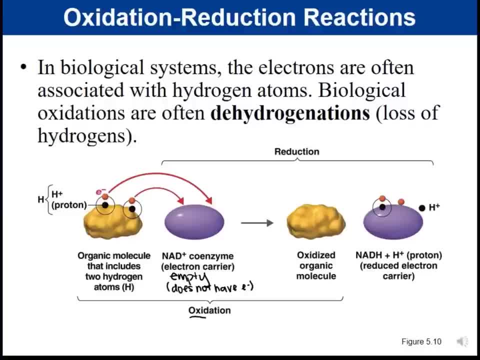 So our organic molecule, then our food becomes oxidized. It loses its electrons. So loss of electrons, The NAD plus, becomes reduced. This is a reduction because we've gained electrons, And so the way that that works is that this whole hydrogen, so one whole hydrogen, gets. 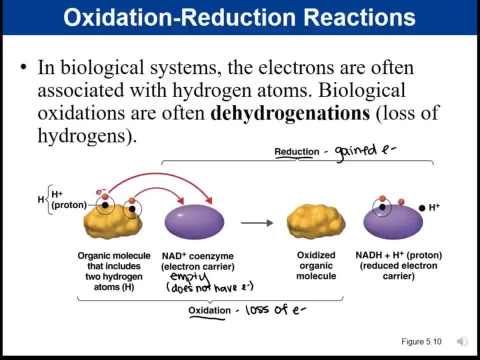 transferred. So that is a proton plus the electron gets transferred, That's the NADH. So one whole hydrogen gets moved And for the other hydrogen only the electron gets transferred on the NAD plus. And when only the electron is transferred, that neutralizes that positive charge. 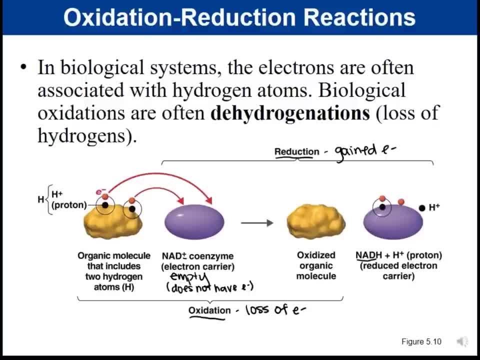 So notice that it's not NADH plus, it's just NADH because that other electron is going to neutralize that charge, And so the electron is going to go onto NADH. So that's the NADH And the hydrogen ion. the proton is going to be released. 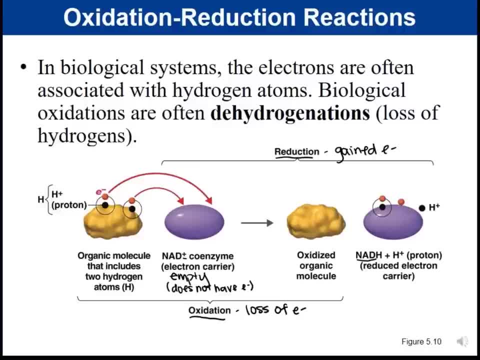 And you're going to see the importance of hydrogen ions later on. So when we talk about biological oxidations, so talking about our redox reactions, where the organic molecule loses electrons, we often call those dehydrogenations. right, They become dehydrogenated. 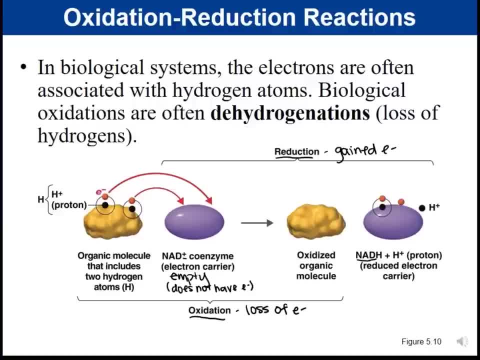 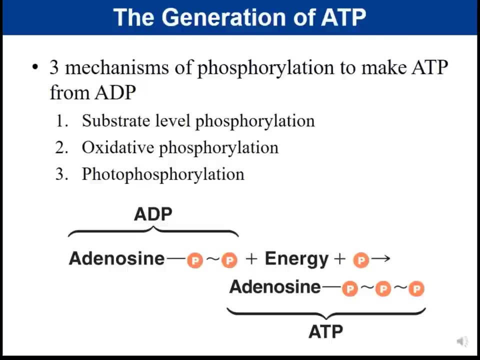 Right, And that's because they are losing their hydrogen, And so the enzymes often that do this are called dehydrogenase. They're responsible for removing electrons from that organic molecule. So now we're going to look at the way that ATP is generated. 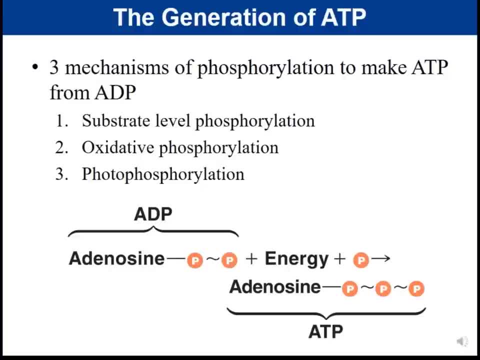 And there are three basic mechanisms of phosphorylation that are used to make ATP from ADP, And so remember that ADP is ATP Right adenosine diphosphate, so notice that it has two phosphate groups and when we go to form ATP, we need to add a phosphate group on to ADP, forming ATP, which is 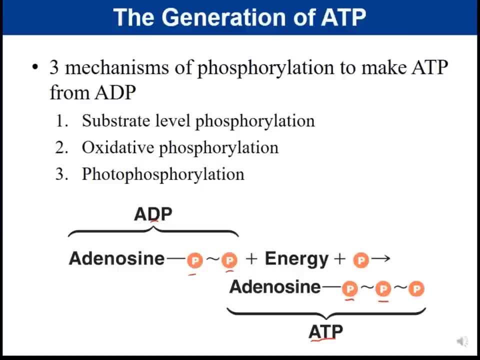 adenosine triphosphate. so notice, we have one, two, three phosphate groups and so we're gonna build ATP. so we call this a phosphorylation because it's the addition of a phosphate group. so we add a phosphate group to ADP, and when we add 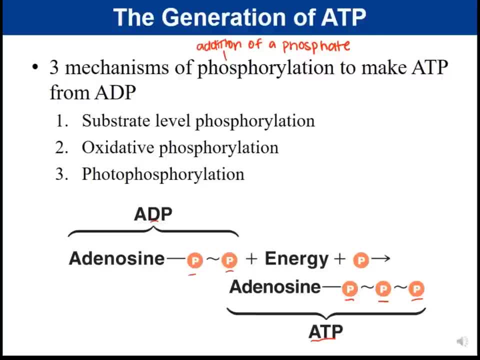 that phosphate group. what we get out is our ATP. now there's three main ways that ATP is produced. the first one is what we call substrate level phosphorylation, and this is simply transferring, so transferring a phosphate from a substrate onto ADP, and that will form our ATP. so it's just like it sounds: substrate level. 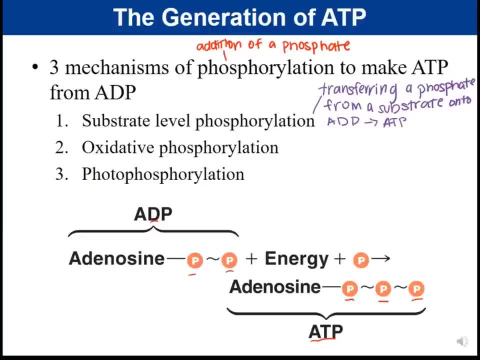 phosphorylation. we're simply just gonna take some substrate that has a phosphate group on it and we're going. an enzyme is going to catalyze the movement of the phosphate from the substrate onto ADP, forming ATP. and that's a P. let me make that a little more clear. the next type of ATP production is what is called 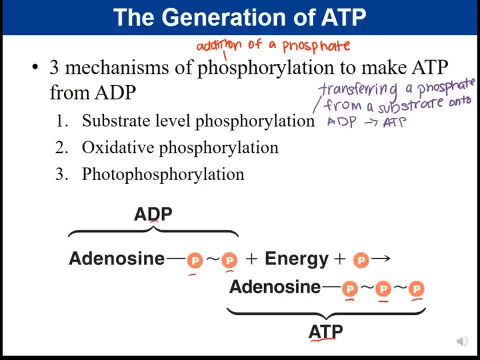 phosphorylation, and oxidative phosphorylation uses redox reactions to form ATP. so an example of this would be the electron transport chain that is going to couple redox reactions to the formation of ATP, and so that's oxydate, a phosphorylation. the last one, photo phosphorylation. phosphorylation is a. 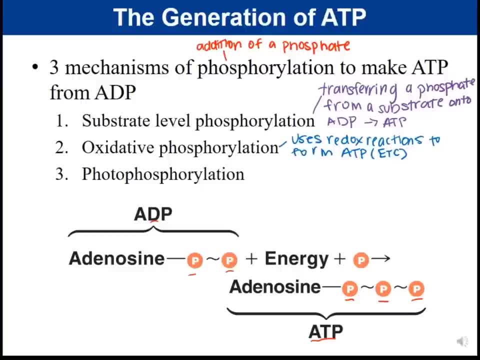 project. it's a photophosphorylation, phosphodyl Photo. What does photo usually refer to? Light? So using light energy to form ATP, And what process, would you guess, uses photophosphorylation? That's going to be photosynthesis, And so we're going to look in a little more detail for each of these three methods. 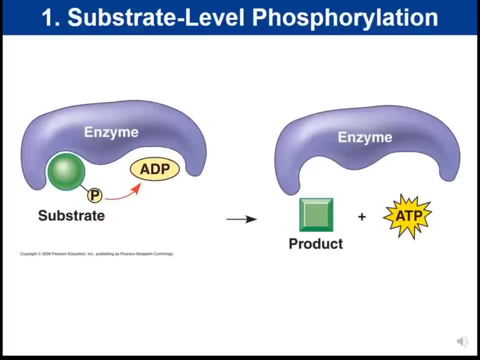 of ATP production. So the first is going to be our substrate level phosphorylation And, just like we used or we wrote on the last slide, all this simply is is the catalyst of moving the phosphate from the substrate. So notice, here's my substrate and it has a phosphate group. 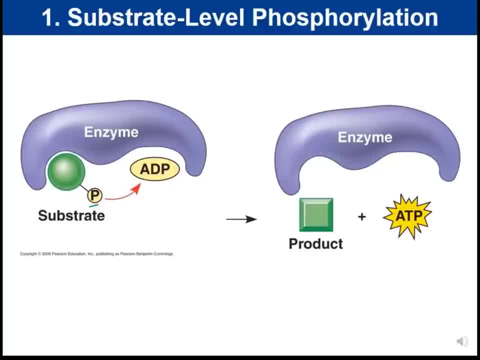 And this specific enzyme is going to bind to the substrate and also bind to ADP, And it's simply going to transfer the phosphate from the substrate onto ADP And what we get out is ATP. This is used, so used in glycolysis and the Krebs cycle. 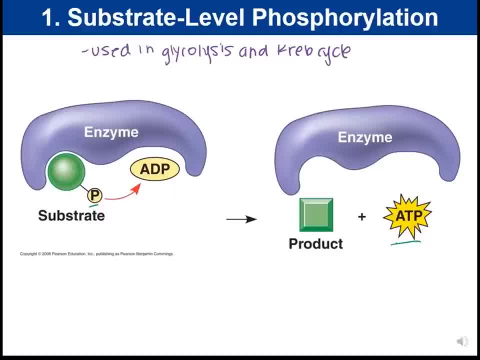 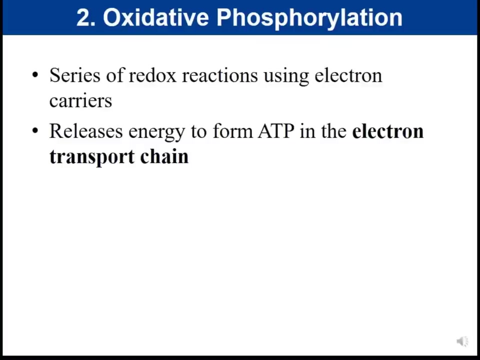 Meaning in those two stages. that is how ATP is produced. It's produced in the substrate level but, as you can all see here, just with phosphorylation, if we were to go into the OH group administration mentioned in omega 1, omega 2.. ADP will take the substrate and that should be the seventh level of XXXEREMA. 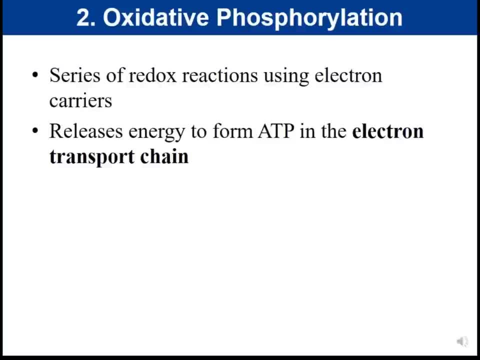 This will oh, the fifth hormone origin, That's diet. So your cholesterol is going to release a lot of ATP in two stages. So that way, AH behaviors outward, Those are essences that are going to further store in your�. Next we have our oxidative phosphorylation And again this is going to be a series of redox reactions. Using electron carriers and it's going to release energy from these redox reactions That is used to form ATP. And if your PA is on ADP, this process of route, time andential engagement stress- is going to cause ATP to Witch and Iron. 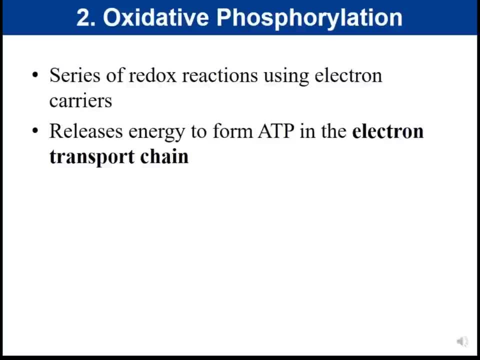 so meaning in that area of glucose derivation is going to allow for overưởngism in the start during the electron transport chain, And so the electron transport chain is where the cell is going to utilize oxidative phosphorylation, And so this is going to actually generate the majority of ATP. 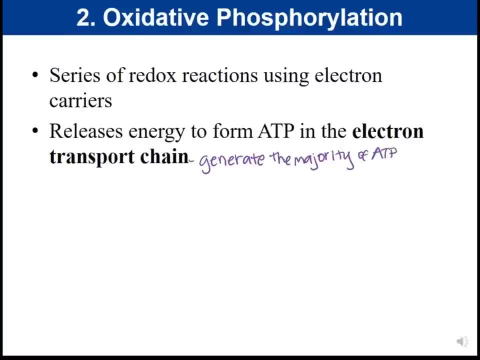 This is going to be the highest yield. So you're going to see in a minute that when the cell does glycolysis, when the cell does the Krebs cycle, in each of those steps we get two ATP per glucose. So the energy yield is not very high. using substrate level phosphorylation: 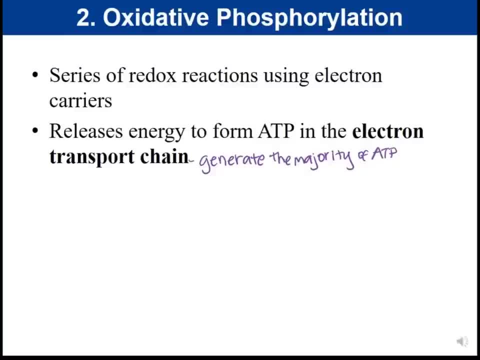 That is in contrast to the electron transport chain. And in the electron transport chain, right in the electron transport chain, we're going to get 26 to 28 ATP per molecule of glucose, So we get the greatest ATP yield in the electron transport chain. 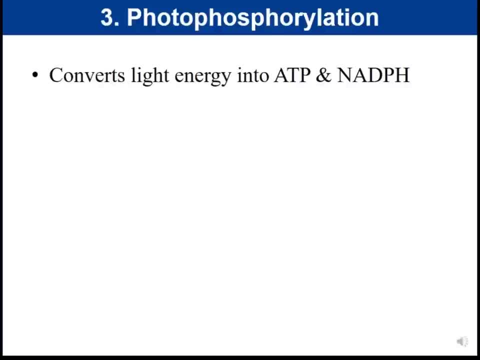 And then, lastly, we have our photophosphorylation, Again, that's going to convert light energy into ATP, and our electron carrier, which is NADPH, And then those two products during what we call the light reaction, those two products. 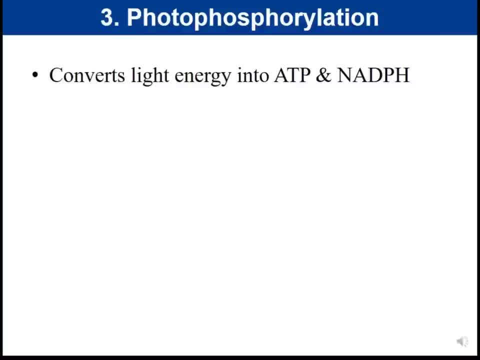 are then going to go on to what's called the Calvin cycle in photosynthesis, and that's where we're going to be able to build, the plant's going to be able to build its sugar, So again used in photosynthesis. Photophosphorylation is used to make ATP in photosynthesis. 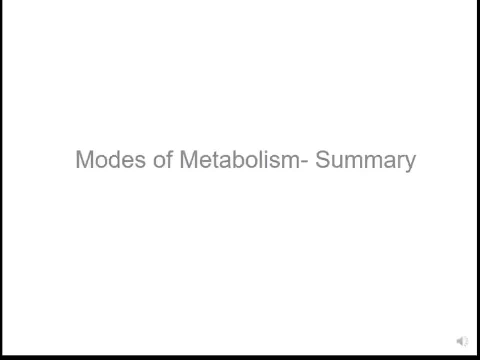 So what we're going to do to start out, is we are going to compare and contrast the different modes of metabolism. So what I'm going to start by focusing on is: what is the difference between aerobic respiration and aerobic respiration and fermentation? What makes these processes different? 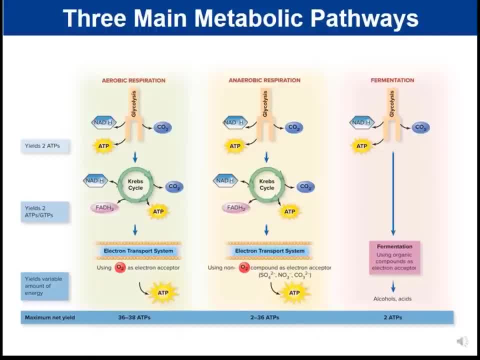 So this slide, This slide is just summarizing and comparing the three different types of metabolism. Now, fermentation is going to give us the lowest ATP yield. It's going to give us three ATPs or, sorry, two ATPs per glucose. This diagram here shows 36 to 38 with aerobic respiration. 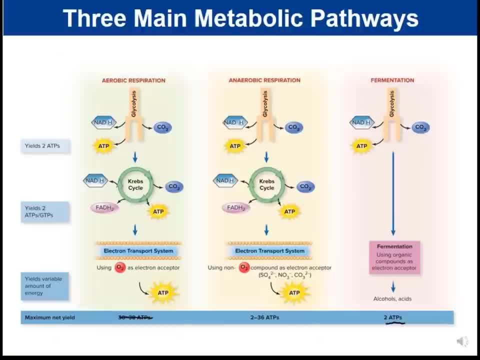 I'm going to cross that out. More recent studies Um, which actually has been done for a while, but um textbooks have not updated this. More recent studies suggest that it's actually 30 to 32 ATP, So not the amount that's written in this diagram, not 36 to 38, it's actually 30 to 32.. 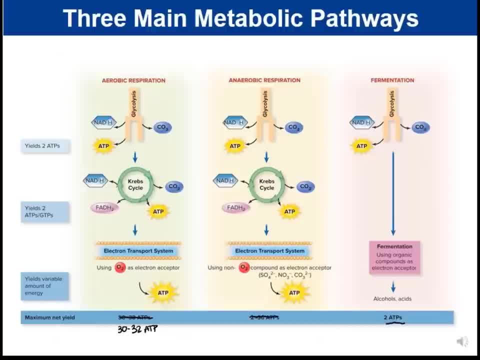 And so, as a result, I'm also going to change the number for the anaerobic. So for anaerobic respiration We get more than fermentation, So I'm going to put the low number being three. So three, but not as much as aerobic respiration. 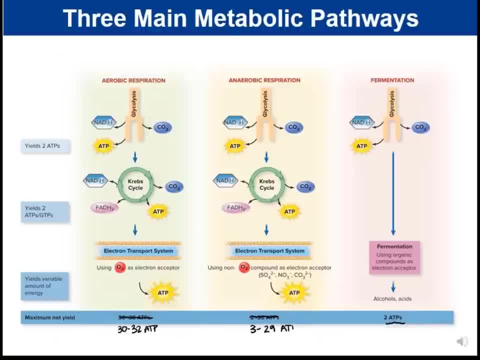 So we're going to put 29.. So we're going to change these numbers a little bit. Now. in anaerobic respiration there's a lot of variability um in terms of ATP yield, Notice three to 29.. That's a pretty big um distinction. 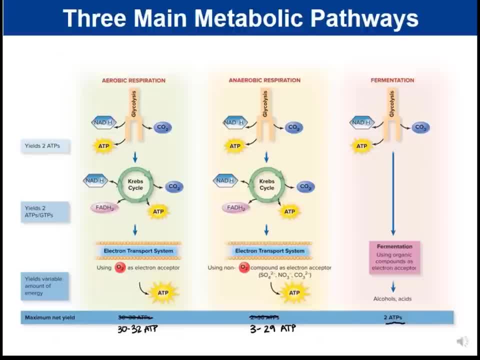 Now, The other thing that I really want to point out is the difference between anaerobic respiration and fermentation, And there is a very key distinction And, in fact, when I looked online, almost probably 90% of the websites that were out. 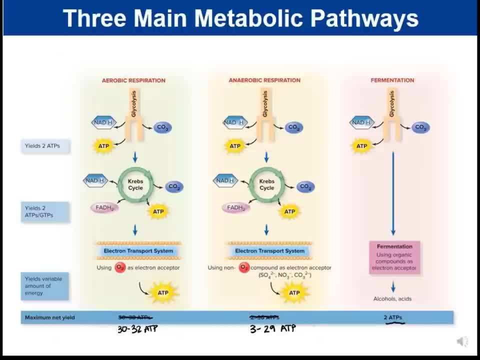 there were using the term anaerobic respiration wrong. They were calling fermentation anaerobic respiration. Yeah, That's absolutely wrong. It's wrong. Bacteria, for example, do true anaerobic respiration. Not many other organisms do. 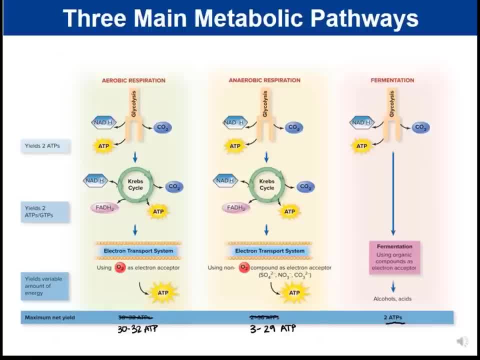 So if you don't study bacteria, a lot of people are using that term incorrectly, So let me compare what is um different and what is the same between these processes. So for aerobic respiration and anaerobic respiration- whenever we call it a respiration- 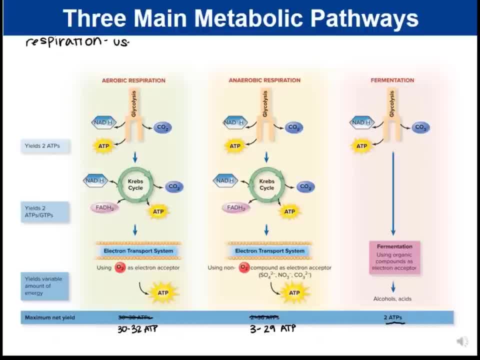 A respiration uses um an electron transport chain, So it uses an electron transport chain. So that's what these two have in common: They both have glycolysis, They both have Krebs cycle and they both use the electron transport chain. 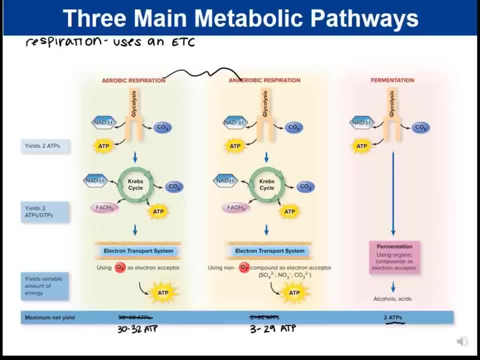 The key distinction between aerobic respiration and anaerobic. Okay, It comes into the final electron acceptor. in aerobic aerobic respiration, O2 is going to be the final electron acceptor. On the flip side, we can use sulfate nitrate carbonate. 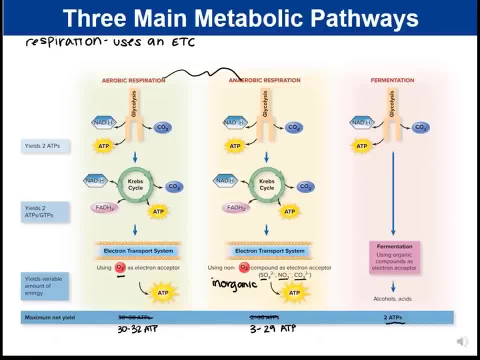 Those are all inorganic final electron acceptors That are not O2.. Okay, Okay, So inorganic final electron acceptor that is not O2.. So notice that none of those molecules has both carbon and hydrogen. In both of the respirations, glucose is broken down completely to form CO2, which is going 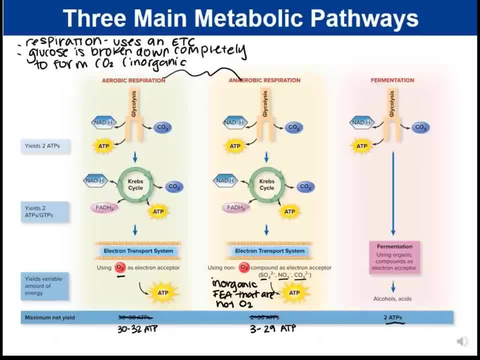 to be inorganic. So inorganic products. We are going to break down glucose completely. So we start with our six carbon sugar. It's broken down into CO2.. Now let's compare anaerobic respiration and fermentation. So key differences between anaerobic respiration and fermentation. 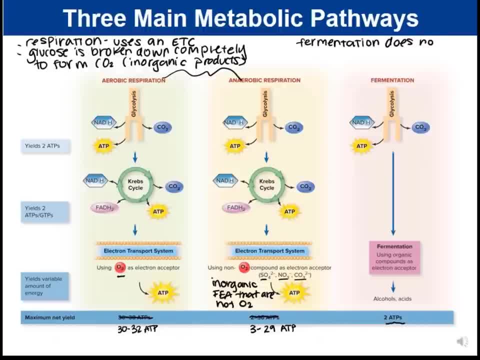 Fermentation does not use an electron transport chain- An electron transport chain, Right. So that's a difference between them. A similarity is both are aerobic or, I'm sorry, both are anaerobic. I said that wrong. Both are anaerobic processes. 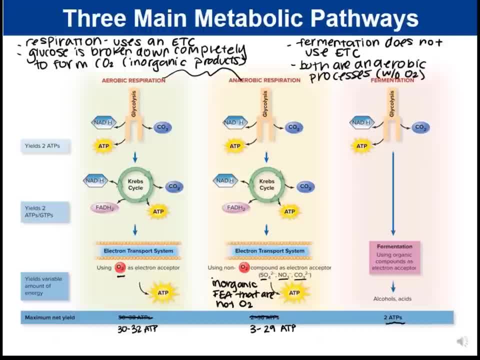 So without O2.. So what they have in common is that they're both anaerobic. Okay, Okay, anaerobic, right? So that's what they have in common: They are both anaerobic processes, but apart from that, they're much more different than they are alike. 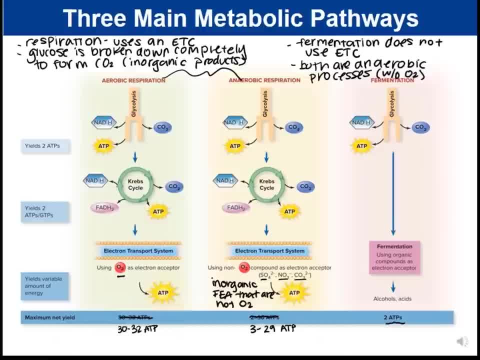 So what I mean by that is that in this case, notice for fermentation uses organic compounds as the electron acceptor. So instead of using an inorganic molecule, we're actually going to use an organic molecule. So our final electron acceptor is either pyruvate- 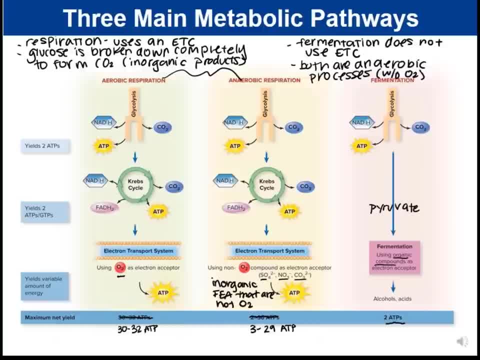 if we're talking about lactic acid fermentation or acetaldehyde, if we're talking about alcoholic fermentation. These, both of these final electron acceptors, are organic And we end up with organic products. So we do not break down glucose all the way. We're not going to end with CO2.. 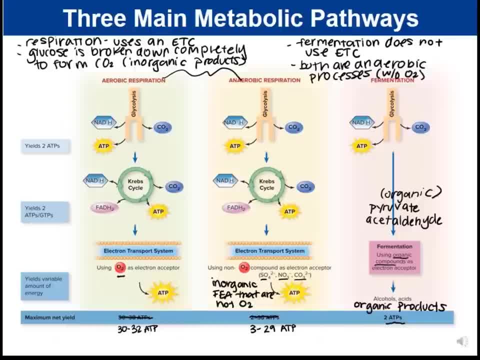 We actually end with organic products that still have a lot of energy left, So alcohol, so ethanol, lactic acid, etc. So notice that anaerobic respiration and fermentation are very, very different processes. They are both anaerobic, meaning they 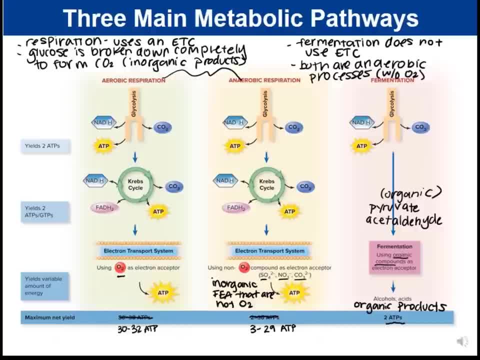 both occur in the absence of oxygen. But anaerobic respiration, remember, when you hear respiration, think electron transport chain. Anaerobic respiration uses an electron transport chain. It uses an inorganic final electron acceptor that is not O2. And anaerobic respiration breaks down. 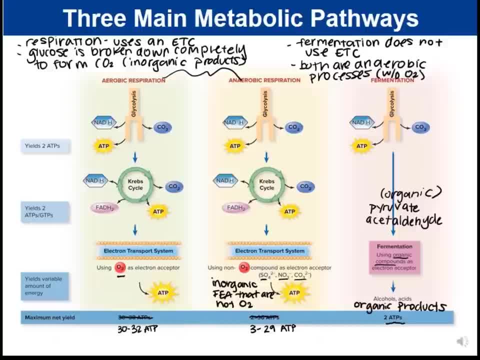 completely to CO2.. Fermentation right. Fermentation does not use an electron transport chain, It only does glycolysis And then goes directly to fermentation. It uses organic final electron acceptors and it produces organic products. So you can clearly see that fermentation and anaerobic respiration are not the same. 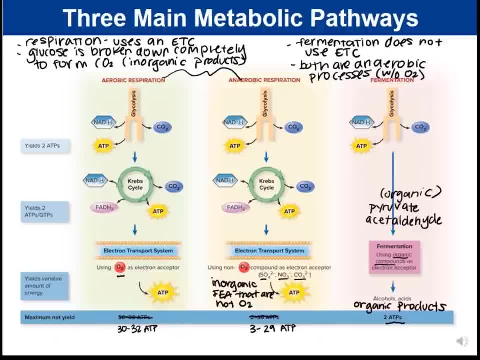 You have to be really careful in how you use this. If you call it respiration again, think electron transport chain, It's going to have an electron transport chain. And so I just wanted to kind of compare and contrast these three different modes of metabolism And we're going to break it down and we're going to go through each one in. 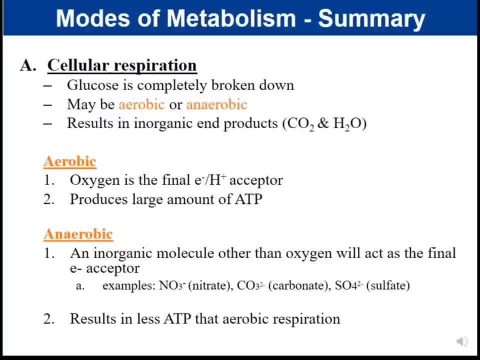 more detail. So, again, this slide is just comparing different types of respiration, And so when we're looking at cellular respiration, again glucose is completely broken down. And when glucose is broken down completely, it results in inorganic end products, meaning we're going to get carbon dioxide and water. 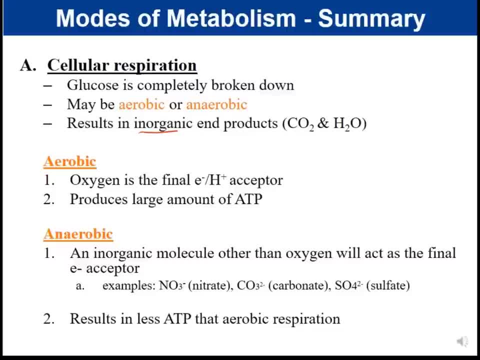 Now, respiration may be aerobic or anaerobic. In both cases, it uses inorganic final electron acceptors. If we call it aerobic respiration, oxygen is the final electron acceptor And this again is going to produce the largest amount of ATP. This is going to give us the highest ATP yield. 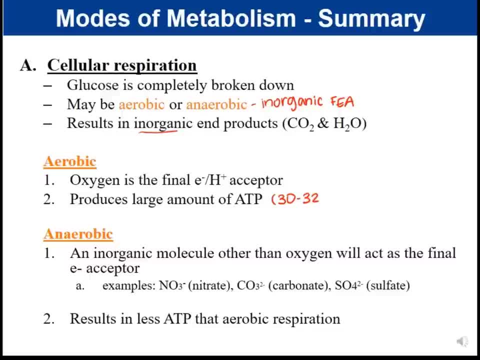 About 30 to 32 ATPs per glucose. In the case of anaerobic respiration, we use an inorganic molecule other than oxygen to serve as our final electron acceptor, And so there are three main types of anaerobic respiration. 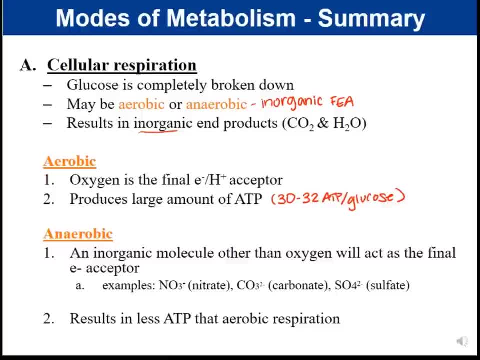 So nitrate: you might recall, when we did our lab and we did our nitrate test, We did our nitrate reduction. What does nitrate get reduced to Remember? if it's reduced, it means that it gains electrons. So what does it get reduced to? 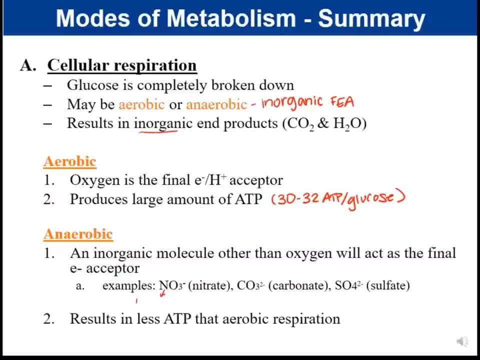 So if nitrate is the final electron acceptor, it's going to produce nitrite, And so our nitrate reduction test was seeing if nitrate could act as the final electron acceptor during anaerobic respiration. So we have: nitrate can be our final electron acceptor. 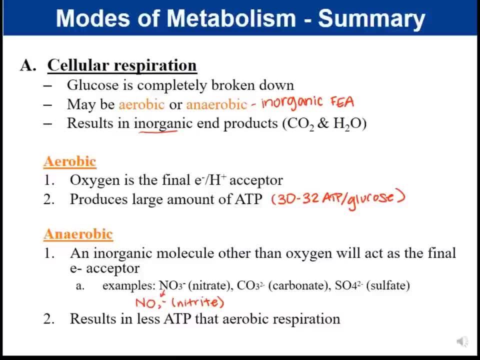 We can have carbonate, and carbonate will be reduced to form methane, CH4.. Sulfate gets reduced to form hydrogen sulfide, H2S. So hydrogen sulfide And for hydrogen sulfide, what test did we do? that was basically looking at this. 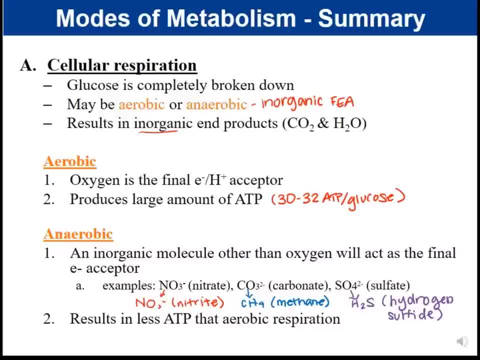 What test did we do that we were seeing if hydrogen sulfide is produced, meaning if sulfur was reduced. So that would be our TSI right? Our TSI was looking at if sulfur can be reduced to form the hydrogen sulfide, And so what we were essentially testing was: can sulfate be the final electron acceptor during anaerobic respiration? 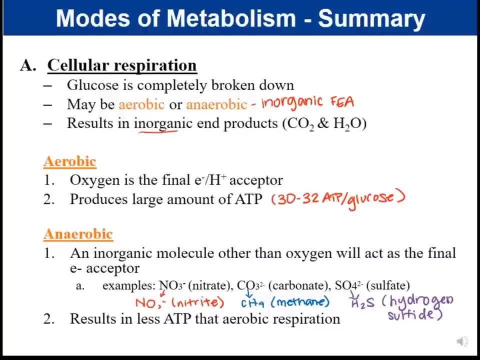 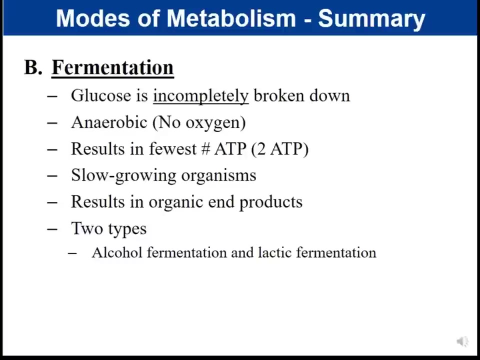 This results in less ATP than aerobic respiration. So again we're going to say between 3 and 29 ATP per glucose, More than fermentation, but less than respiration than aerobic respiration. So next we have fermentation And again in fermentation glucose is incompletely broken down. 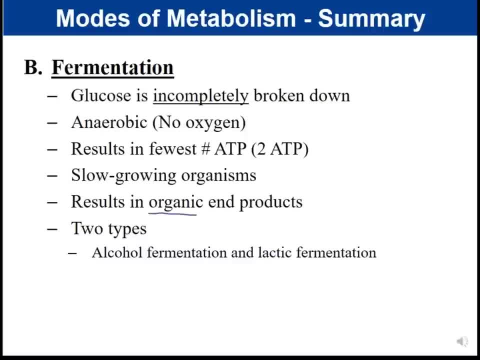 It is not broken down completely. It results in organic end products. We still end up with organic products, And so our organic products can either be alcohol or lactic acid. Now, this is an anaerobic process, meaning it occurs in the absence of oxygen. 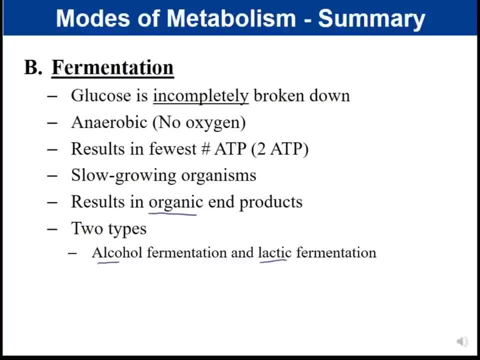 But again, it is not anaerobic respiration. This results in the fewest number of ATP. We only get 2 ATP per glucose, So it is the lowest energy yield And because those products are organic, they still have a lot of energy left. 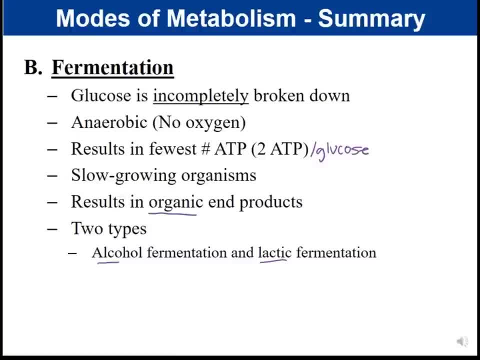 So they're not done Because they get the fewest ATP. these are organisms that are going to be slow growing. Their generation time is a lot longer because they don't get enough ATP to reproduce rapidly. So in this next part we're going to focus on aerobic respiration. 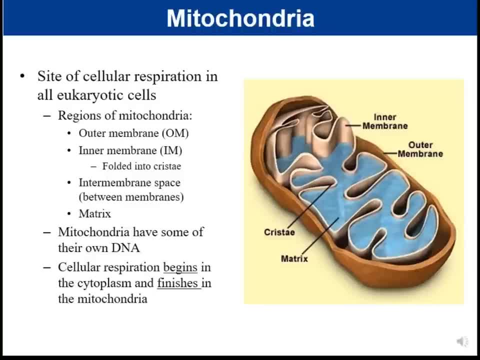 So in eukaryotic cells. eukaryotic cells have cellular respiration take place in the mitochondria. And so, if you recall, when we talked about mitochondria, mitochondria is a double membrane system. It has this smooth outer membrane. 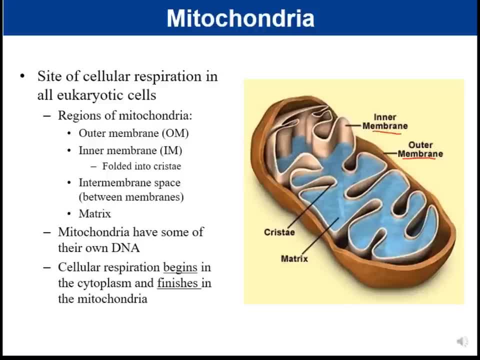 And it has this extensively enfolded inner membrane which is also referred to as the cristae, And so the cristae is just another name for the inner membrane. Now, the reason that the cristae has all of these enfoldings is because structure and function are related. 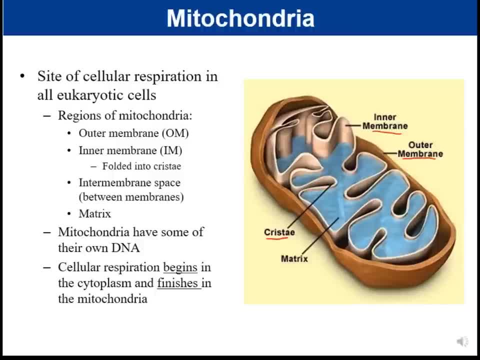 Meaning that there's a reason that that membrane, that inner membrane, is extensively enfolded, And that's because the last step of respiration is the electron transport chain And that happens in the cristae. So there are these proteins embedded in the membrane. 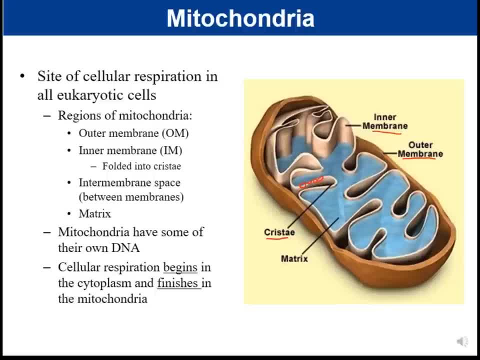 And that's where the electron transport chain is going to occur. So if we have all these enfoldings, we increase the surface area of that membrane, which means we get a higher ATP yield. So there is a reason that the inner membrane has these inner foldings. 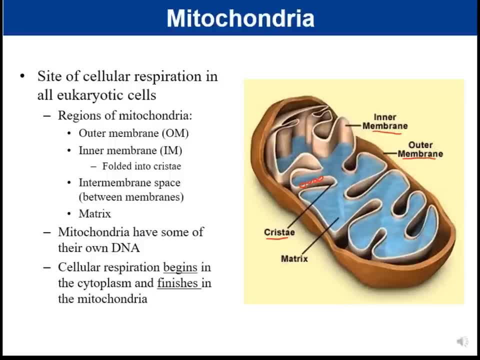 Now, in terms of compartments, because we have this two membrane system. the matrix is the space inside the inner membrane And we have the space between the two membranes, which is called the intermembrane space. So we have two compartments And that's going to come into play when we start to talk about the electron transport chain. 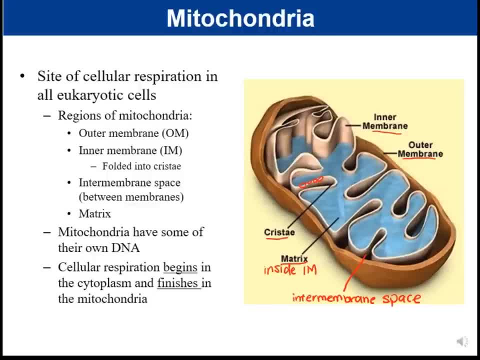 We're going to talk about where each of these steps happens. Now, interestingly, about mitochondria. remember that mitochondria are believed to have once been free-living prokaryotic cells. Right, And we talked about all the reasons why, Right. 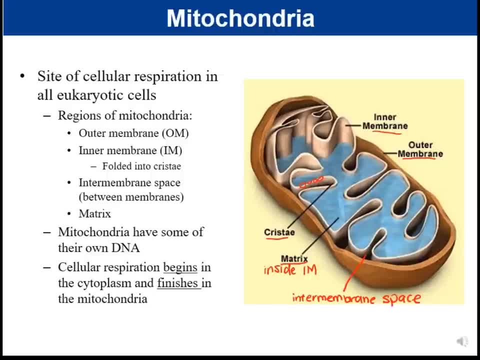 Mitochondria have circular DNA. They have some of their own DNA. It's circular like prokaryotic cells. The sequences are similar to prokaryotic cells. They have their own ribosomes, meaning they can make some of their own proteins. 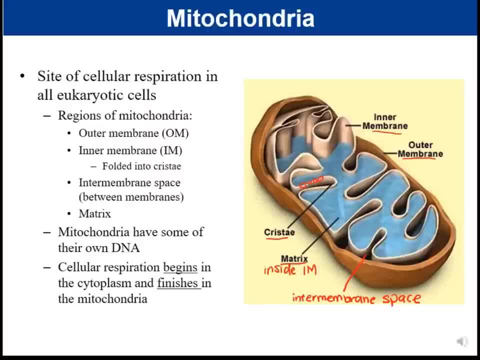 Those ribosomes are 70S ribosomes, just like prokaryotic ribosomes. The ribosomes in your cell are 80S, And the list goes on and on. It's believed that the mitochondria was once a free-living prokaryotic cell. 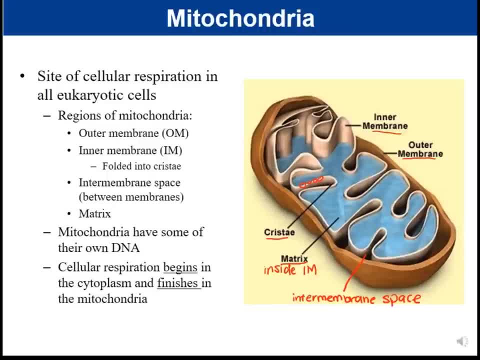 Now in terms of how cellular respiration plays out In eukaryotic cells. cellular respiration begins in the cytoplasm and finishes in the mitochondria. So glycolysis is going to happen in the cytoplasm, The Krebs cycle and the electron transport chain- all are going to take place within the mitochondria. 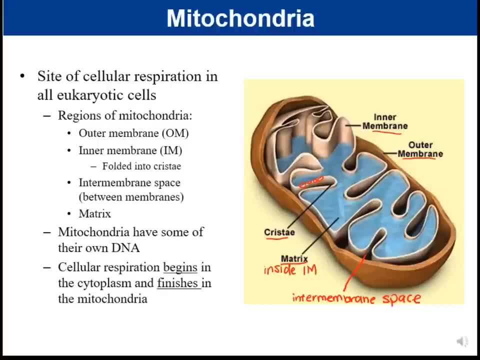 Now, do prokaryotic cells, like bacteria, have mitochondria? And the answer is no. They don't have membrane-bound organelles. So in prokaryotic cells all of the early steps- so glycolysis, the Krebs cycle- are going to happen in the cytoplasm. 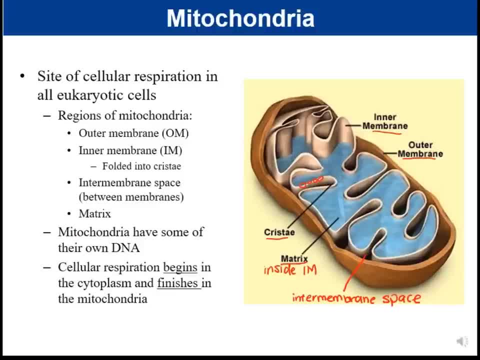 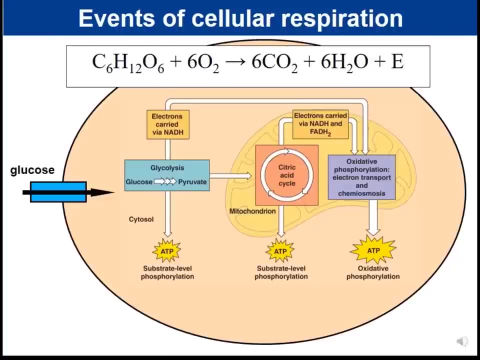 And then the electron transport chain needs to happen across a membrane In prokaryotic cells. what membrane will they use? And again we talked about this, They will use their cell membrane, because that is their membrane that they can use. This slide is just summarizing cellular respiration. 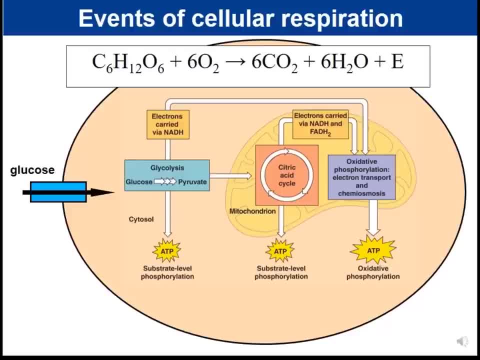 And so glucose. C6H12O6,. glucose is a six-carbon sugar. It is polar right. Think of table sugar, which is sucrose. If I put sugar into coffee, will it dissolve? The answer is yes. 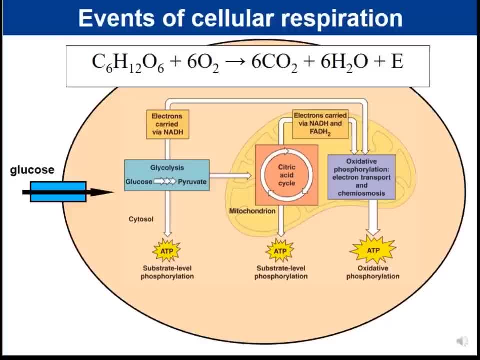 Because sugar is polar, right, It's able to interact with water, which is why it's able to dissolve. So what that means is that glucose- glucose can't cross the cell membrane on its own. It can't get in on its own because it's polar. 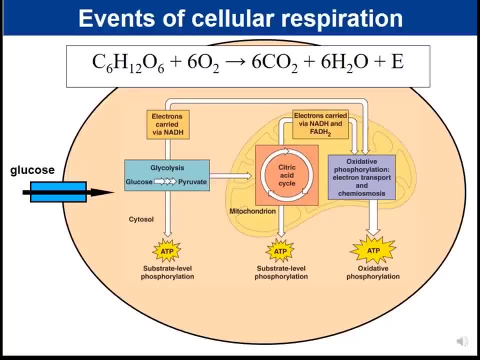 It can't get through the hydrophobic middle of the cell membrane. So in order for glucose to get in, glucose has to be transported using a glucose transporter. So it's going to transport the glucose in. Now again, what happens is is that respiration begins in the cytoplasm. 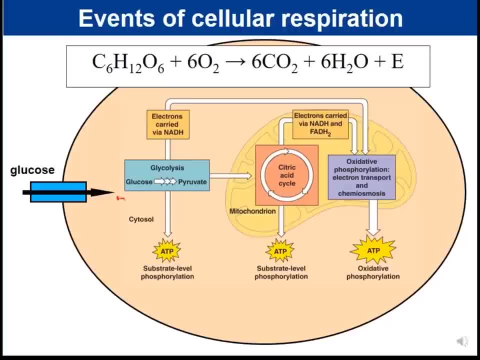 And so what we're going to do is we're going to take the six-carbon sugar- Each of these dots represents a carbon And in glycolysis- glyco sugar lysis breaking. we are going to chop that glucose in half. 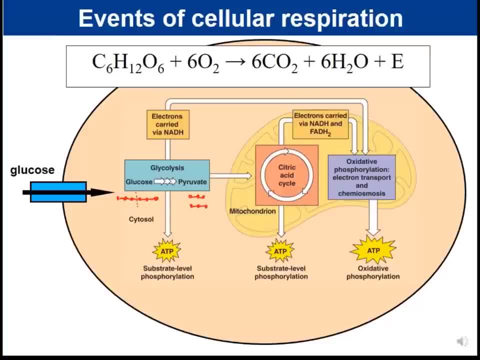 And we get two three-carbon pyruvates. Now, during glycolysis, we do get two ATP And we're going to get that by substrate level phosphorylation, which you'll see in a minute. One of the things you're also going to see is, for each of these steps, when we're breaking bonds. 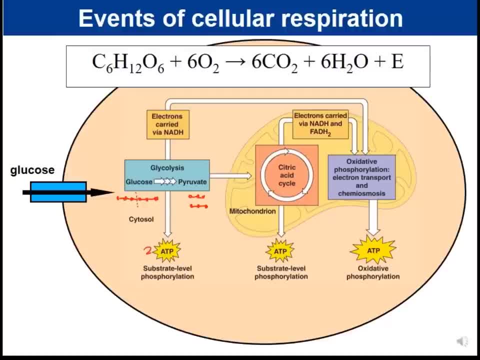 we are going to get electron carriers. So, in addition, one of the other things that is produced during glycolysis is NADH. Remember that that is my reduced electron. It's a reduced electron carrier. It has its hydrogen, It has its electron. 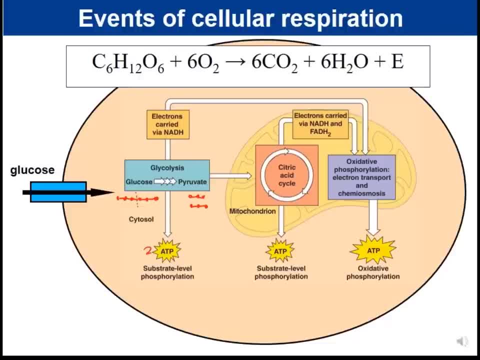 So that is going to be a very important product that's produced during glycolysis. Pyruvate is going to go through a transition step as it's transported into the mitochondria, And when it does this, it's going to break down more. 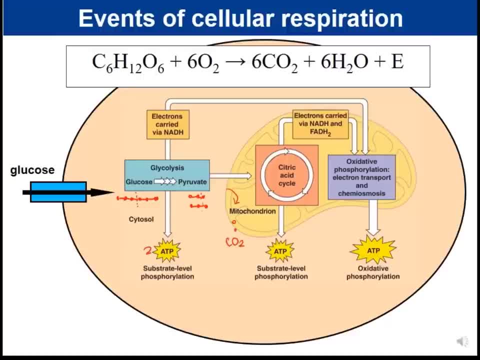 CO2 is released at this point And the remaining two-carbon fragment has a CoA, coenzyme A, added to it, And those will form two acetyl CoAs during this transition. The acetyl CoAs will then go into the citric acid cycle. 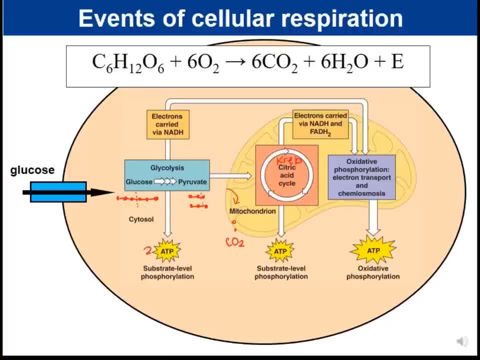 which is also known as the Krebs cycle. Those two names are used interchangeably- And what we're going to do is to the remaining two-carbon fragment. we are going to break it down completely, And so, during this process, we're going to get four CO2s. 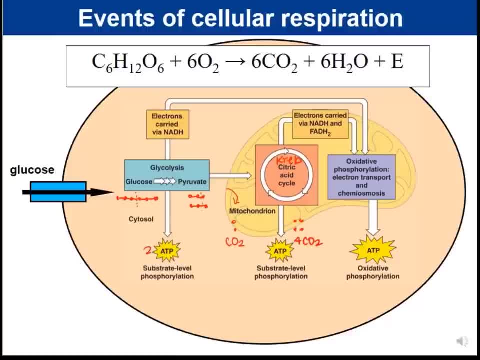 four carbon dioxide, That's the remaining four carbons. We get two ATP by substrate level, phosphorylation, And because we broke down a bunch more bonds, we are also going to get our electron carriers, And in this step we get NADH and we get FADH too. 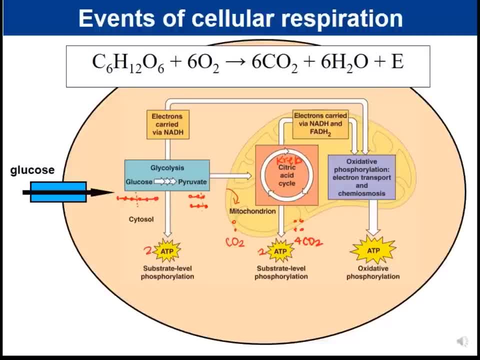 Now the first two steps, the glycolysis and the Krebs cycle- notice- only give two ATP per glucose. The electron transport, so oxidative phosphorylation, is going to give us between 26 to 28 ATP. So the highest yield is going to come from the electron transport chain. 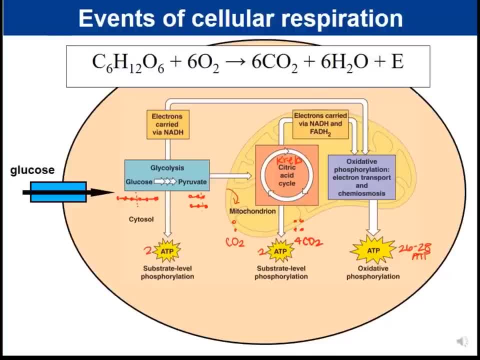 And so what that tells us is that those early steps are not as important for the ATP that's produced, because they produce very little ATP, But actually the important products that get produced during these early steps are going to be those electron carriers, Because those electron carriers 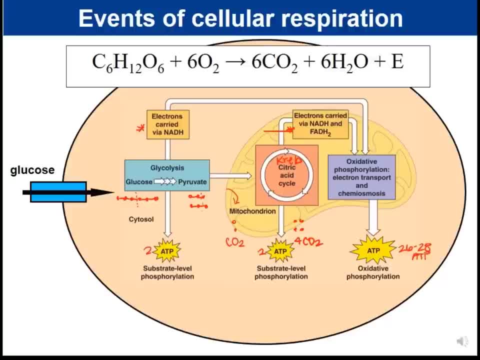 when they go to the electron transport chain and they drop off electrons. those electrons are going to be used to produce the bulk of the ATP, And so what we put in for cellular respiration is going to be our sugar. We also need our O2. 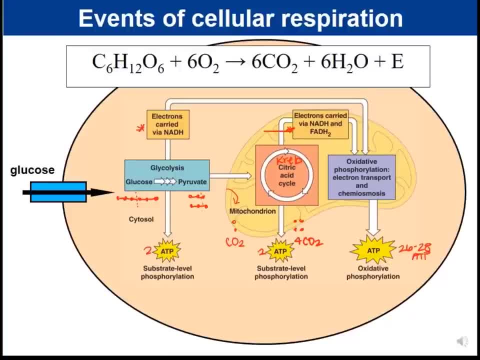 because O2 is going to be our final electron acceptor. What we get out is carbon dioxide. So when we break down the sugar completely, each of those carbons is released as a CO2.. We're going to get water, And the water comes from when oxygen acts. 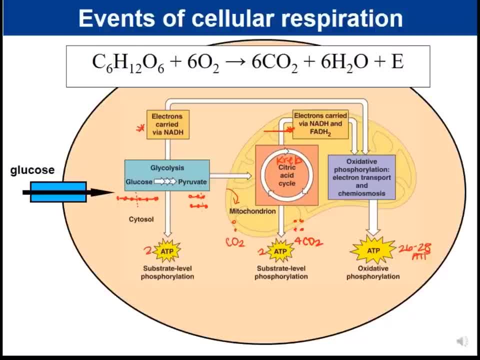 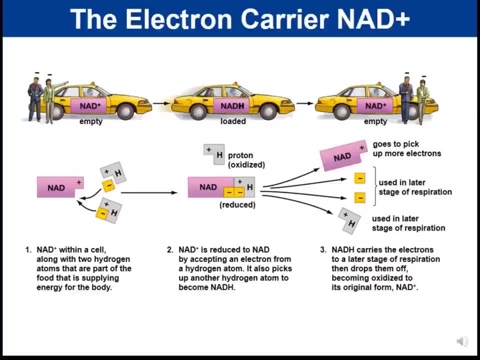 as the final electron acceptor, And also the E is going to be energy because we get ATP. So we need to talk a little more about electron carriers And so, again, you can think of electron carriers as electron taxicabs or electron Ubers in these days. 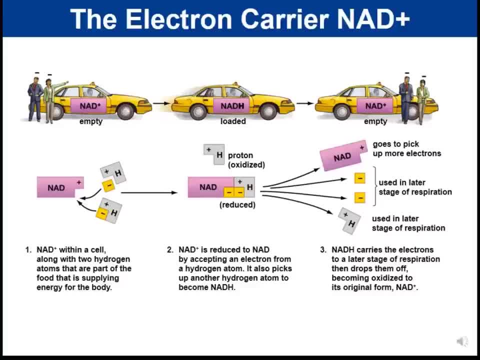 And so when the cab is empty, so the empty state of our electron carriers would be like for the NAD+ right. So NAD plus is empty. It doesn't have its passengers yet and its passengers being the electrons, So NADH, or sorry, NAD plus is empty. 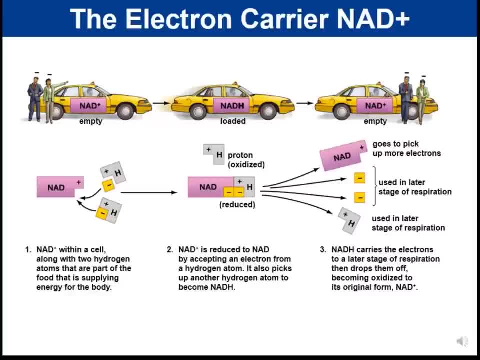 and it needs to pick up its passengers, And so its passengers are going to be electrons. Where do those electrons come from? Well, they come from the food that we eat. So when we break down the glucose, remember that glucose becomes oxidized. 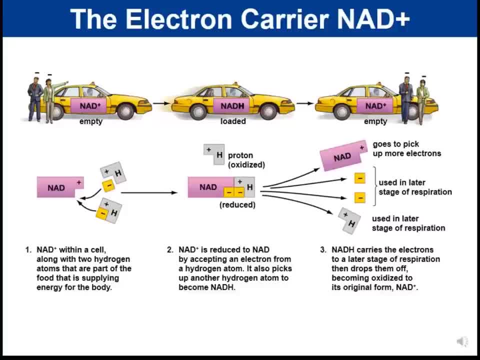 And so glucose and the molecules, the intermediates after glucose, are going to donate hydrogens and electrons and put them on to NAD plus. And so again, like we saw in the dehydrogenation slide, the way that this works is: 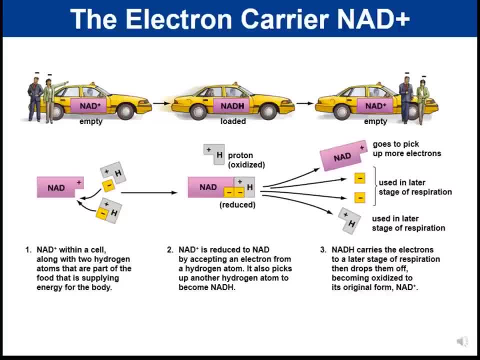 one whole hydrogen is transferred. So that would be- let me put on my laser pointer. So this whole hydrogen gets transferred onto NAD plus, And remember that the second hydrogen, the electron, gets transferred and the proton is going to be released. And so now NAD plus became reduced. 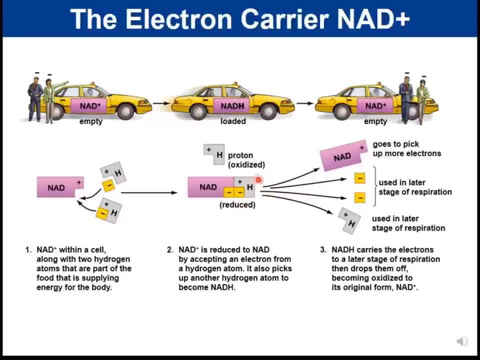 It gained electrons, it gained hydrogens, And again those hydrogens and those electrons came from the food right, And so the food becomes oxidized. So notice that it became oxidized and the NAD plus became reduced. It gained the electrons. 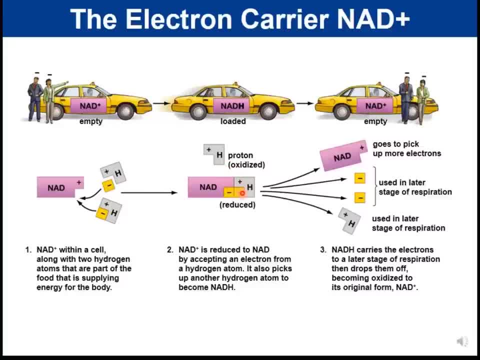 Now, once NAD plus has its passengers- meaning it's loaded- it has its NADH once it has its passengers. now, those passengers, or the electron carriers, rather, the NADH is going to take the electrons and it's going to drop off electrons. 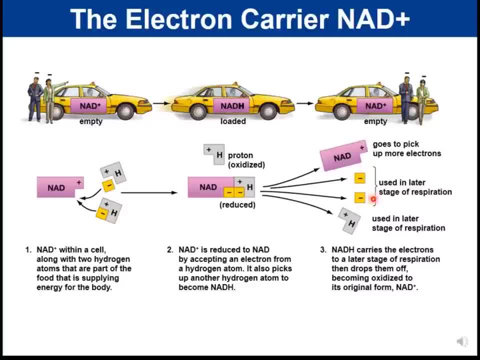 at the electron transport chain, And so you can see here. so these electrons get dropped off, These hydrogen ions get released- You'll see what those do later on- And then we get back to being NAD plus. So now the taxicab is empty. 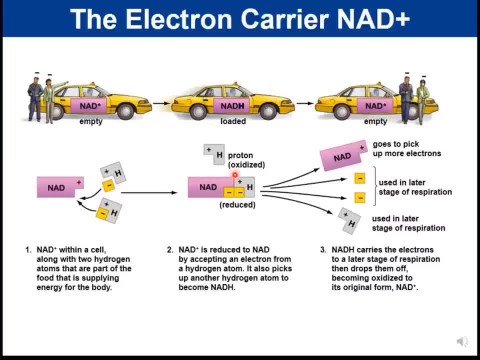 It's ready to go back and pick up a new set of passengers. And so in the cell, the cell is constantly cycling between NAD plus and NADH, And again it's when it has its electrons, when it's in the NADH form. 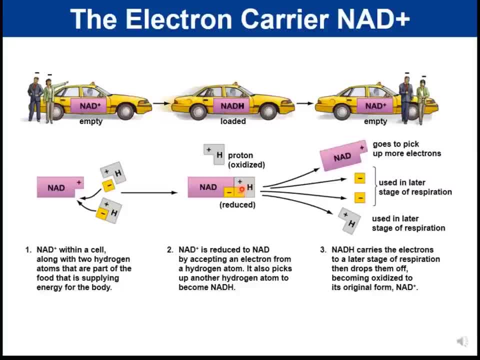 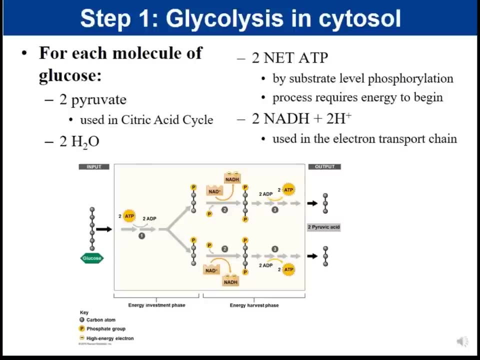 that this molecule is energy rich, Because when they drop off electrons at the electron transport chain, those electrons are used to generate the bulk of the ATP, And so this is kind of an overview of how our electron carriers work. So again, when you are studying cellular respiration, 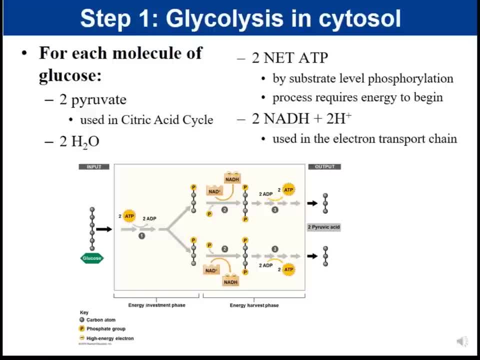 you want to study for each step what goes in, what comes out and where does it take place. You do not need to know all of the intermediates along the pathway. You just need to know what goes in and what goes out. So what goes in. 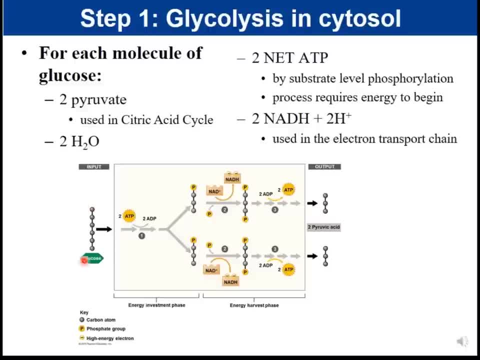 Our input. we need to put in a glucose, And glucose is a six carbon sugar. So we put in our glucose And even though this reaction is exergonic when we break down glucose, we still have to invest a little bit of energy. 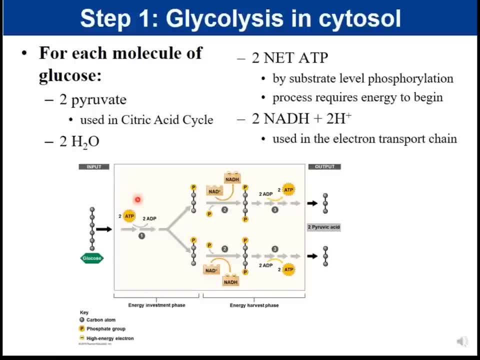 to get the reaction going, And so two ATPs have to be put in and they get hydrolyzed to form ADP, and that will get the reaction started. Now we are going to break the bond in the glucose and we are going to break it into. 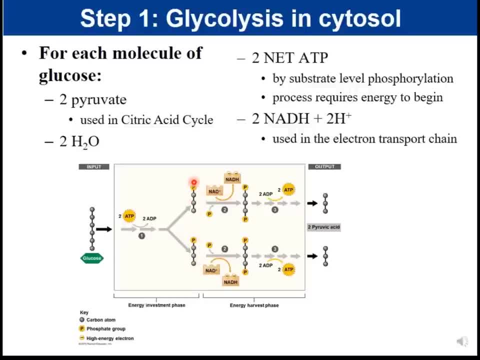 two, three carbon fragments. Now electrons during this process are going to get transferred onto NAD+. So remember I said that the food, so the sugar, is going to become oxidized and it is going to put those electrons onto NAD+ and we get the reduced form, which is the NADH. 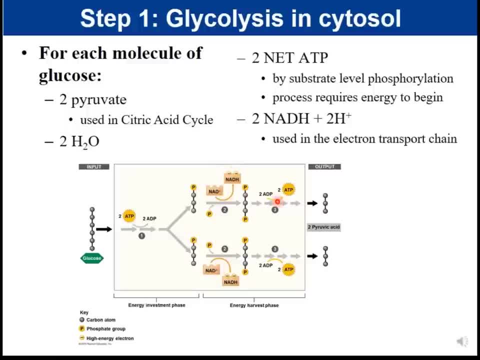 And so that is true for both of these three carbon sugars. Now the other thing that is going to happen is that you are going to get two ATP for each of these three carbon sugars, So notice that your products are going to be four ATP. 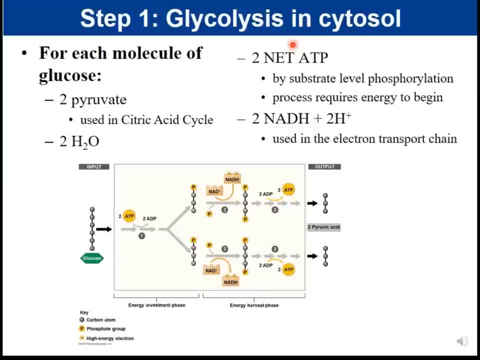 but you had to put in two ATP to get the reaction started. And so we say that you get two net ATP. So you net, you gain two ATP during this process. And again, that is because it requires energy to get the process started. 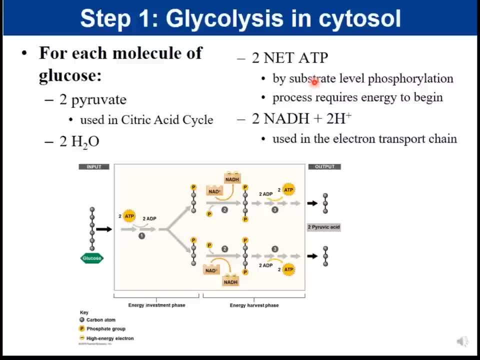 and so the net gain is two ATP. These ATP, remember, are produced by substrate level phosphorylation. So notice that this substrate has these phosphate groups on it, and those phosphate groups are going to be transferred onto ADP and we are going to form ATP. 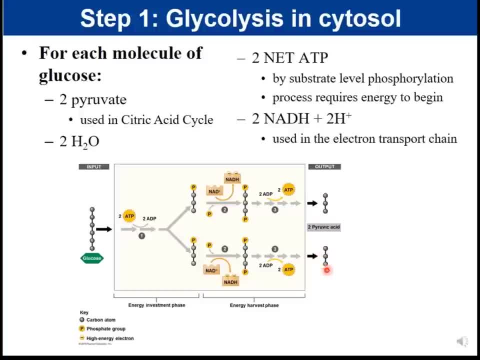 And so our other products that we are going to get that are important are two pyruvic acids or pyruvates. Those names are kind of used interchangeably. So we end up with two, three carbon sugars, and then the pyruvate is going to go into. 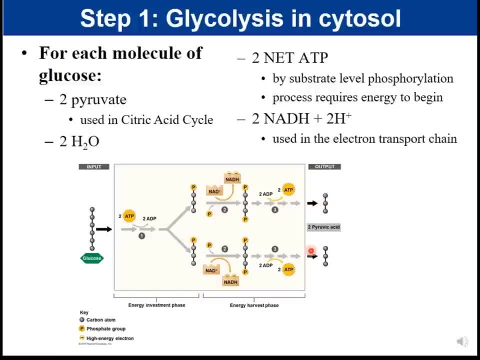 the citric acid cycle, meaning that the sugar is going to continue to be broken down little by little In terms of the water. don't worry about that as much, But the products that I want you to be aware about. so, pyruvate: you get two pyruvates. 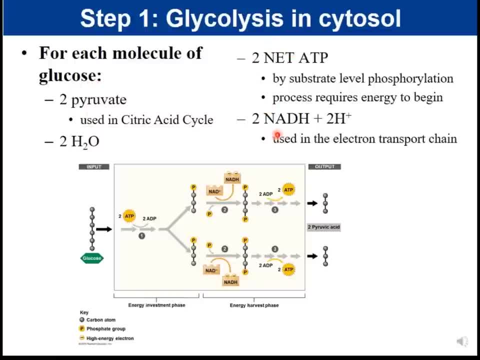 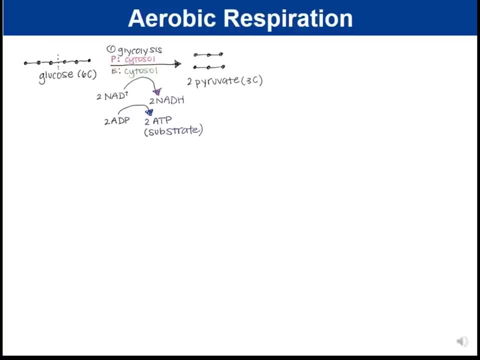 You get two ATP and you get two NADH, And again these NADH are going to be used in the electron transport chain. So what I did is normally in class. I would draw this out, but I've already drawn part of it for you. 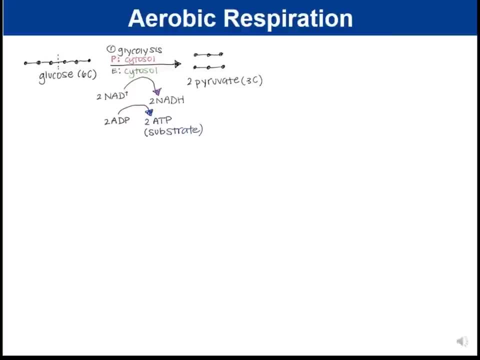 and I'm going to walk you through this, This diagram. as I go through the aerobic respiration talk, I would study this diagram And if it's me and I'm trying to study for the exam, I would try and recreate this diagram from memory. 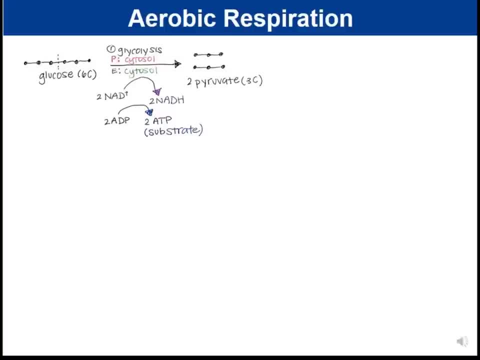 If you can do that, anything I ask you related to this topic is going to be easy. You're going to have no problem whatsoever, So use this as a tool. This is going to be a summary of all the steps of cellular respiration. 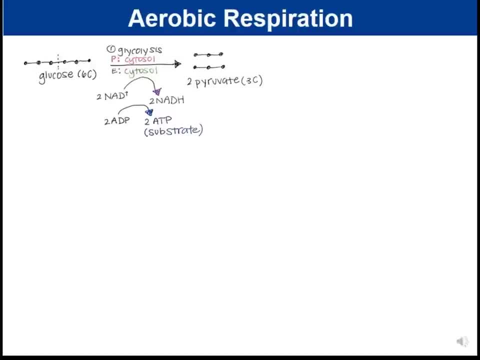 and I've color coded the different parts to try and make it a little easier on you. So here we have our glucose, And glucose, remember, is a six carbon sugar, And so, again, the first step in cellular respiration is referred to as glycolysis. 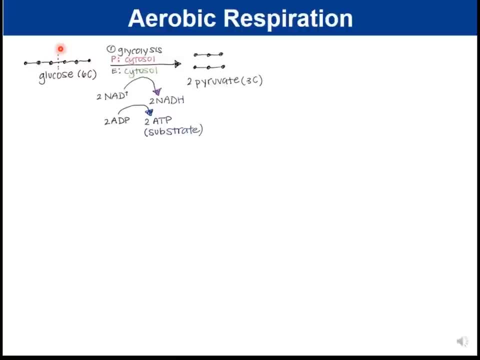 Glyco sugar lysis breaking, And so what that means again is that we're going to break the sugar in half. Now where does it take place? So notice, I've color coded prokaryotic cells. that's the P. 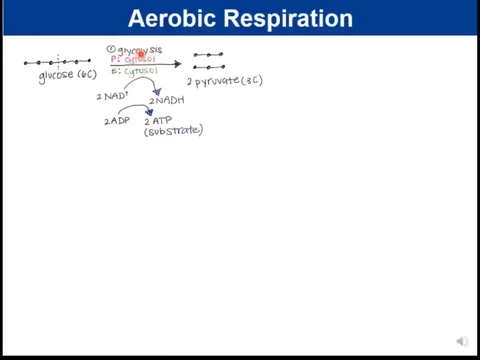 Prokaryotic cells. this happens in the cytosol or the cytoplasm Eukaryotic cells. this also happens in the cytosol. So in both cases this process is going to begin in the cytosol. 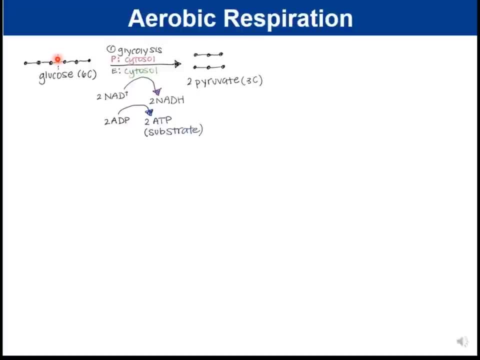 Happens in the cytoplasm of the cell. So in glycolysis again, we're going to break that sugar in half And what we get out are the two, three carbon pyruvates. We also, when we break bonds, 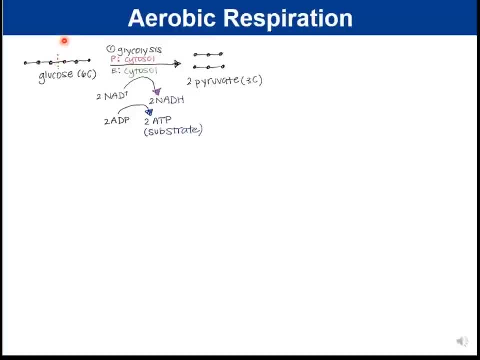 you're going to see this. every time we go through this and we break bonds, electrons are going to be transferred onto electron carriers, So we put in two NAD plus and when the electrons get put on my product, I'm going to get two NADH. 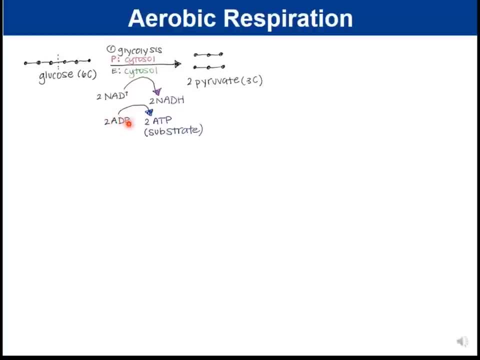 Also, during this process, two ADPs need to be put in adenosine diphosphates and two ATPs are produced by substrate level phosphorylation. So when you're looking at this diagram, everything on this side of the arrow- 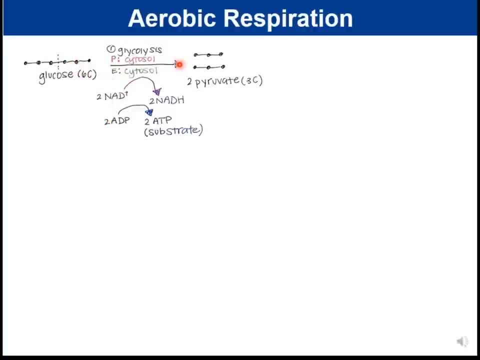 are things that go in. Everything by the arrowhead are things that come out, meaning those are the products. So these are what you need to go in and these are your products. So for each of these steps, you need to study the name of the step. 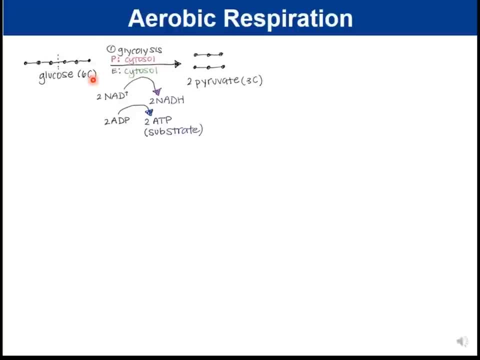 where do they take place? what goes in here's our, what goes in over here and what comes out. These are my products, So keep that in mind when you're studying this. This is what you want to use as your tool to help you understand respiration. 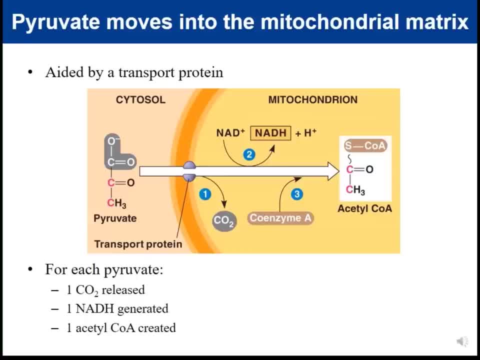 Now remember that I said that in eukaryotic cells, for example, in eukaryotic cells, respiration begins in the cytoplasm or the cytosol and it ends in the mitochondria. So what that means is that the pyruvate 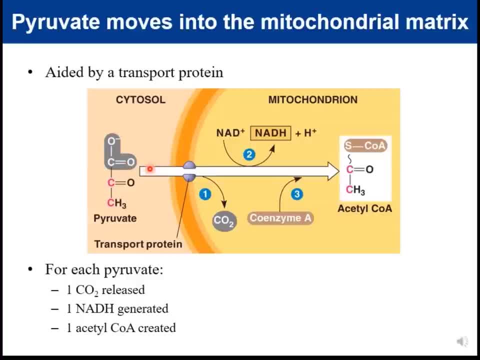 that we produce during glycolysis needs to get transported into the mitochondria. Now notice that this is charged right. There's this charge region. So pyruvate doesn't cross the membrane on its own, It needs a transport protein. 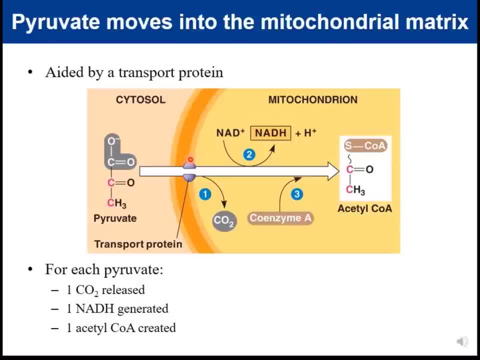 to help transport it. Now, when this happens, when pyruvate goes into the mitochondria, we are going to break off a carbon and we get CO2.. So per pyruvate we get one CO2.. To the remaining two carbon fragments: 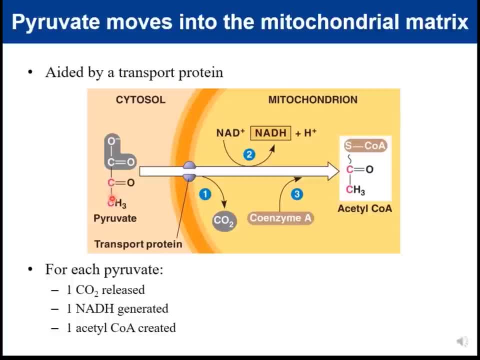 so these two carbons here to the remaining two carbon fragments. coenzyme A is going to come in and it's going to attach to that remaining two carbons. So here's those remaining two carbons from pyruvate and they get a CoA added to them. 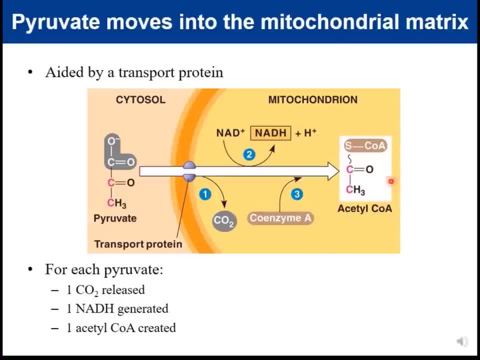 And so now those products are acetyl CoA, So we get an acetyl CoA per pyruvate Notice breaking bonds. We're also going to get our electron carriers, So NAD plus is going to pick up electrons and it's going to form NADH. 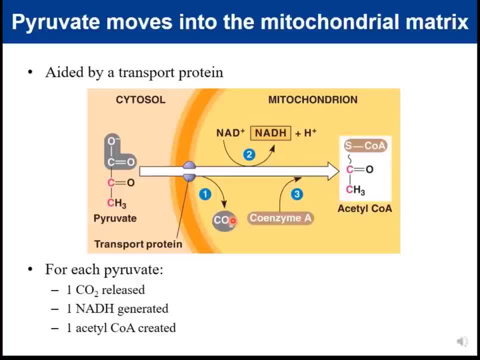 So our products, for each pyruvate, we get one CO2,, we get one NADH and we get one acetyl CoA. So per glycolysis, per glucose, how many CO2s do we get? And the answer is two. 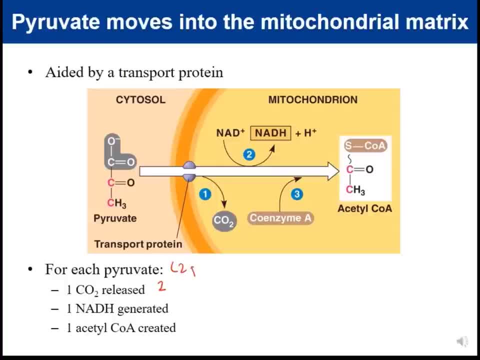 Because per glucose, so two pyruvates per glucose, so we get two CO2s per glucose, we get two NADH per glucose and we get two acetyl CoAs per glucose. So notice this part's easy. Everything is multiples of two. 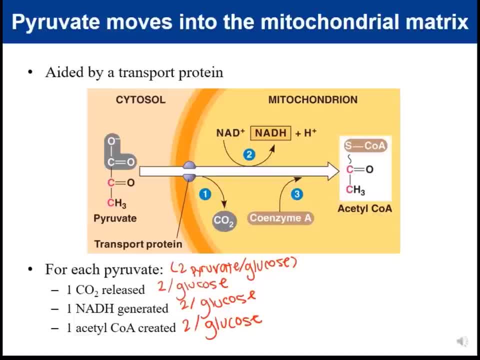 And so this step is not technically a separate step. This step has several different names for it. Sometimes you'll hear it referred to as the transition step. Sometimes you'll hear it referred to as the intermediate step. Sometimes you'll hear it referred to as pyruvate oxidation. 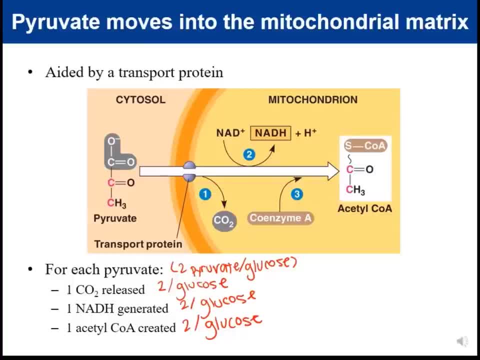 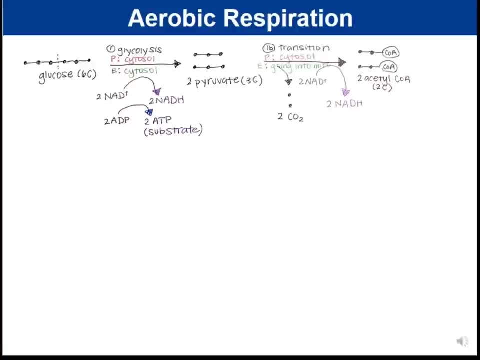 There are a lot of names for this process And so this is basically as the pyruvate is going into the mitochondria, but before the Krebs cycle, So this is like a transition between the two steps. So if we look at our diagram, we're adding on. 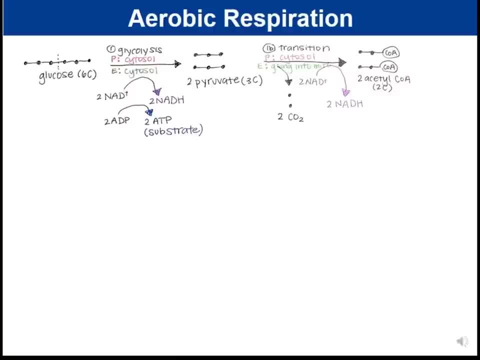 so here are the pyruvates that formed from glycolysis, And so what's going to happen now is we are going to break those bonds. That's where the two CO2s came from, right. So this is going to be a CO2,. 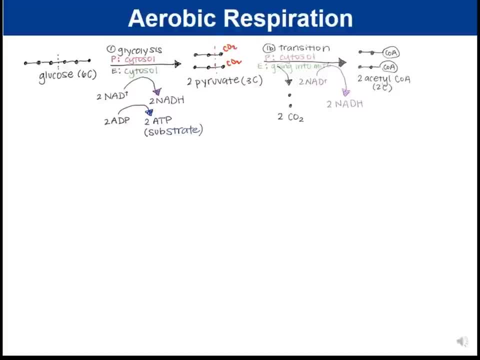 and this is going to be a CO2.. So there's my two CO2s that get produced Broke. some bonds also get some electron carriers. So NAD plus goes in. two NAD plus goes in. per glucose, two NADH come out. 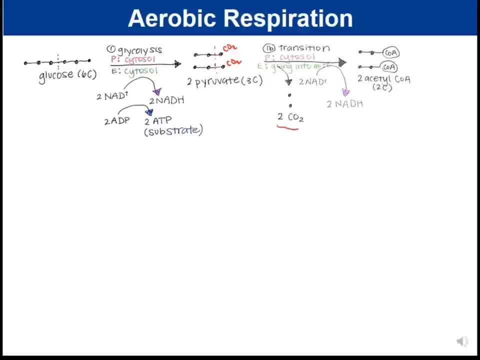 So now we have electrons transferred onto our electron carriers, To the remaining two carbon fragment, so to the rest of the sugar from pyruvate, the two carbon fragment. we get CoA, coenzyme A, added on, So our product is going to be two acetyl CoAs. 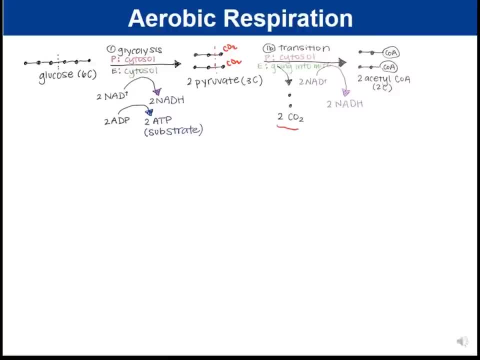 Each acetyl CoA is two carbons, So notice we still have four carbons left. Now I numbered this one B. It's not a separate step, so I'm not going to call it step two. It's the transition or the intermediate. 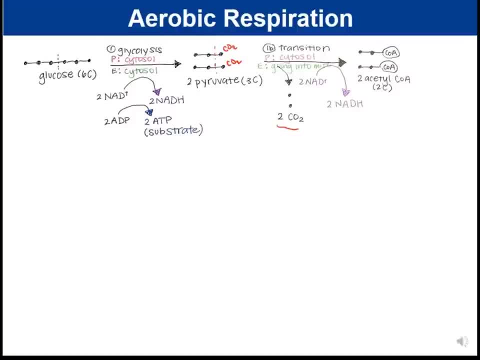 between glycolysis and the Krebs cycle In prokaryotic cells. this is going to happen in the cytosol In eukaryotic cells. this is as the pyruvate is going into the mitochondria, So pyruvate is going to go into the mitochondria. 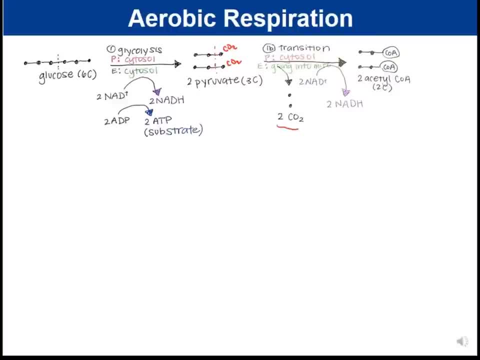 That doesn't happen in prokaryotic cells, because remember that prokaryotic cells do not have membrane-bound organelles, So that going into the mitochondria is distinct for eukaryotic cells. So what goes in Two pyruvates? 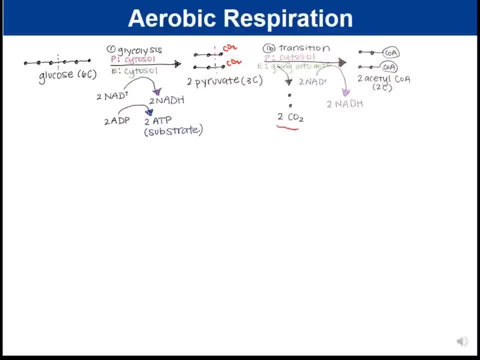 two NAD+. what comes out? Two carbon dioxide, two NADH and two acetyl CoAs. And so again, when you're studying this or when you're taking notes on this, I would actually take the time yourself and draw it out. 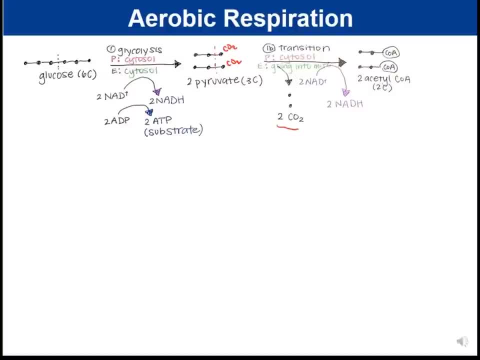 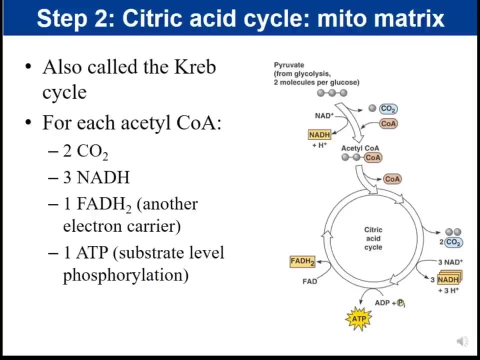 The act of writing it out is going to help you remember it. So this is going to be our transition. Now, step two is going to be the citric acid cycle. Now, when we look at the citric acid cycle, this is going to take place. 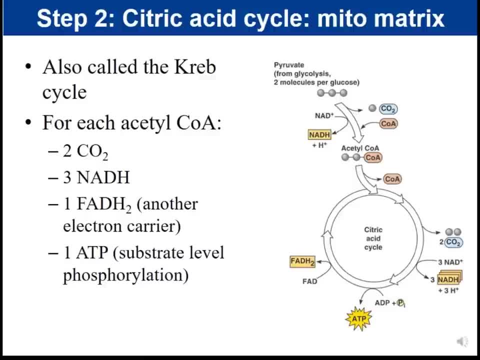 in eukaryotic cells in the mito matrix. So if you recall kind of the structure of the mitochondria, it has the smooth outer membrane, It has this extensively enfolded inner membrane Which is also called the cristae, And the matrix is the space. 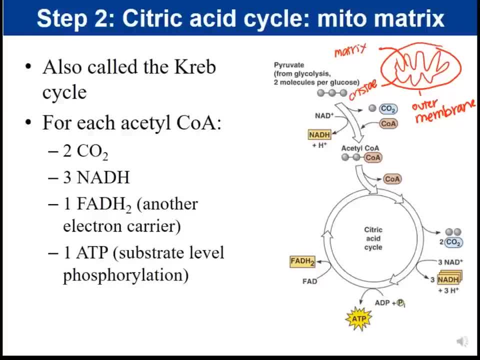 inside the inner membrane. So this is going to take place, this citric acid cycle, otherwise known as the Krebs cycle. I more often will call it the Krebs cycle. But again, citric acid cycle is another name. The TCA cycle is another name. 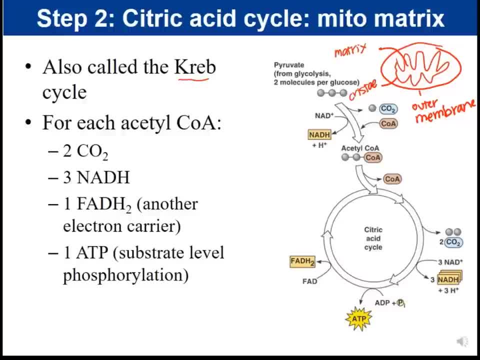 There are multiple names that this process is referred to as. And so in eukaryotic cells, this is going to take place in the mitochondrial matrix. Where would you guess that this takes place in prokaryotic cells? In prokaryotic cells? 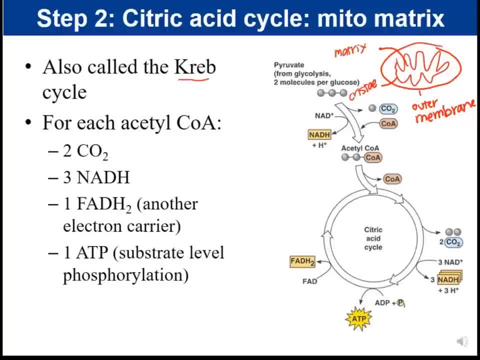 still in the cytoplasm Right. They don't have a separate membrane bound organelle to do this, So they're going to do this in their cytoplasm. So now, here we have our acetyl CoA. that was produced from: 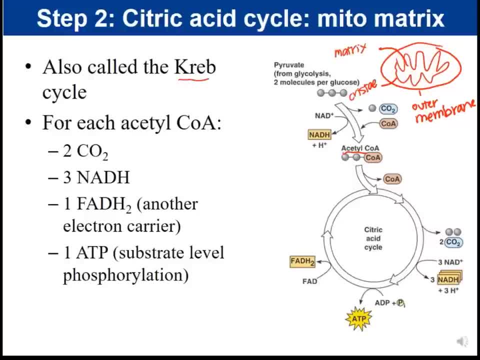 the transition step. So per acetyl CoA. when acetyl CoA goes into the Krebs cycle, we are going to break down the sugar or break down this molecule completely. We're going to release each carbon. So notice that my product. 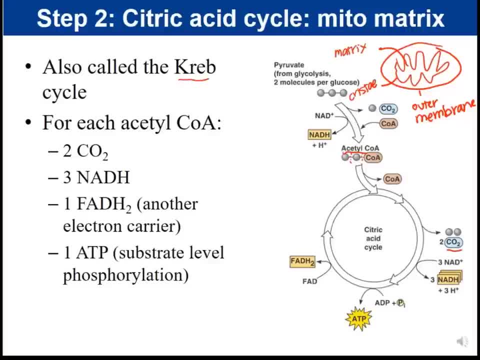 two carbon dioxide. This is one CO2.. This is a second, So we get two CO2s. We broke more bonds, So we're going to get more electron carriers. in this step, We have three NAD plus going in. They're going to pick up electrons. 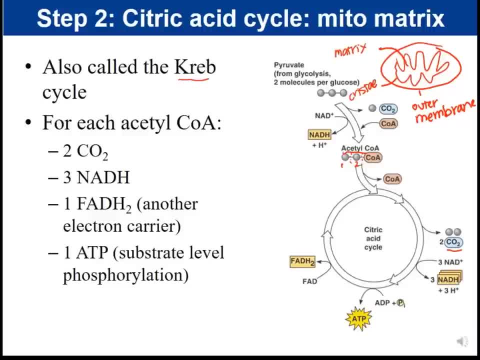 and they're going to form three NADH. So three NADH are the products per acetyl CoA. We also get one ATP by substrate level, phosphorylation, And we get another electron carrier and that is the empty one is FAD. 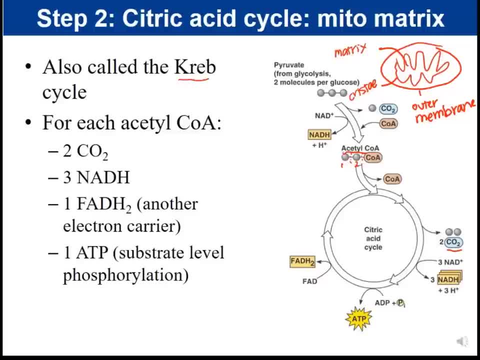 And when it picks up its electrons and its hydrogen, it becomes FADH2.. So per acetyl CoA, we get two carbon dioxide, We get three NADH, We get one FADH2, which is again another electron carrier. 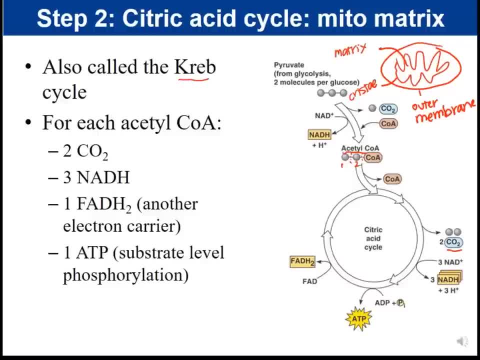 and one ATP per substrate level phosphorylation. So, per glucose, how many CO2s do we get? And the answer is four, because we had two acetyl CoAs. So we get six NADH. per glucose, We get two FADH2s. 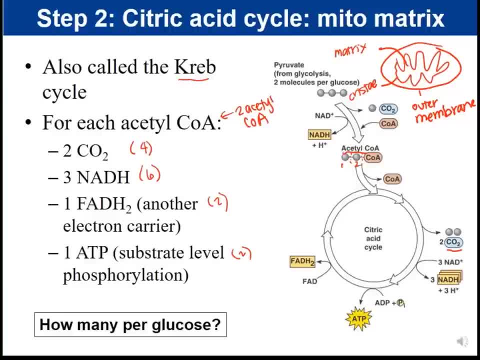 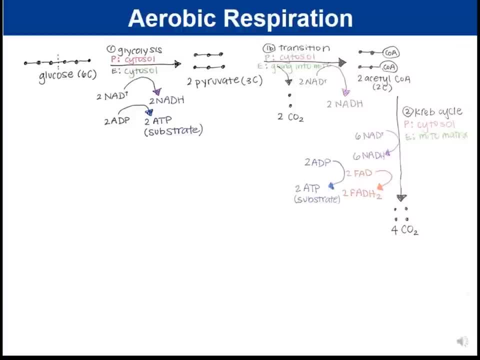 And we get two ATP by substrate level, phosphorylation, And so we're going to add this on to our diagram. So here is the next part of our diagram. So here we have step two: Krebs cycle, Again in prokaryotic cells. 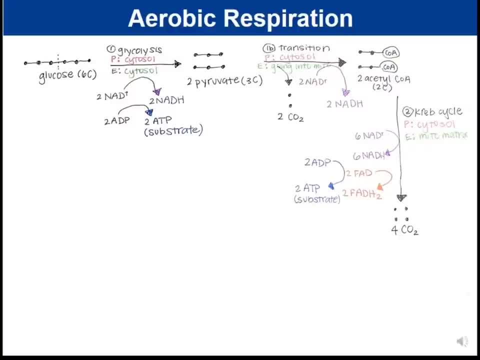 that's going to take place in the cytosol. So all of this still happens in the cytosol. In eukaryotic cells, this is going to take place in the mito matrix, the innermost part of the mitochondria. 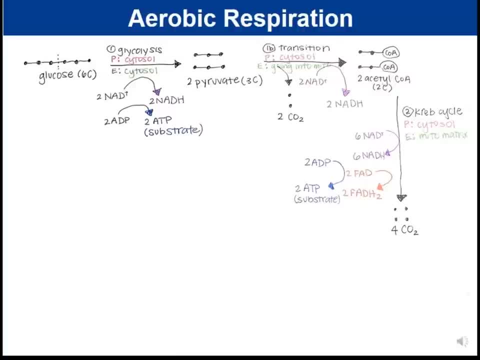 And so what's going to happen again is per glucose. these are all per glucose. we have six NAD plus going in. They're going to pick up electrons. We get out our product. Our product is six NADH. We put in two FADs. 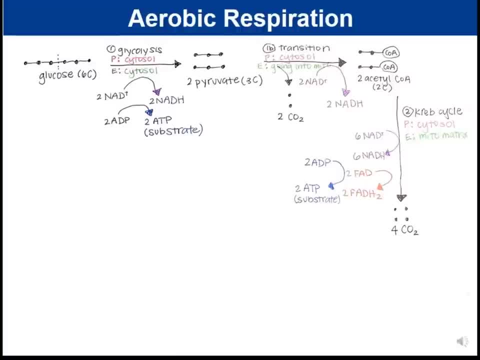 which is another electron carrier. What we get out are two FADH2s. So the FAD has become reduced, It's gained its electrons, It's gained its hydrogens And it's energy rich. We put in two ADPs. 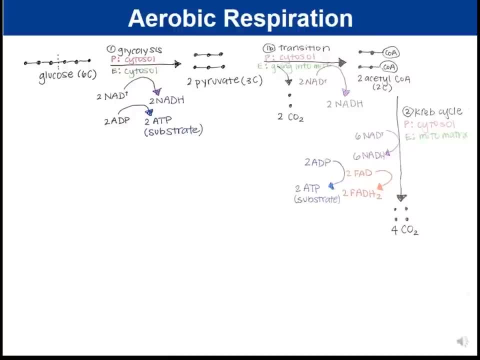 adenosine diphosphates, And what we get out are two ATPs, And those ATPs are produced by substrate level phosphorylation. So again, it's going to be a substrate during this process that's going to transfer a phosphate group. 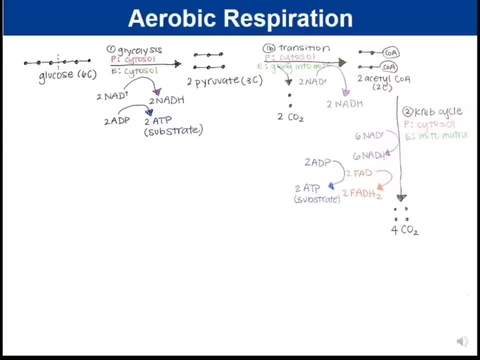 onto ADP And that's going to form ATP. Now the other important thing is we're breaking all of these bonds, And so notice that the other product that we get out are four carbon dioxide, So notice that we got two during the transition step. 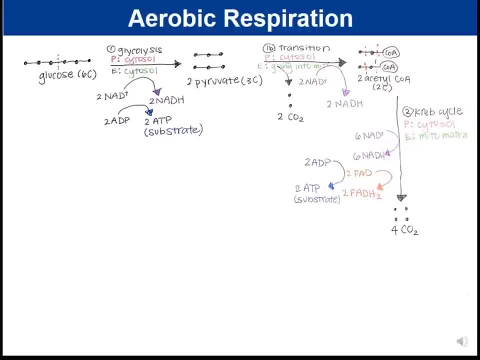 and four during the Krebs cycle. That's a total of six CO2s. Does that make sense to you? And it should, because we started with a six carbon sugar. We should end with six carbons when we're done. We do. 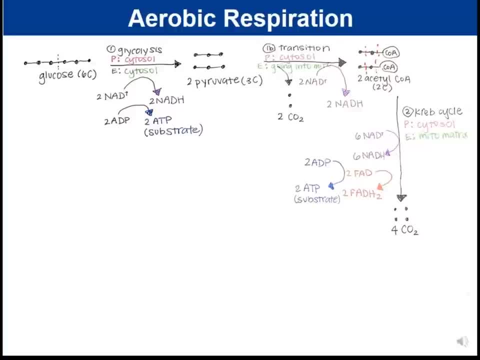 We have six CO2s. Those are six carbons, So that tells you that you did this right. You should still have six carbons when this is all finished. If not, you forgot some, because glucose is a six carbon molecule. So those are our six carbons. 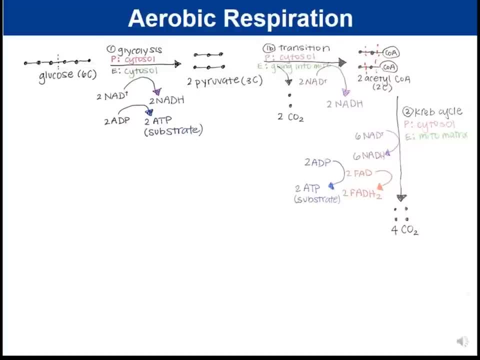 Those are the six CO2s that we get, So this is going to be our Krebs cycle. Now what I want you to really notice, though, is when you look at this diagram, look how little ATP is produced. We get two ATP in glycolysis. 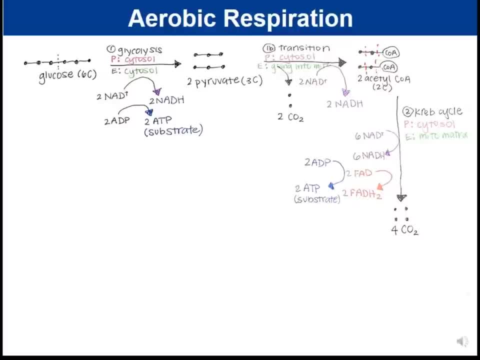 We get two ATP during the Krebs cycle, Yet in the overall process of aerobic respiration we get 30 to 32.. So that means that 26 to 28 ATP are produced in the last step, meaning in the electron transport chain. 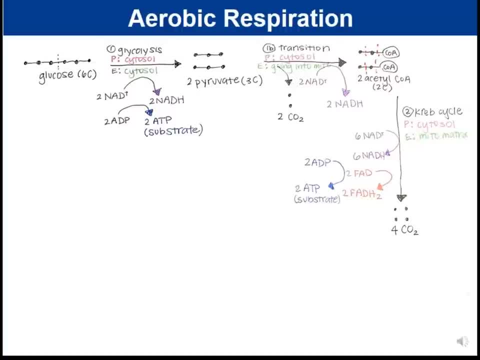 So then, what was the point of doing all of those earlier steps? It wasn't to yield ATP, because we didn't get much ATP. The important products that you get from the beginning of the cycle are the electron carriers. That's where the energy is. 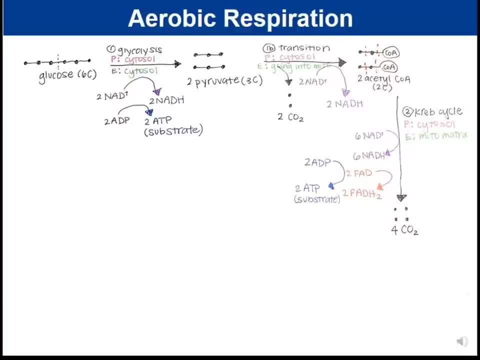 So we got two in glycolysis, two NADH in glycolysis, We got two NADH in the transition, We got six more in the Krebs cycle And we got two FADH2s. So those electron carriers. 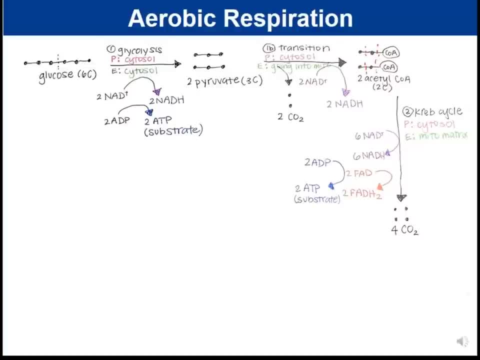 are actually the important products that happen during those earlier steps. So the whole idea of this is that we're breaking down the sugar little by little, And when we do this in a stepwise manner, what's actually happening is is that we're transferring electrons. 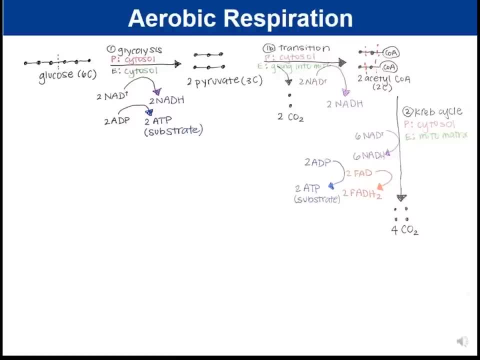 onto these electron carriers. The electron carriers can then go drop off electrons at the electron transport chain, And when they do that, that is where the bulk of the ATP is going to come from. So again, the important products during the first two steps. 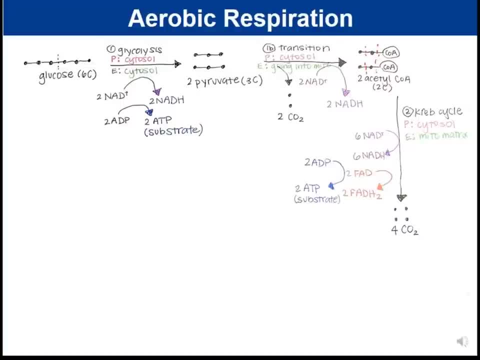 are the electron carriers. That's where the energy is. When they have their electrons, they are energy rich, And when they drop off those electrons, those electrons can be used to make ATP by oxidative phosphorylation, which we're going to see in a minute. 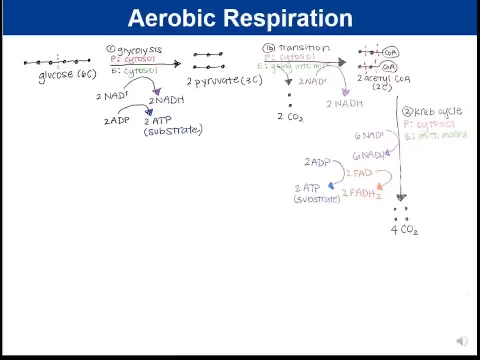 So, again, what I want you to take out of this is: what is the point of this? The point of these early steps is not ATP, because we get relatively little ATP, but the purpose is break down the sugar little by little and get your electron carriers. 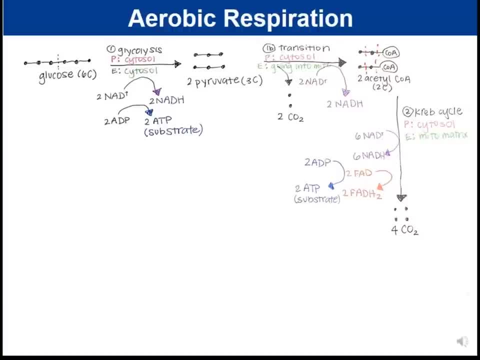 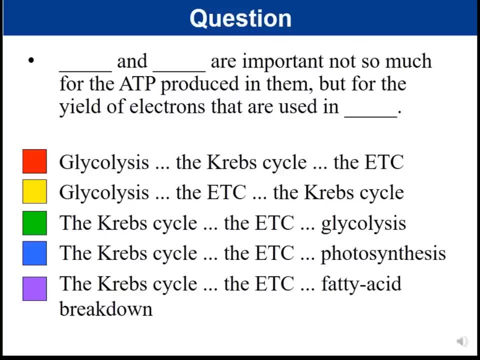 That's where all the energy is, because the electron carriers are going to go to the electron transport chain and that's going to be where the bulk of the energy is going to come from. So I have a question for you. Blank and blank are important. 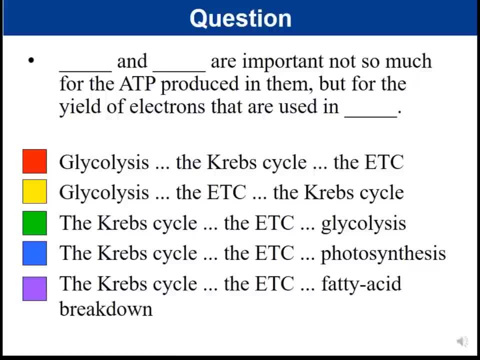 not so much for the ATP produced in them but for the yield of electrons that are used in blank. So red says glycolysis, the Krebs cycle and the ETC. ETC stands for electron transport chain, Yellow says glycolysis. 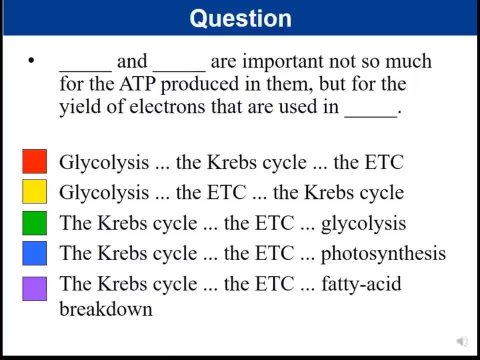 the ETC- the Krebs cycle- Green Krebs cycle, ETC- glycolysis- Blue Krebs cycle. ETC- photosynthesis- Purple- the Krebs cycle, the electron transport chain and fatty acid breakdown. 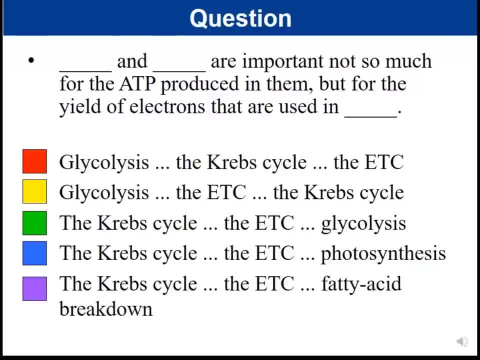 So you can pause your video and when you're ready again push play to hear the answer. And so the correct answer. red Glycolysis and the Krebs cycle are important, not so much for the ATP produced in them. so, again, they don't produce much ATP. 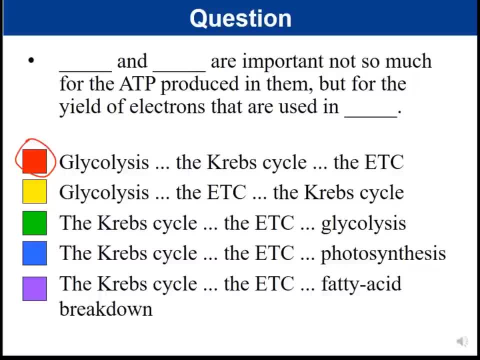 but for the yield of electrons that are then used in the electron transport chain. So again, we're breaking down the sugar little by little and transferring electrons onto electron carriers. Those electrons will then go to the electron transport chain to generate the bulk of the energy. 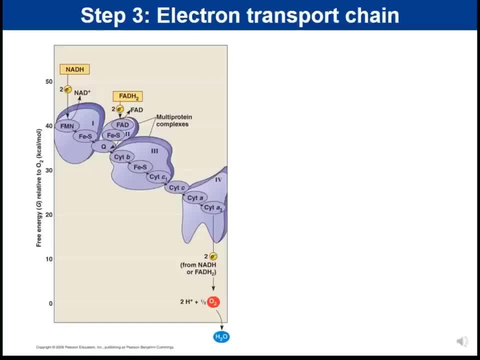 So we're going to move on to step three And we're going to talk about the electron transport chain. So if we're talking about eukaryotic cells, right In eukaryotic cells, this is going to take place in the cristae. 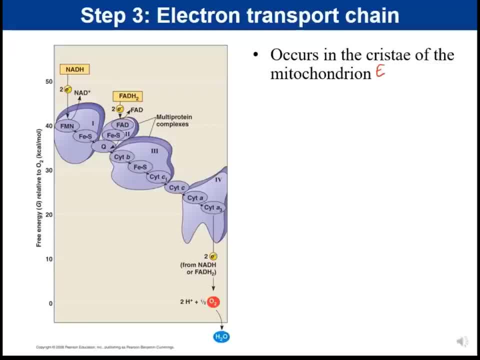 So eukaryotic cells is going to take place in the cristae, which, remember, is the inner membrane of the mitochondria, And so what happens in this process is that embedded in that membrane are these large multiprotein complexes, And they're just numbered. 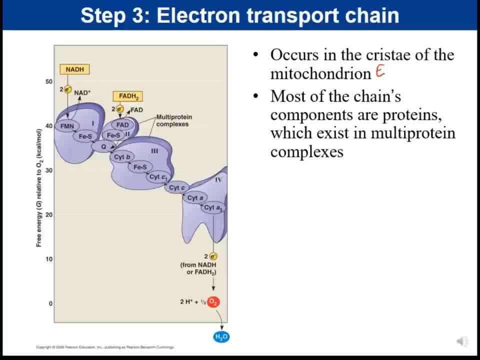 so this is complex one on the far left, and then complex two, complex three and then complex four. And so there are these large multiprotein complexes Now in eukaryotic cells. this occurs in the cristae of the mitochondria. 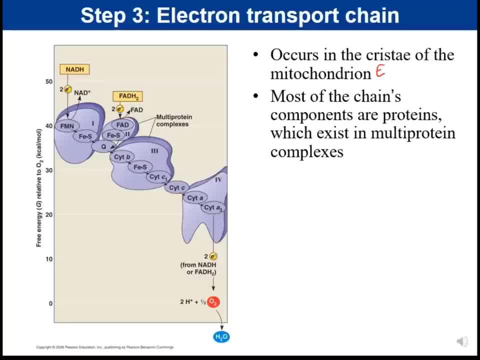 Meaning that these electron carriers, these protein complexes, right? These are embedded in a membrane. Do prokaryotic cells have a mitochondria? And the answer is no. Prokaryotic cells do not have membrane-bound organelles. However, do prokaryotic cells 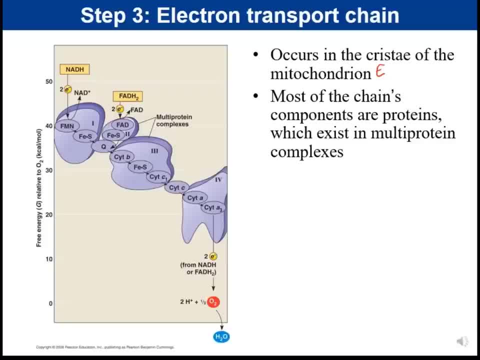 do the electron transport chain? And the answer is yes, they do. What membrane are they going to use instead? They're going to use their cell membrane, Because you're going to see in a minute that you need to have a gradient of hydrogens. 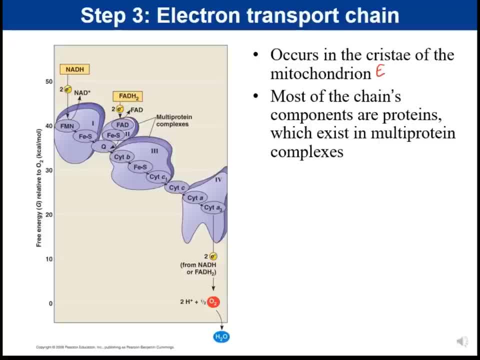 across the membrane. So you have to have this process spanning a membrane, And we'll come back to the hydrogens in a minute. So let's talk about how the electron transport chain works. We have our electron carriers, our NADH. 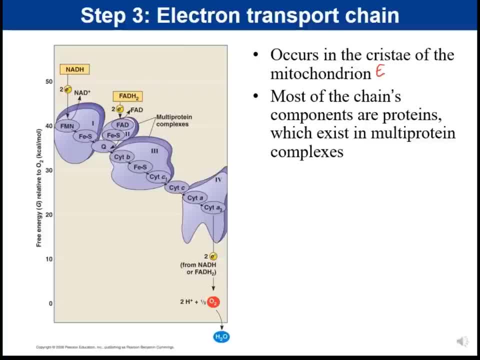 NADH is going to drop off electrons at the electron transport chain And when it drops off electrons it's going to produce NAD+. Now it's released its passengers. it's empty. the NAD plus is ready to go back and pick up more passengers. 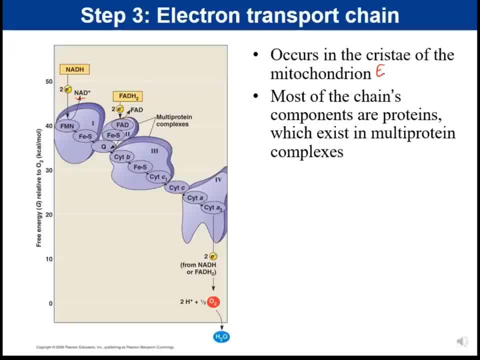 pick up more electrons and keep the process going. NADH, when it drops off electrons, it drops it off to the first electron carrier in the pathway, So the FMN is the first one. So NADH donates electrons. 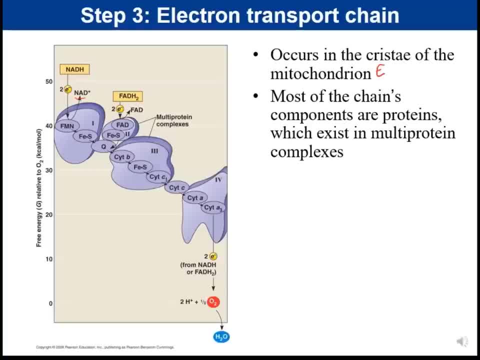 So do we say that NADH became oxidized or reduced? It lost electrons, so it became oxidized and the FMN became reduced. It gained the electrons. Now that FMN is going to pass it to FES, the next carrier, 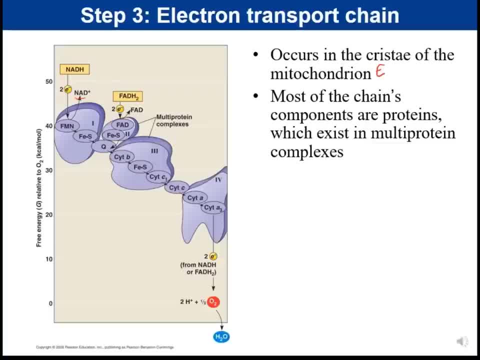 So it's going to pass the electrons to the next carrier. So now it was reduced when it gained electrons- FMN- but when it donates it now it becomes oxidized and the next carrier becomes reduced And then that carrier passes it. 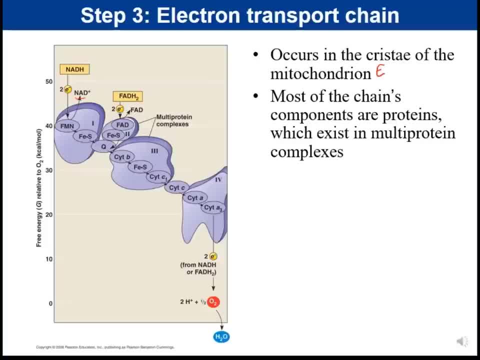 and it goes from being reduced to being oxidized, and the process continues. So what you end up with is: you end up with these alternations of oxidation and reduction: Oxidation and reduction as the electrons are passed down the chain, And so they're going to. 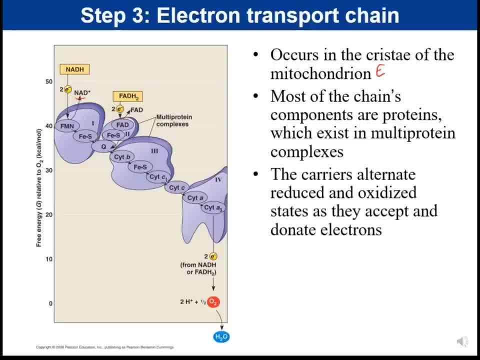 alternate between these oxidized and reduced states. Now, why do electrons even move down the chain? What is the force that is pulling them down the chain? Well, remember in lecture when we talked about- in the chemistry part of our lecture we talked about 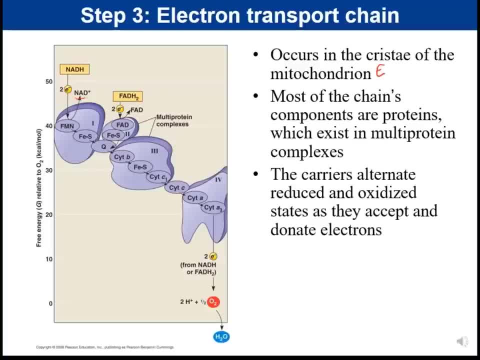 electronegativity, And electronegativity is the affinity of atoms for electrons, meaning how much do they want those electrons? So if something has a higher electronegativity, it means that they have a greater affinity for electrons than they have a higher affinity for the electrons. 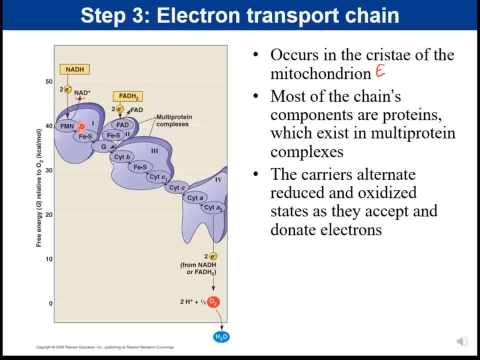 So this carrier is more electronegative than this one, which means it has a higher affinity and it's going to pull the electrons from this one. This one is more electronegative than this one. It's going to pull the electrons. 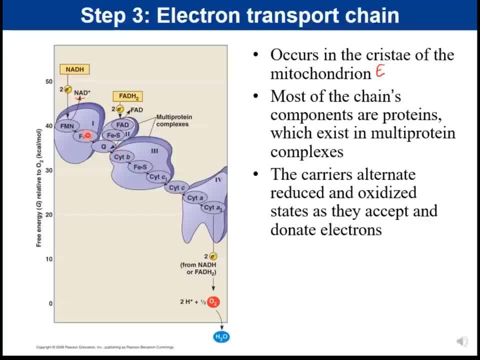 This one is more electronegative. It's going to pull the electrons, And so each of these carriers gets progressively more and more and more electronegative, which is helping pull the electrons down the chain. Now, when the electrons 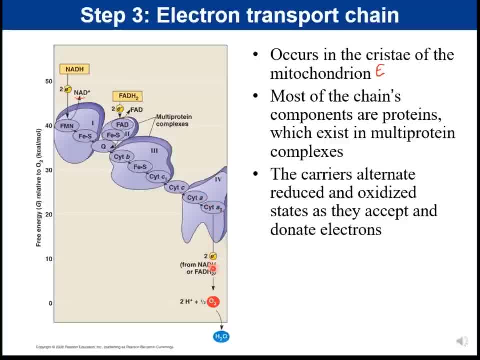 get to the end of the chain, we are going to have the electrons transferred onto O2.. Remember we said, if we're talking about anaerobic respiration, O2 is our final electron acceptor. It's what's going to take the electrons. 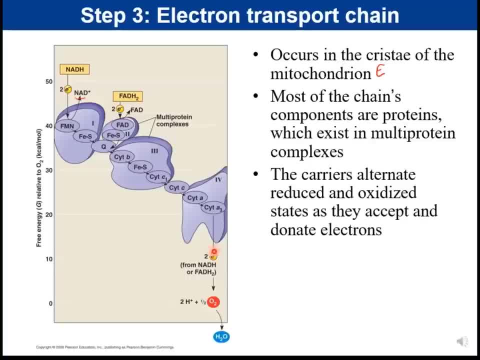 from the electron transport chain. When it takes the electrons, O2 is going to become reduced, right? It gained electrons and it gained hydrogens and it formed water. So the water that we get in cellular respiration comes from O2 being reduced. 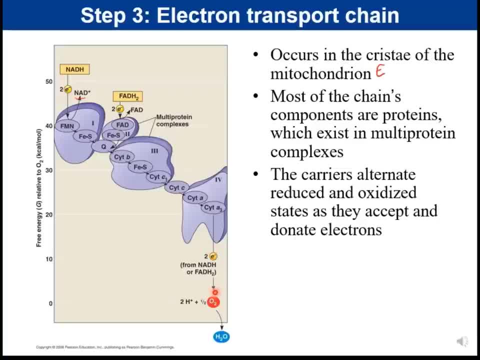 O2 is going to gain electrons and hydrogens and it's going to form water. So, if you ever think about, why do you have to breathe? well, the reason you have to breathe is that you need this O2 to be the final electron acceptor. 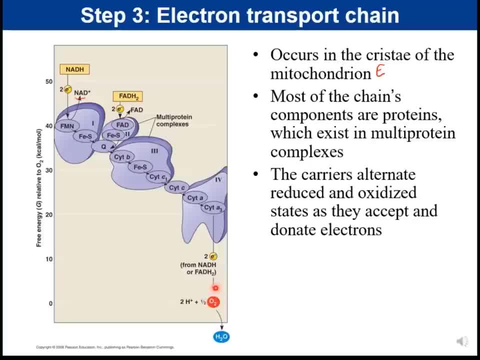 Right, Something has to take the electrons from the chain. So if O2 is not available, the electron gets stuck at this one. And then the electron then gets backed up at this one Because it can't pass it to the next carrier. 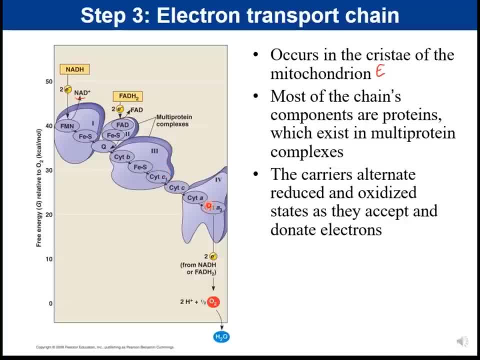 That can't pass it to this one. So what you end up with is you end up with this backlog of electrons that can't move down the chain because they have nowhere to go. There's an electron stuck here, So you can imagine this being like a pipe. 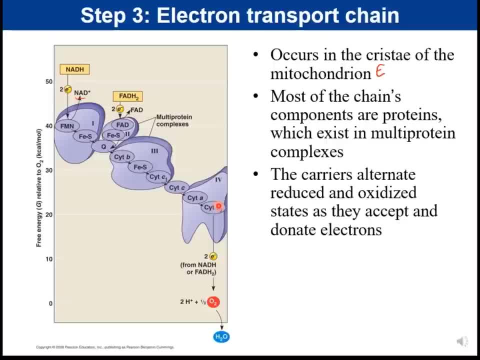 and there's a clog in the pipe, There's something that's blocking that let's say hairball from moving through the pipe, Because if it's blocked, nothing else is going to pass. There's nothing to get it out of the way. So 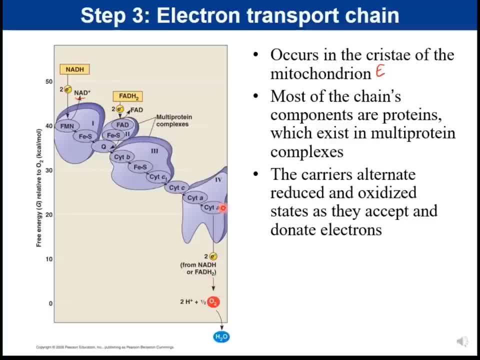 we have to breathe. The reason we need to breathe is we need O2 to be that final electron acceptor, And so O2 is going to be the final electron acceptor, And if it's not, then these electrons can't get passed down the chain and 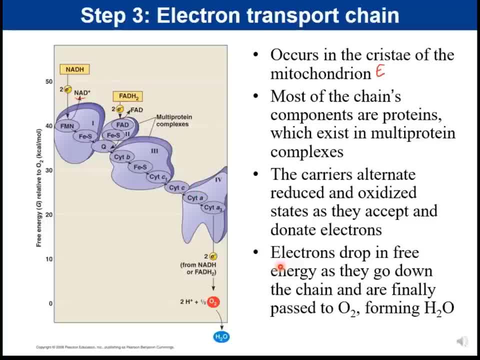 therefore can't produce ATP. So one of the things that you're going to see in a minute: electrons drop in energy as they go down the chain, And what that means is that as they're moving down our chain, they're going to give off a little bit of energy. 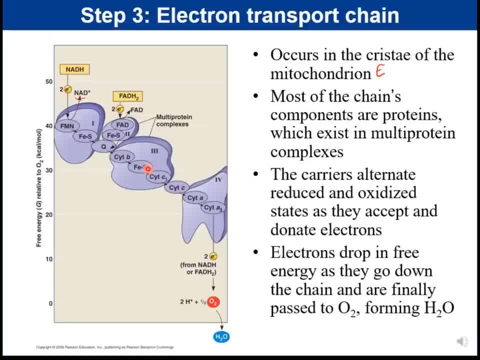 They're going to lose a little bit of energy along the way. You're going to see in a minute that the energy that is released from the electrons moving down the chain is going to be used to pump hydrogens against the gradient. So we're going to see that in just a second. 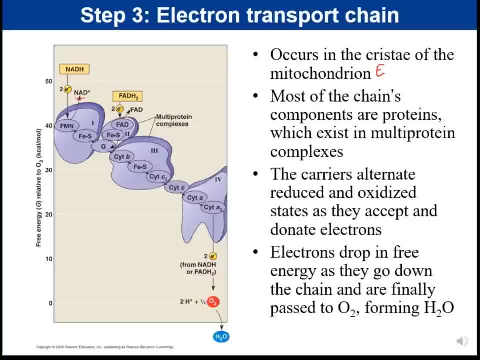 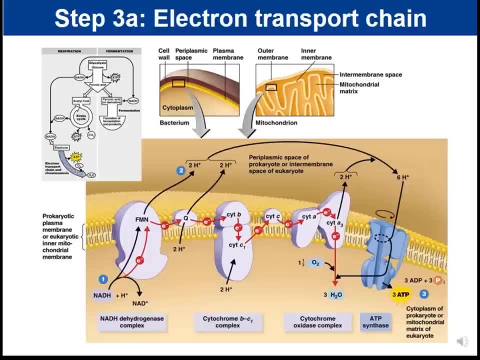 Because, again, notice, this part we're looking at here shows nothing about ATP production. Notice, there's nothing that has to do with ATP production in this slide yet. So what we're looking at here is we're looking at the electron transport chain and how ATP 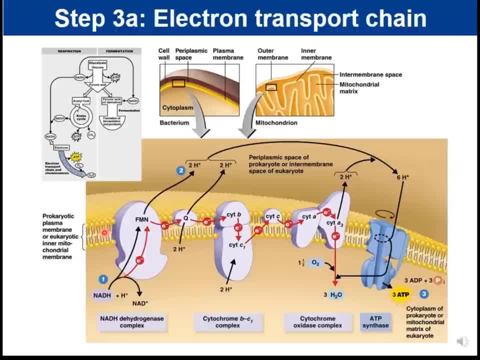 is produced. So again, this is the membrane. This membrane is going to be the cristae of the mitochondria. the inner membrane, This space down here, is going to be the matrix. That's where the NADH is going to be. 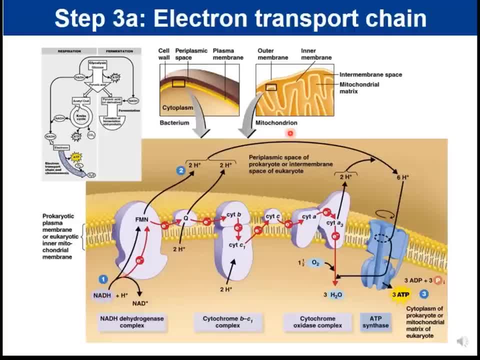 produced from the Krebs cycle. So this is the matrix. Out here in eukaryotic cells is the intermembrane space. Now in prokaryotic cells this is a little bit different. This membrane is not the cristae. 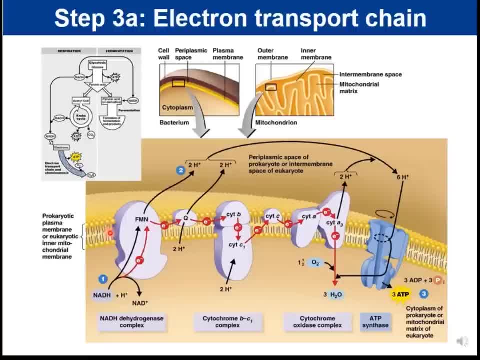 because, again, they don't have mitochondria. This is their cell membrane, Prokaryotic cells, this is their cytoplasm or cytosol, And this is the periplasmic space, so the space between the cell membrane and the cell wall. 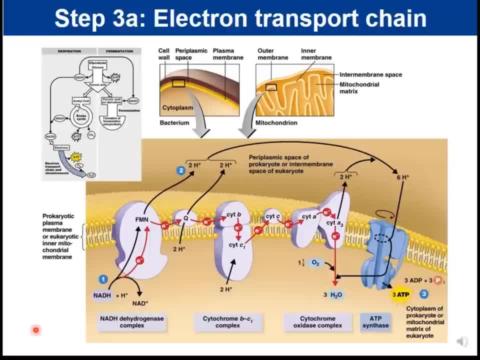 In prokaryotic cells. So, to understand the electron transport chain, one of the things that we need to put on here are the hydrogen ions. So on this side of the membrane, which let's say that we're talking about, 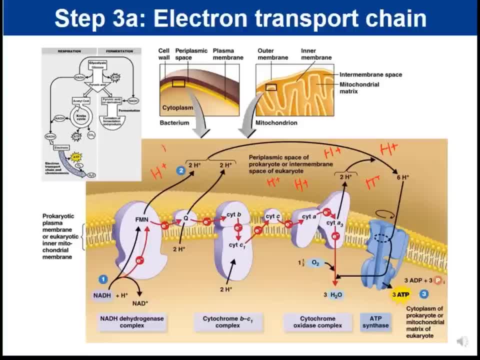 eukaryotic cells for a minute. this would be the intermembrane space And in here would be the matrix, So notice that again, I'm going to use this as in terms of eukaryotic cells, So notice that. out here the 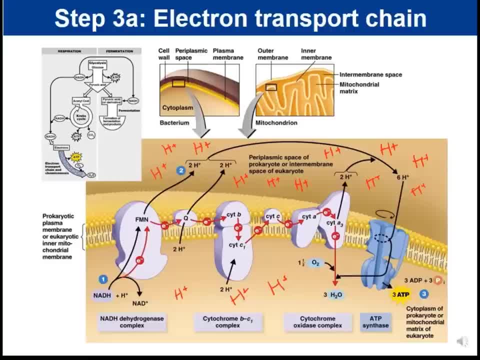 intermembrane space has a higher hydrogen ion concentration relative to the matrix. So when my NADH comes in and it drops off electrons at the electron transport chain, again NADH becomes oxidized. it's going to produce the NAD+. 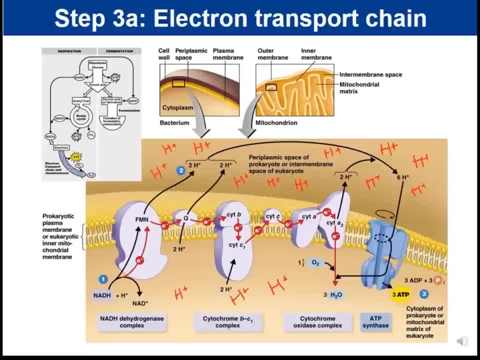 NAD plus can go back and it's going to pick up more electrons to bring back to the electron transport chain. So NADH comes along, it's going to drop off electrons at the electron transport chain. Now this carrier is more electronegative. 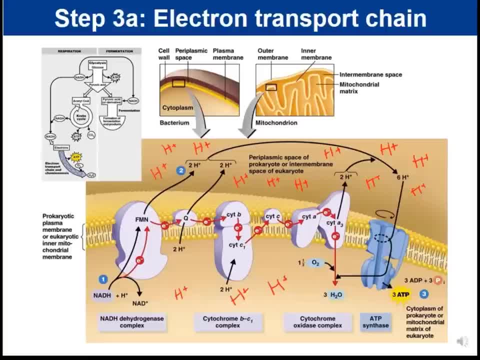 the FMN and then it's going to pass it to the next carrier. and remember that each of these carriers becomes more and more and more electronegative. So as the electrons go down the chain, remember that they're going to give up a little bit of energy. 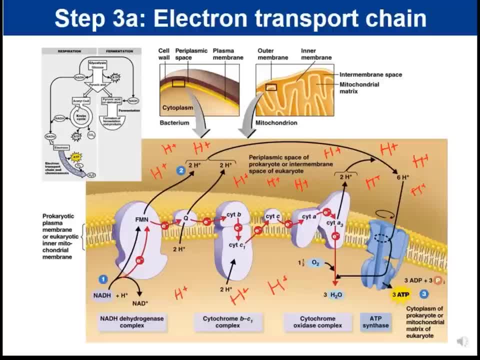 They're going to lose some energy along the way, And what happens is that the energy that it's giving off is used to pump hydrogens against the gradient Meaning: it's going to pump hydrogens from a low concentration to where it's high. 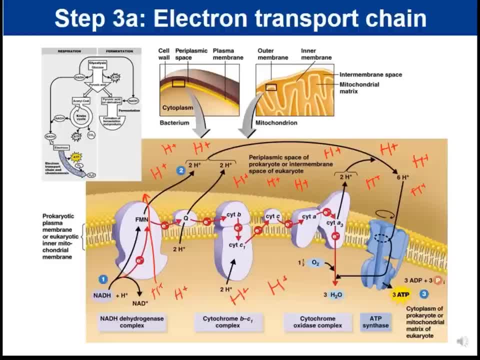 Do molecules normally want to move from low to high spontaneously? And the answer is no, Right, If I have a beaker of water and I add food coloring to that beaker, the dye is going to go from the high concentration, meaning the drop. 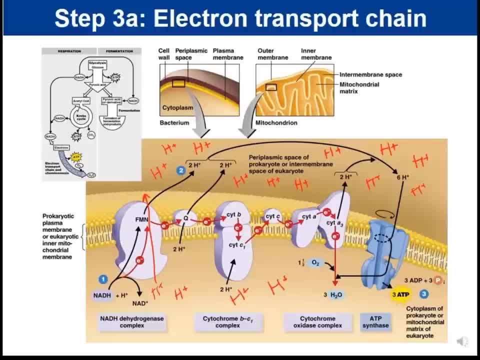 to the low concentration which is the water around it. It's never going to be all spread out and spontaneously go back to being a drop. Not going to happen. Going from low concentration to high is not a spontaneous process, So hydrogens don't want to. 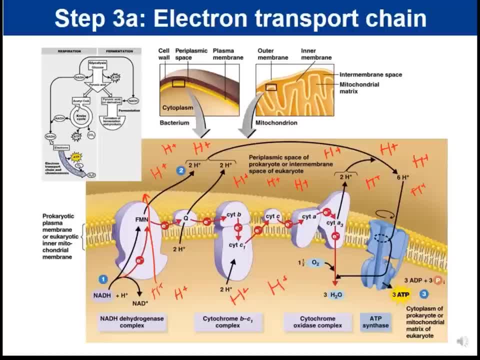 move from low to high, Something has to drive that movement, And what is powering the hydrogens to be pumped across the gradient- or against the gradient, I should say- is that those electrons, as they go down the chain, they give off energy. 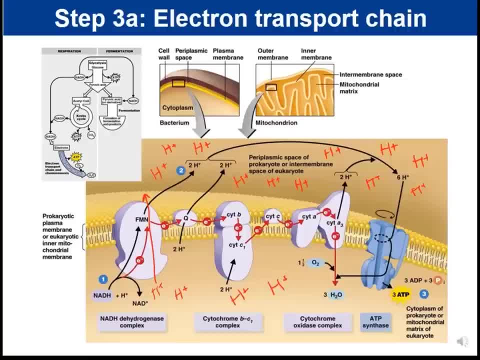 And it's that energy that's used to pump the hydrogens against the gradient. So the energy to pump the hydrogens comes from the electrons. Now again, O2 is going to be our final electron acceptor. It's what's going to take the electrons. 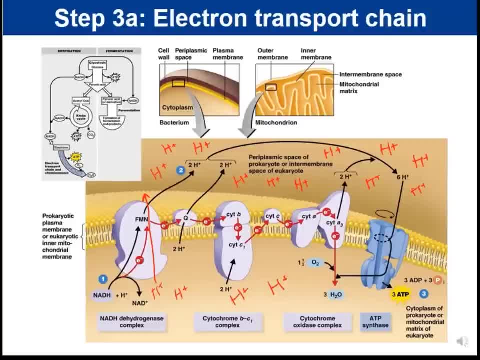 from the chain and it's going to take the electrons and it's going to reduce the O2 to form water. Now, again, that part is still not showing us anything about ATP production. So where does the ATP come from? Well, 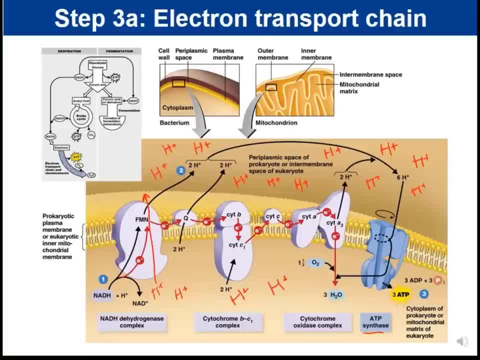 if you look at this blue molecule over here, this is ATP synthase. The name tells you what it does. ATP synthase is used to synthesize ATP. It's going to make ATP. How does this work? Well, hydrogens are now going to. 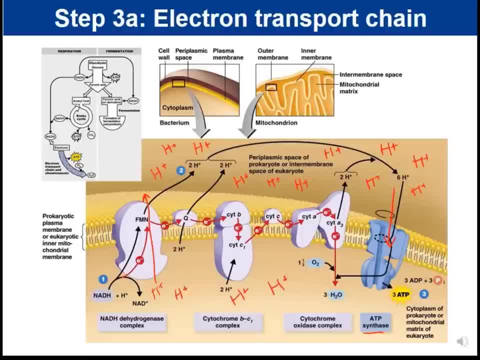 flow back down the concentration gradient. Now hydrogens are going to go from high to low, and when they go from high to low, that movement is favorable. right Things want to go from high to low. That is a spontaneous process That is energetically favorable. 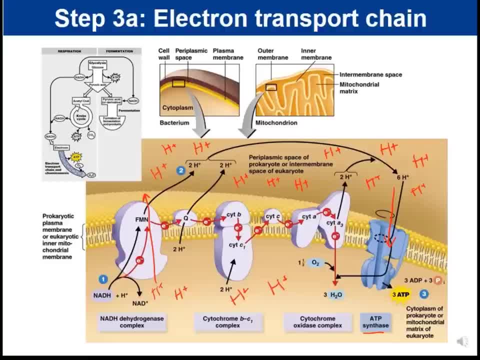 So what happens is is when the hydrogens go back down the gradient, that movement of hydrogens through ATP synthase causes this rotor to spin. It causes this rotation And that rotation, that movement, when it causes the rotor to spin, causes. 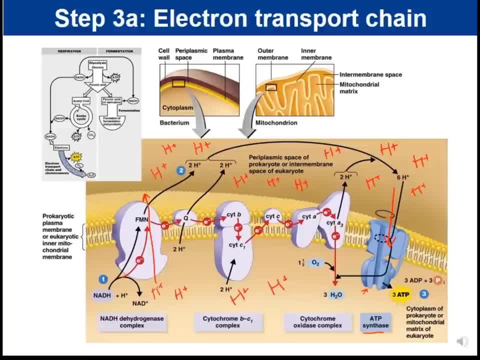 these catalytic knobs, this bottom part, to move. We have now mechanical motion right, And so these catalytic knobs are going to move and that kinetic energy, that energy of motion, is going to be used to produce ATP. So 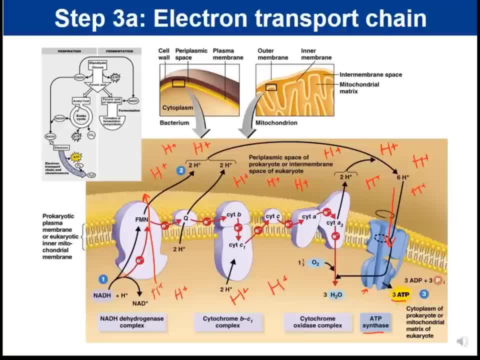 this type of ATP production again is referred to as oxidative phosphorylation, Because we're getting ATP not from transferring a phosphate from a substrate. in this case, we're producing ATP because of these redox reactions, So the electron transport chain, which is basically a 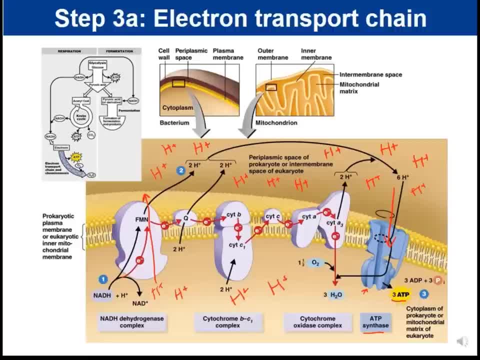 big redox reaction when we donate electrons from one carrier to the next. when they get passed along the chain, that pumps hydrogens against the gradient. So it's going to pump the hydrogens from low to high, Those high concentrations. now we have an even greater hydrogen ion. 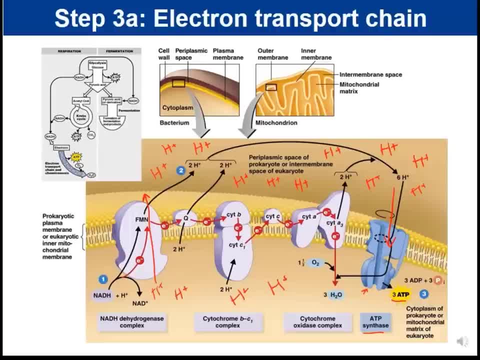 gradient, meaning we have more hydrogens in the space out here. Hydrogens are going to go back down. They're going to go from high to low. That is energetically favorable, That is going to produce the ATP. And so this is where 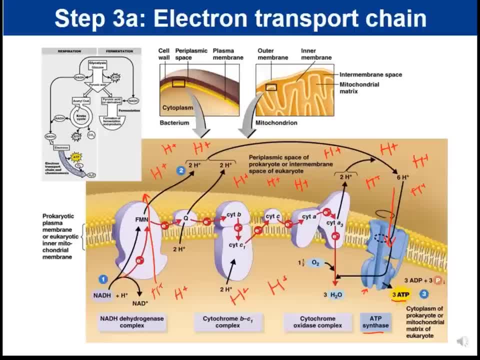 the bulk of the ATP comes from. Now back to why oxygen has to be your final electron acceptor, Because what happens is, if O2 is not present, the electron gets stuck here. It has nowhere to go. The electron gets stuck here, It gets stuck. 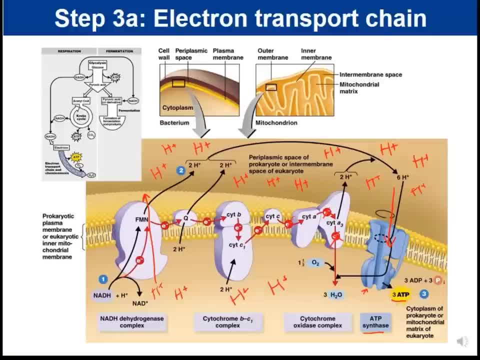 here, all along the chain, The electrons can't move from the carrier they're at. If they can't move, we can't pump hydrogens, because the electrons moving down the chain is what's giving off energy and that energy is what's pumping hydrogens. 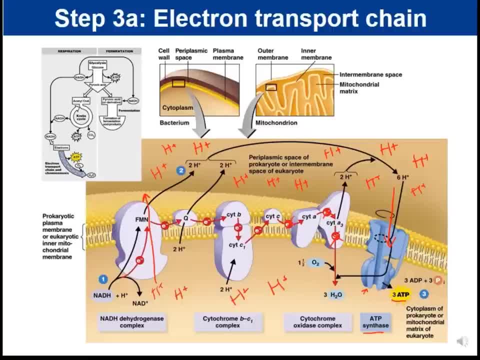 against the gradient. So notice that without O2, we can't pump hydrogens against the gradient. If we no longer have that gradient, if we no longer have that high concentration of hydrogens, the hydrogens are not going to flow from high to low because that gradient. 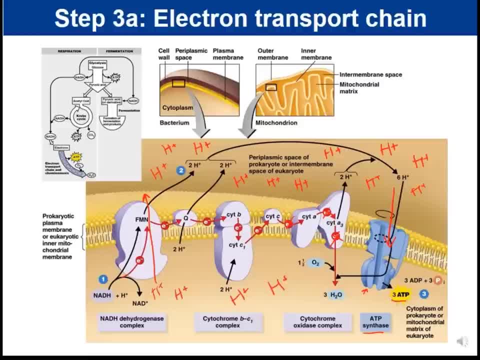 is disrupted and the cell's not going to be able to produce ATP. And this is why, if you go without oxygen for too long, you end up dying, Because your cells need that O2 in order to make ATP. Without it, they're not going to make enough ATP. 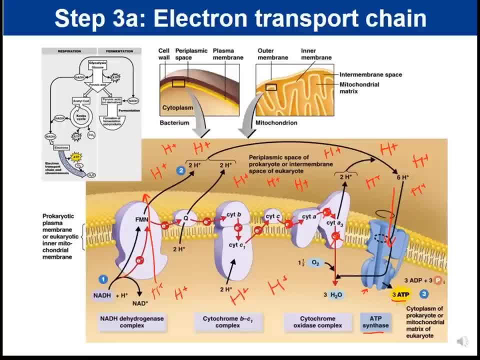 for you to survive. Now let me give you a little bit of an analogy about how ATP synthase works. I do have some videos that I'm going to include on Canvas that are good study tools for studying cellular respiration And it kind of helps illustrate how. 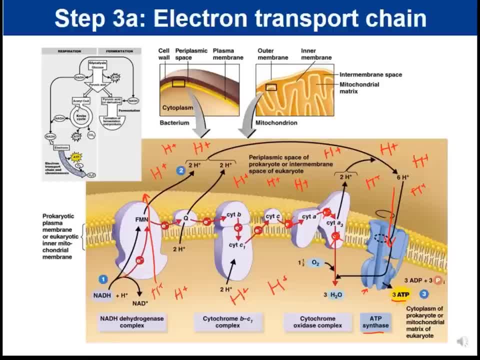 this ATP synthase, how it rotates, And so it's good to watch and kind of see how ATP synthase works. But let me kind of describe it for you. So if you've ever seen a dam, right, so here's our dam. 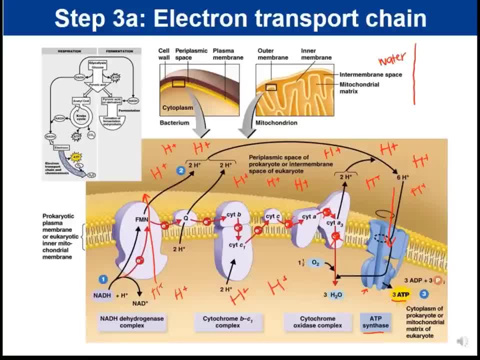 and here's our water. And so the water is behind the dam, and then there is a pinstock, this tubing or this opening where, when they open the dam, the water can go into this pinstock. Now at the 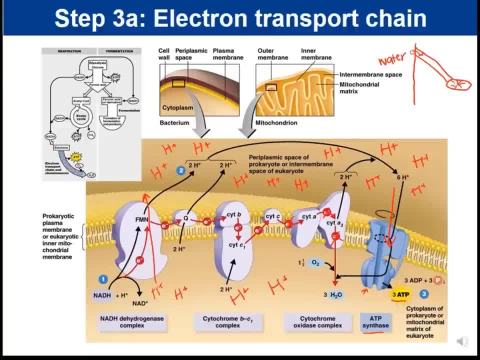 bottom is a little turbine that spins. So if the water, if the dam is opened and the water goes down, notice it's going from higher up to lower, it's going from high to low and that movement of water causes that turbine at the bottom to 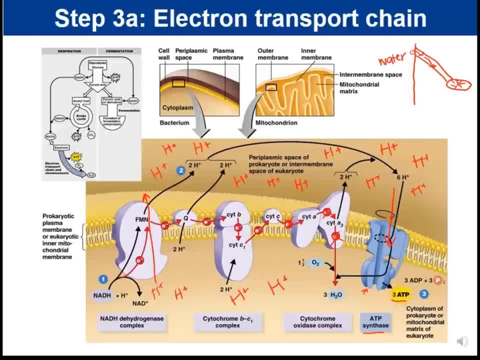 spin. So the flow of water is going to cause that turbine to spin, And when that turbine spins, that generates electricity. So that's how electricity can be generated. right, We're using water, the movement of water, to cause the turbine to spin. 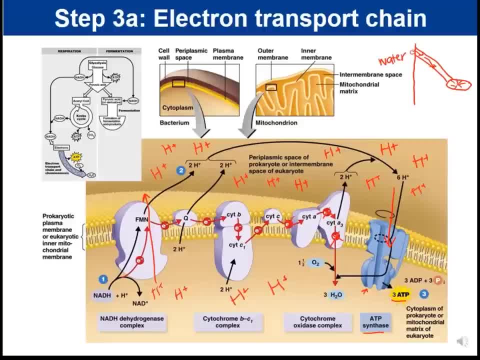 If you've ever seen the like windmills on the way out to Palm Springs, those are using wind energy. They're using wind to cause those turbines to spin and that is used to generate electricity. Same idea here: ATP synthase. think of like a. 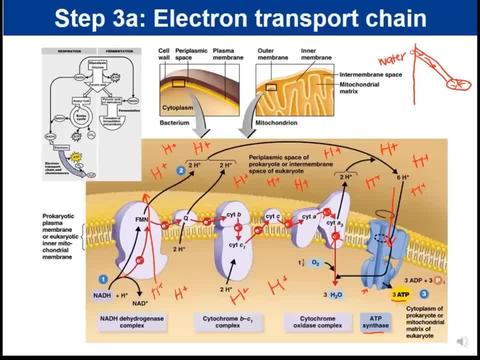 turbine. Instead of water flowing across it, though, it's the movement of hydrogens, So it's the hydrogens going from high to low that's causing this turbine to spin. And when this turbine is spinning, notice it has this arrow, like it's going in a circle. 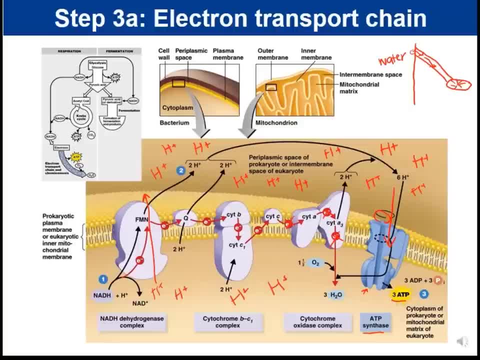 when that turbine is spinning, when that rotor is moving. that creates energy, because that is kinetic energy. It's energy of motion that causes these catalytic knobs to move, which is going. that energy is now going to be transferred to take ADP. 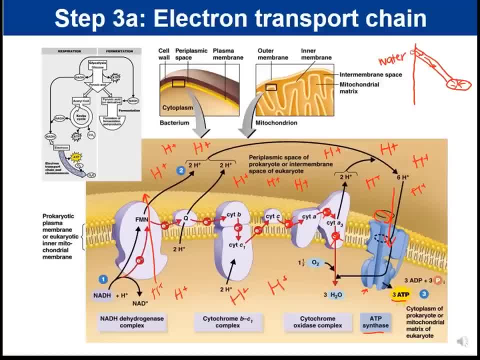 and produce ATP. So it's that energy of motion that is going to produce the ATP. And that motion comes from redox reactions. right, because the redox reactions are what are driving the hydrogen ion gradient. So the energy stored in the hydrogen 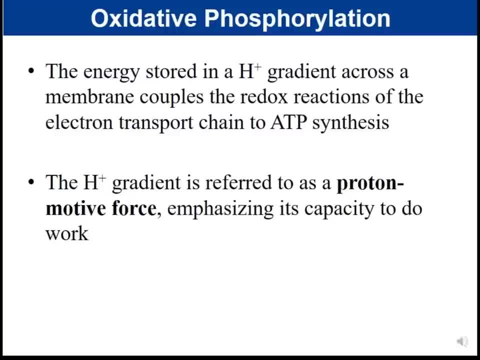 ion gradient across the membrane couples the redox reactions of the electron transport chain to ATP synthesis right, and so the these two types of reactions are coupled And the hydrogen ion gradient is referred to as proton motive force, meaning we use protons motive referring to motion. 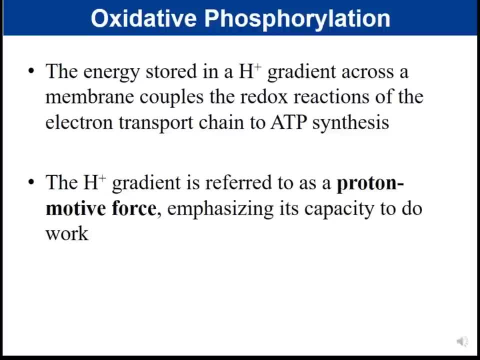 proton motive force, meaning that the hydrogen ions, that gradient and then moving from high to low, is basically going to do work, because the motion of those hydrogens going from high to low is going to cause ATP synthase to move, And so again, we call this. 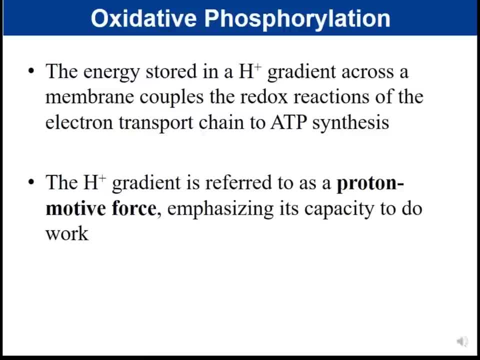 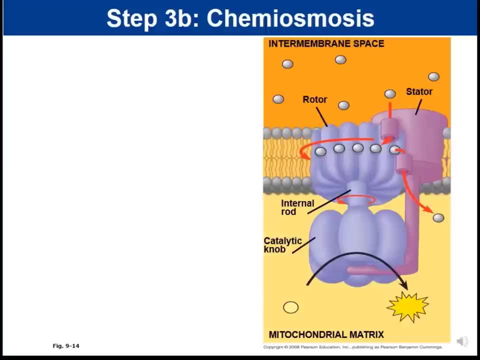 process, oxidative phosphorylation. We're using redox reactions to generate that hydrogen ion gradient and then we're going to use that hydrogen ion gradient to produce ATP. So this is just looking at more detail of ATP synthase. So this is our ATP synthase. 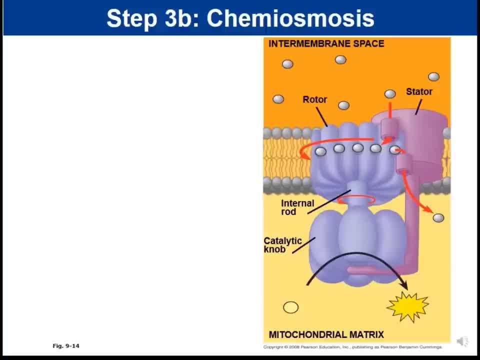 that you're looking at here. This part has a rotor, So here's the rotor, and the rotor can rotate, and so the intermembrane space has the higher hydrogen ion concentration and that's because the electron transport chain- you can think of it- being over here. 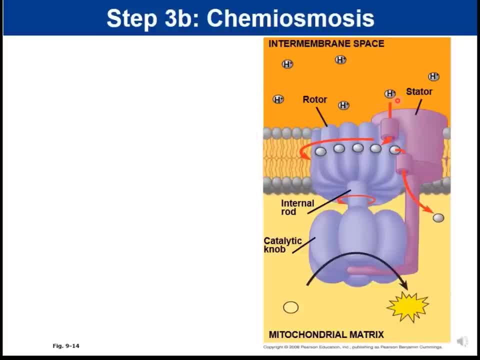 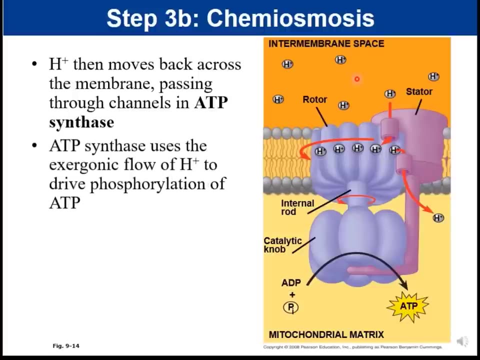 the electron transport chain is going to pump hydrogens into the intermembrane space, So we have a higher hydrogen ion concentration here and a lower concentration in the mitochondrial matrix. Let's put all this on here, So as the hydrogens move back, 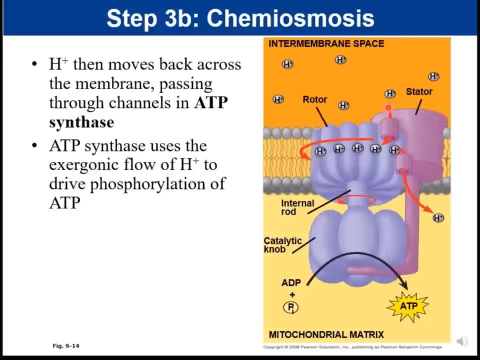 across the membrane. meaning when they go back from their high concentration to low, it's going to pass through these channels in ATP synthase And it's going to cause this rotor to move. So the hydrogens are going to go down the gradient. 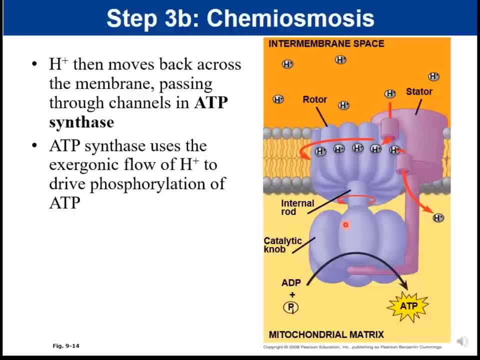 it causes this rotation of the rotor, which then is going to cause these catalytic knobs to move. They're going to move out and in, And that is going to catalyze the production of ATP. So what happens is is ATP synthase. 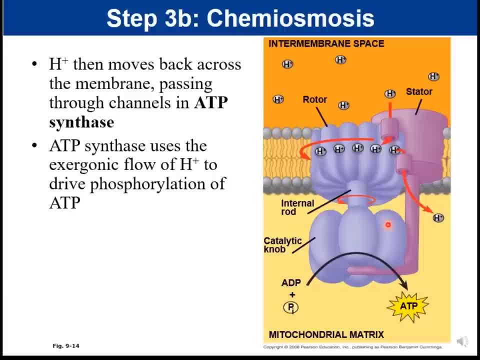 is going to use the exergonic flow of hydrogens. Exergonic meaning energy is released because going from high to low is energetically favorable. Right Things want to go from high to low, So that is exergonic, It's a favorable reaction. 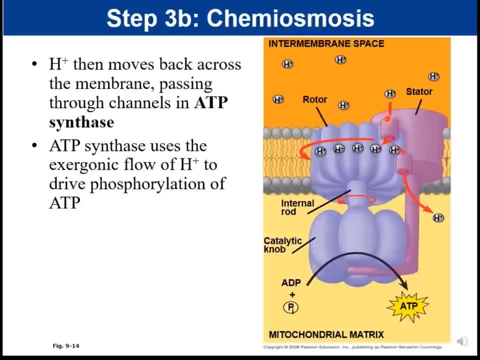 It's going to release energy. When that energy is released, that energy is transferred onto forming ATP Right, Going from ADP and inorganic phosphate to form ATP. that step is endergonic Right. It requires the input of energy to form that bond. Remember that phosphate. 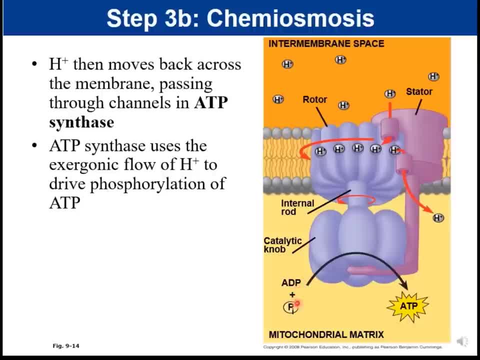 groups do not want to be together. So to add this phosphate onto adenosine diphosphate is not easy, It's not favorable, It's not something that's going to happen spontaneously, because it takes a lot of energy to link those phosphates. 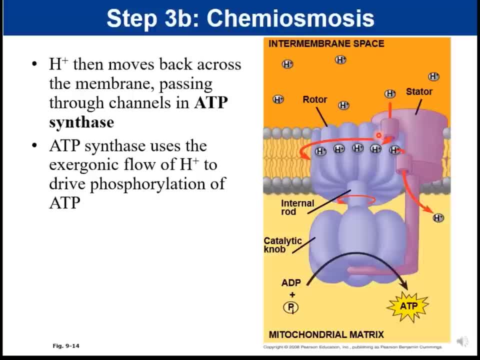 together. So again, this shows us a coupled reaction. We have an exergonic reaction: The hydrogen is flowing down the gradient, coupled to the endergonic reaction of forming ATP. So this is just another example of a coupled reaction. You have to get energy from somewhere. 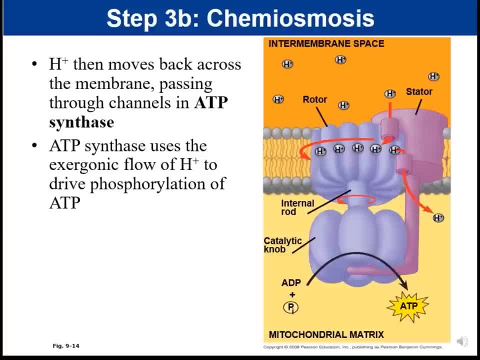 And in this case it's hydrogens going down the gradient that is providing the energy to make the ATP, And so this is an example of what we call chemiosmosis. If you know what osmosis is, it's the movement of water. 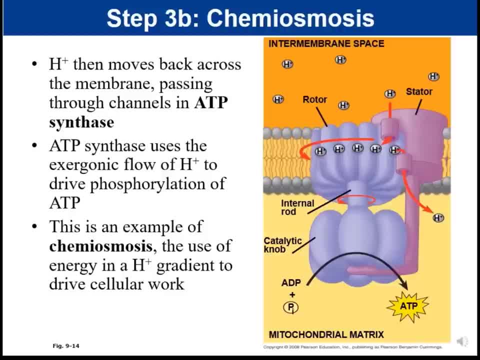 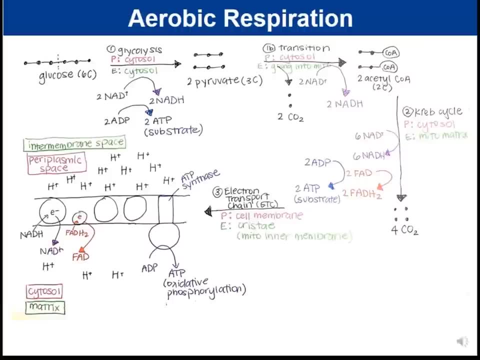 In this case it's chemiosmosis. So we're using chemicals. hydrogen ions: We're using the energy and hydrogen ion gradients to drive cellular work. We're using that gradient to produce our ATP. So let's continue on with our diagram. 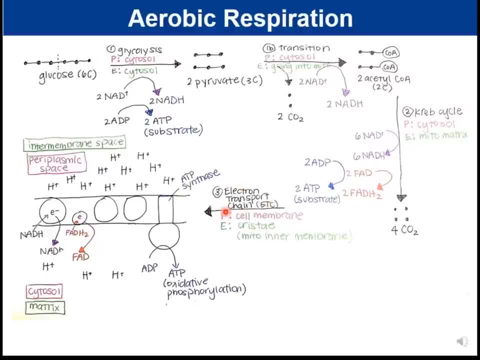 So step number three: we have on here our electron transport chain. Here's my electron transport chain In prokaryotic cells. remember that this is going to be the cell membrane In eukaryotic cells. this is the cristae. 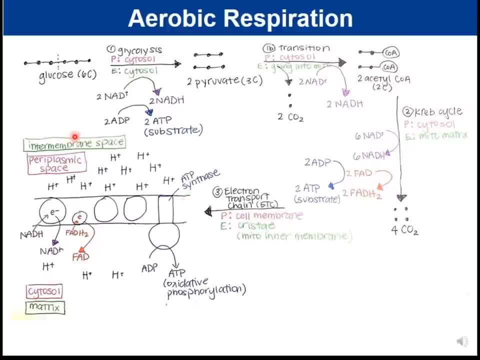 which again is the mitochondrial inner membrane. I went ahead and I labeled both of these spaces depending on if it's prokaryotic or eukaryotic. Prokaryotic: I kept pink, So this would represent the space out. here is the periplasmic. 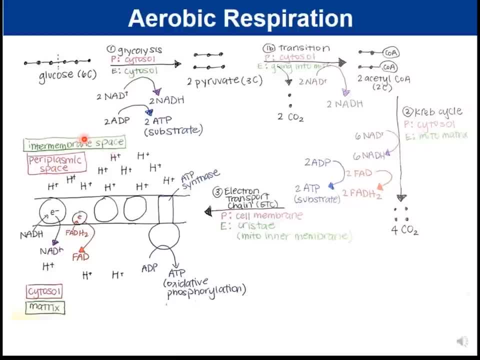 space in prokaryotic Or in eukaryotic cells it's the intermembrane space, the space between the inner and the outer membrane, This space in here that is the cytosol or the cytoplasm in prokaryotic. 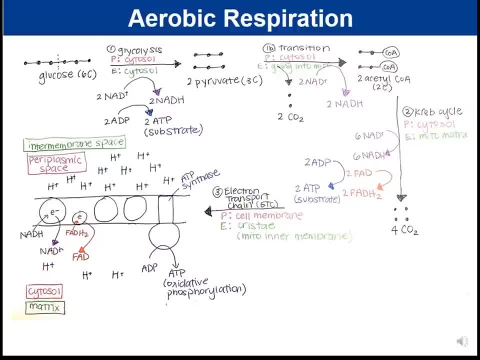 cells, But in eukaryotic cells it's the mitochondrial matrix, meaning the innermost part of the mitochondria. What is going to happen in the electron transport chain? Again, I'm going to draw this on here. NADH is going. 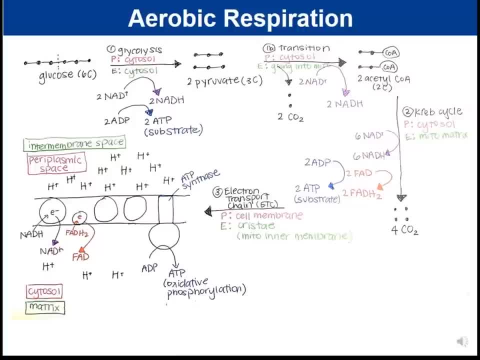 to drop off electrons at the electron transport chain. Again, when it drops it off, NADH becomes oxidized, it loses its electron and we're going to get NAD+. We have our NAD+, but the electron is going to move. 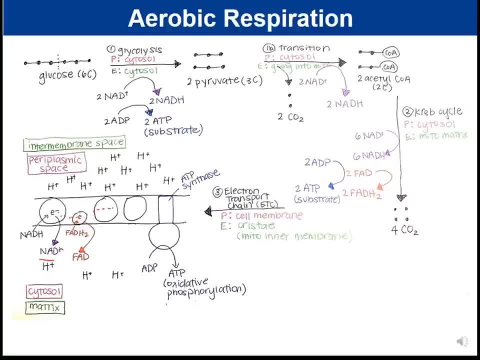 down the chain FADH2, remember that was the other electron carrier that was generated during the Krebs cycle. FADH2 will also come in and drop off electrons at the electron transport chain and when it drops off electrons it becomes FAD. 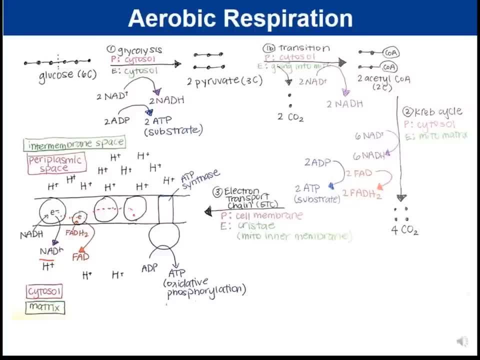 So electrons go down the chain. What is going to take the electrons from the electron transport chain? if this is aerobic respiration, What is going to remove the electrons? Oxygen O2 is our final electron acceptor. It's going to take. 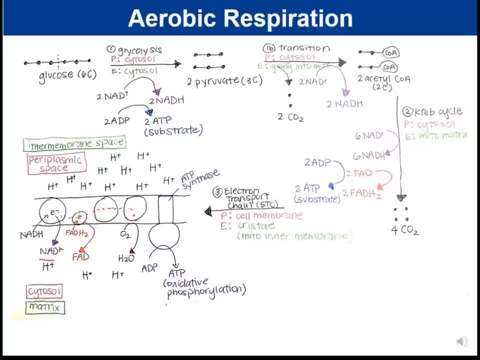 the electrons, it's going to become reduced and it forms water. You don't need to worry about balancing that equation. I don't care. I just want you to know that O2 is the final electron acceptor, and when it does. 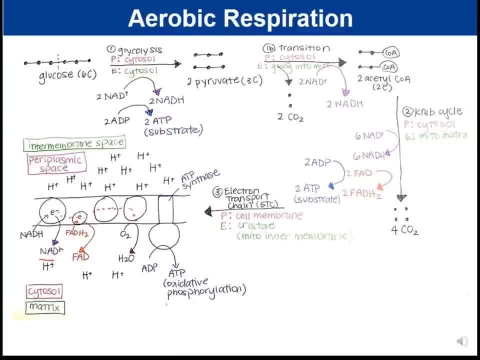 that it's going to form water. So there's our water. Now, as the electrons go down the chain, they're used to pump hydrogens against the gradient. So we're going to pump hydrogens from the low concentration to the high concentration. 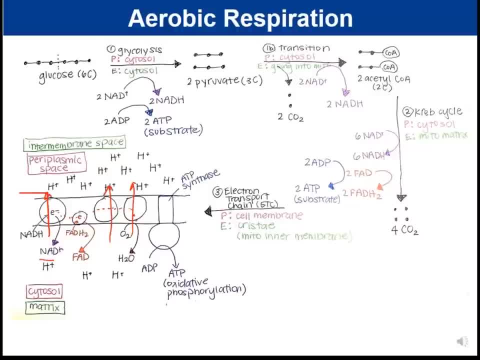 So we're going to pump these hydrogens, And so the hydrogens will go against the gradient. we're going to make an even higher hydrogen ion concentration in the intermembrane space or the periplasmic space, depending on which cell type. 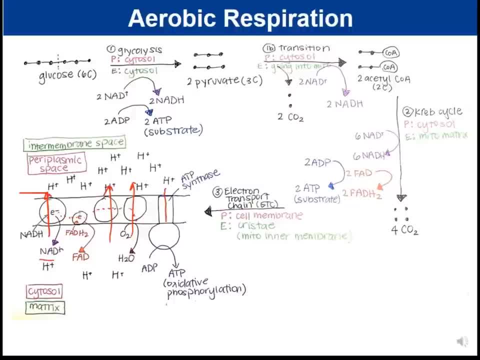 you're talking about. Then hydrogens go back down the gradient, They go from high to low And that process across ATP synthase. that is energetically favorable. right, Going from high to low is favorable And it's the flow of the hydrogen. 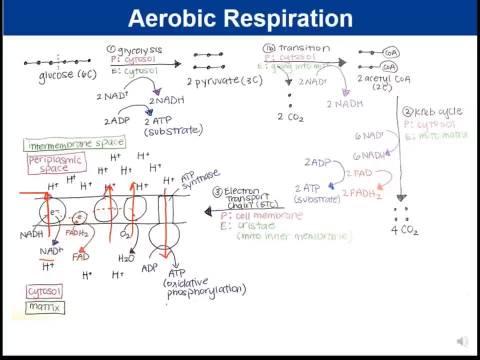 ions down the gradient that causes ATP synthase to move, which is going to generate ATP by oxidative phosphorylation. In terms of the number of ATP, remember that from this step we get about 26 to 28 ATP, So that is where the bulk of the energy is. 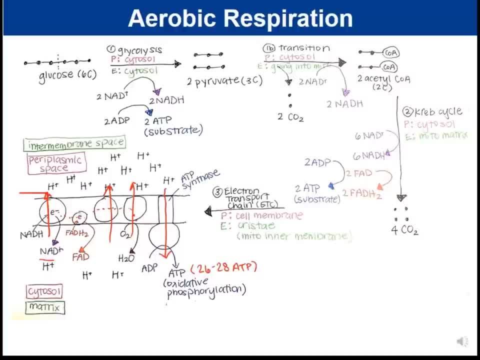 going to come from. The bulk of the energy is going to come from oxidative phosphorylation, And so, again, this is where you can see that those early steps, those early steps are important for those electron carriers, Because you need the electron carriers to drop off the electrons. 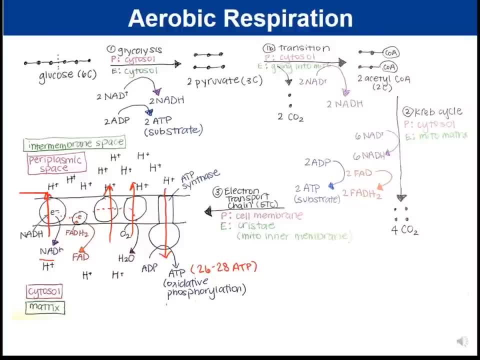 you need the electrons to move across the or down the electron transport chain, because it's the movement of the electrons that pumps hydrogens against the gradient. you need that hydrogen ion gradient in order to produce the ATP. So again, those early steps, big picture here. 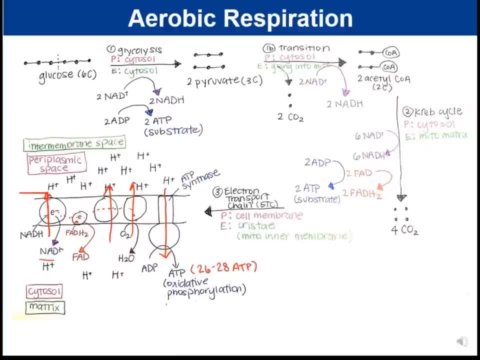 again. I want you to see the big picture. the early steps are important because they generate the electron carriers. Those electron carriers are then used in the electron transport chain And that is where the bulk of the ATP is going to come from. So again, when you study, 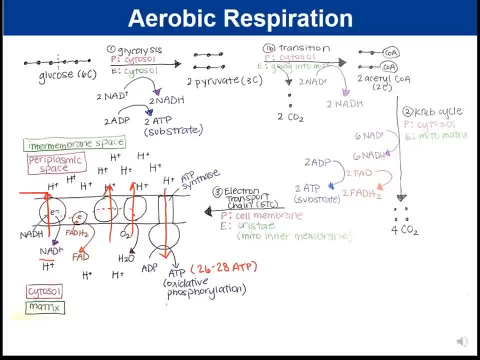 this: you want to study for each step what goes in, what comes out, and I would recommend just to practice studying, just keep drawing this out, Keep trying to draw this out by memory. If you can draw this out by memory, you can answer any. 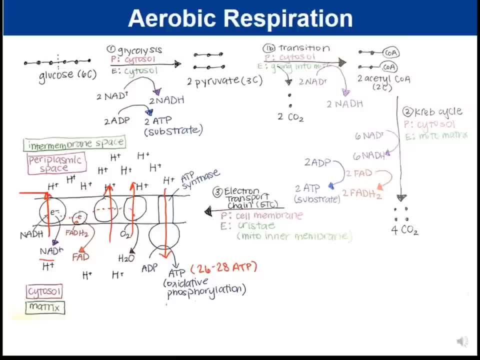 question that I have related to this, Because that means that you understand the process, And that's what I want you to take away from this. I want you to walk away with an understanding of why does it work this way. What is the point of all this? 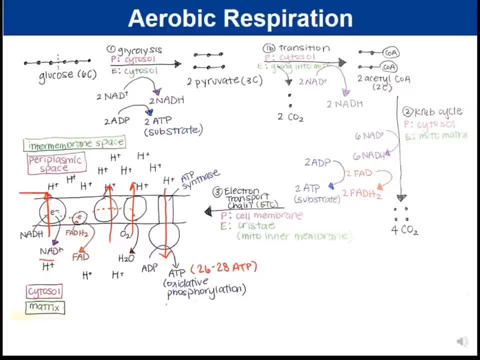 Right, And the point of all this is to break down the food little by little, and when we do that we release electrons and they get put on the electron carriers. Electron carriers go to the electron transport chain that's going to produce the bulk. 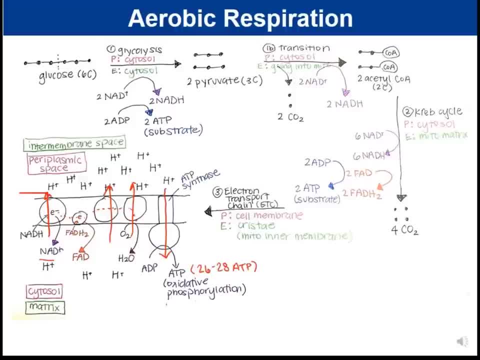 of the ATP. So that's the point of this. right Now, when we talk about aerobic respiration, notice that we have glucose. Is glucose or sugar the only food source that we use? The answer is no, Right, Glucose is. 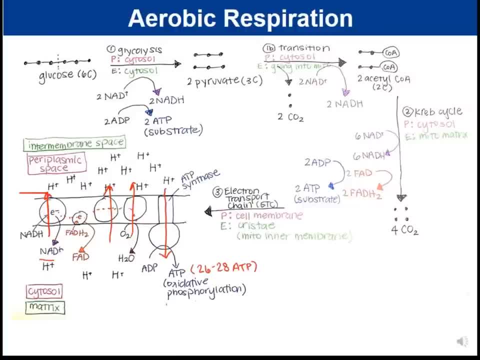 one food source right. We can use lipids, we can use fats, we could use proteins. Those other types of macromolecules can get converted into different components that can come in at different points in this pathway. So what you need to realize is that while we 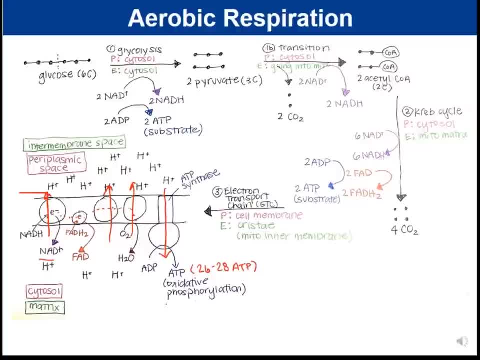 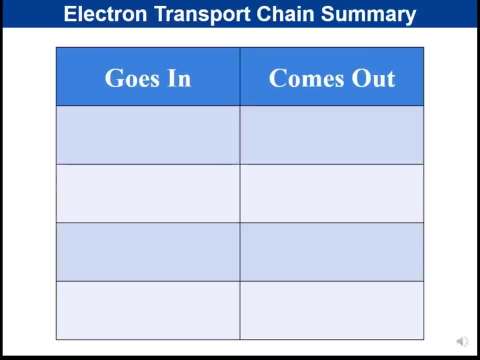 draw this with aerobic respiration using glucose. glucose is not the only food source. Other types of food that we eat can also help drive this process. It just does it in a slightly different manner. So let's summarize what goes in and what comes out. 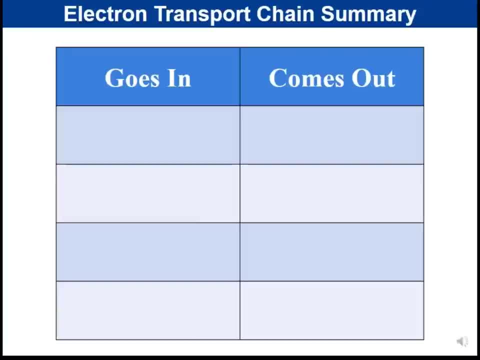 during the electron transport chain. So what goes in NADH? Right, It's going to drop off electrons at the electron transport chain. What is going to come out? NAD+? We have our other electron carrier, FADH2. 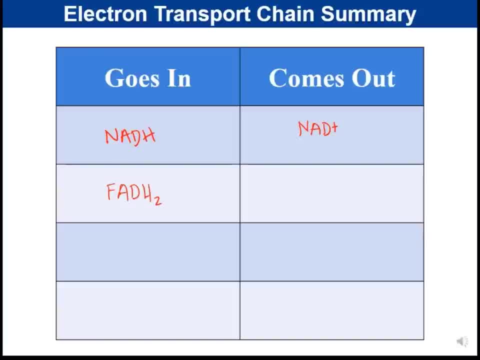 comes in. FAD is what comes out. It's not plus in this case, it's just FAD. It's what comes out, Because, again, it's when the electrons get dropped off at the electron transport chain What comes out, Those empty. 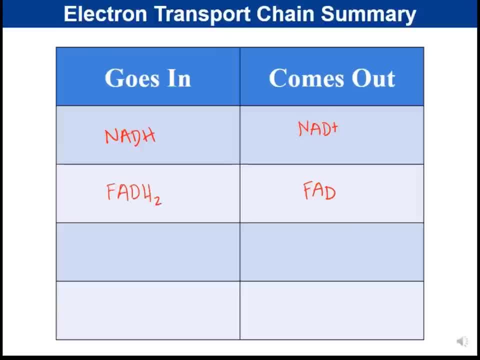 electron carriers are free to go back and pick up more electrons. What goes in? We need O2.. What comes out from the O2? Water. So when the oxygen acts as the final electron acceptor, it's going to have water being. 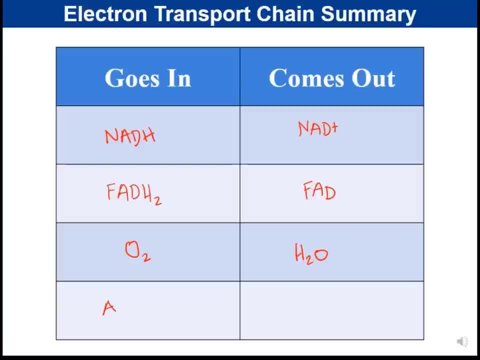 produced. And then, lastly, we have adenosine diphosphate plus inorganic phosphate, And what comes out? ATP, Adenosine triphosphate, That's our product. And so, again, this is just summarizing for the electron transport chain. 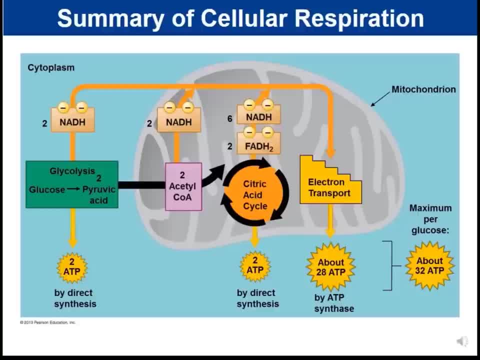 what goes in and what comes out. So this slide is summarizing cellular respiration, And so, again, the first step is going to be glycolysis. Glyco refers to sugar. Lysis is breaking, So we take that six carbon sugar and we chop it in half. 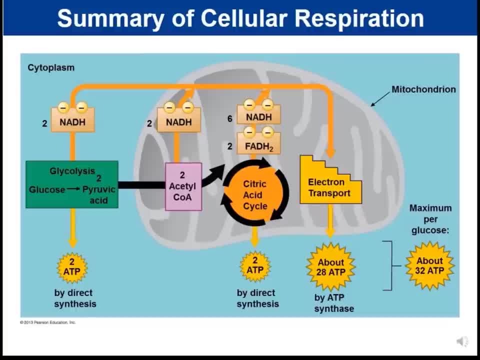 to two, three carbon pyruvates. Now when we break these bonds, we transfer electrons onto electron carriers, So during this process we also get two NADH. So here are our two NADH. We get two ATP And the ATP. 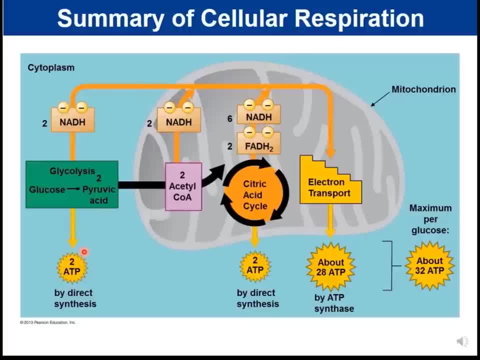 produced during glycolysis is by substrate level phosphorylation. We simply take a substrate that has a phosphate and we transfer it onto ADP, forming ADP. Those two pyruvates or pyruvic acids will go into the mitochondria and they will go. 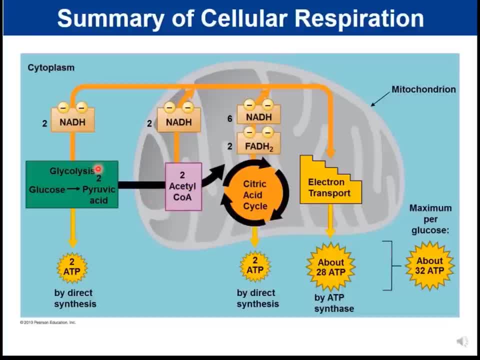 through a transition step, And so during that transition step for those three carbon pyruvates, they're going to break off one carbon. So you end up at this transition step with two CO2s And to the remaining two carbon fragment. 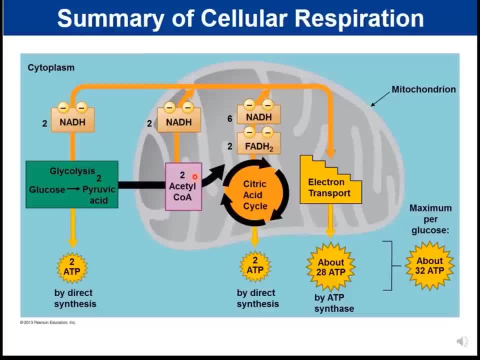 you're going to add a CoA on And your product is going to be acetyl CoA- Two of them. Now, again, we're breaking some bonds, so we get some electron carriers. So during this process, we also get two NADH. 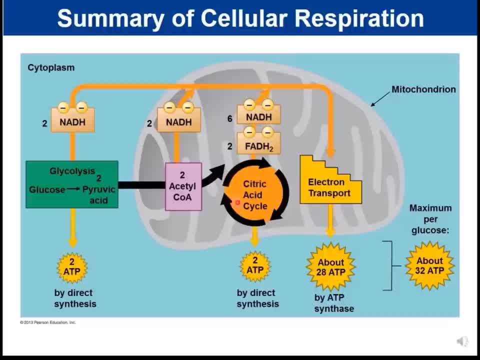 Acetyl CoA is going to go into the Krebs cycle, which is also known as the citric acid cycle, And during this process we're going to break down the acetyl CoA completely, And what we get out is we get four. 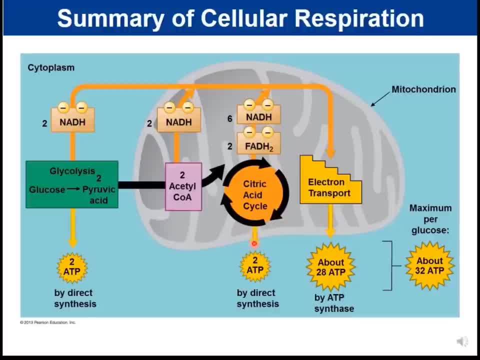 carbon dioxides, We also get a little bit of ATP, so we get about two ATP per glucose, And this ATP is produced by substrate level phosphorylation, just like in glycolysis: We broke a lot more bonds, So we get a lot more electron. 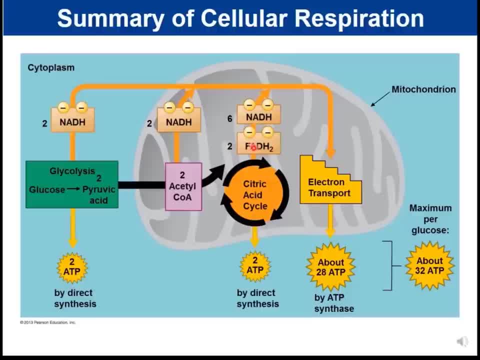 carriers. We get six NADH, We get two FADH2s, And then these electron carriers are now going to go to the electron transport chain. And so, again, just to remind you, these early steps are not so critical for the ATP, because 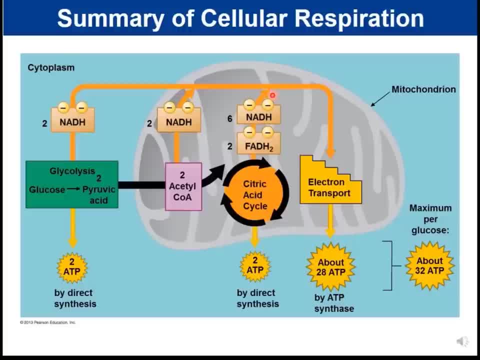 we get very little ATP during these early steps. We only get two in glycolysis, We only get two in the Krebs cycle. The important product of the earlier part of this pathway is actually going to be these electron carriers, because those electrons are energy rich And 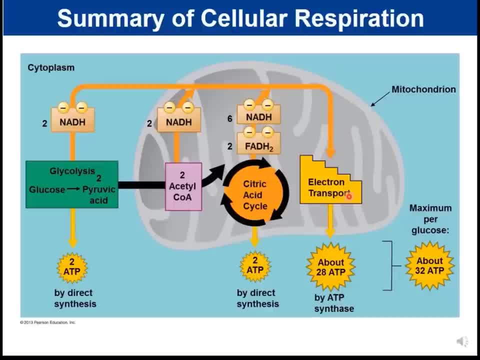 when they go and drop off electrons at the electron transport chain. so when they drop off these electrons, the electrons are going to go down the chain And as they go down the chain, that's going to be used to pump hydrogens against the gradient. 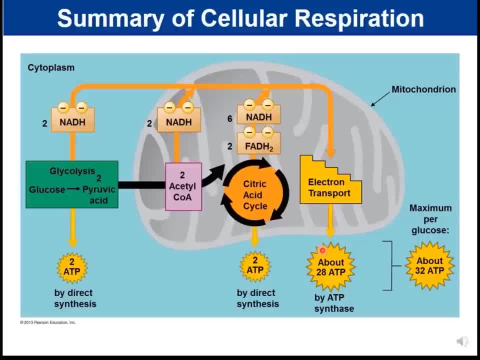 pumping hydrogens from a low concentration to high Hydrogens will go back down the gradient through ATP synthase, and that movement of hydrogens across the membrane is what's going to power the production of ATP And so during the electron transport chain. 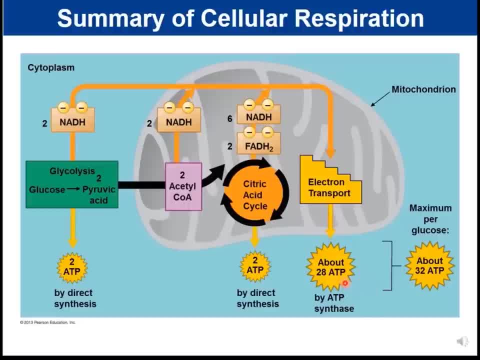 we get about 28 ATP through oxidative phosphorylation, So using those redox reactions to make ATP, And so we get about 28 ATP during this process. So, total, we get about 32 ATP. Now you might wonder, sometimes you'll see it written. 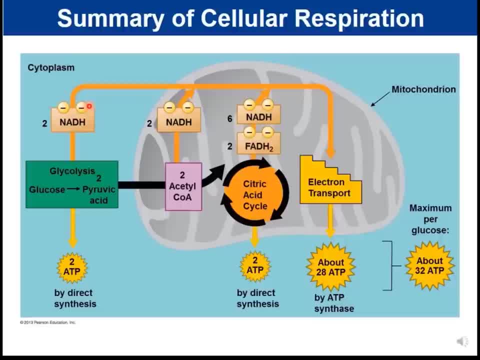 we get 30 to 32.. And you might wonder well what dictates if you get 30 or 32?? And it has to do within eukaryotic cells. So notice that in glycolysis we make these NADH out in the 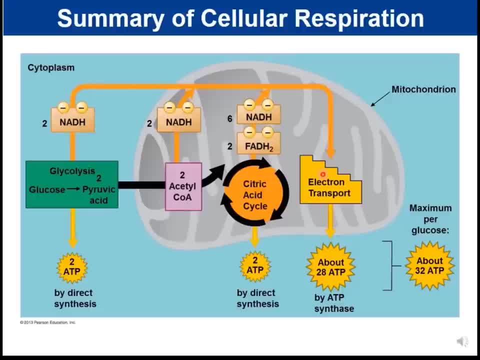 cytoplasm. The NADH needs to drop off electrons to the electron transport chain, which happens inside the mitochondria, And so what actually happens is that the electrons have to get shuttled across the membrane, So the NADH itself, 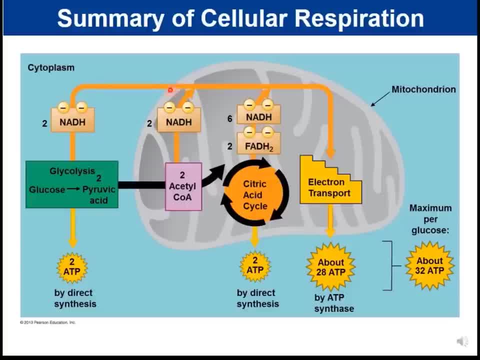 actually does not come in. Instead, it's going to have a shuttle here and those shuttles are going to transfer electrons to empty electron carriers in the mitochondria. Now, different cells in the body have different types of electron transporters. 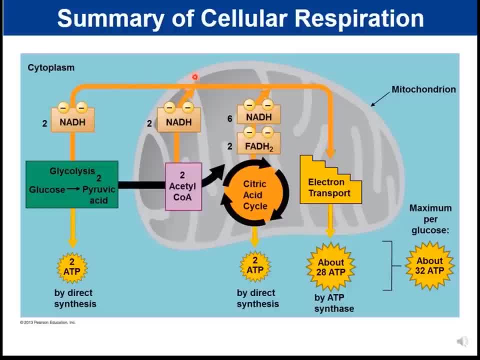 In some cells the electrons get transferred onto NAD+ and we get NADH. In other cells there is an FAD transporter, meaning that the electrons from the NADH actually get put onto FAD and form more FADH2.. 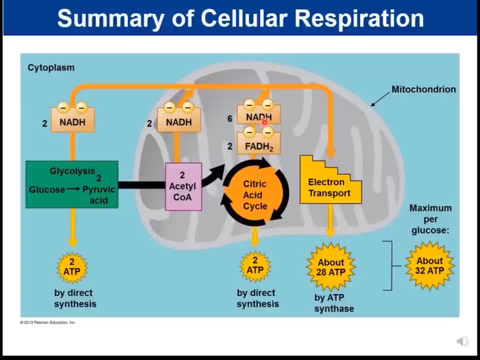 Now why does that matter? NADH comes in at complex 1.. FADH comes in at complex 2.. So when we use NADH, we get more ATP than if we use FADH2.. I won't. 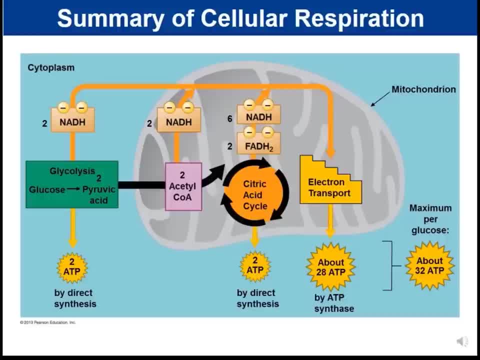 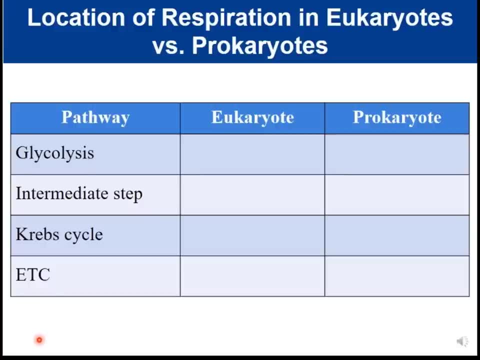 ask you that, but just in case you're wondering where that difference comes from. So now we're going to fill in and just review where these different steps take place. And so if we're talking about glycolysis in eukaryotic cells, 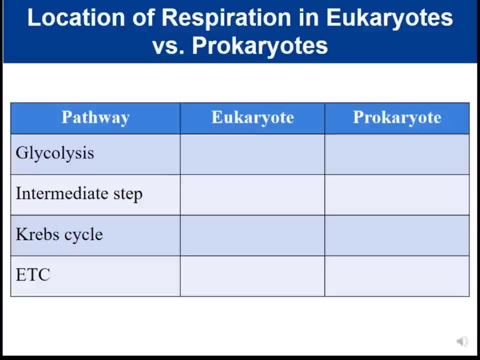 where does that take place? in eukaryotic cells? And the answer is the cytosol. In prokaryotic cells it's also the cytosol. The intermediate or transition step in eukaryotic cells is going into mitochondria. 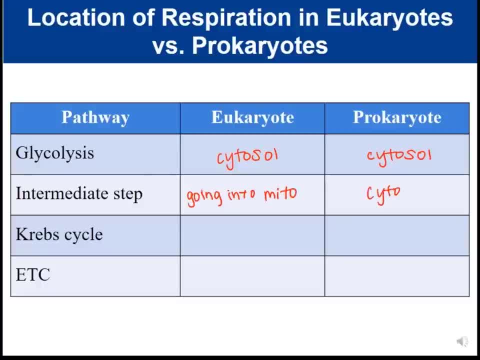 In prokaryotic cells: cytosol. The Krebs cycle: The Krebs cycle in eukaryotic cells is going to take place in the mito matrix, So the innermost part of the mitochondria In prokaryotic. 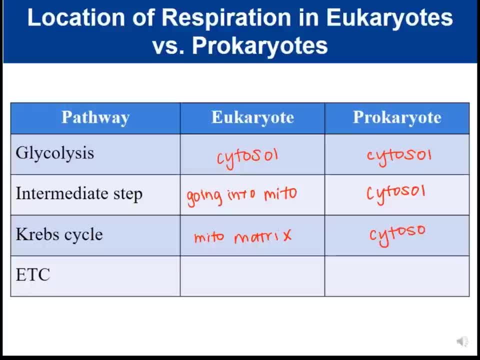 cells, it still happens in the cytosol. If we get to our electron transport chain in eukaryotic cells, this happens in the mitochondrial cristae. So again, that's the inner membrane of the mitochondria Prokaryotic. 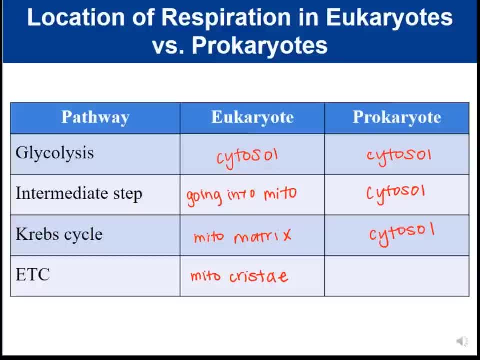 cells, however, don't have mitochondria, so they can't use that membrane. What membrane do prokaryotic cells use to do their electron transport chain? And the answer is they use their cell membrane. And so back when we talked about different structures within the 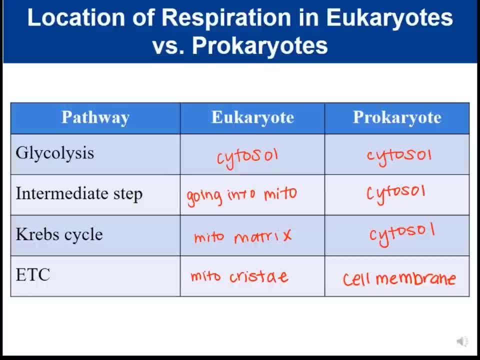 cell. you might recall that when we talked about the cell membrane, we said that in prokaryotic cells, one of the functions of the cell membrane is that it's used to produce ATP, And so that is true in prokaryotic cells. In prokaryotic cells. 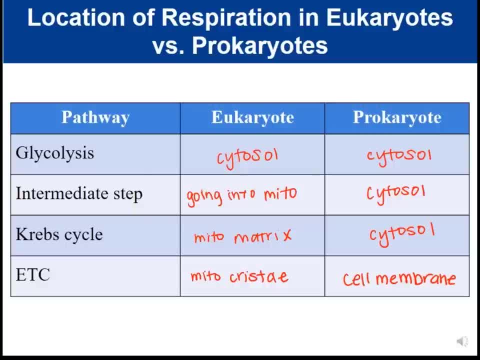 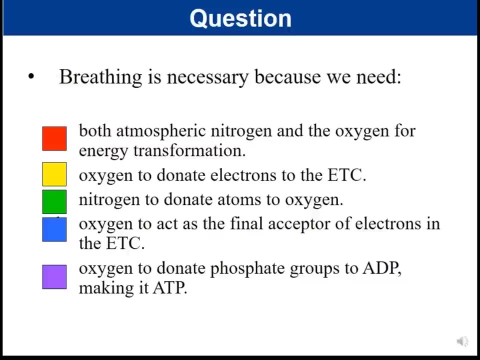 the cell membrane is used to make ATP. In eukaryotic cells this electron transport chain is going to happen in the cristae of the mitochondria. So question for you. Breathing is necessary because we need red, both atmospheric nitrogen and 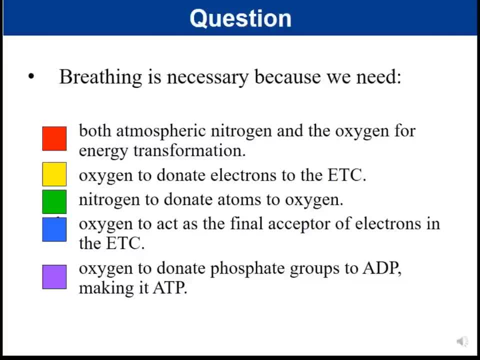 the oxygen for energy transformation: Yellow oxygen to donate electrons to the electron transport chain. Green nitrogen to donate atoms to oxygen. Blue oxygen to act as the final acceptor of electrons in the electron transport chain. Or purple oxygen to donate phosphate. 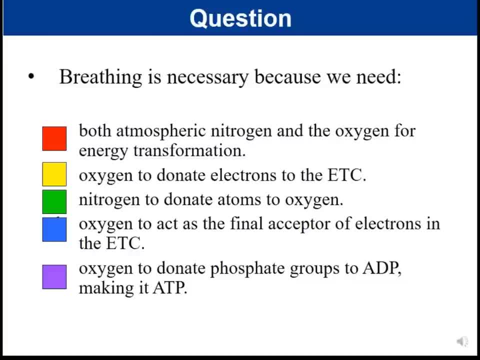 groups to ADP, making it ATP, And so, when you're ready, go ahead and pause the video and think about your answer And then, when you're ready, go ahead and push play to hear the correct answer. So if you said: 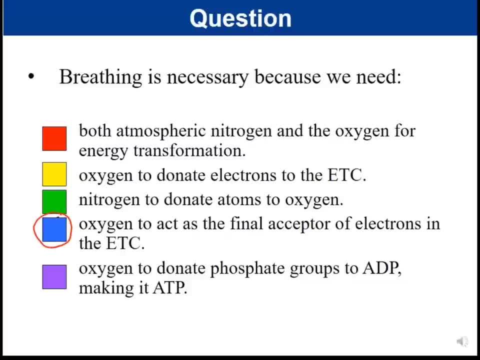 blue, you are correct. Breathing is necessary because we need oxygen to act as the final electron acceptor in the electron transport chain. That's what's going to take the electrons from the chain And that allows the electron transport chain to occur, because we need the 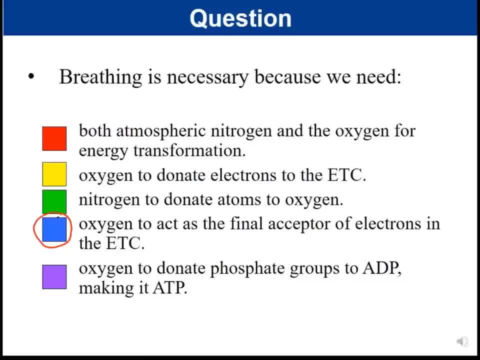 electrons to be able to move, In order to pump hydrogens against the gradient and then to make ATP. So we need to breathe because we need O2, oxygen as our final electron acceptor. It's not read: both atmospheric nitrogen and the oxygen for energy. 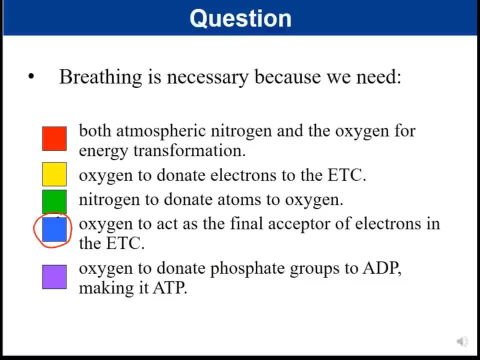 transformation. That is not true, because most organisms actually cannot use atmospheric nitrogen, which is N2 gas. There are a few exceptions. Some organisms can be nitrogen, can do a process called nitrogen fixation, But again most organisms don't utilize atmospheric 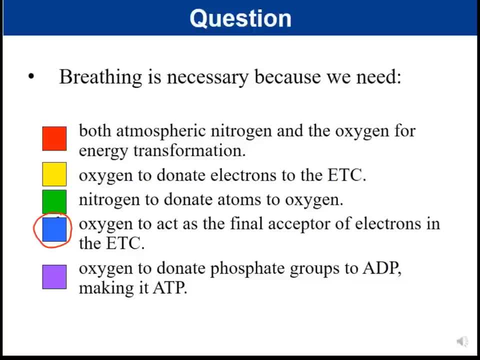 nitrogen, so that one's not true Oxygen to donate electrons to the electron transport chain? That's not true. They're not going to donate, They're going to receive. What molecule is going to donate electrons to the electron transport chain? And the answer is it's. 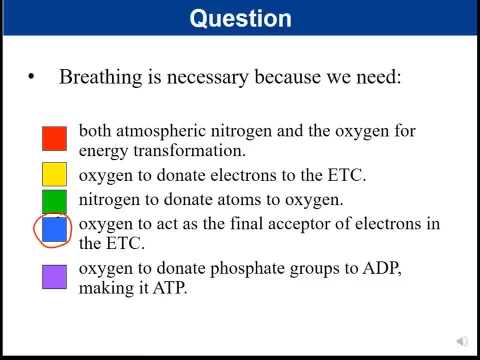 the NADH and the FADH2.. Those are what are going to drop off electrons to the electron transport chain. Where do those electrons come from? initially, They come from the food that we eat, meaning they come from when glucose becomes oxidized as 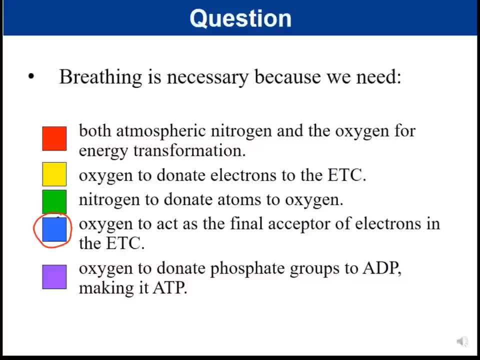 we break down the glucose, But directly they come from NADH and FADH2.. Green nitrogen to donate atoms to oxygen. That's not true, That one doesn't even make sense. Purple oxygen to donate phosphate groups to. 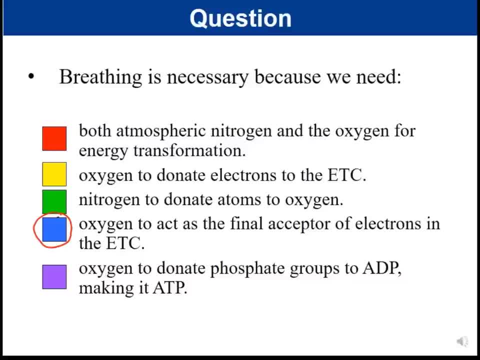 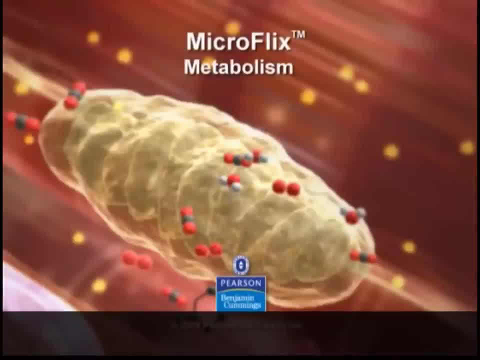 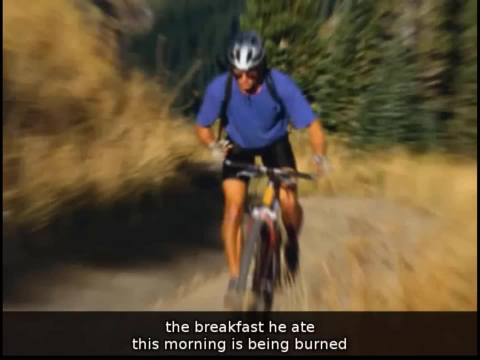 ADP, making it ATP. O2 does not have phosphate groups, therefore it can't donate them to ADP. As this mountain biker heads up the trail, the breakfast he ate this morning is being burned to power his bike ride. Let's zoom down to where. 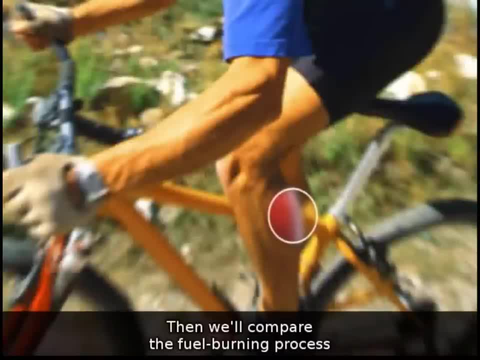 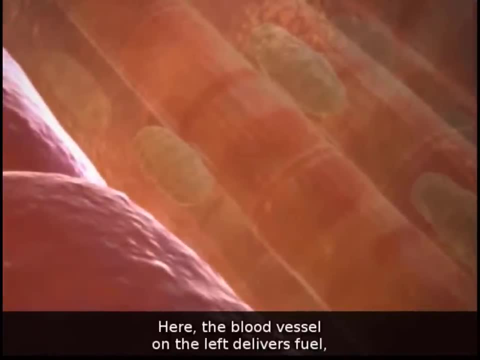 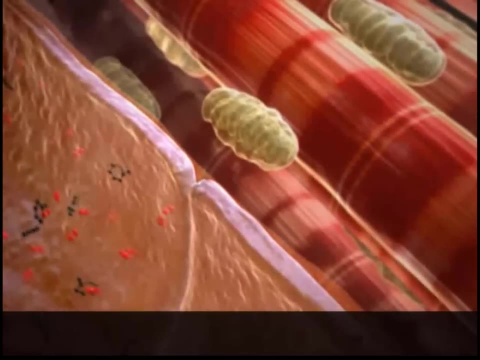 this fuel is burned his cells. Then we'll compare the fuel burning process in his muscle cells with a very similar process in bacteria. Here the blood vessel on the left delivers fuel- the black molecules- and oxygen- the red molecules- to. 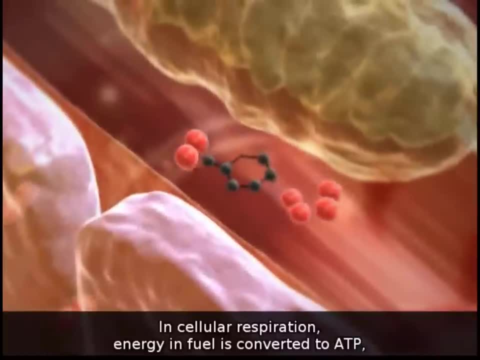 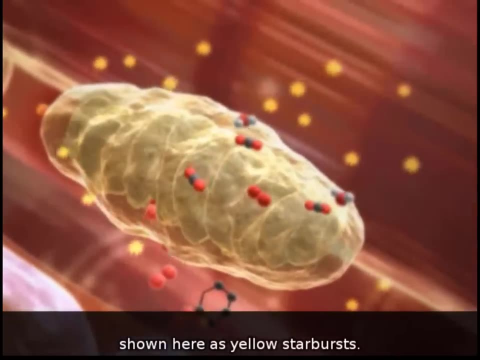 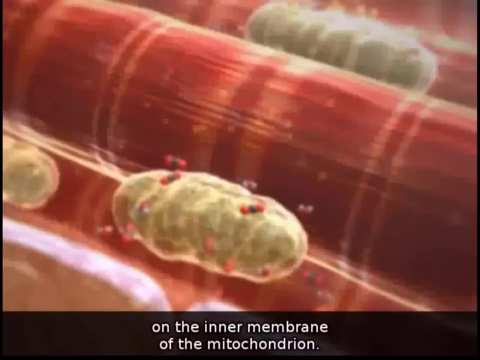 a single muscle cell shown on the right. In cellular respiration, energy in fuel is converted to ATP, shown here as yellow starbursts. Most ATP in a eukaryotic cell is made by an enzyme on the inner membrane of the mitochondria. 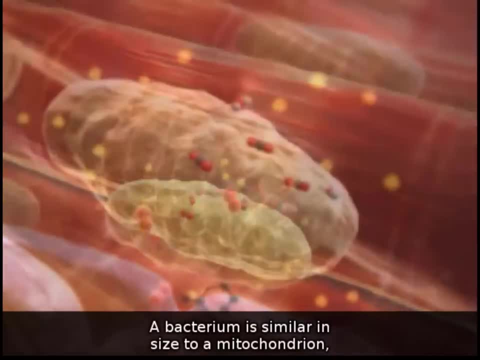 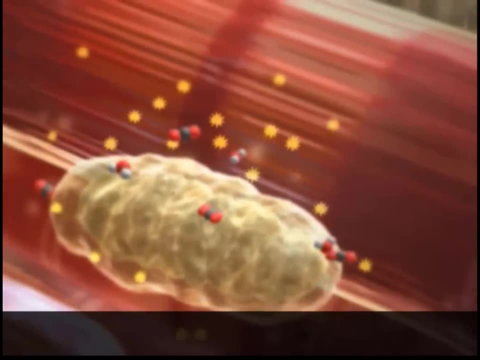 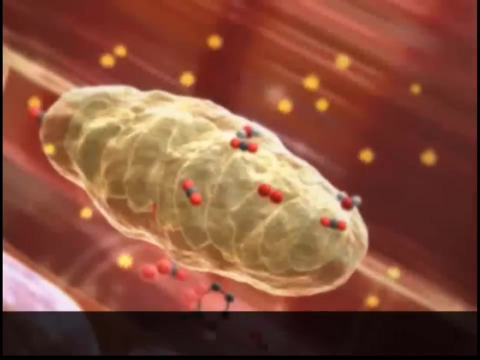 A bacterium is similar in size to a mitochondrion and its ATP is formed by an enzyme on the cytoplasmic membrane. This information supports the theory that mitochondria evolved from bacteria. ATP powers the work of the cell, such as muscle contraction. 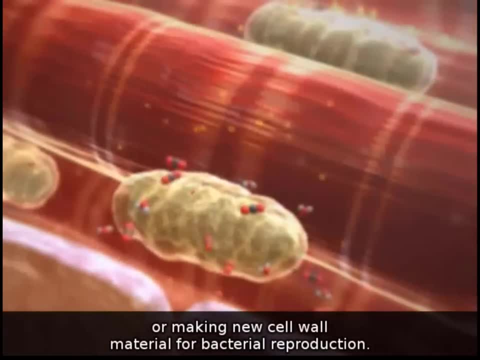 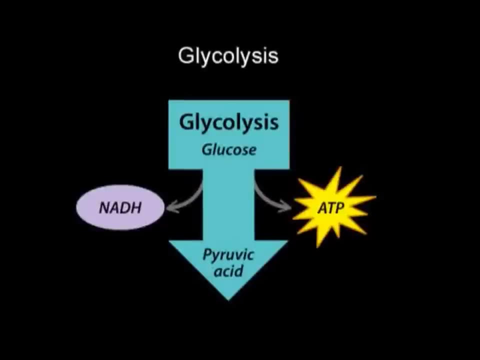 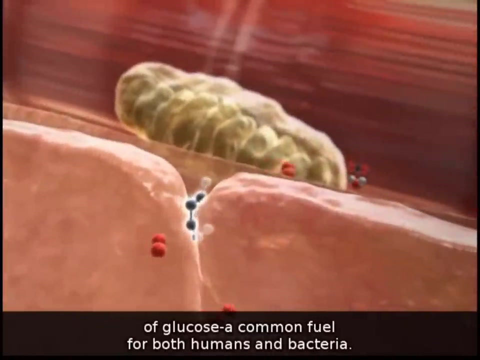 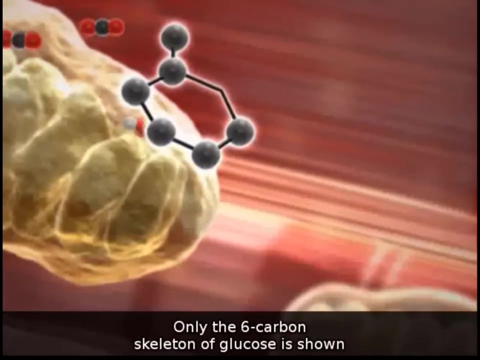 or making new cell wall material for bacterial reproduction. Let's take a closer look at how ATP is produced from a molecule of glucose, a common fuel for both humans and bacteria. Only the six-carbon skeleton of glucose is shown. to keep things simple, 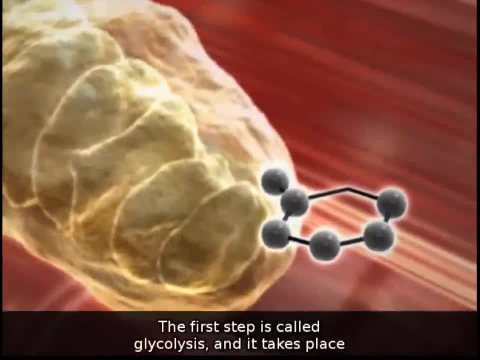 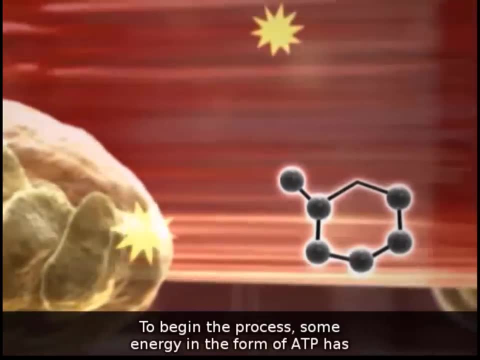 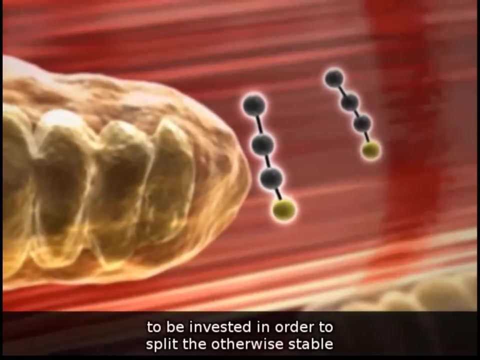 The first step is called glycolysis, and it takes place in the cytoplasm of both bacterial and eukaryotic cells. To begin the process, some energy in the form of ATP has to be invested in order to split the otherwise. 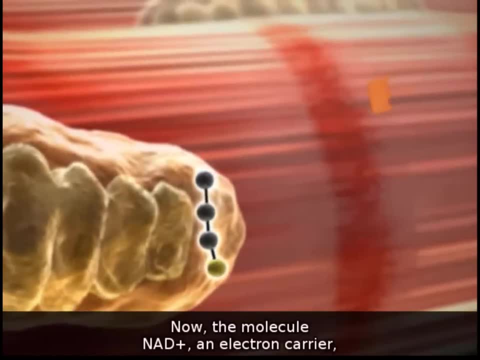 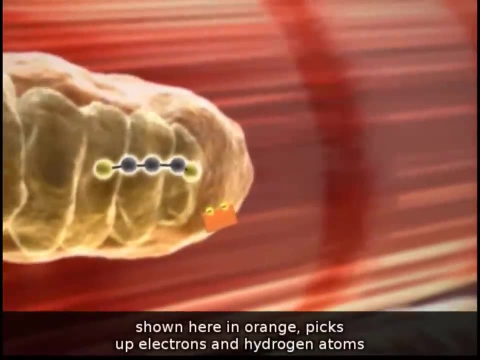 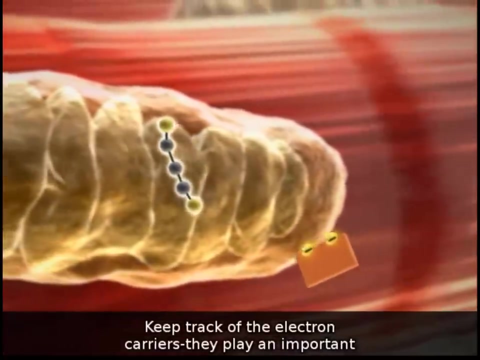 stable glucose molecule. Now the molecule NAD+, an electron carrier shown here in orange, picks up electrons and hydrogen atoms from one of the three carbon molecules becoming NADH. Keep track of the electron carriers. They play an important role by transporting electrons. 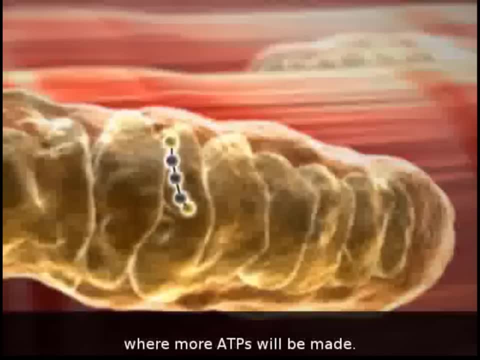 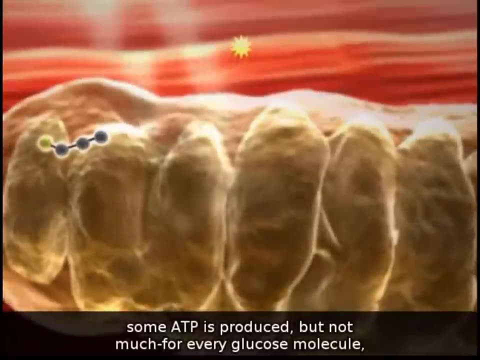 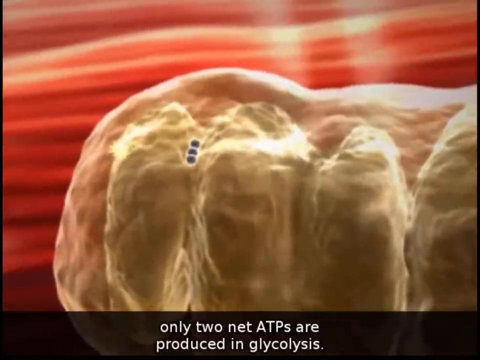 to the electron transport chain, where more ATPs will be made. In the final steps of glycolysis, some ATP is produced, but not much. For every glucose molecule. only two net ATPs are produced in glycolysis, However. glycolysis- 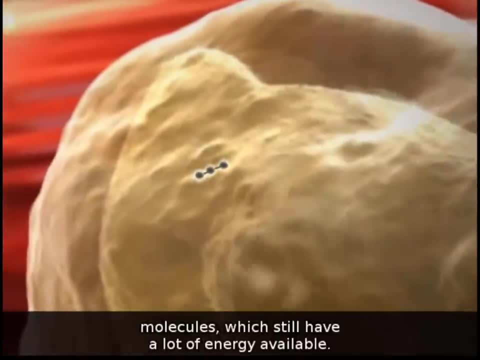 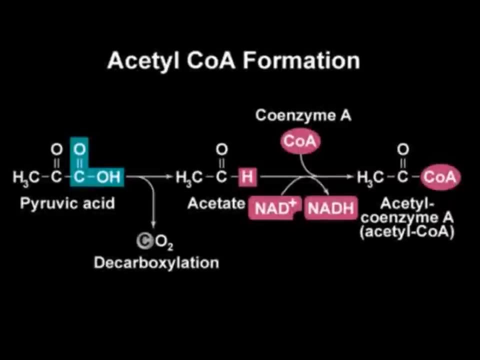 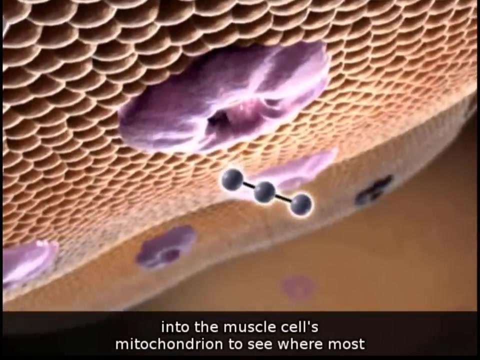 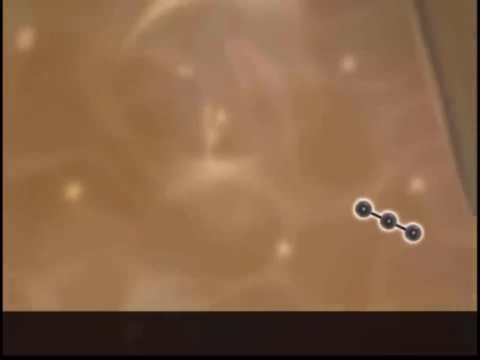 has produced two three-carbon pyruvic acid molecules which still have a lot of energy available. Let's follow one of the pyruvic acid molecules into the muscle cell's mitochondrion to see where most of the energy is extracted As the molecule enters. 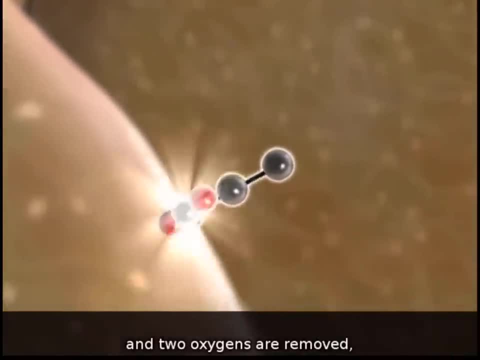 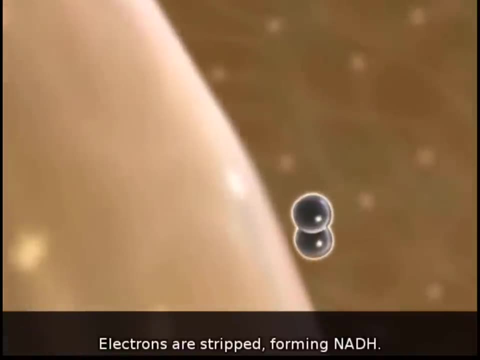 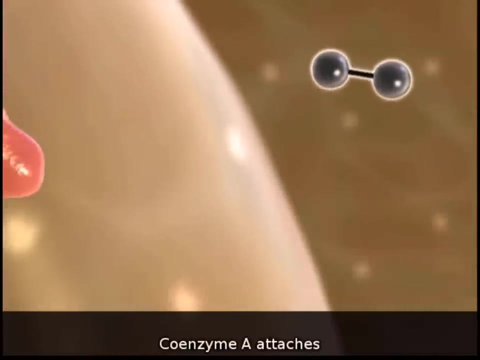 the mitochondrion, one carbon and two oxygens are removed, forming carbon dioxide. as a byproduct, Electrons are stripped, forming NADH. Coenzyme A attaches to the two-carbon fragment, forming acetyl-CoA In bacteria pyruvic acid. 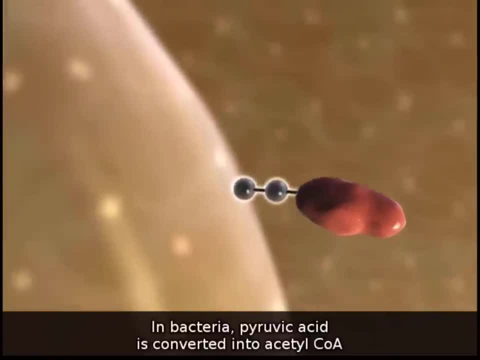 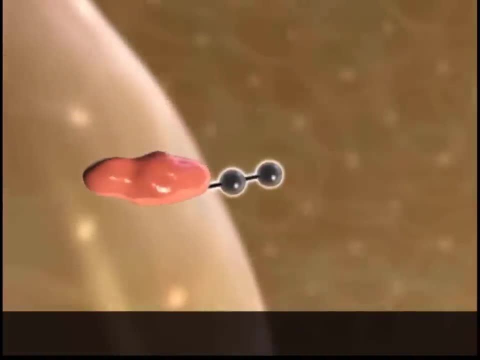 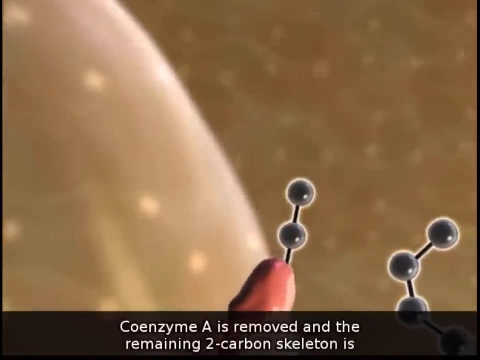 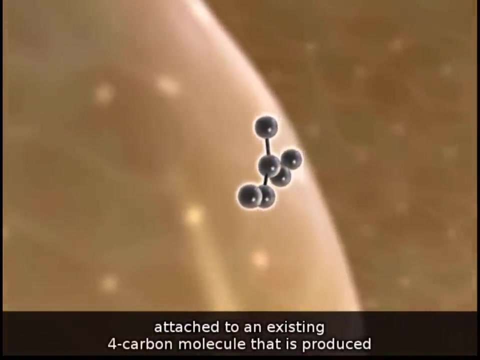 is converted into acetyl-CoA in the cytoplasm. since bacteria do not have mitochondria, Coenzyme A is removed and the remaining two-carbon skeleton is attached to an existing four-carbon molecule that is produced at the end of the last turn of the Krebs cycle. 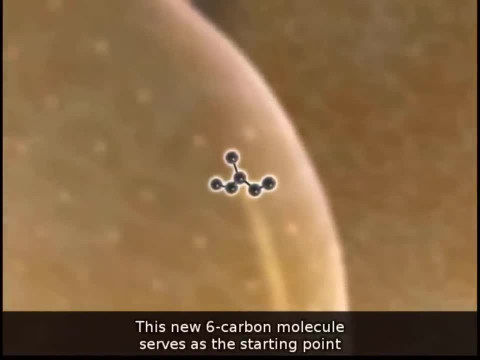 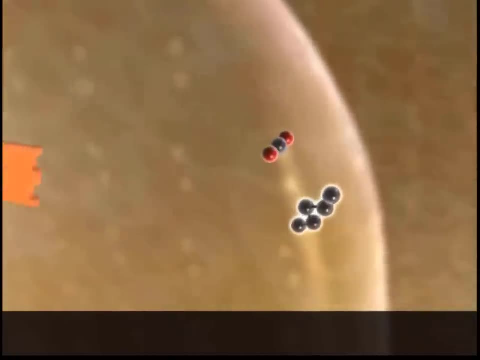 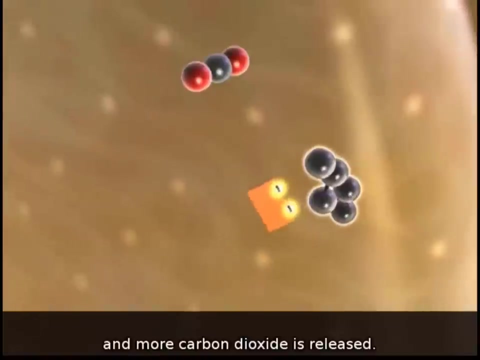 This new six-carbon molecule serves as the starting point for the next round of the Krebs cycle. The new six-carbon chain is partially broken down, releasing carbon dioxide. Several electrons are captured by electron carriers and more carbon dioxide is released In humans. 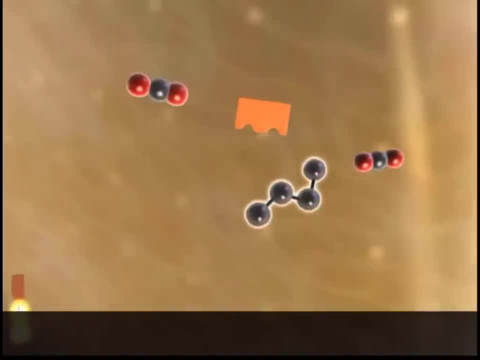 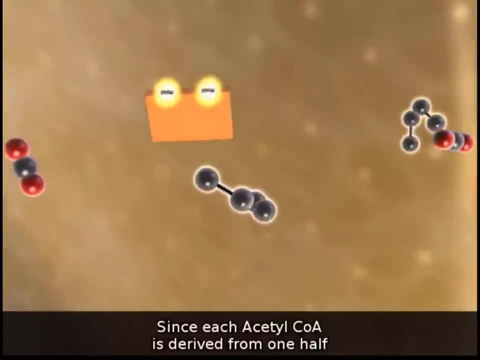 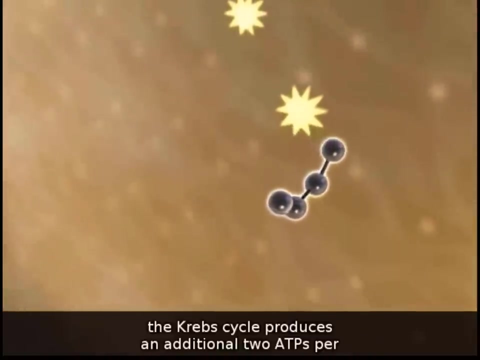 this carbon dioxide is exhaled as you breathe. Each turn of the Krebs cycle that begins with one acetyl-CoA produces one ATP. Since each acetyl-CoA is derived from one half of the original glucose molecule, the Krebs cycle produces an additional two. 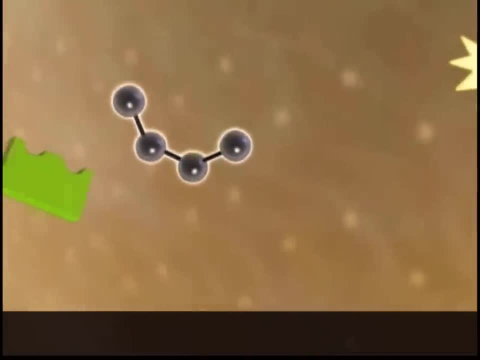 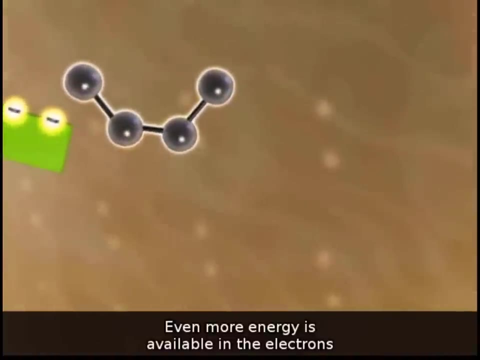 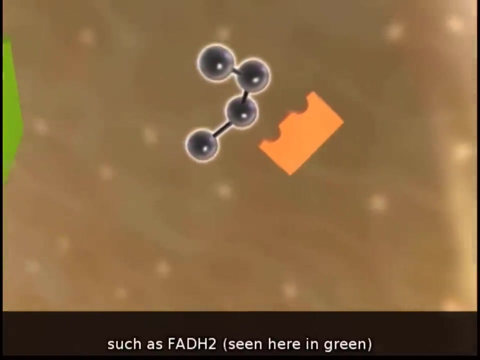 ATPs per original glucose. These ATPs are produced by substrate level phosphorylation. Even more energy is available in the electrons that are being transported by electron carriers, such as FADH2, seen here in green, and NADH, shown here in orange. 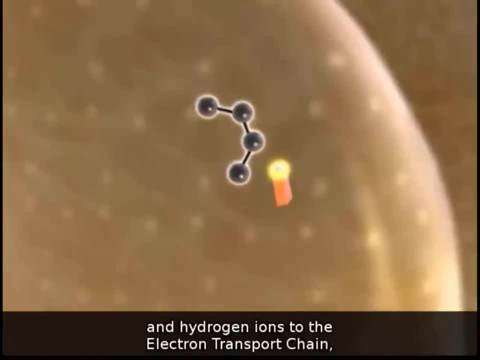 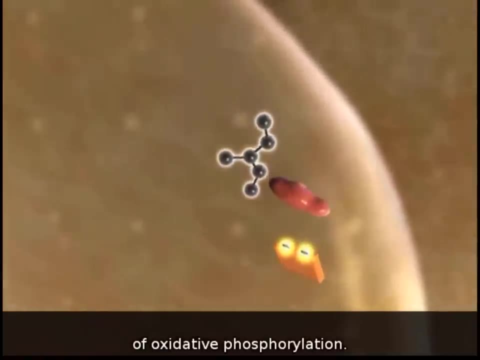 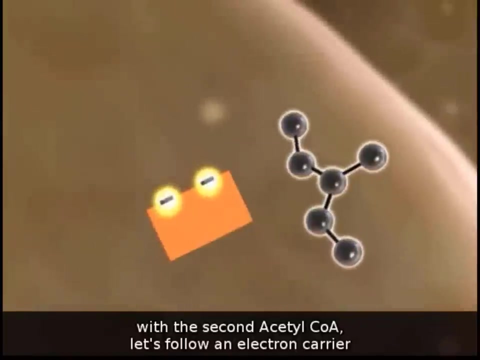 These electron carriers will take their electrons and hydrogen ions to the electron transport chain, where more ATP is made in the process of oxidative phosphorylation. While the Krebs cycle starts another round with a second acetyl-CoA, let's follow an electron carrier to the 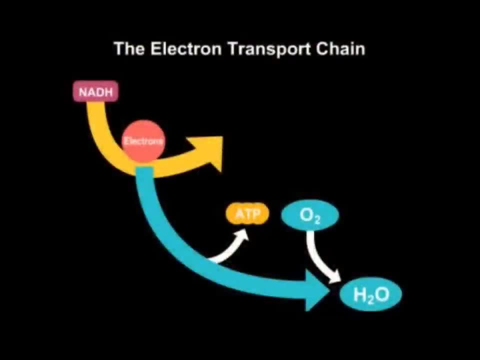 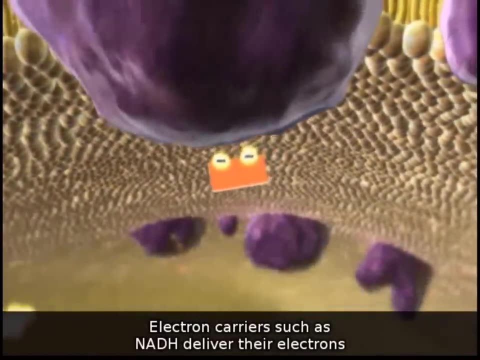 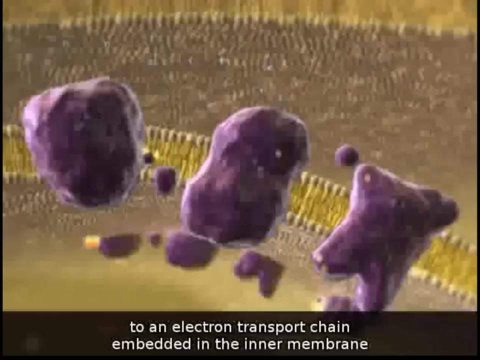 next step in the process. Electron carriers such as NADH deliver their electrons to an electron transport chain embedded in the inner membrane of the mitochondrion. in eukaryotic cells such as this muscle cell In bacteria, the electron transport chain is located. 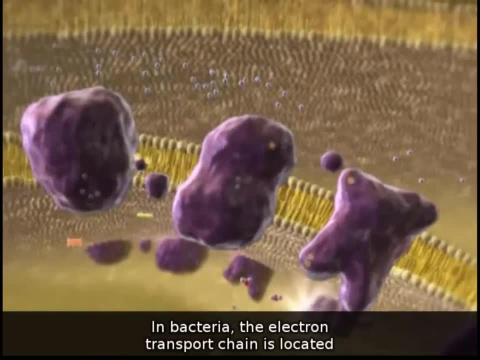 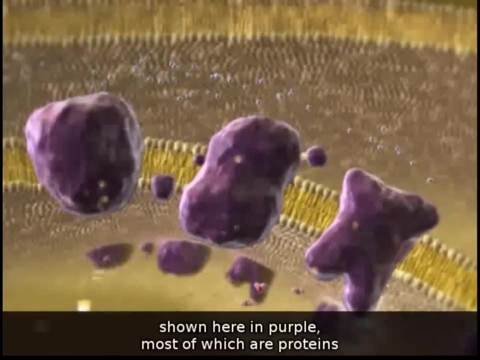 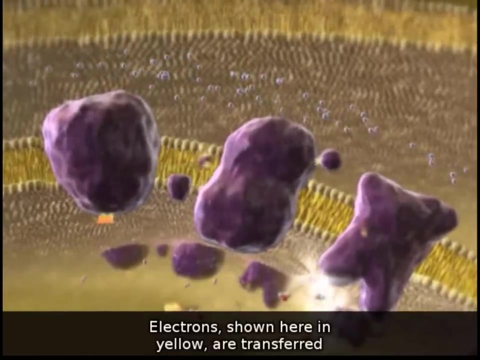 on the cytoplasmic membrane. The chain consists of a series of electron carriers that are located on the cytoplasmic membrane: Electrons shown here in purple, most of which are proteins that exist in large complexes. Electrons shown here in yellow. 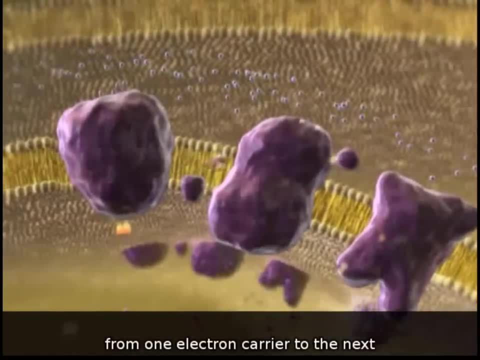 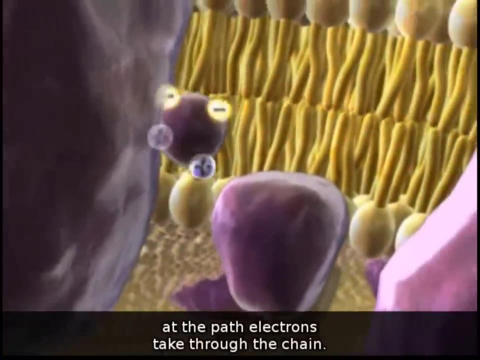 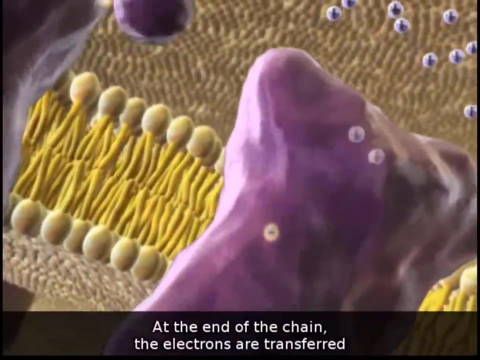 are transferred from one electron carrier to the next in the electron transport chain. Let's take a closer look at the path electrons take through the chain. As electrons move along each step of the chain, they give up a bit of energy. At the end of the chain, the electrons 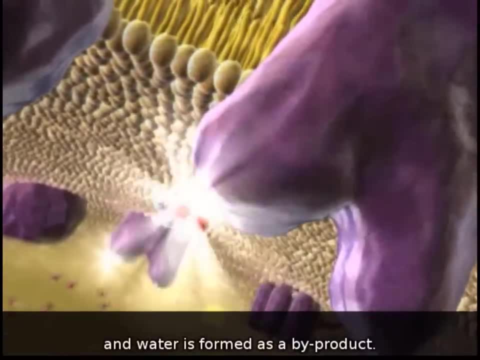 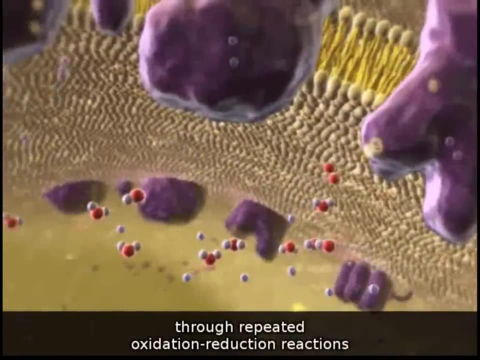 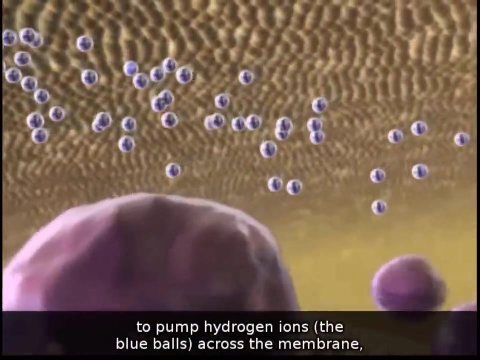 are transferred to oxygen and water is formed as a byproduct. The energy released by electrons through repeated oxidation-reduction reactions as they are passed along the chain is used to pump hydrogen ions across the membrane, creating an area of high hydrogen ion concentration. 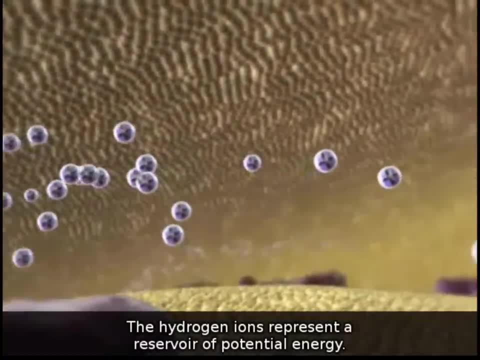 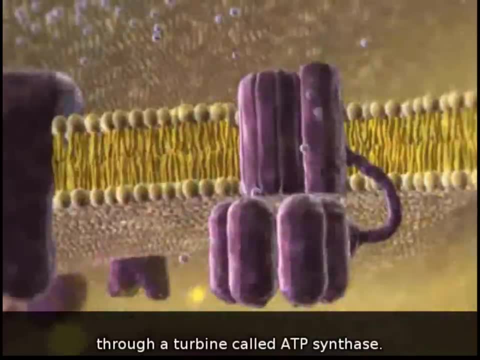 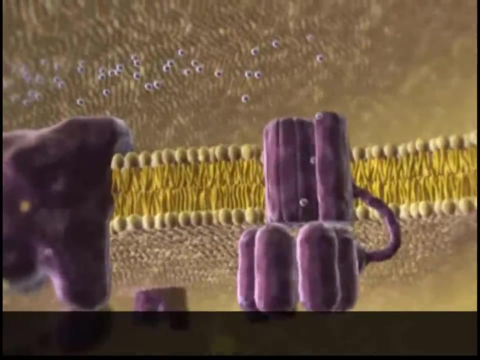 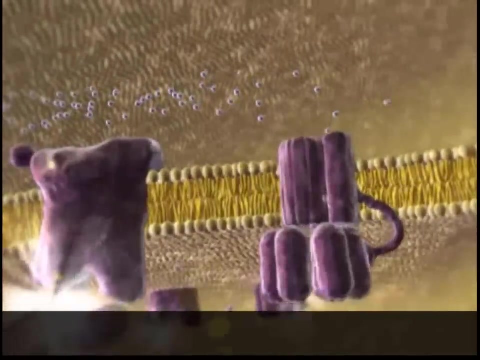 The hydrogen ions represent a reservoir of potential energy. The hydrogen ions diffuse back across the membrane through a turbine called ATP synthase. Much like water flowing through a dam, the flow of hydrogen ions spins the turbine which activates the production of ATP. These spinning turbines in cells 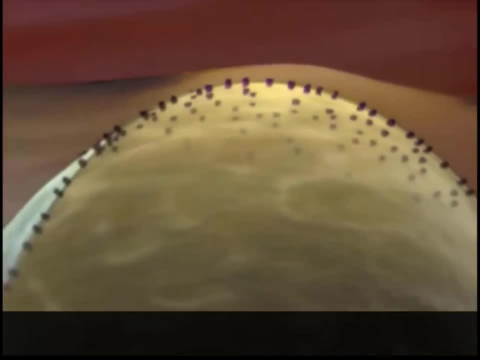 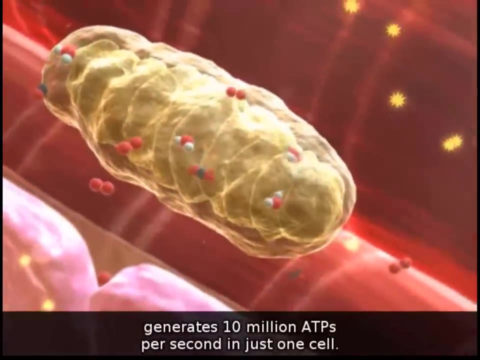 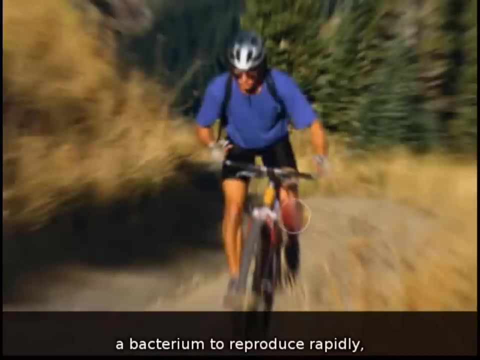 produce most of the ATP that is generated from food. The process you've just observed- cellular respiration- generates 10 million ATPs per second in just one cell. That ATP can power a biker up the trail, a bacterium, to reproduce rapidly. 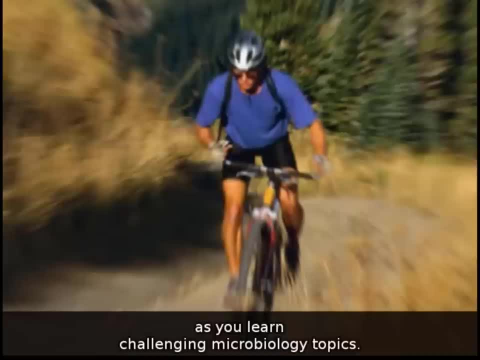 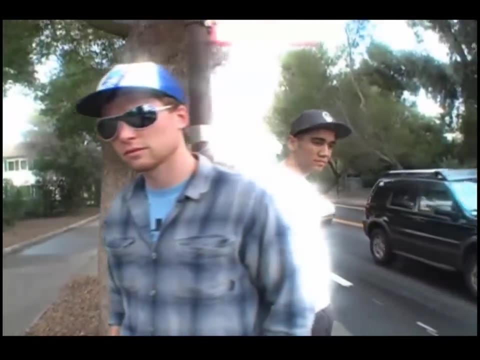 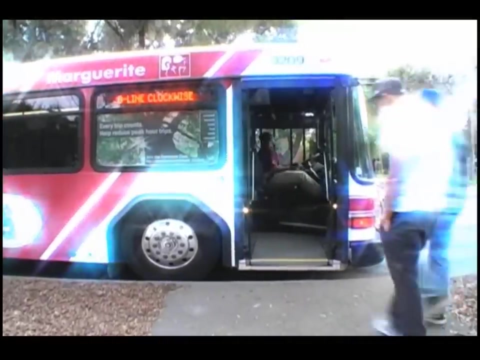 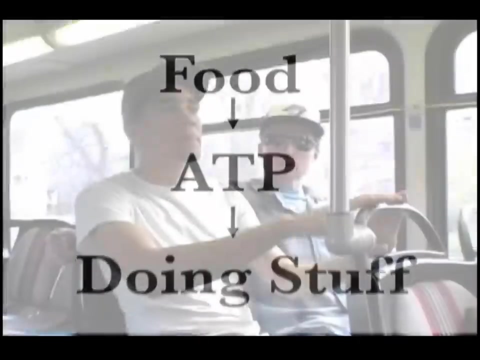 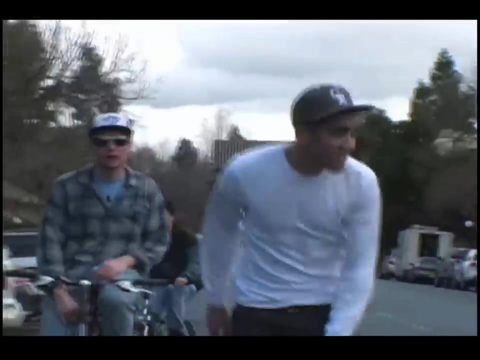 or it can power your brain cells as you learn challenging microbiology topics. I'm not trying to have me confused, but it's a simple concept. so now I'm in the mood for learning how I'm burning glucose as a Fusos. I wanna live good. so my cells take energy from the bonds in the sugar, put them into ATP. Takes ten enzymes, takes ten steps. wind up with two pyruvates- yeah, still got energy left. So mitochondria can take them to burn and down to acetyl-CoA. 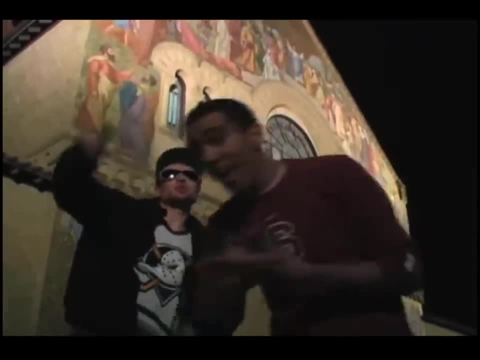 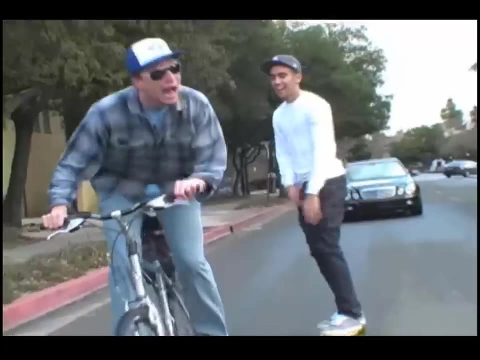 and study me. I make ATP and I'ma be on your test, so you should get to know me. And if you got enough oxygen in stock, Krebs gon' psych my homie until your heart stops. Go and study me. I help make ATP by making NADH, so you should get to know me. In the membrane of the mitochondrion, using NADH from Krebs to pump protons based to electrons, I'ma make ATP. So you should get to know me. 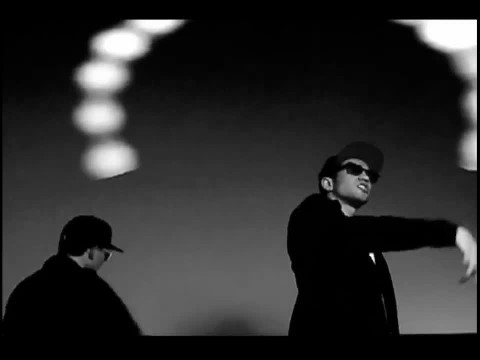 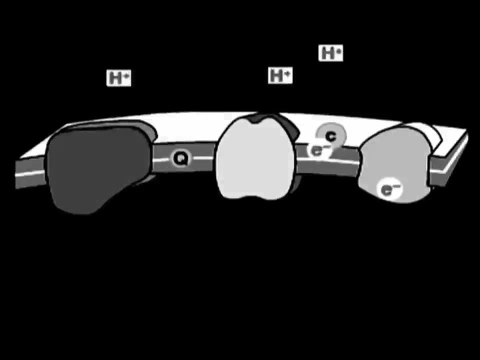 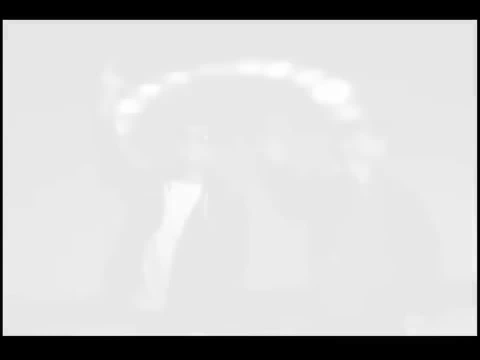 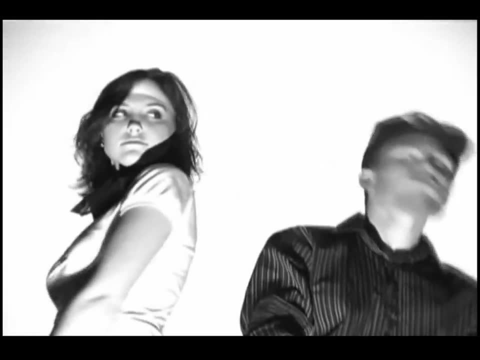 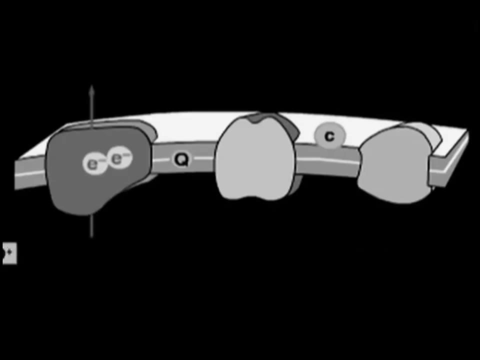 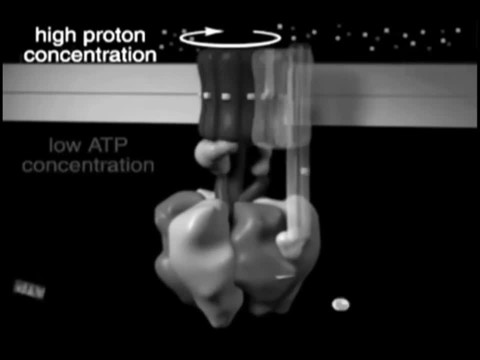 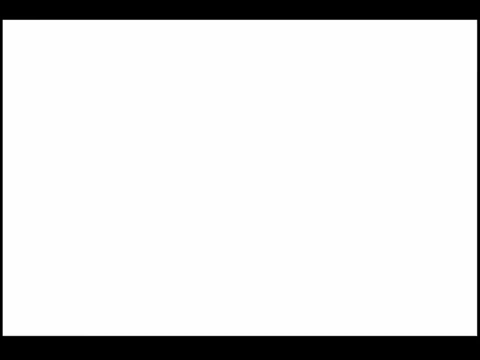 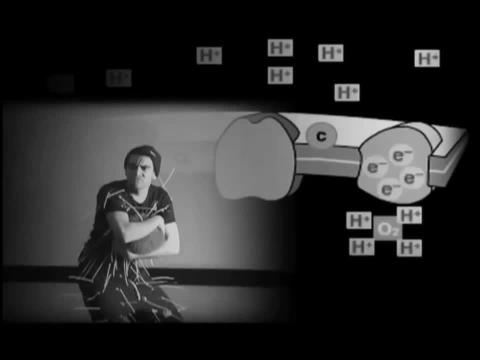 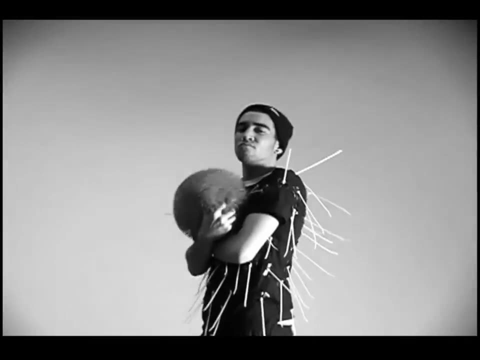 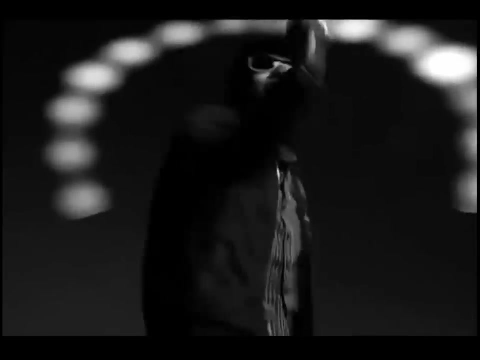 to remove the key and keep it rolling, like Yassi Krebs, making CO2 oxy oxidating. why you think they call it cellular oxygen? your little respiration burning our food to make ATP stack. some oxygen present lectron to the next one: lollipops and tangerines. somebody synthesize some ATPs, so why you? 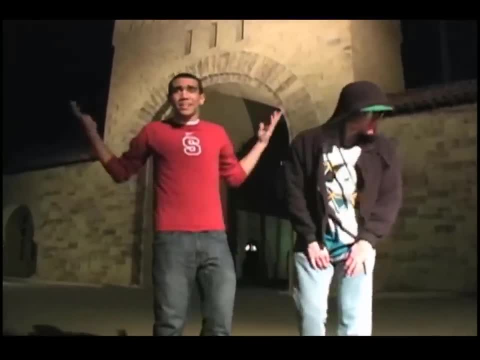 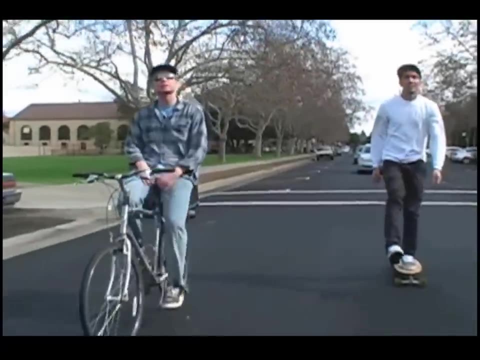 pissed again. what's the point of all these crazy steps? what a mess making ATPs. why you gotta do from blue to pyru, from coays to sedays shoot. why you think we need to breathe. well, adenosine triphosphate's beauty, it ain't hard to tell, helps us sell do. 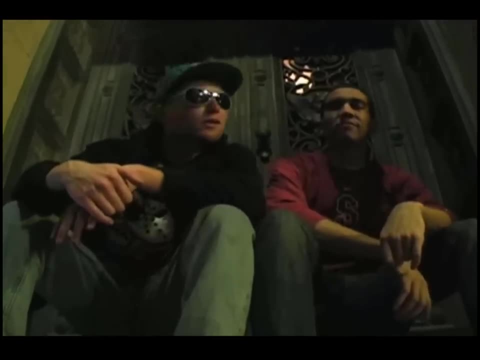 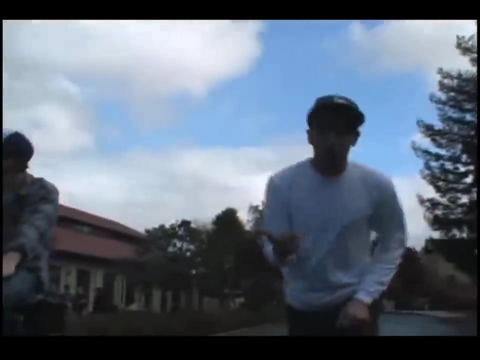 his duty. even Jewie can judge that. it's crucial to me pump sodium and keep myosin moving, which is to say that it's fuel for your brain or your muscles in a tussle- insane. so when you think jerk rum ball, take a test and drop new blows. remember how you. 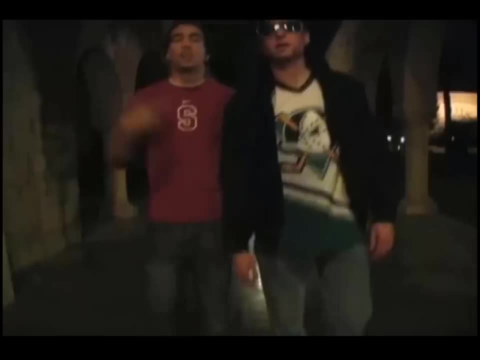 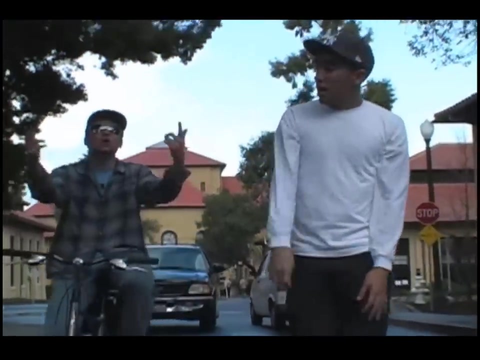 make ATP. how to grade your lovers? psychologists gon' chop glucose down to two, three C-blocks. go ahead, study me, I'll make ATP. and if you eat a burrito, then he gon' get to know me. and if you got enough oxygen in stock, mitochondria will do octopause. go ahead. 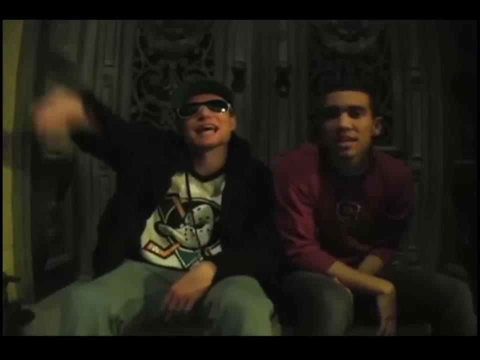 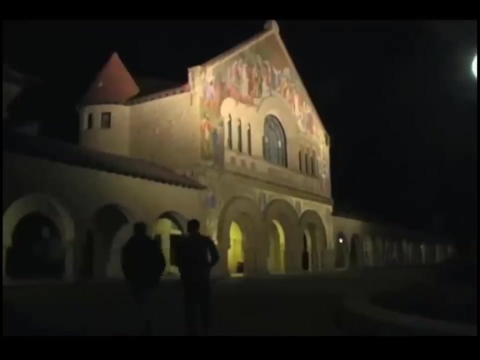 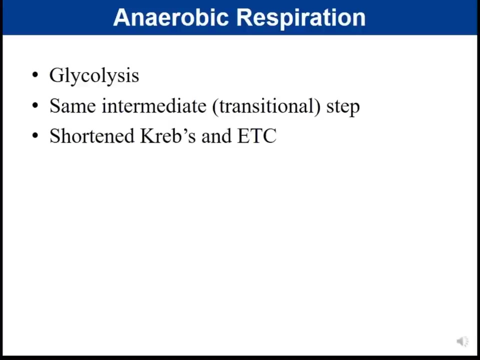 study me, I'll make ATP. I make a hell of a lot, so you should get to know me. So we talked about aerobic respiration. now we need to talk about anaerobic respiration and again anaerobic respiration. 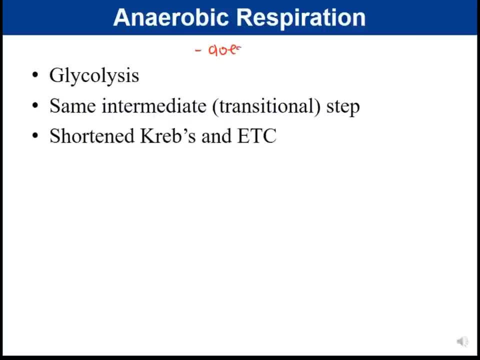 um does does not use O2 as the final electron acceptor. Does use inorganic final electron acceptors- right, so they do use um inorganic final electron acceptors like nitrate, sulfate, carbonate, etc. 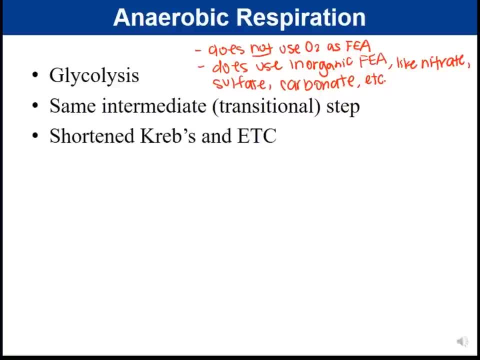 So, when we talk about anaerobic respiration, we still have glycolysis, we still have the same intermediate and transition step um, but we have a slight variation in terms of the Krebs cycle and the electron transport chain. So, while the majority of the process is the same, they're not identical, and so, as 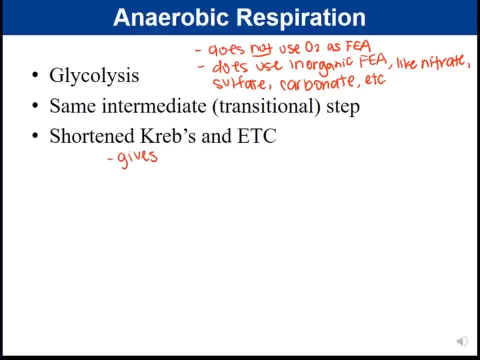 a result gives about 3 to 29 ATP per glucose. So during anaerobic respiration um during anaerobic respiration we get more ATP than fermentation, but we get less than aerobic respiration. So during anaerobic respiration um during anaerobic respiration we get more ATP than fermentation, but we get less than aerobic respiration. 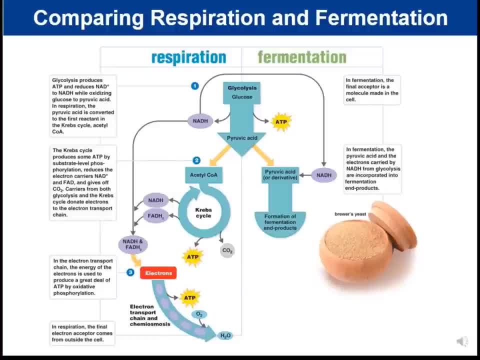 So in anaerobic respiration um during anaerobic respiration we get less than aerobic respiration. So this slide is comparing and contrasting respiration and fermentation, And so in both respiration and fermentation we still go through glycolysis. 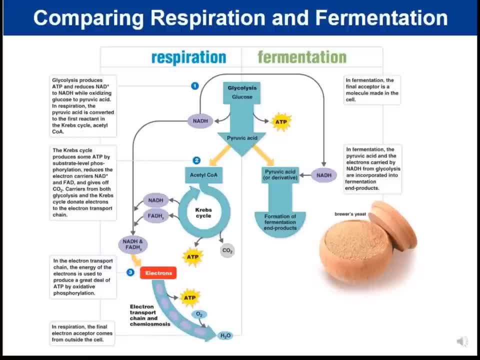 So notice that's right down the middle. that part is the same. So in glycolysis we are going to chop glucose in half to two 3-carbon pyruvates, And when we do that, NAD-plus. 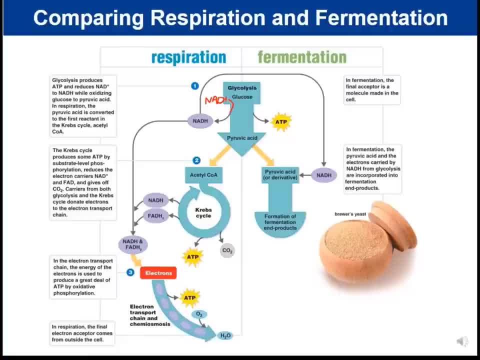 is going to pick up electrons and it's going to form NADH. So during glycolysis we form NADH. We also get a little bit of ATP. We get 2 ATP per glucose. Pyruvate serves as this key juncture. 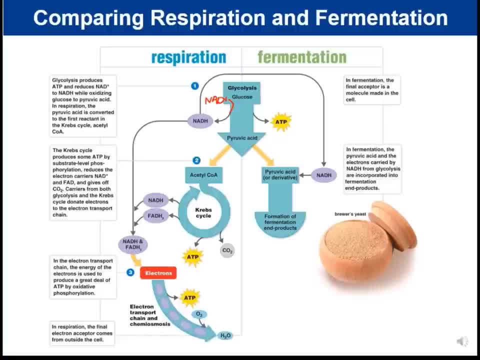 between whether the cell is going to do respiration or fermentation. If O2 is present, we're going to go through the rest of respiration. If there's no O2, the cell can switch over to fermentation. Now, if we look at this process right, So notice, if we look at respiration, 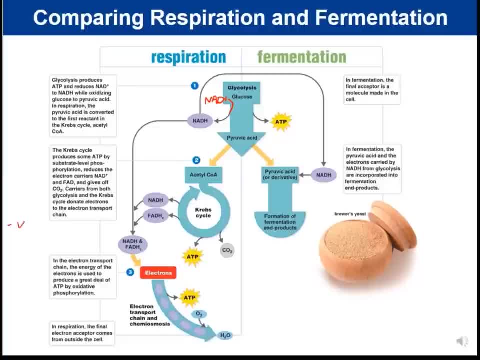 If we use respiration, we use inorganic final electron acceptors, right, So O2, if we're talking about anaerobic, it would be nitrate, sulfate carbonate, etc. Those are all inorganic final electron acceptors and produces inorganic products. 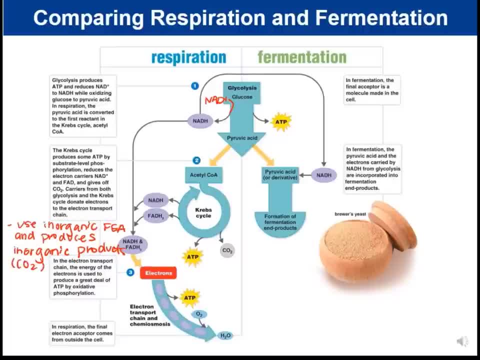 meaning it's going to break the glucose down completely to CO2.. So during respiration we're going to have our Krebs cycle. We have the electron transport chain, We use our inorganic final electron acceptor and we're going to produce inorganic products. 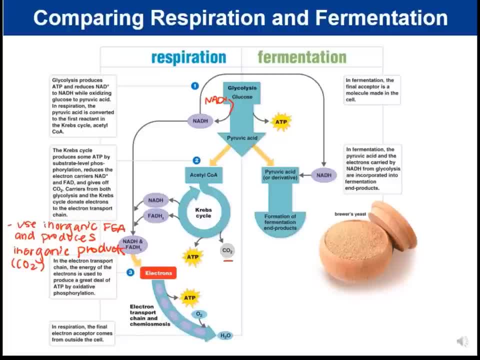 meaning we break it down completely. The sugar is broken down completely to carbon dioxide. Now, in order for respiration to continue- notice that glycolysis in the beginning- We need NAD+ to be able to to take electrons during the process of glycolysis. 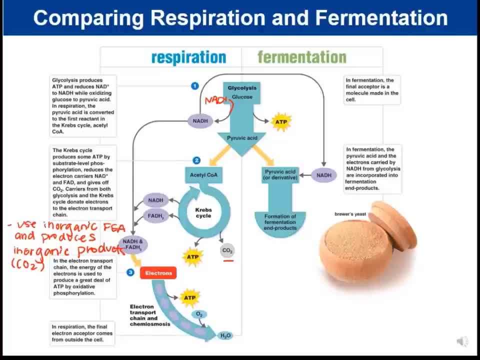 NAD plus is going to pick up electrons and it's going to become NADH. And so I said that all of these early steps are important- not for the ATP that's produced in them, because we get actually very little ATP, But the important thing that's produced during the early steps. 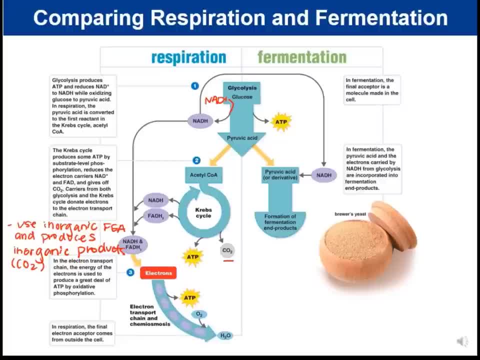 are those electron carriers, And so those electron carriers will go to electron transport chain. they will drop off electrons, And when they drop off electrons, that's going to produce the bulk of the ATP. Now, in order for this process to keep occurring when those electron carriers drop off, 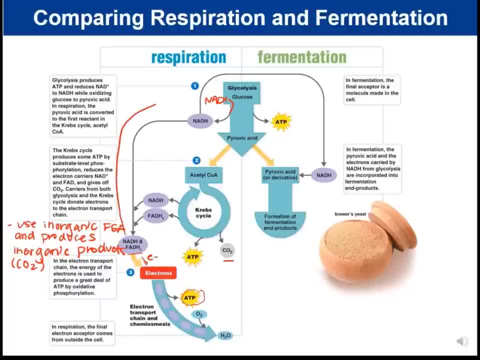 their electrons. they are going to go back right, So they will form the NAD+ or they will form the FAD. So when they drop off electrons, it's back to being NAD+. Now the NAD+ can go back and pick. 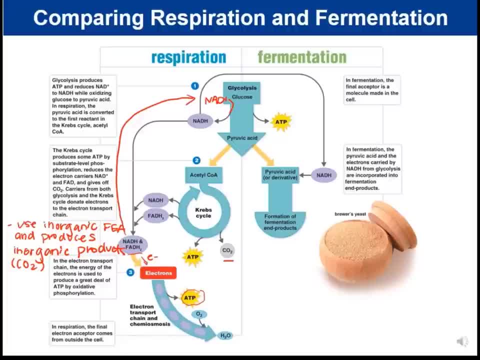 up more electrons, So in respiration, the way that we regenerate the NAD+ to keep this going is that the electron carriers need to be able to drop off electrons at the electron transport chain. So again, if O2 is not available, right. If O2 is not available, then the 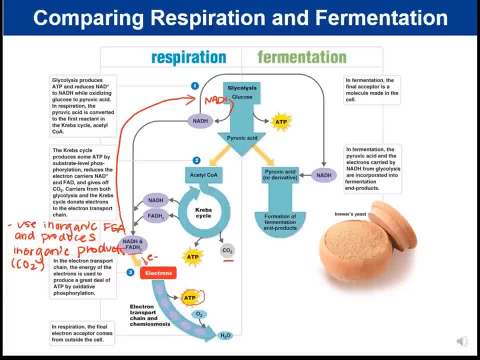 electron carriers need to be able to drop off electrons at the electron transport chain. If the electron transport chain can't go, we can't get ATP and we get this buildup of these reduced electron carriers, meaning we get a lot of NADH and FADH2 in the cell because they can't. 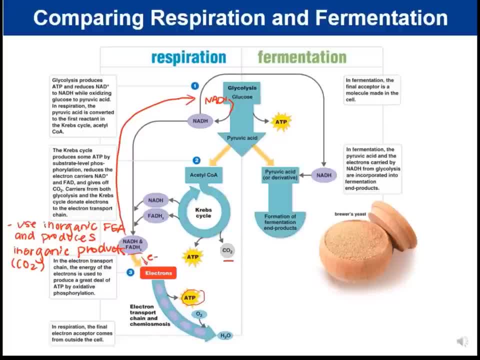 drop off their electrons, We would run out of NAD+. So if we compare that to fermentation, fermentation uses organic final electron acceptors and produces organic products. So fermentation is a little bit different. It uses organic final electron acceptors, either pyruvate, 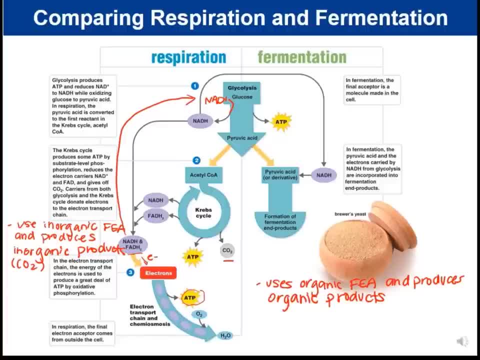 or acetaldehyde, depending on if it's lactic acid fermentation or alcoholic fermentation, But we will use organic final electron acceptors, and we will use organic final electron acceptors and, as a result, we also produce organic products, ethanol or lactic acid. They still have a lot of 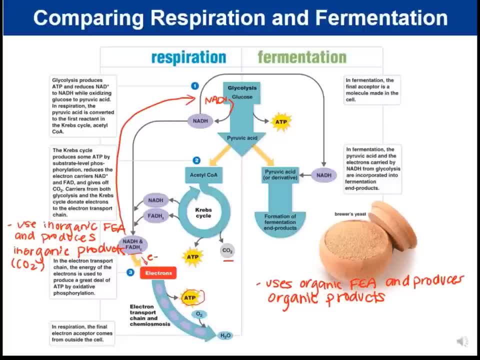 energy left Now during the process of fermentation itself, so meaning going from pyruvate to form lactic acid, that part of the pathway actually doesn't generate ATP. So when we talk about fermentation, the ATP that gets produced actually comes from glycolysis. 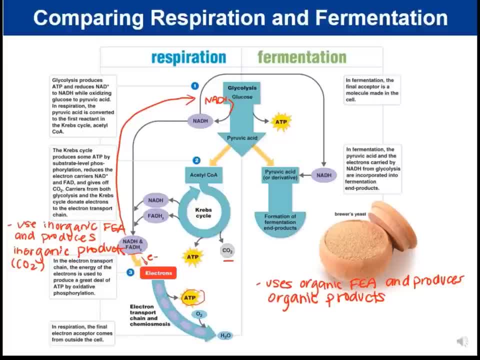 because, no matter which type of sugar metabolism that they do, glycolysis is going to occur. So in fermentation they get their ATP from glycolysis. So if that's true, why do we even have to have the fermentation part? Why do we have to use pyruvate, for example, as the final electron? acceptor And the answer is permutist. So the final electronic acceptor turns out to be the final electronic receptor of glycol. So if we take the final electronic acceptor and put it into the final electronic effector, the final electronic acceptor turns out to be the final electronic acceptor of glycol. 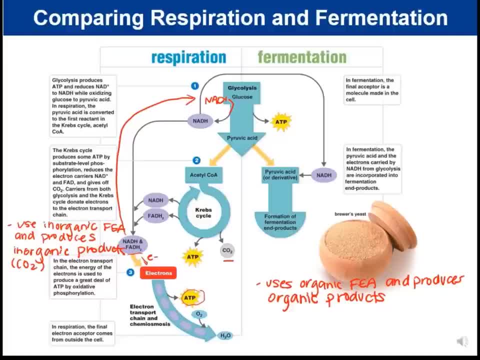 is that, in order for this to occur, notice that in respiration, the NAD plus gets regenerated when the NADH drops off electrons at the electron transport chain. That's how we get back to having NAD plus, so that this process can keep continuing. In fermentation we don't have an electron. 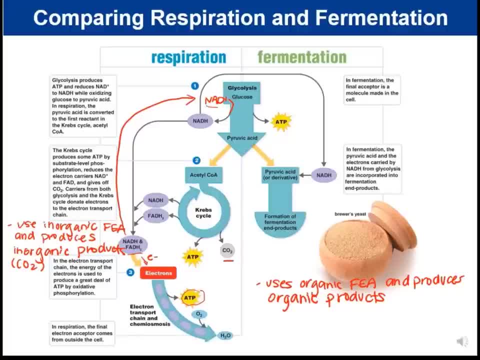 transport chain, so we can't use that method to regenerate the NAD plus. So, in terms of fermentation, the purpose of fermentation is to generate ATP- and the key here- and regenerate NAD plus. NAD plus needs to be produced so that glycolysis can keep happening. 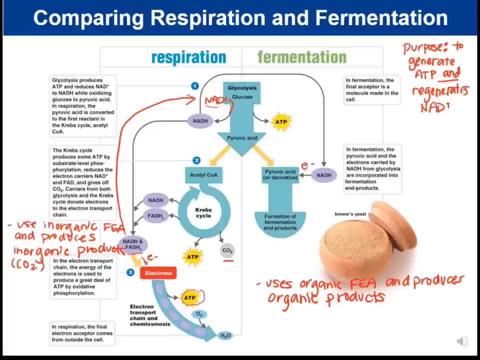 So NADH is going to drop off electrons to pyruvate and when it does that it forms the NAD plus. And then now the NAD plus can go back and can be used in glycolysis so that at least glycolysis can continue, so that we can get the ATP during glycolysis. 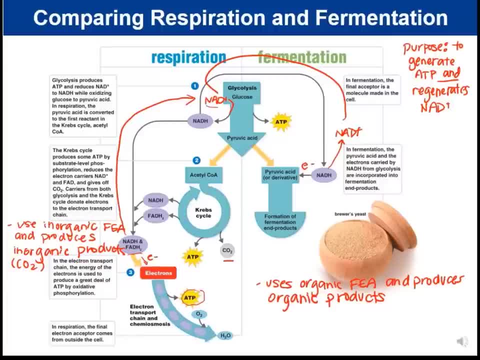 So when we talk about fermentation, again, you want to see the big picture. What is the point of doing this? And the point is is that if O2 is not available and the organism is not doing an electron transport, then it's going to be used to generate ATP. And so when we talk about fermentation, 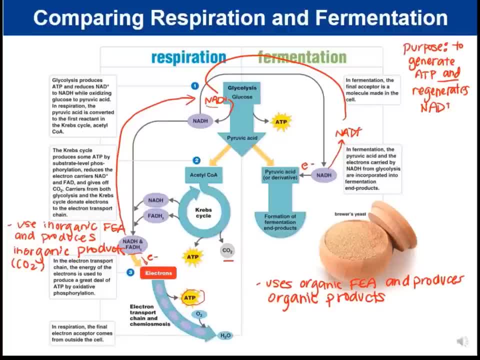 transport chain, they still need to be able to do glycolysis to get their ATP, And so, in order to keep glycolysis going, we need a way to regenerate NAD+, And so, again, the way that we do that is that we use organic final electron acceptors, like 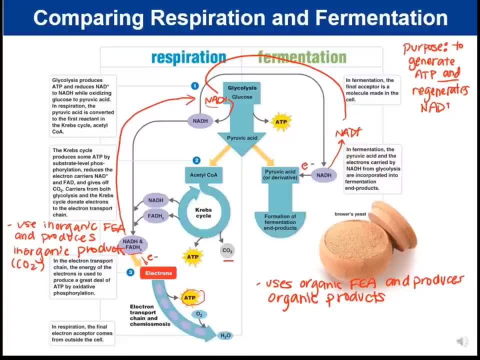 pyruvate like acetaldehyde and we're going to use those organic products to take the electrons so that NADH can go back to being NAD+ and NAD+ can go back to glycolysis and pick up more electrons so that at least glycolysis can occur and at least we can. 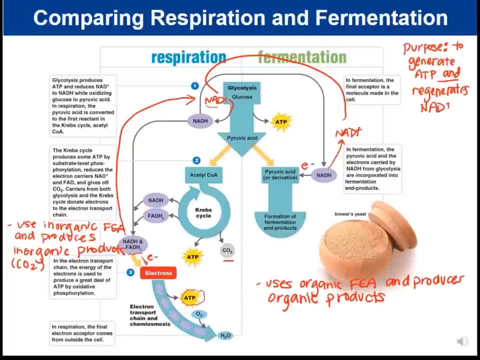 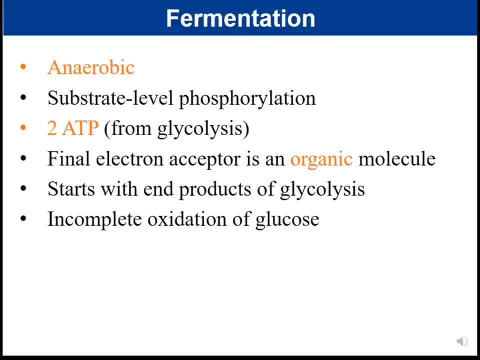 get some ATP during this process. It's not much, it's only two ATP per glucose- but it works well enough for slow growing organisms. So now we're going to move on and we're going to talk about fermentation. So fermentation. 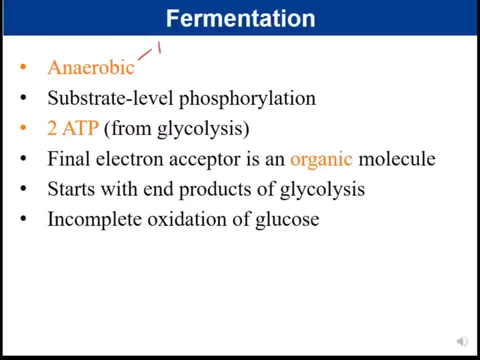 Fermentation is an anaerobic process, but is not anaerobic respiration, And so, again, there's a key distinction. You'll see this online, you'll see this in some books, where they call fermentation anaerobic respiration. 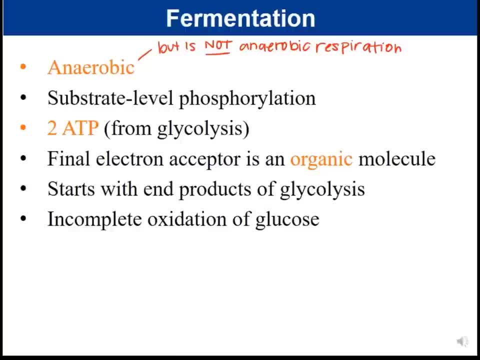 That is incorrect And the reason is is that in fermentation, fermentation is using a final electron acceptor that is organic and produces organic products. That's different than in anaerobic respiration. Anaerobic respiration breaks down the glucose completely to inorganic products like carbon. 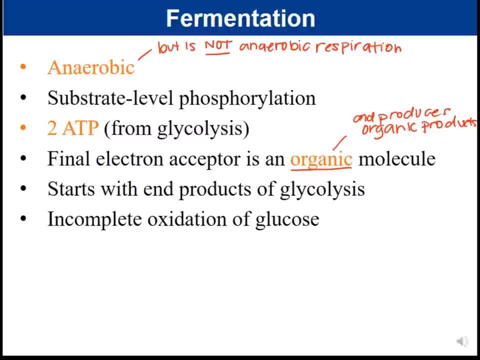 dioxide And in anaerobic respiration we have an electron transport chain and we also have in the case of anaerobic respiration, the final electron acceptor is NADH. So the final electron acceptor is NADH. 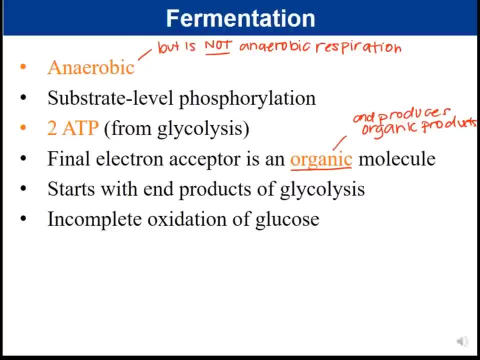 And that's one thing we're going to talk about later- is inorganic. But again, in fermentation the final electron acceptor is organic. So again, make sure that you don't get tripped up on fermentation and anaerobic respiration. They're. 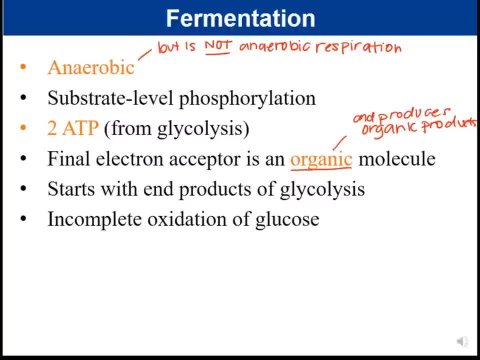 totally different processes. In the case of fermentation, we get two ATP, and those two ATPs come from glycolysis, And so the ATP produced during glycolysis comes from substrate level phosphorylation. So again, it's simply going to be that during glycolysis a substrate has a 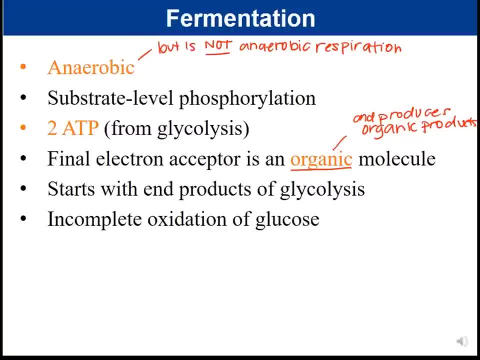 phosphate and it's going to transfer it onto ADP, forming ATP. So fermentation is going to use our substrate level, phosphorylation. The fermentation itself starts with the end products of glycolysis, meaning that it starts with pyruvate. So it starts with the pyruvate. 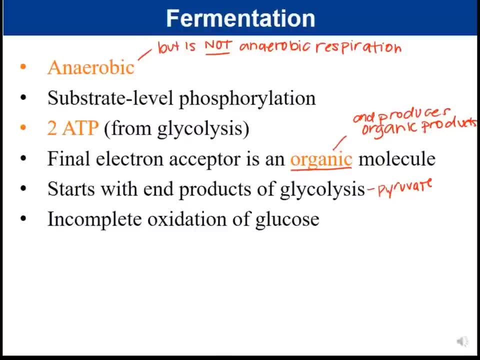 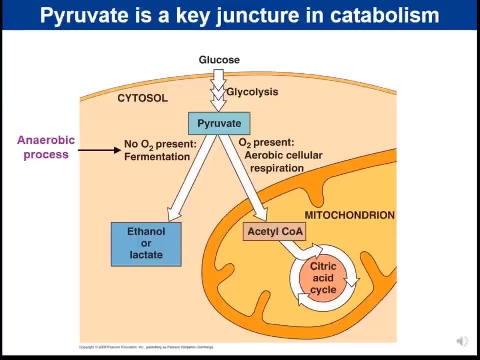 And again during fermentation, we get incomplete oxidation of glucose, meaning that the glucose is not broken down fully And we end up with organic products. They still have a lot of energy left, So pyruvate serves as the key juncture. 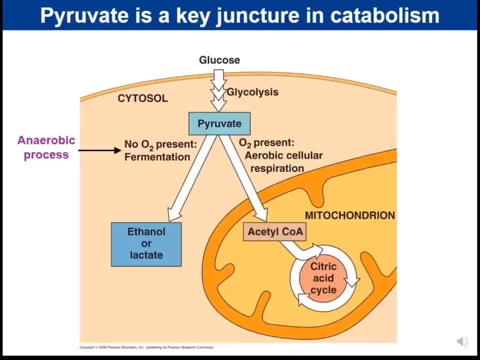 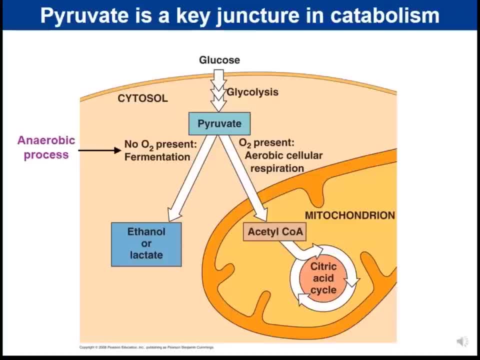 If O2 is present, pyruvate will get transferred into the mitochondria. It will go through the transition step, It'll go through the citric acid cycle step, It will go through an electron transport chain And again the purpose is in this case right. So to do acetyl-CoA and the 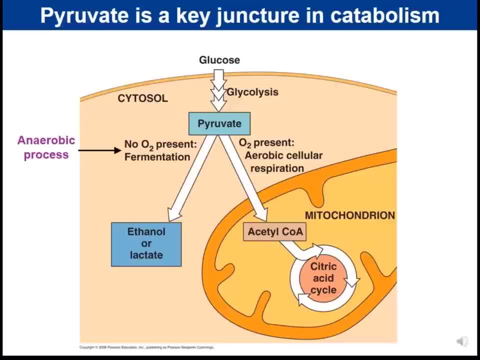 Krebs cycle, you need to have O2. Because in order to do the electron transport chain, you need O2 to be the final electron acceptor. If O2 is available, pyruvate will go into the mitochondria. However, if O2 is not available, 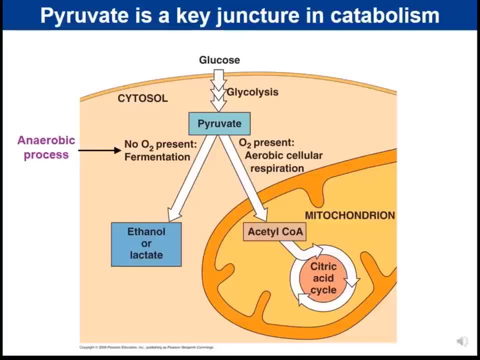 right. if O2 is not present, then the cell is not going to transport the pyruvate into the mitochondria, Because without O2, the electron transport chain can't occur. So in that case, if there's no O2 present, the organism is going to switch to fermentation, And fermentation is 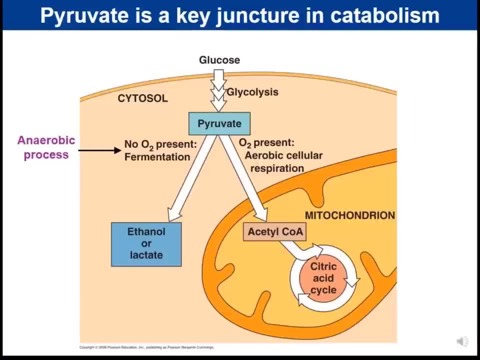 going to be an anaerobic process. So if O2 is not present, then the cell is not going to transport the Teflonuren in the mitochondria And in that case this will not be a process. Again, it does not. 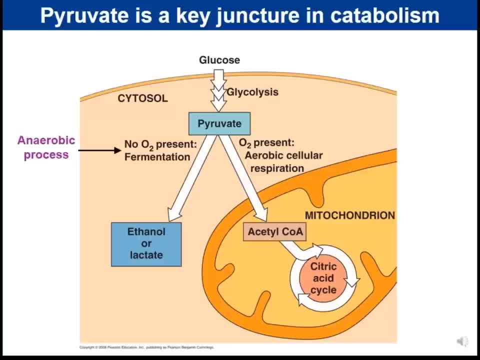 mean it's anaerobic respiration, But it will switch to fermentation, which is an anaerobic process, And so what's going to happen is that, in fermentation, the pyruvate itself can act as the final electron acceptor. if we're talking about lactate, as the product hobby vet can be. converted to acetaldehyde. Acetaldehyde acts as the final electron acceptor And then from there the Lactate can also also be converted to benothorin and phenoli, which is a pattern of the contact pathologies, And it will be linked to the concentration of nitrate, and then from there we'll go into the 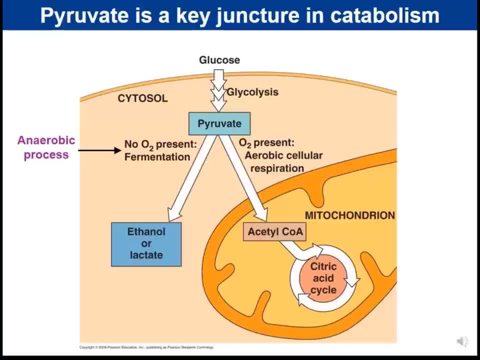 process In that example simply talked about this exercise. a small ethanol Watson universe is acts as the final electron acceptor and it produces ethanol. So pyruvate is kind of this key decision between whether the cell will do aerobic cellular respiration or whether it will. 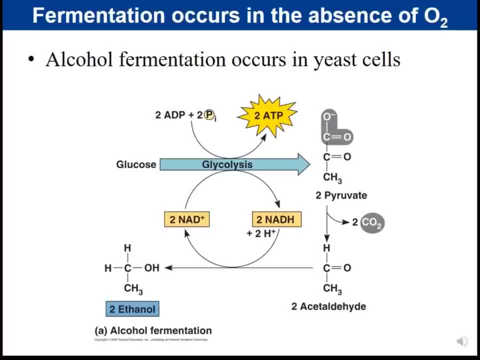 do fermentation. So we're going to look at the types of fermentation, And the first type of fermentation that we're going to talk about is our alcoholic fermentation, And alcoholic fermentation occurs in yeast cells like Saccharomyces cerevisiae. It's also used by some bacteria. 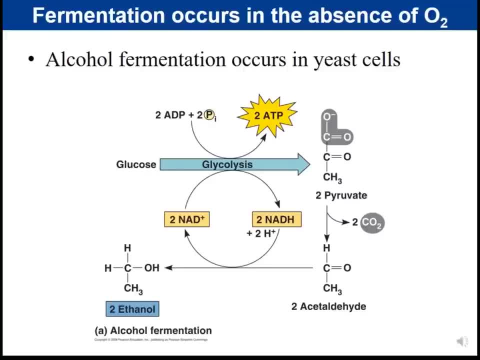 And so the way that this works is that we still have glycolysis, And notice, here's my glycolysis. Glucose is going to get broken down into that three-carbon pyruvate right, Glyco sugar lysis breaking. When we break down the glucose, electrons are going to be transferred onto an. 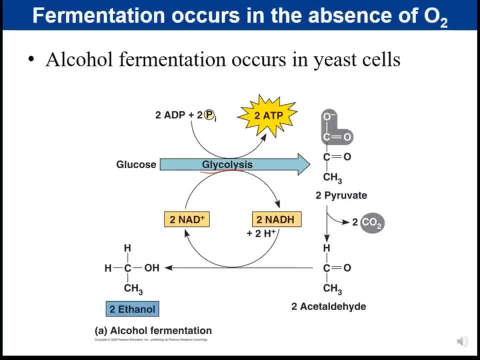 electron carrier. So NAD plus is going to take electrons and it's going to form NADH during glycolysis. We also get a net gain of ATP of 2ATP per glucose during glycolysis And again the purpose of doing. 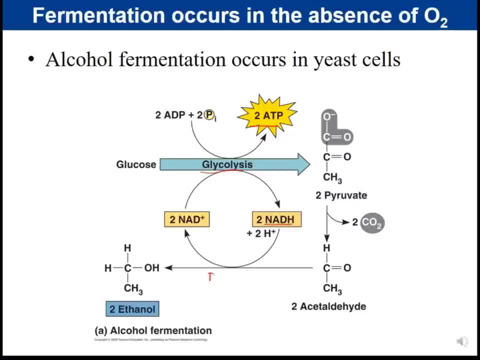 fermentation. So purpose: Regenerate Whoops. Regenerate To regenerate NAD plus, And so what ends up happening is is that pyruvate is going to break off a carbon and we get carbon dioxide. This remaining two-carbon molecule is called. 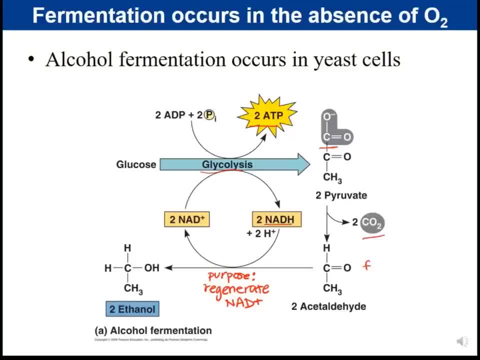 acetaldehyde. Acetaldehyde is going to be our final electron Acceptor. It's what's going to take the electrons from the NADH. So during the fermentation part, acetaldehyde is going to accept the electrons, right? So this NADH is going to donate electrons. 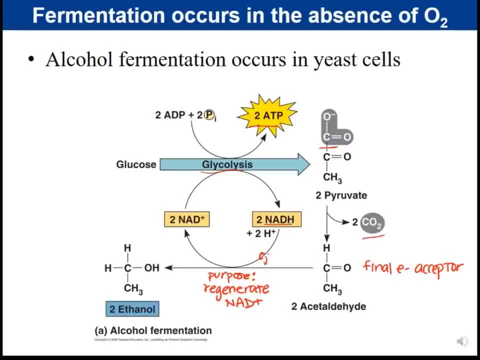 to the acetaldehyde And when it donates its electrons it goes back to being NAD plus. right, Because it's losing its passengers. So it's back to being NAD plus. And so when it's getting that electron, when it's low, Make the silicon breathing. family members is going. 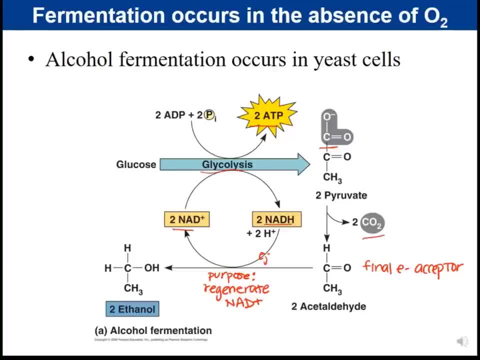 that NAD plus And then that NAD, NAD plus can go back and do glycolysis so that at least the cell can make two ATP per glucose, So that scallop can make two ATPs per glucose. The product during this process is going to be alcohol, ethanol. 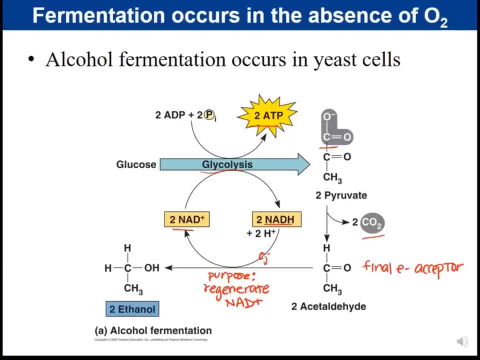 So this is our product. Notice that my product is organic Because it Carbon and hydrogen. my final electron acceptor was organic. The NAD Acceptor Was Organic. organic because it had carbon and hydrogen. So we end up with an organic product and we have an organic final electron acceptor. 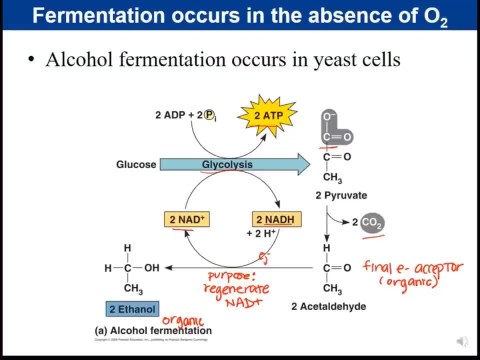 And so this is what fermentation looks like. There's no electron transport chain- that's why it's not called respiration- and the purpose is that we need to regenerate the NAD+. That's the main purpose, because we need to keep the NAD-plus coming, so that at least 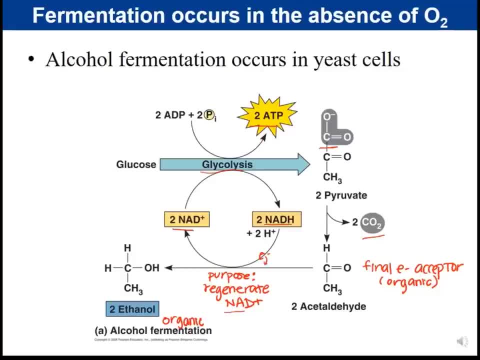 the cell can continue to do glycolysis and make ATP, Because you can imagine that if you don't regenerate NAD-plus, normally during respiration the NADH drops off electrons at the electron transport chain and that's what allows the NAD-plus to be regenerated. 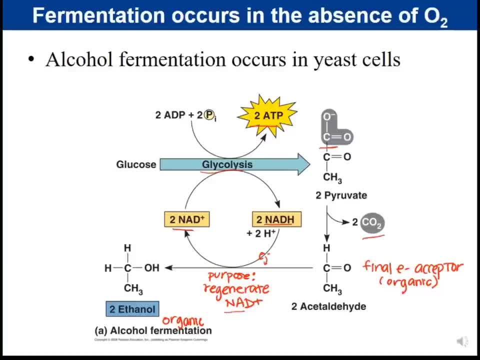 If, however, we don't have an electron transport chain because there is no oxygen, if we were just doing glycolysis to get ATP and that was it, that's a problem, Because, as the cell continues to do glycolysis, it's going to keep producing NADH, but not. 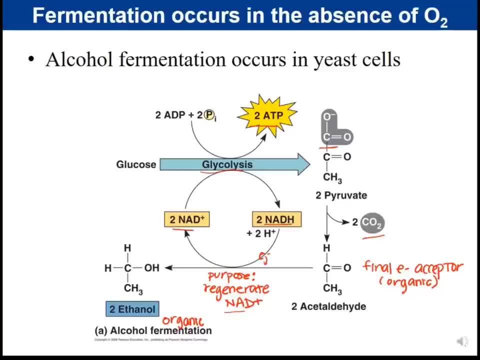 having any more empty NAD-plus, because all the NAD-plus is being utilized to form the NADH during glycolysis. So in fermentation we need to regenerate the NAD-plus. That's pretty much the goal of fermentation, because without oxygen we're not using an. 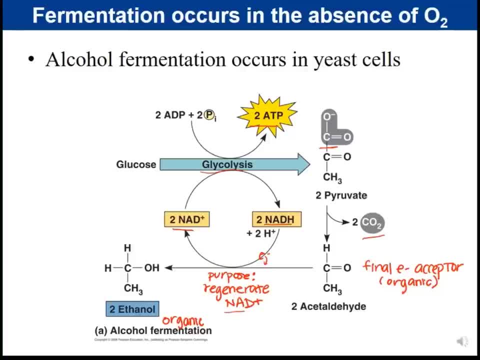 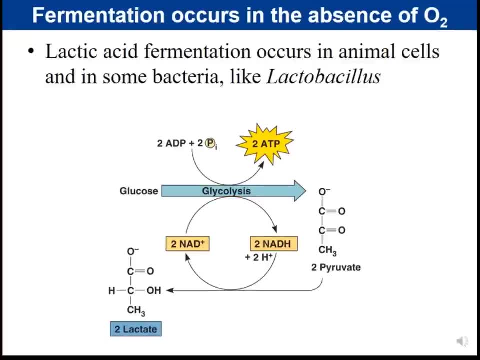 electron transport chain. So cells have to have an alternate way to regenerate the NAD-plus so that at least glycolysis can continue to occur. So the next type of fermentation that we're going to talk about is going to be our lactic acid fermentation. 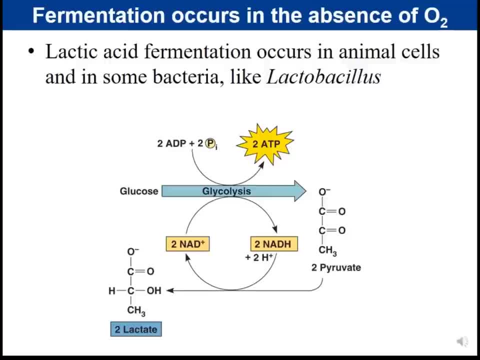 And lactic acid fermentation. Glycolysis occurs in animal cells, in the muscles for example, and in some bacteria like lactobacillus, which is used to make yogurt. So these organisms have a different set of enzymes to do a different type of metabolism. 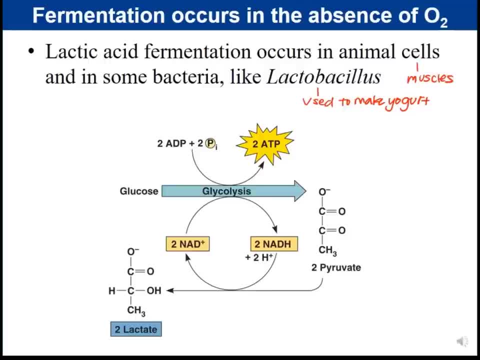 And so they're able to do lactic acid fermentation. So again, we still have glycolysis And glycolysis. again Glycolysis, Glycolysis, Glycolysis: We're going to break down glucose into the two three-carbon pyruvates. 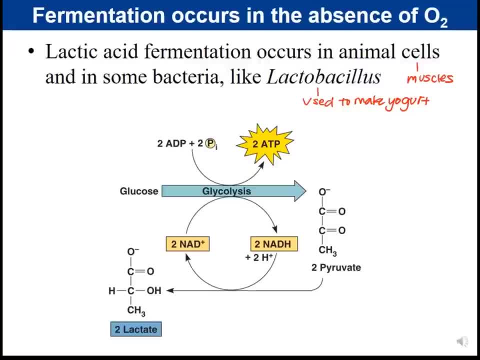 That process is also going to transfer electrons onto NAD-plus and we get NADH. We also get 2 ATP by this process. Again, goal of fermentation: regenerate the NAD-plus, And so in this process, pyruvate acts as the final electron acceptor. 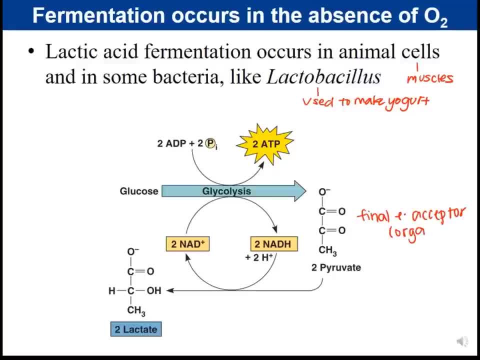 Again, it's organic, And so pyruvate itself is going to be our final electron acceptor, And so when it takes the electrons right and it becomes reduced, it's going to form lactate, otherwise known as lactic acid. 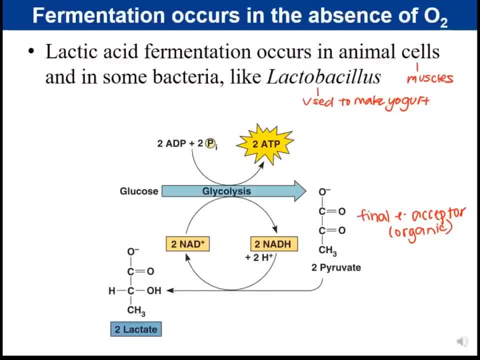 Now lactic acid you might hear about for a specific reason if you think of like being an athlete and working out or playing sports. Now lactic acid is thought to be. although there is some debate, lactic acid is thought to be responsible for the reason why your muscles burn after a hard workout. 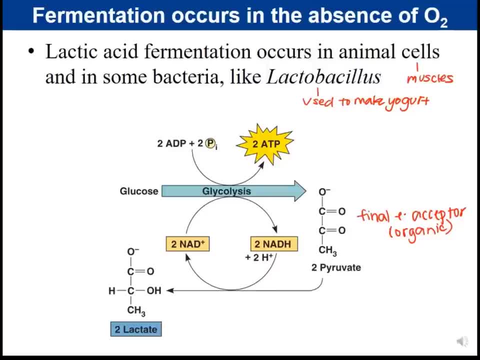 And that's because, if you think about it right, if I'm exercising really hard, if I'm doing a lot of cardio, and I'm exercising really hard and I'm breathing heavy, if I'm breathing heavy I might not be getting enough oxygen to my tissues. 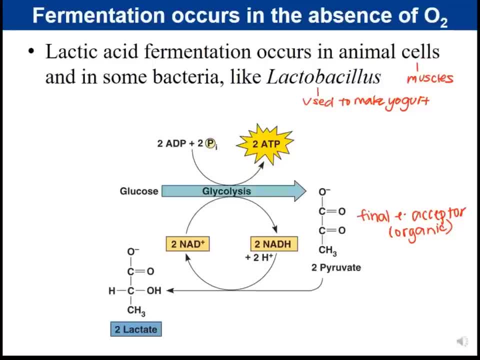 And so muscle cells need ATP in order for the muscle cells to contract, because they need to hydrolyze ATP for muscle contraction. So if those muscle cells are not getting any oxygen, then those muscle cells are going to switch to fermentation, at least in the short term. 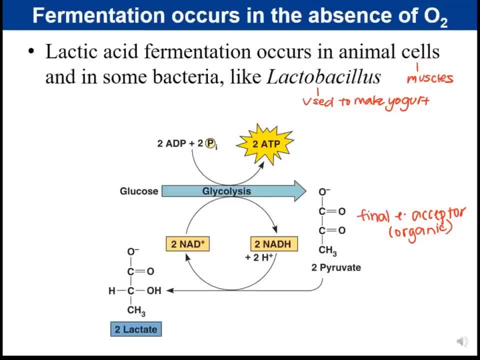 And when they switch to fermentation, they produce lactic acid. Now, this is not the case. This is not the case That lactic acid could build up in the muscle cells and that might be why muscles burn after a hard workout. Now, if you think about it, does that last forever? 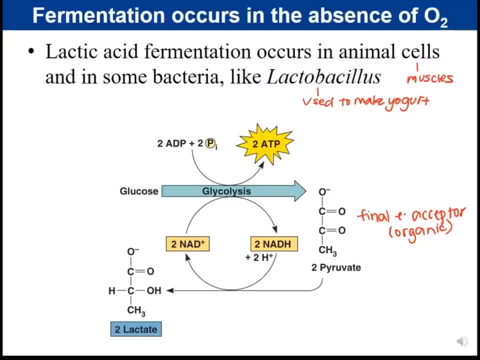 Do your muscles permanently burn like that? No, because that lactic acid is still energy rich, still has some energy in it and it can be put back into metabolism and broken down further, And then that muscle burn will subside. And so again, the purpose of fermentation is to regenerate the NAD+ so that at least 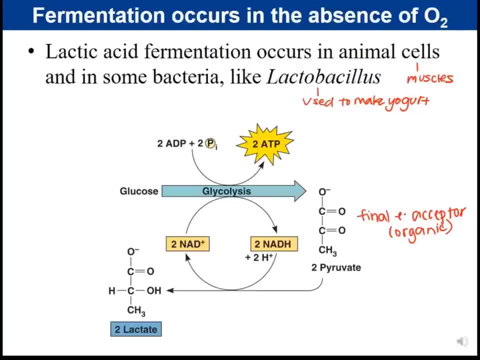 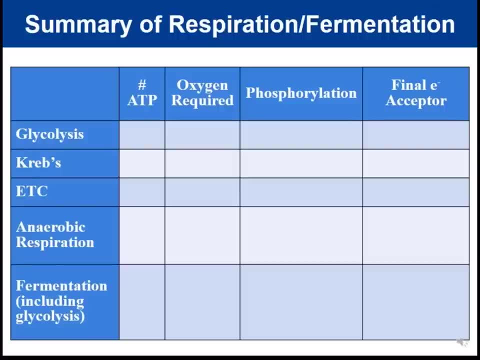 glycolysis can continue and we can at least get to ATP during this process. So this is just a slide summarizing respiration and fermentation, And so what I'm going to do is I'm going to explain to you what I'm looking for in this. 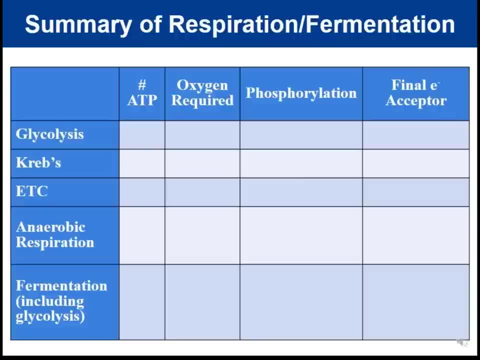 table. Okay, And I'm going to actually have you do this as a participation assignment. So I will go into Canvas and I will change one of the participation assignments to be a submission. You can either print this slide and fill it in or you can draw your own table on a separate. 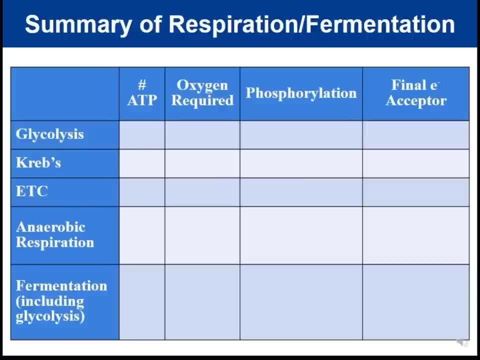 sheet of paper And then you're just going to upload your filled in table into Canvas, so into that assignment, Just like you guys are doing for your parasite video, for example. right, You're filling out the questions and then you're uploading them into Canvas. 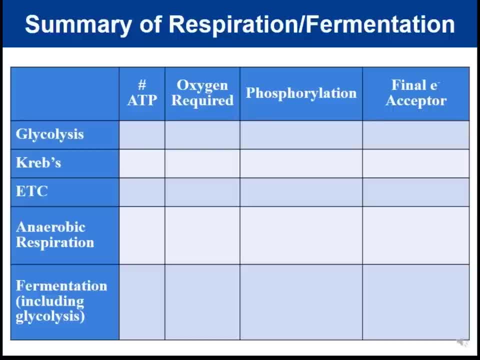 Same idea for this. This is going to count, though, as a class participation, So when the due date closes for this, then I will post the answers so that you're studying the right material. So what we're looking for in this table is we are looking at how many ATP are produced. 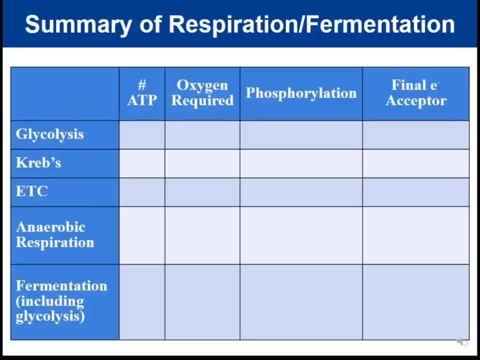 So in glycolysis. So we'll walk through this together for the first row. In glycolysis, how many ATP do we get? And the answer is two. We get two. ATP Is O2, is oxygen required for glycolysis to happen? 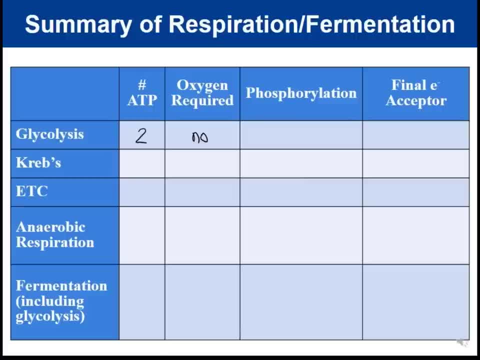 No, And that's because glycolysis happens, whether we're talking about aerobic respiration, anaerobic respiration and fermentation, Okay, Okay. So phosphorylation is basically how ATP is made. So what is the mechanism that ATP gets made during that step? 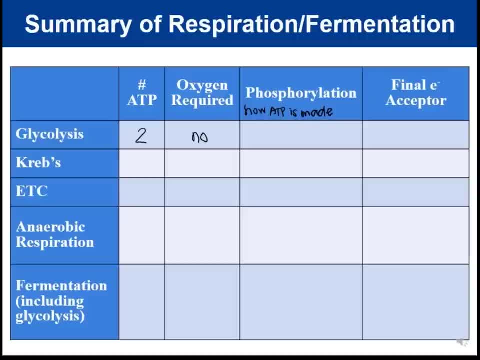 So, if we're talking about glycolysis, what is the method that ATP gets produced during glycolysis? And that is, it's produced by substrate level four, Okay, Okay, So substrate level phosphorylation. So the method that it's using is substrate level phosphorylation. 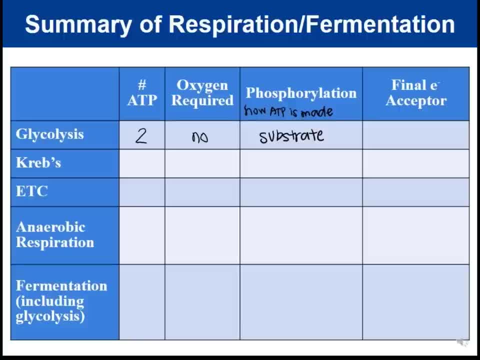 In terms of final electron acceptor. there's a couple ways that you could interpret this. You could interpret this that there is no final electron acceptor in glycolysis because it's going to keep going to later steps, or you could interpret this as what is taking. 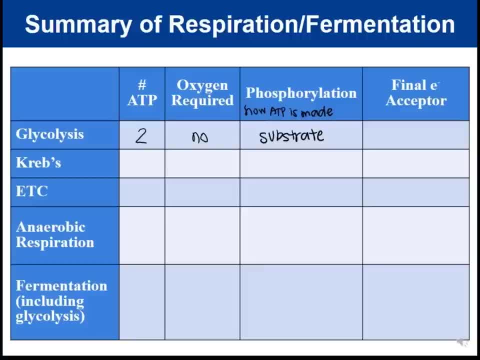 the electrons during this step. So if I'm interpreting this as what is taking the electrons during this step? what is accepting those electrons? that's going to be the NAD plus and it's going to form NADH. So the electrons from the food are going to get transferred on to NAD plus and it's going 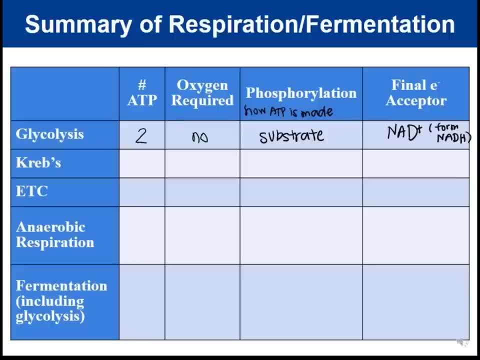 to form our NADH. Okay, So we get our NADH from this process and that's what is taking. so the NAD plus is what's taking the electrons during this step. So you're going to fill in this table, the rest of this table, for your participation.